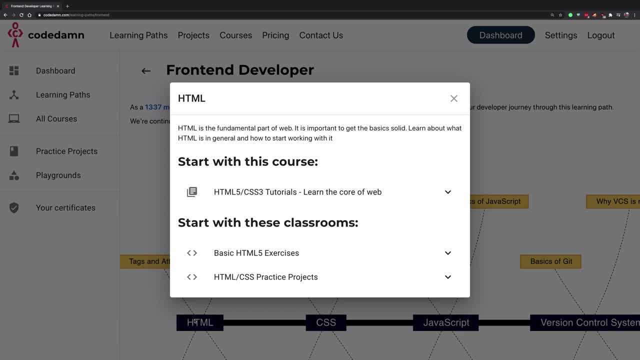 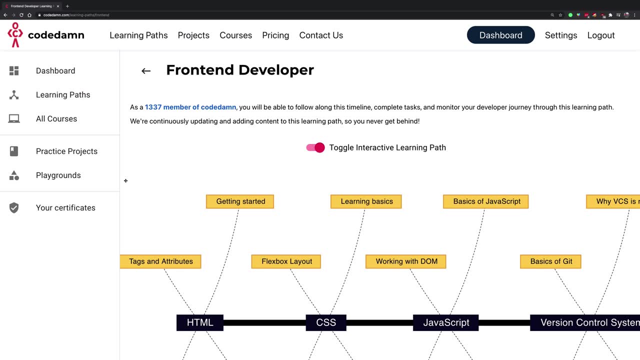 just complete the basics one, because that will just get you started with coding, And in this one we'll just discuss a lot of things which you would probably not really find anywhere else as a video series or as a video tutorial. So, yeah, pay close attention to this course. 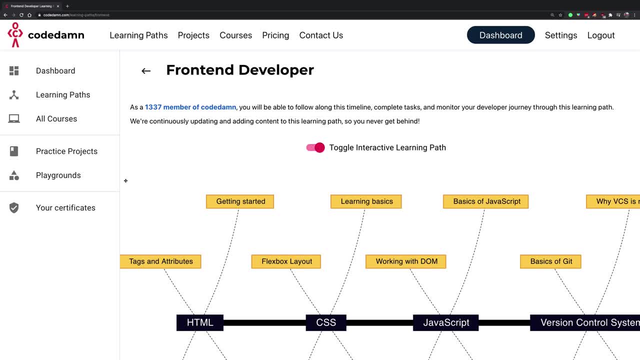 it's going to be a lot of fun and a lot of learning if you just follow along with whatever material is given. So that is all for this video. Hope to see you very soon in the next one. Hey, everyone, welcome back In this video. let's just go ahead and first of all discuss what HTML5. 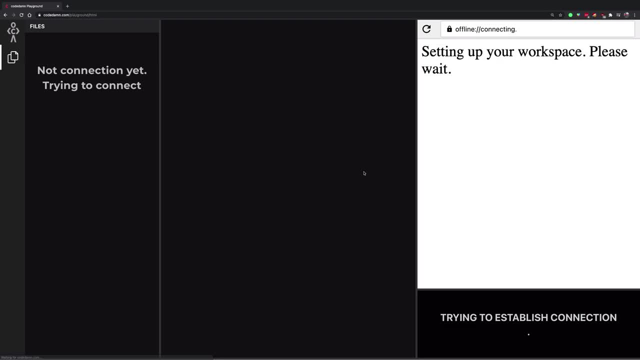 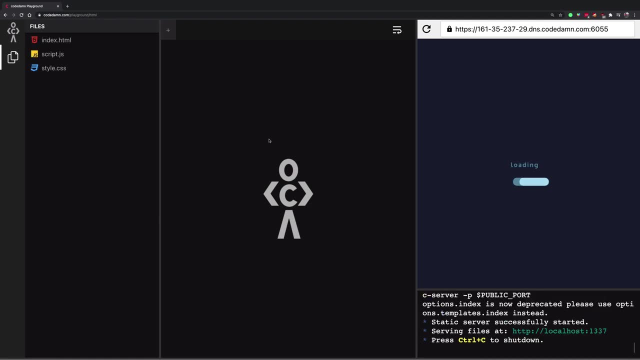 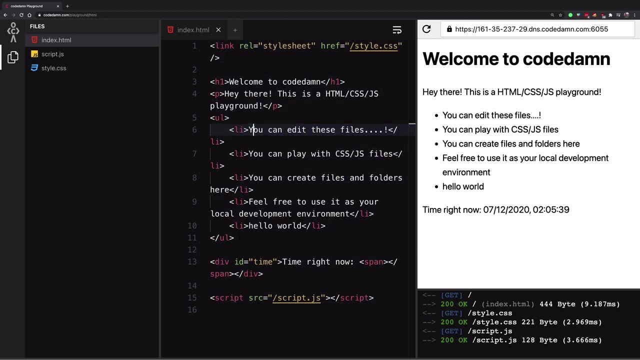 exactly is. So I'm going to go to playgrounds and open an HTML5 playground right here, which is going to give me access to my own little environment where I can just play around with HTML and CSS for the most part. So let's open the indexhtml file And you can see we already have some contents from this file. 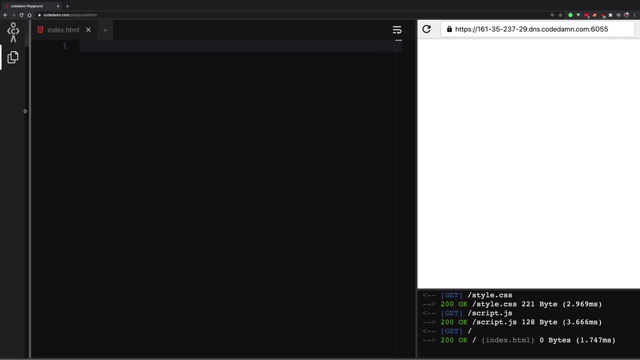 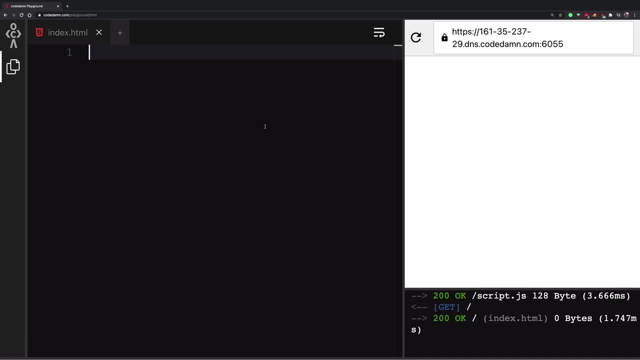 So let's just go ahead and remove this and start from a clean slate. I'm also going to just get rid of this so that we have more space with us for the IDE, All right, So first things first. what is HTML5?? Now, we have already discussed HTML in depth, and you know all those things like simple tags. 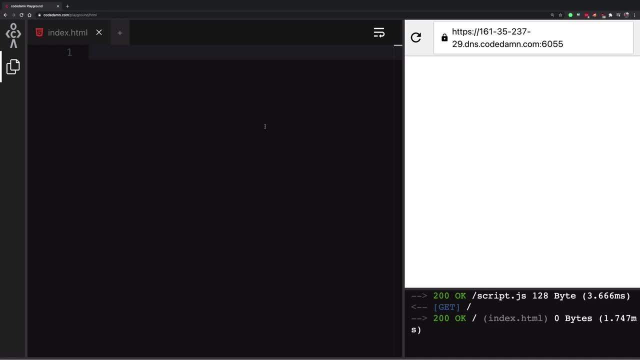 and all that stuff, But if you think about it, HTML comes with a number in front of it, right? Why that is a number? HTML5.. This five is the fifth sort of version of HTML specification, right? So what you have to understand is that there are certain people who are responsible. 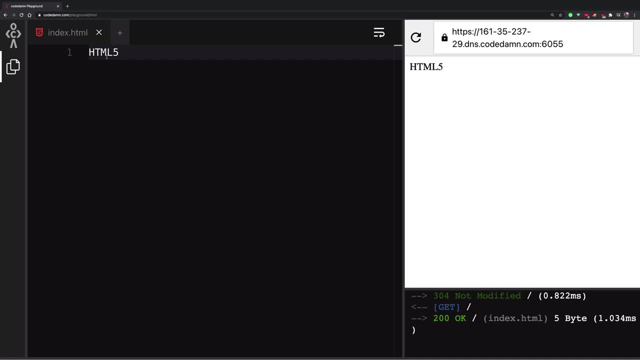 for you know, just just sort of designing the spec of HTML, like what exactly HTML should consist of all these, you know, inbuilt tags, the P tag, the span tag, the div tag, which you see, this has been thought of and created by somebody, right. So these people, this is a community of. 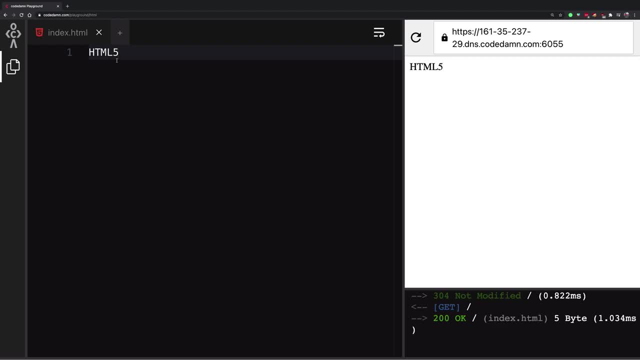 people. these people sit down and when they think that you know there's an update necessary, or we should take browsers to the next level, or you know whatever they think, they have to draft out a new specification. This specification is just a document which browsers like Google Chrome. 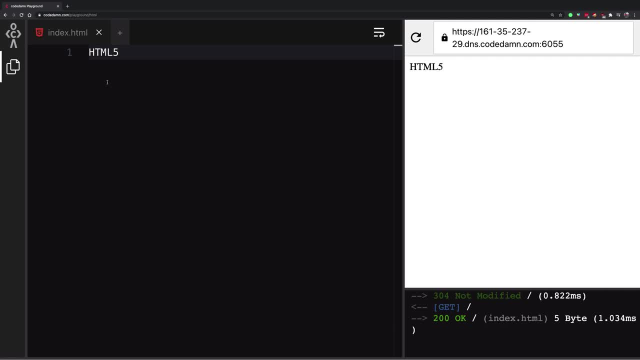 and Firefox and Safari and all other browsers have to follow right Now. specification just lays down that you know, this should be the tag, this should have this behavior, this should be this behavior, But it does not tell them. you know, it does not really contain. 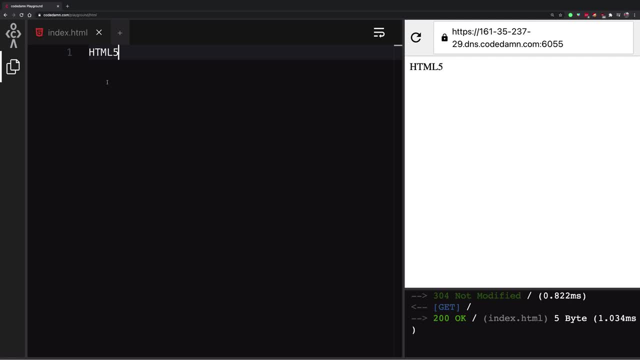 any code or anything, right? So it's just a specification, right? So if you are cooking a recipe, you just get the recipe. you don't really get the ingredients and all that stuff you do, you have to do it yourself. Similarly, this community is just responsible for drafting. 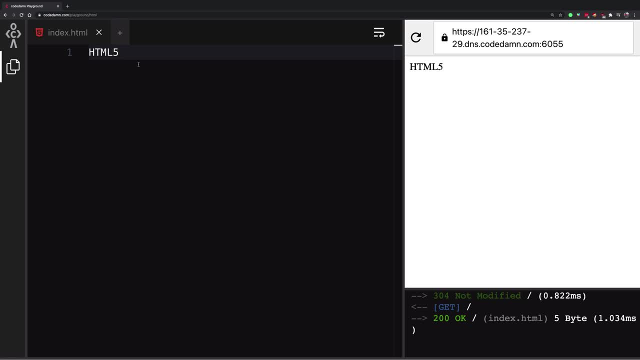 out a specification and then the browsers have to follow and implement them. So what exactly is HTML5?? HTML5 is the revision of HTML 4.1. So the last version of HTML before HTML5 was HTML 4.1, which had certain tags, certain things. here and there there were some changes. 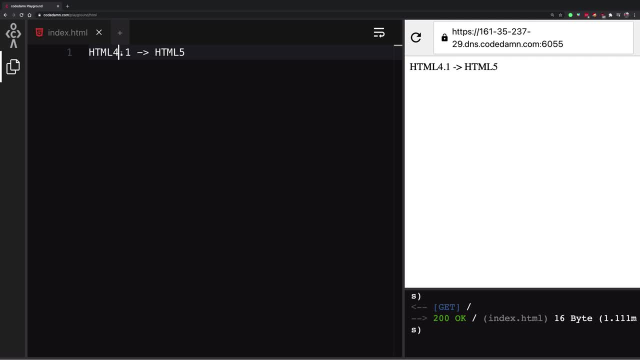 but for the most part it is not really necessary for you on day to day basis to know you know things and differences between HTML 4.1 and 5.. All you have to remember is that in HTML 5, you have to start the doc type like this: that's it. HTML 4.1 had a weird doc type: HTML. 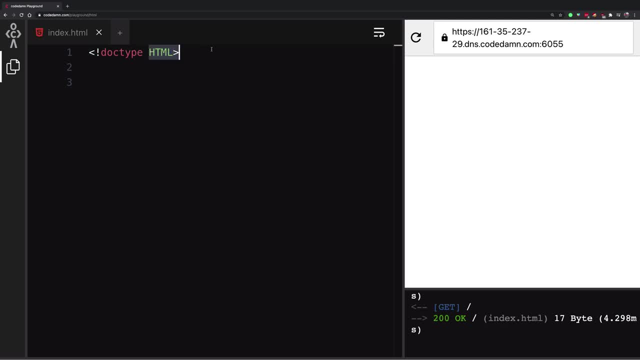 which was huge, and you have to probably copy paste it all the time from your older projects or from other websites. And the next thing you have to sort of remember is that there is a little bit of semantics change in HTML 5, right? So by semantics change, what I mean is that there are 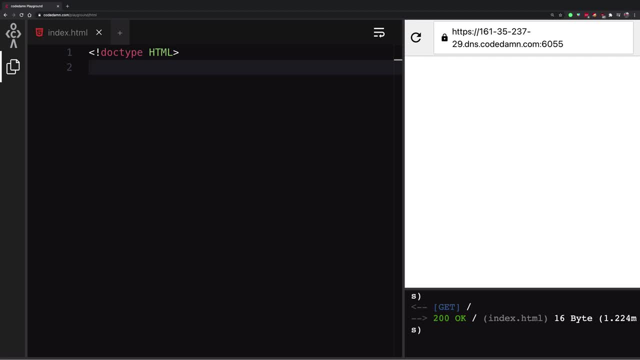 certain more things you have to like be sure of if you want to pass all the accessibility and all the HTML 5 validator test. But for the most part you don't really have to worry a lot about other stuff, right? So in a nutshell, HTML 5, first of all, brings a lot of 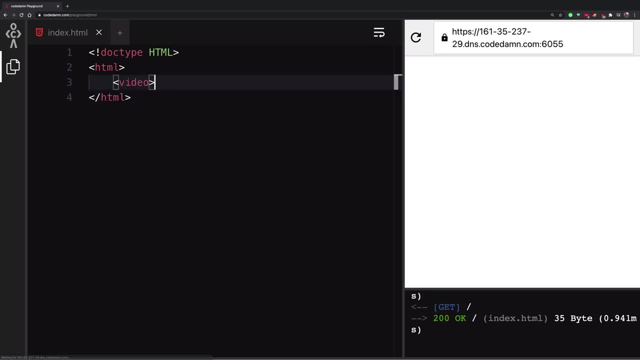 new support to browser in terms of, you know, video tags, embedding videos and audio tags, And we'll also take a look at canvas later on when we are doing JavaScript things. So these things, these are new tags which have special 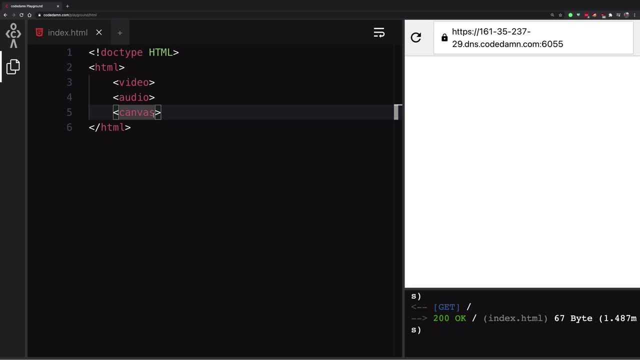 sort of functionality, right, And these are like very limited tags in HTML. Once you realize that most of the stuff, most of the HTML tags- like you can see, p, span, div- all these tags you can just manipulate using CSS and they'll just behave like any other tag. 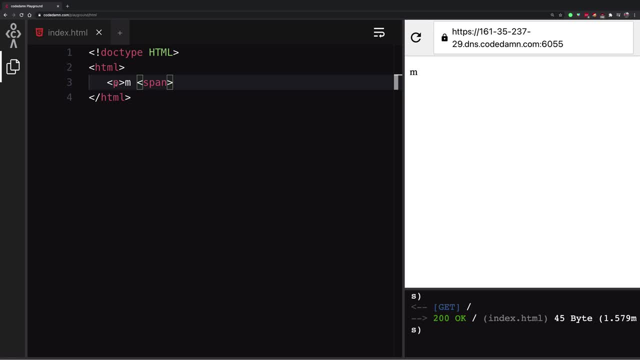 So they're not. they're not. there are not a lot of tags in HTML specification which you would say have very special meaning, except for, you know, just like I said, video, or, you know, image or, as a matter of fact, audio or canvas. I can just remember these handful of tags. 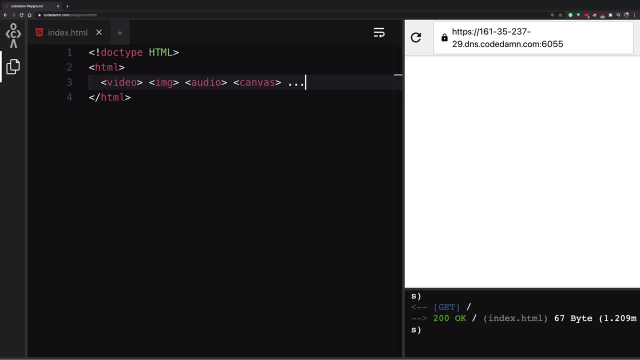 which have a special meaning Other than that. most tags are, just you know, convertible with the help of CSS. But the actual meaning, the true meaning of HTML is to convey meaning to a particular, let's say a particular software. just assume a software which cannot really see. 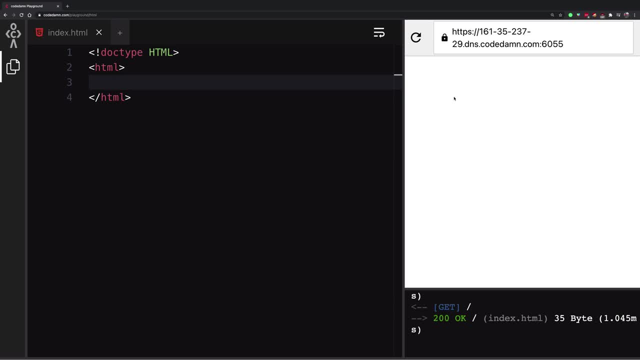 your web page. But if that software is able to data mine that hey, this is how the web page would probably look like. that means you have written correct HTML. What do I mean by that? Let's say you're creating a website where you have a header or footer, let's say content area in between. 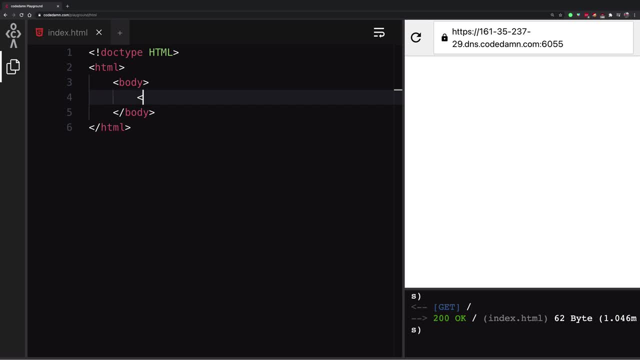 So in HTML 4.1, what you would probably do is just to have div ID header, you know, div ID footer and maybe like div ID content, right. This is, although this is fine, but what HTML 5 says, the. 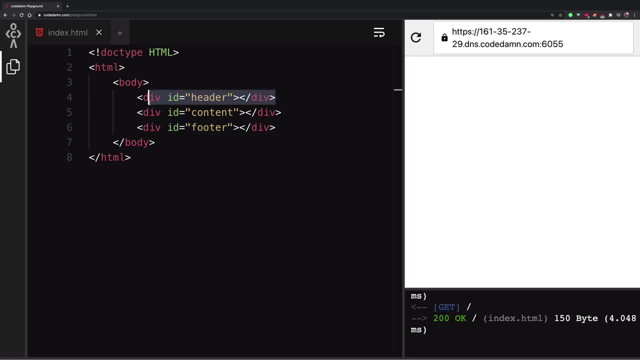 more HTML 5 fee. way of doing this is actually using the semantics tags. So HTML 5 brings in a header tag, right. HTML 5 brings in a footer tag And HTML 5 also brings in, for example, let's say, a: 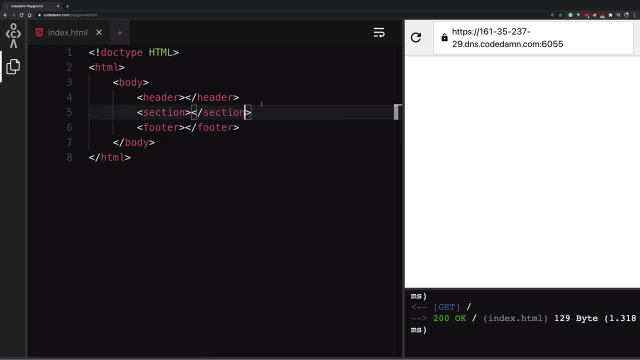 section right. So just to define some sections: If you want to have a sidebar, there's also an aside tag. So all these things, you know, these new tags exist in HTML 5.. But we're not going to go into very depth of these in this. 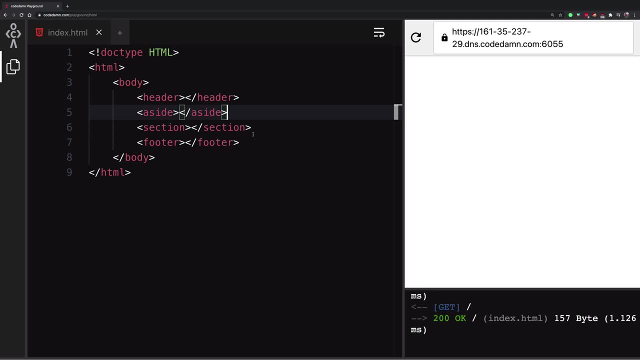 because I want to cover other other important things. These things probably would be more interesting if we pick up an accessibility course or something like that, But that is something for some other day. So that is Yeah, that is what HTML 5 essentially is: more semantics, less of. 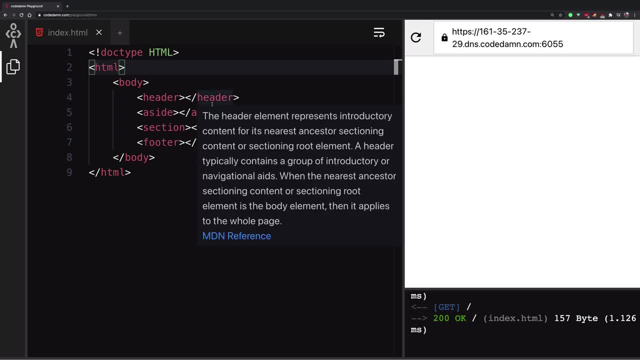 doc, type HTML thingy And more or less the same HTML as before. So that's all for this video. I'm going to see you in the next one really soon. Hey, everyone, welcome back. And in this video let's just go ahead and discuss about meta tags. 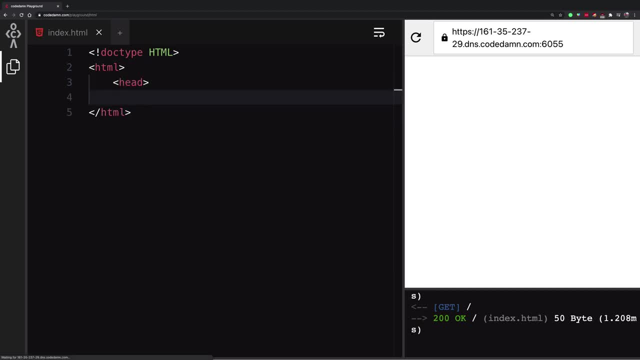 Meta tags is a very interesting thing And, as a sort of a front end web developer, if you're working in a company or in a startup which wants to have SEO, that is, search engine optimization- meta tags are going to be your friend. Why? Because you know meta tags serve a. 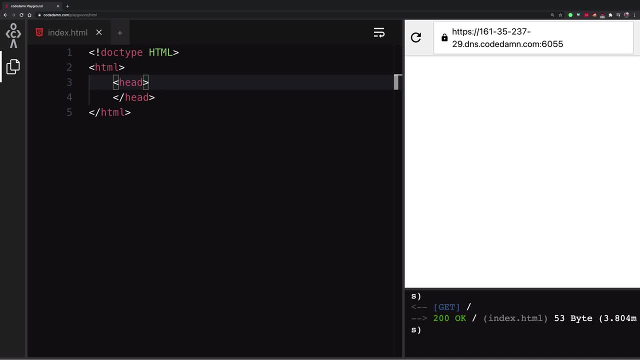 lot of information to these bots and crawlers and search engines about what your page is or how your page. you know what your page contains as a sort of header information, So by now you might have guessed that meta tags goes into a head section And they are not, like you know you. 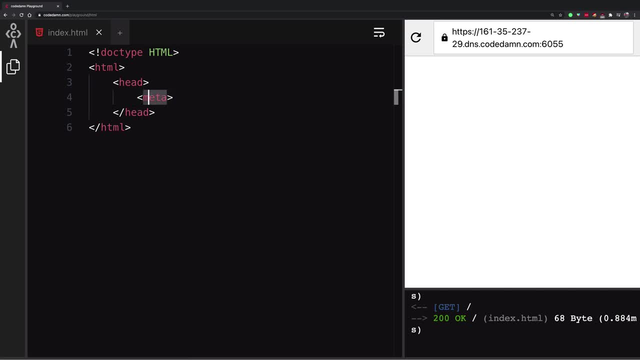 don't really have to close them, just like image tags. So it starts with, you know, just meta keyword, but it obviously needs to have more sort of information. So the first thing that I'm going to do is I'm going to go ahead and click on the meta tags And I'm going to go ahead and click on the. 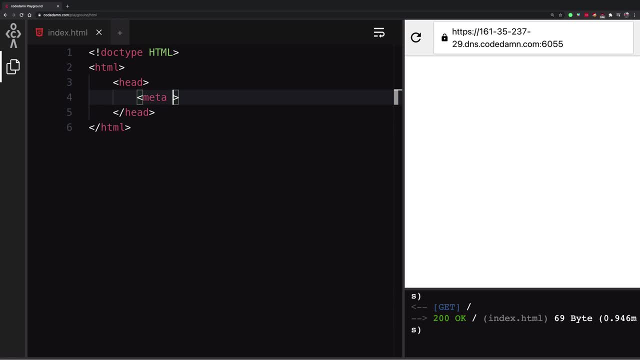 first tag which you know, the first thing which you'll actually see, which is sort of like required in html as well, i guess, is meta charset, and then you have to specify utf-8 here. what this really means is that when your browser is reading this document, it means that whatever characters you're 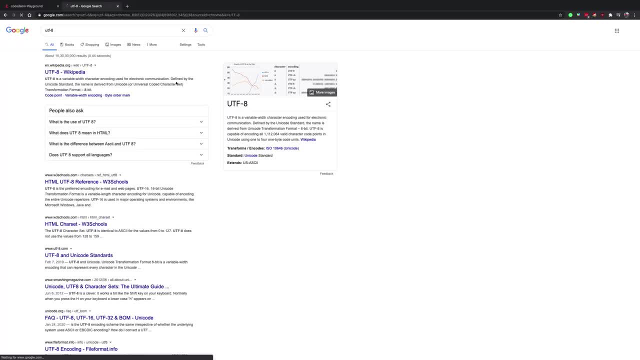 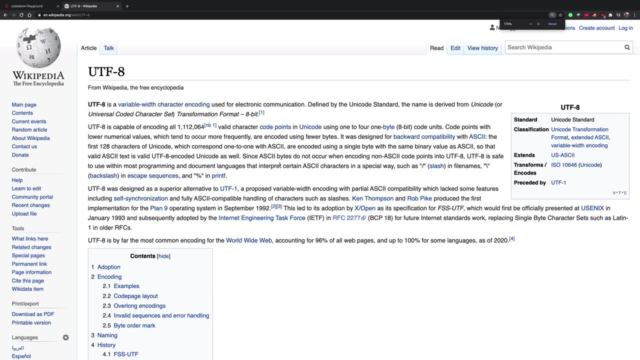 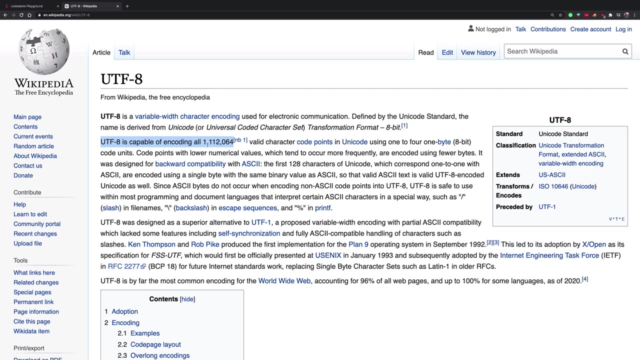 going to be using are going to lie in the utf-8 charset. so if you go to like wikipedia page of utf-8, you're gonna. you can go ahead and read more about, uh, what utf-8 is, but it's more like you know if you read about. it is capable of encoding all the uh, what is, what is one million? 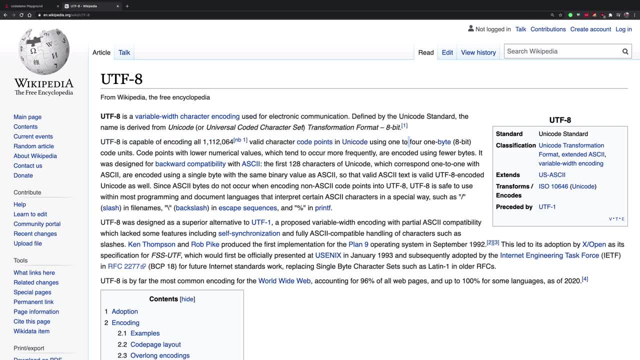 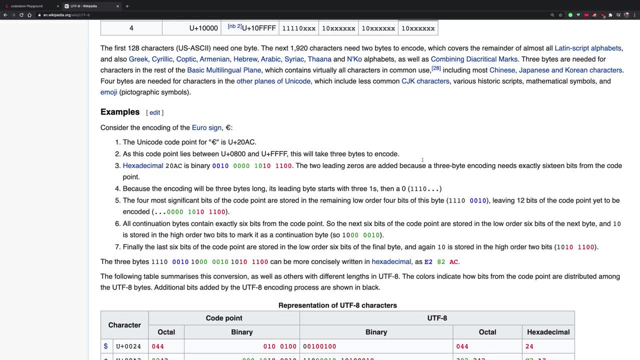 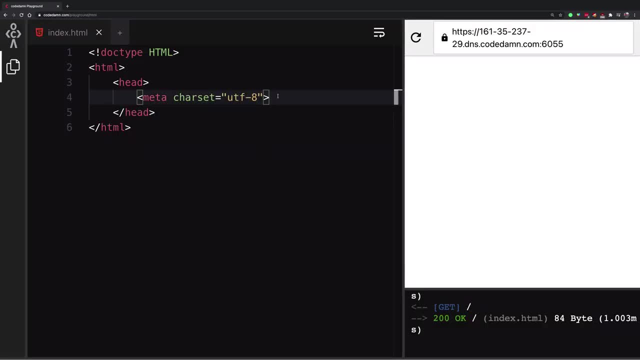 over a million characters code points in unicode right. so, yeah, this is basically that. this means that you will not be using some weird sort of character which is not present in unicode right. and if you're using it- i don't know- probably your browser- might you just not display it in the way you like. so this is like informing the browser right and other. 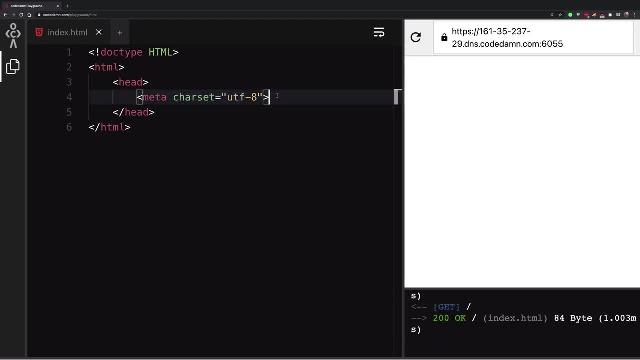 people like search engine could also use this to get information. the next thing is that you know there is sort of a variant of meta which is interesting, i'll tell you why- and that is http equivalent right or eq. i don't know if this is equivalent or eq, but yeah, that's how you spell. 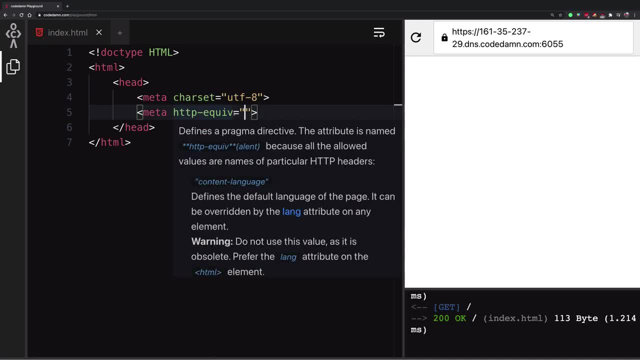 it. what this tag is is that it can sort of mimic how the response comes from a back end. now hear me out. in your uh, the fundamentals of html, uh fundamentals of http course, which you have taken for the front-end developer learning path, you have learned how websites work right. when you visit a url like 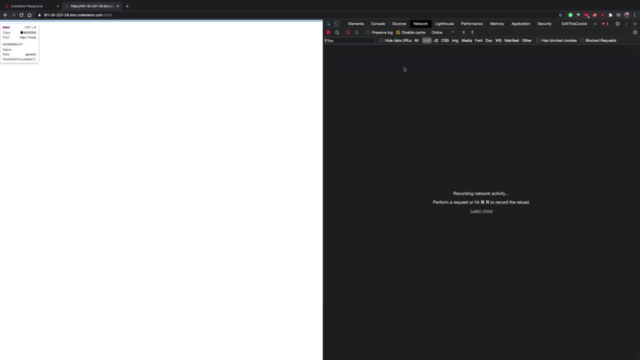 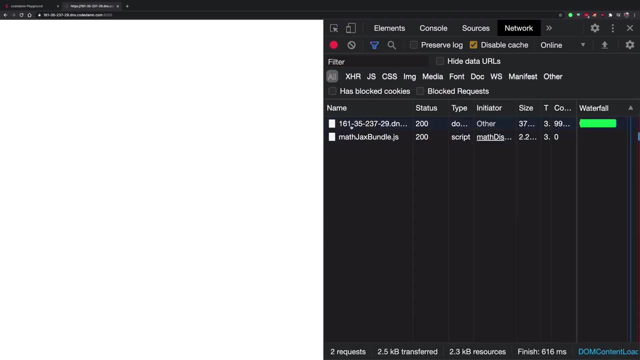 this if i go to console inspect. don't worry if you don't know about this interface. we'll actually learn this in chrome dev tools course. so if i refresh this, you can see that we have a couple of requests here. the first one is the request which i'm looking for. 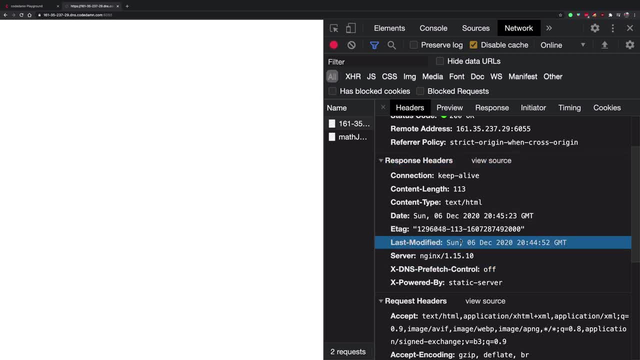 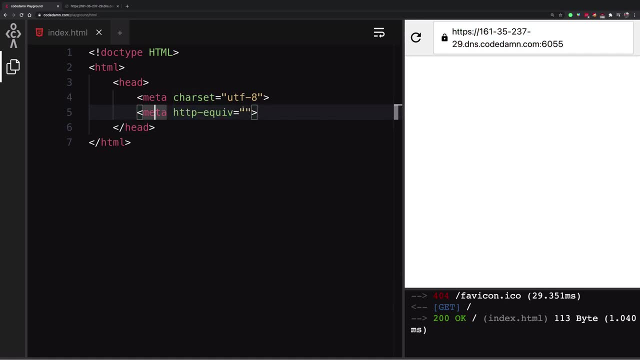 you see, we have certain response headers which tells some information, right. so, in a similar way, there are a few things, a few values which you can use here, which will mimic as if, uh, it is coming as a response header right now. this is not, you know, something which you'll use very often. this is 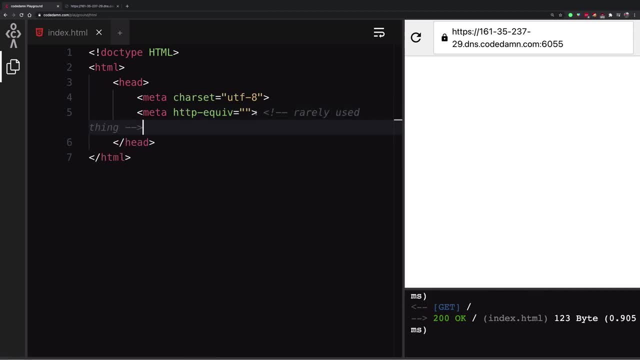 actually a rarely used thing, but when you need it it's pretty cool. i'll give you one example which is like the- i think the 99% of the times you'll use this is because of this, and that is to refresh your page on the html level. 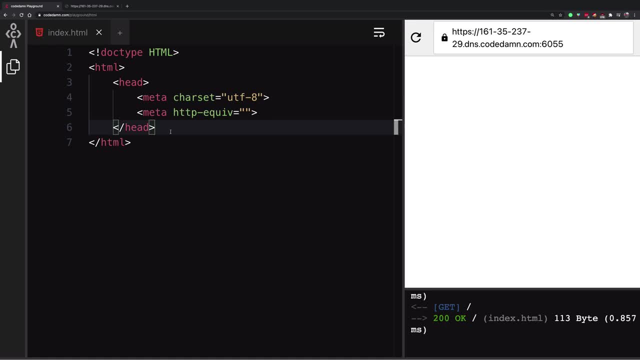 right. so if you're, if you have a little bit experience with javascript, you know that you can refresh with javascript. but did you know that you can actually refresh your page automatically with html itself, without actually involving any user click or anything like link click? you can do that by saying http eq is. 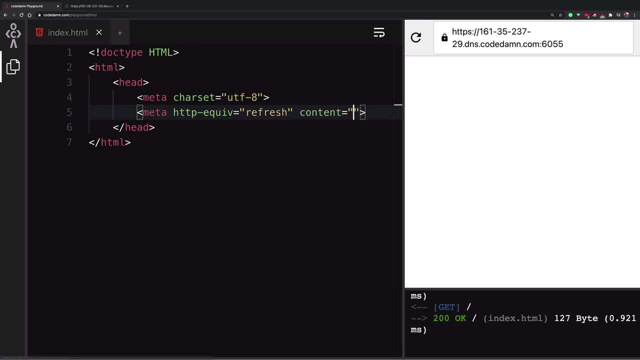 just to actually refresh your page so you can refresh, and then your content will actually, you know, be a duration in which you want the content to refresh, let's say every five seconds. i'm going to have a body here and i'll just say: i am refreshed, right? let's see if we can observe that. 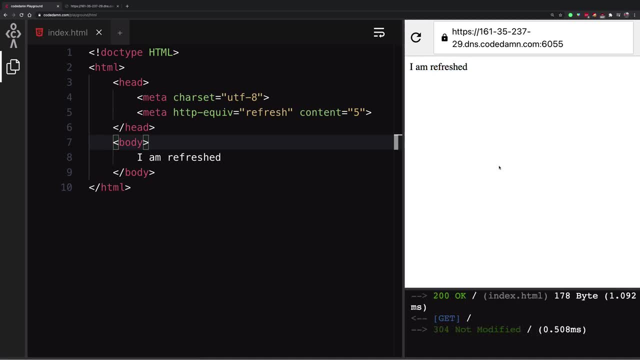 so you see i'm refreshed this here. i have selected this text and within five seconds you see the page refreshes and you can also see that the request here is the server right. so if i select this again after five seconds, it should probably just refresh, right. 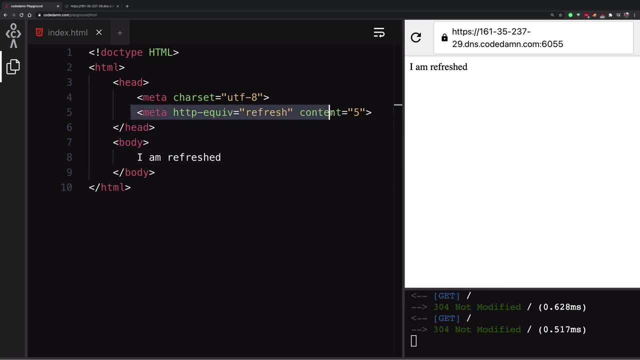 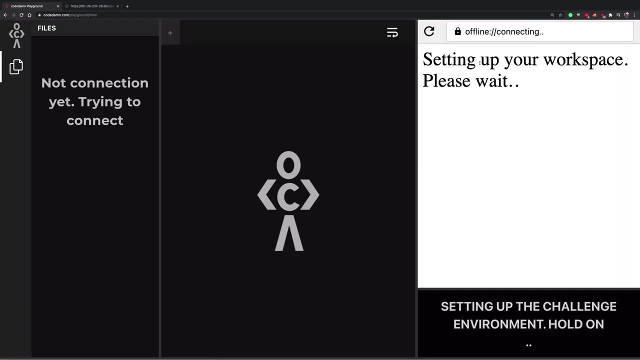 so it just refreshes automatically. so this is how you can automatically refresh with html. not the best use case, but i'll tell you, i'll tell you a little secret: if i refresh this page itself, what you're gonna see is that when your playground is loading, you're gonna see this: nice, uh, you know. 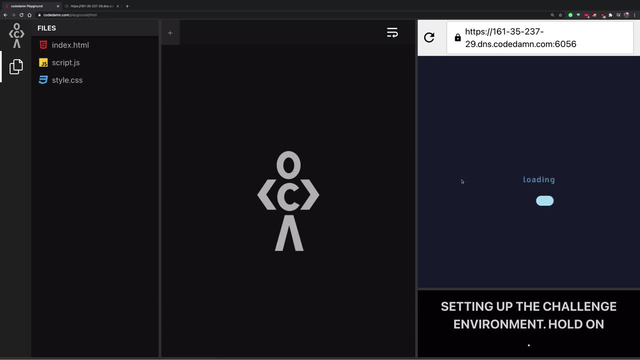 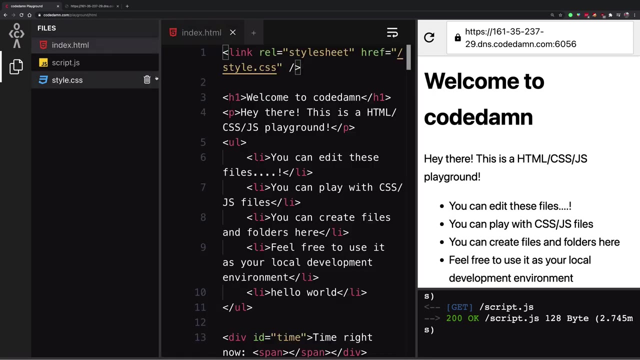 this interface right. this interface right here refreshes every three seconds to check if your environment is set up right. and the way it does that is using the same sort of http eq right. so that is. that is one use case. so we are using it on codename itself. 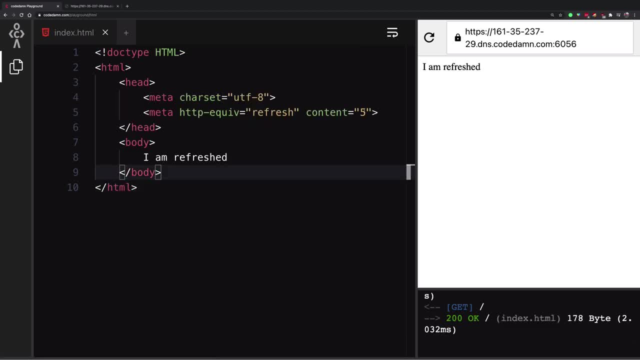 which i just showed you. so anyway, this is like one way of uh http eq using http eq. the other ways, which are most common with meta tags, are basically using the name and the content format. so you're gonna have meta name, as, for example, let's say description, and content is gonna be 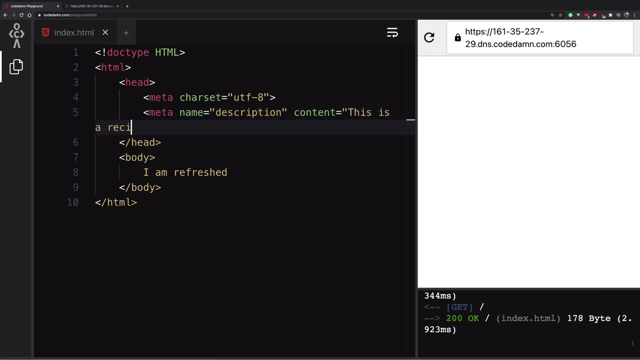 something like this is a recipe website for, let's say, pizzas, right? so let's say you're creating a personal blog on how to make best pizzas or how different pizzas are created or made, and you want your website to be indexable. that is, if somebody goes to google and types how to create a pizza, you want your website to be. 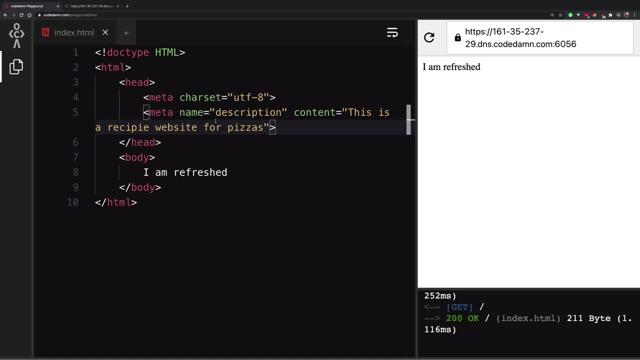 probably shown right. so this is how you can make sure of things like these. this is like a first step you should do in order to optimize your on-page seo. that is, you should have correct meta tags. meta description, title of the page, you know. title: how to make pizzas. 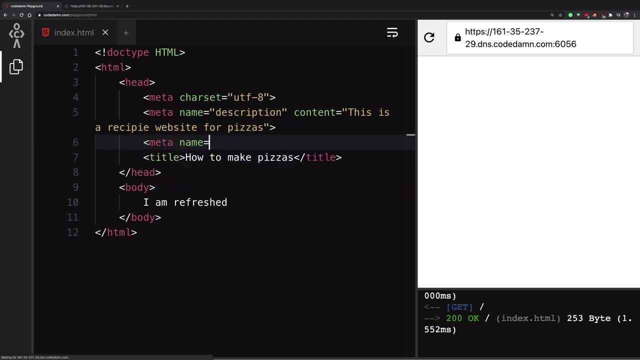 then there's also a meta name keyword, as far as i remember, but i think google does not really support it anymore. but you know, you get the idea. you can just go ahead and read about seo meta tags if you want. uh, but yeah, this is how that's. that's basically the use case of meta tags in terms of. 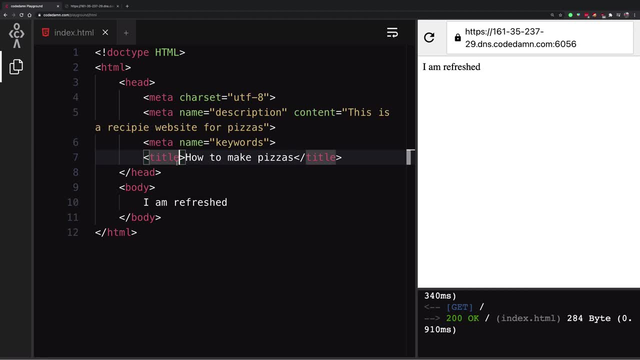 seo and we also saw an interesting use case with that. uh, http eq, right. so yeah, that's. that's basically to meta tags, nothing related to as such, uh, your page that you can use as a source of your page. That is why it is actually called meta, because this is meta information to your page, right? 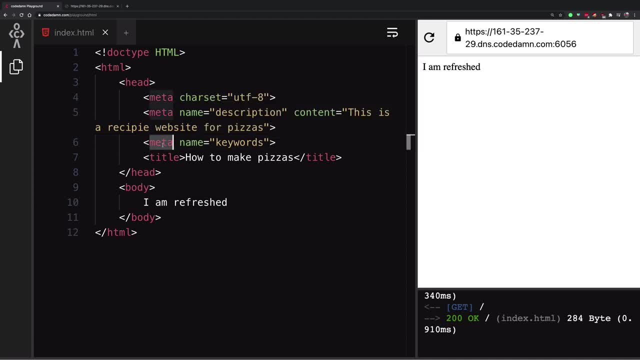 So it's not really meta tag would not really affect your page anyway, except for that HTTP queue refresh. So it will just be a very quiet sort of tag and would be just sitting on your page. That's it. So yeah, that's pretty much it for this video. 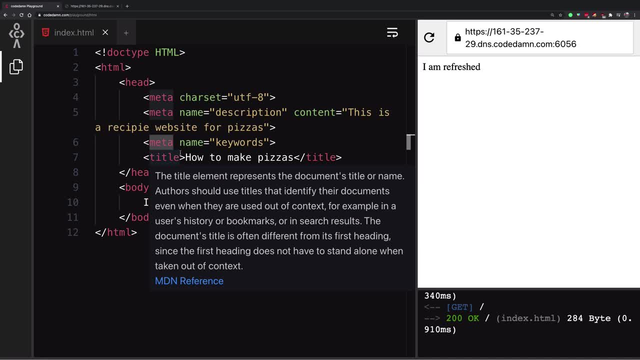 I'm going to see you and discuss more interesting stuff about HTML in the next one. Hey, everyone, welcome back. And in this video let's just discuss the difference between logical and physical tags. Now, this is a sort of- not a technical- term. 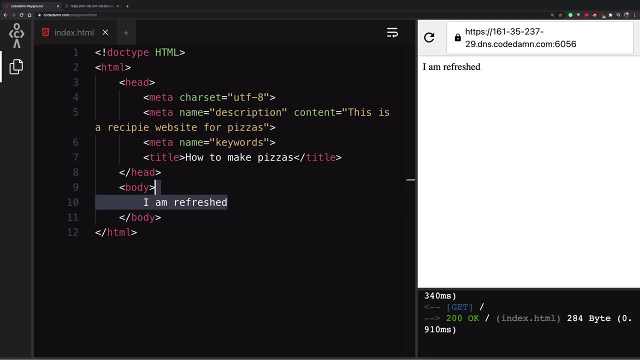 I've just used it because some people use it and I like it kind of. but I'll just explain you what this means. So in HTML, from the last course, from our basic course, you have seen that you can make some text bold. 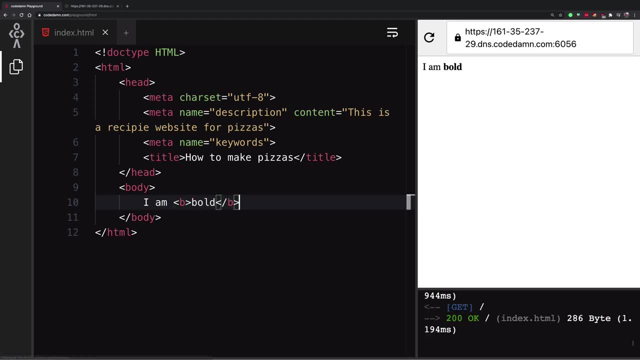 You can say: I am bold like this and the browser will appreciate that and, would you know, just render your text as bold. Well, if you think about it, you also have something known as strong tag right, Strong And bold and strong sort of. if you think about it, do the same thing. 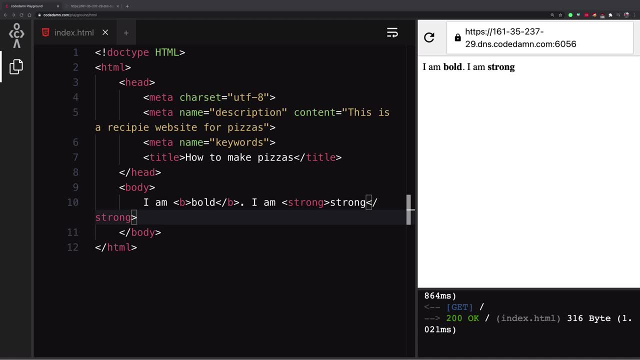 So, uh, you know what? what is the difference? What exactly is the difference for them? Now, first of all, let me tell you how I would have explained this difference 10 years, 10 years ago, right, Because 10 years ago we would be working on HTML 4.1. 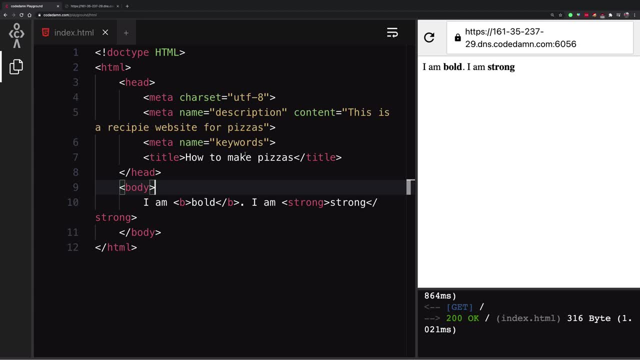 I'll tell you why I'm saying 10 years ago and not right now. I'll explain the difference today also. but let's assume we are 10 years back, right When HTML 4.1 was the thing. So in that time you're going to see that B bold is actually just bolding the text on. 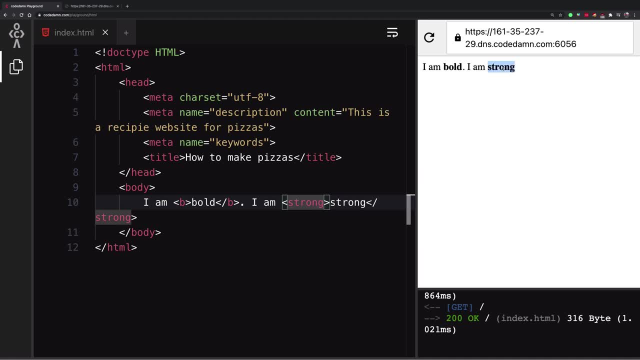 the screen right Strong is also doing the same thing. However, B tag, Romantically speaking, does not convey a lot of value, right? What do I mean by that? Is that? well, you just say: Hey, I want this text to be bold. 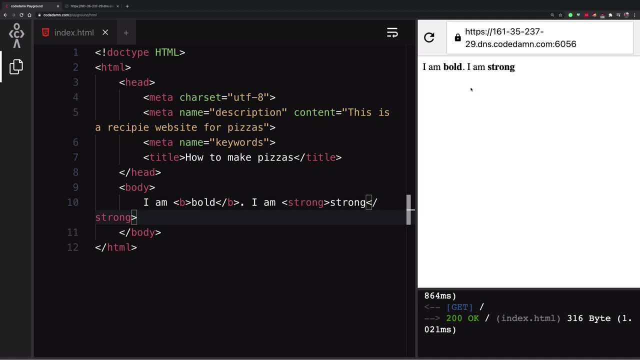 That is something which you will see as a visual person who can see right. Assume that somebody is using a sort of a reader which just goes through the webpage and tries to read back the content. Now that particular reader should it like mention is the if the text is bold or would 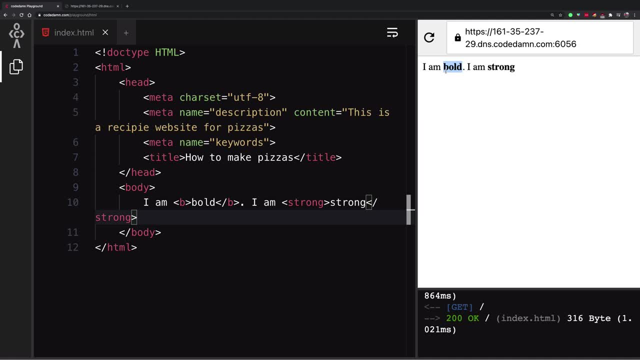 it be like just a wasted sort of opportunity or time, right? So this B tag basically does not convey a lot of meaning in the semantic world. It just says that I want this particular piece of text to be bolded. not really, you know. 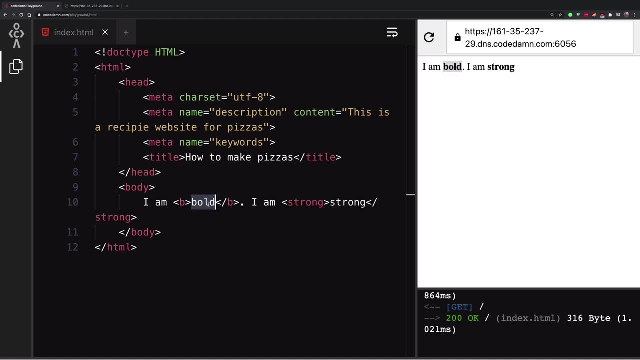 if this is important or if this is something which should be highlighted, distinguished and all that stuff- right. So you could pretty much just go ahead and bold anything which is which might not be important as well, right. However, when you're using strong, you should be able to say: Hey, I want this text to be. 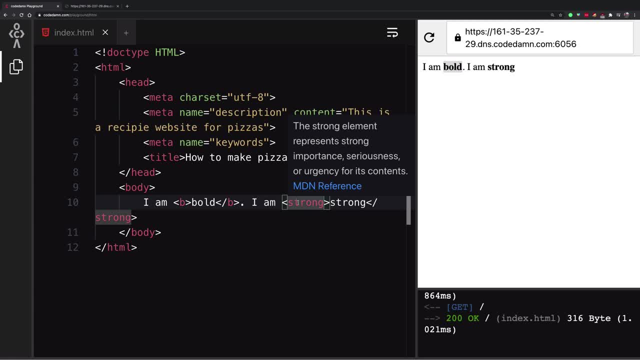 strong. You're sort of, like you know, conveying the message that, Hey, this particular piece of text should stand out right. So you can see that even the sort of helper says is the strong element represents strong importance, seriousness or urgency for its content. 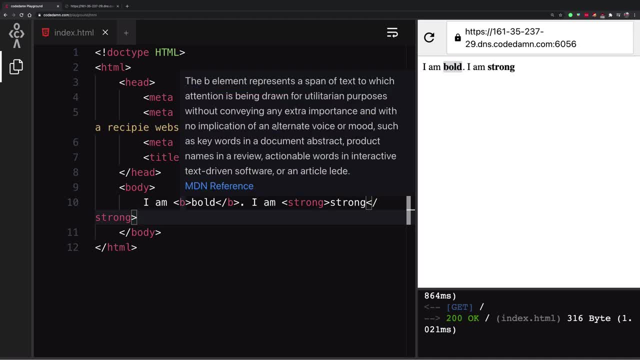 But if you check the B element, you can see the well. it is the HTML5 version. but HTML 4.1 would just say that Hey, B element is just used to bold the text. That's it. Now let's just come back to HTML5.. 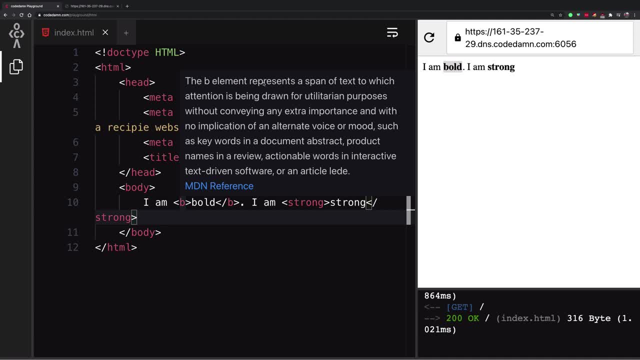 And the difference in today's world versus the 10 year old world is sort of like I don't really understand. to be honest, right, It's not a very great difference. So the spec now says: the B element represents a span of text to which attention is being. 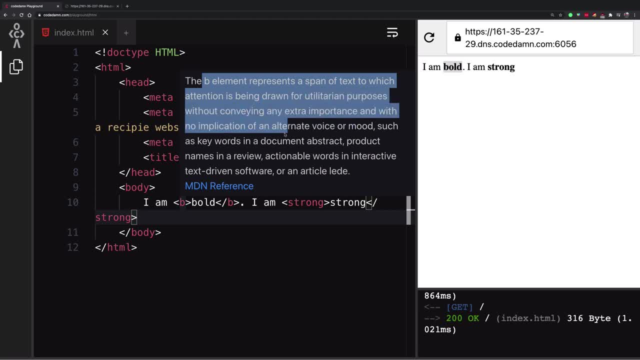 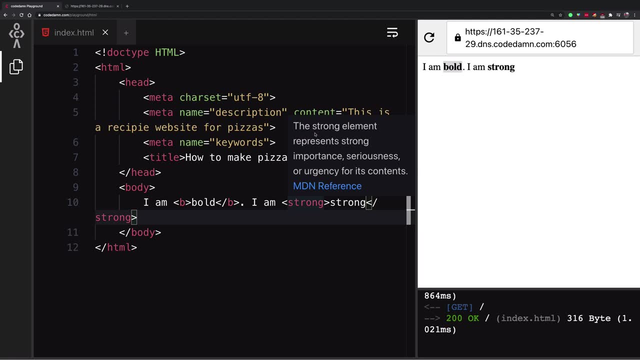 drawn, you know, without conveying any extra importance and with no implication of an alternate voice or mood such as keywords and document abstract. you know all that stuff, But strong just says that you have to see this. This is serious business, right? 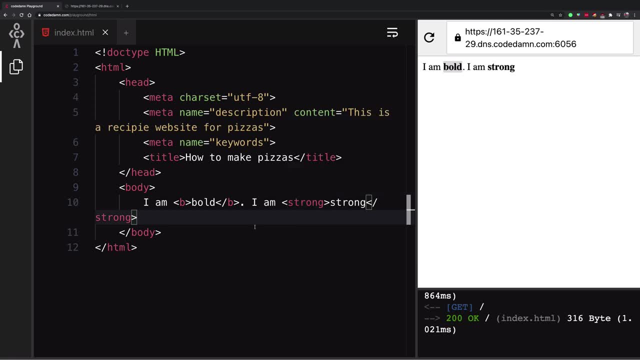 So I don't know like HTML5 spec is sort of like not really distinguishing both of them very strongly, you know, ironically, but yeah, so what you should use as a, as a person I would say, don't really. you know, think a lot about this. use whatever comes. 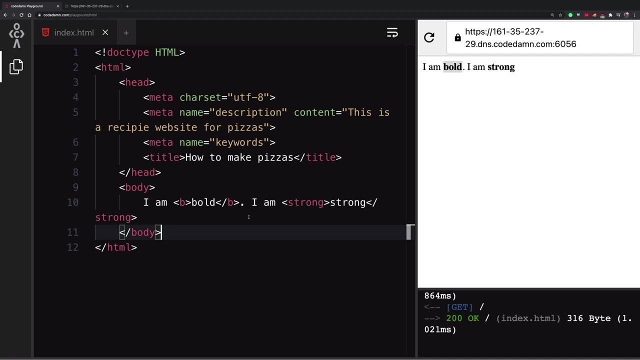 to your mind. honestly, you can worry about these things when you're actually, you know, either learning about accessibility in HTML- very important thing- or maybe you know you just want to. I don't know. just just if you like B or strong personally, you can just go ahead and use any one of them. 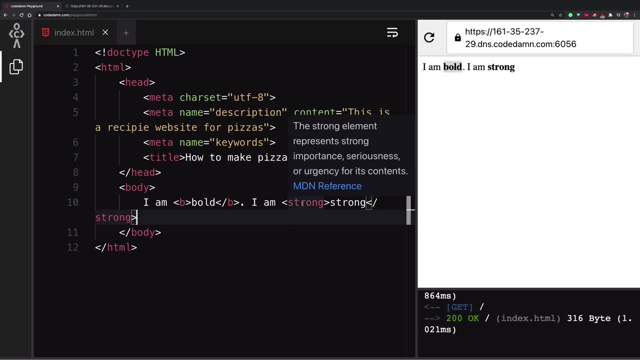 But personally, I would say just just the semantics says that if you want to drive some attention, why not just go ahead and use strong all the time, or be all the time, or maybe just go ahead and use CSS. As a matter of fact, it does not matter, right? 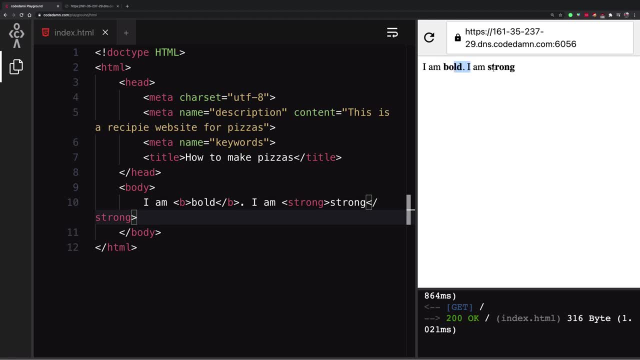 Apart from the accessibility reasons, if you assume that the person is going to see your web page, it does. It does not matter. Now, what is the, the title of the video then? logical versus physical tag. This is a logical tag, right. 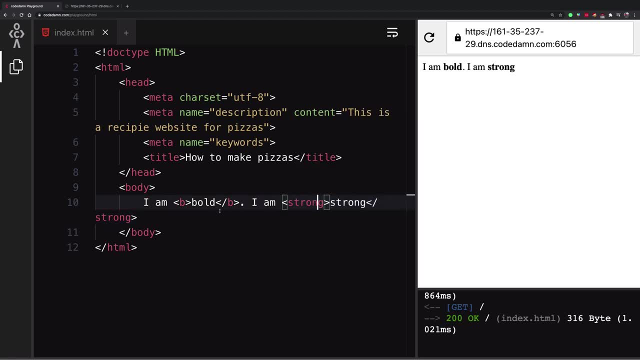 Because strong logically says that, hey, this means something. but be right here, does not say that In a similar way, there's this tag called italics. I hope you have heard about this, right? We just makes the text italics. 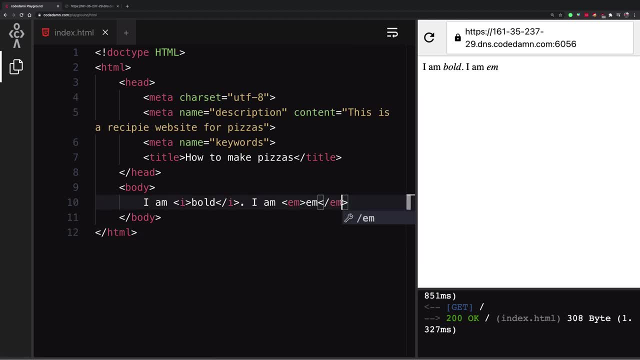 But on the other hand, we have this EM tag right here Which also does the same thing, But this tag represents stress or emphasis on its content, whereas italics again that long description, just like we had had in the bold tag. so you know, it's basically. 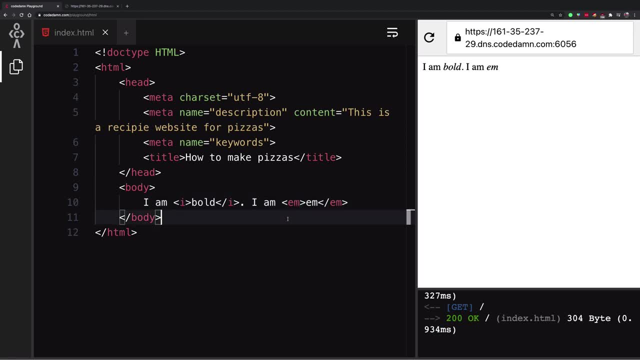 the same thing. So, yeah, that's. that's basically it. you're going to see some elements from HTML 4.1 world, sort of like, behave in the same way in the HTML 5 world, but their semantics differ a little right. 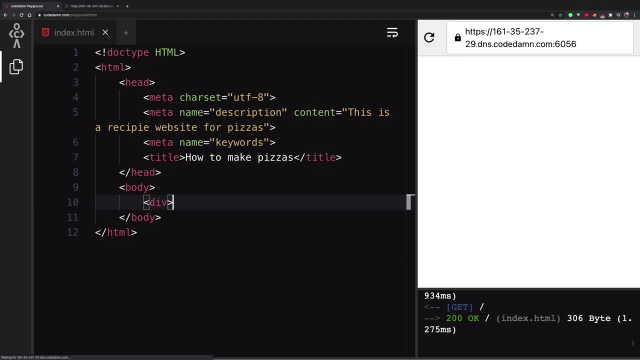 Just like in a similar way, you're going to see that div is a block level element And so is a header. But if you're using HTML 5, or maybe like if you're watching this video in HTML 5 world- which is obviously true because, well, I'm shooting this in HTML 5 world- then you should. 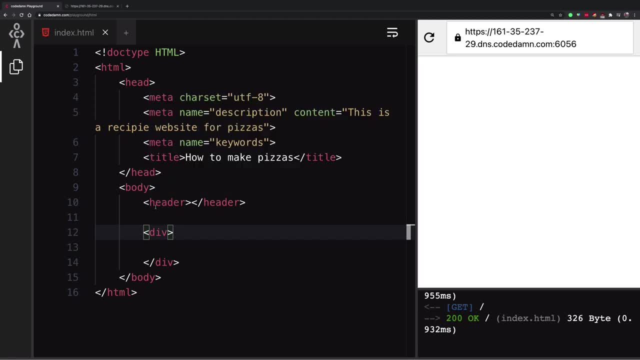 probably use this in the. you should probably use these tags, headers and footers where the places are appropriate, right, if you're creating a header sort of, if you're creating a footer sort of, then it is better to use the semantics, because you know some readers. 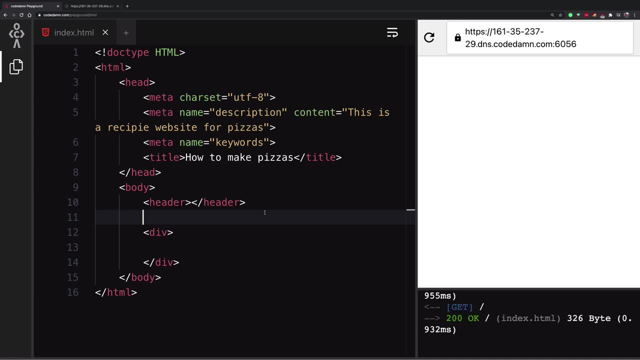 or some softwares which are programmed for accessibility more will be having a much better time in determining what is what on your page. So yeah, that's pretty much it. That's a sort of a simple small introduction or sort of like overview of how HTML 5 semantics. 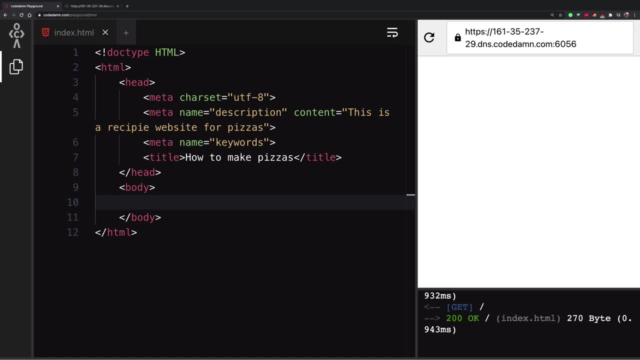 are defined And as well as these sort of overlapping tags. So yeah, that's pretty much it. That's a sort of a simple small introduction or sort of like overview of how HTML 5 semantics are defined and as well as these sort of overlapping tags. 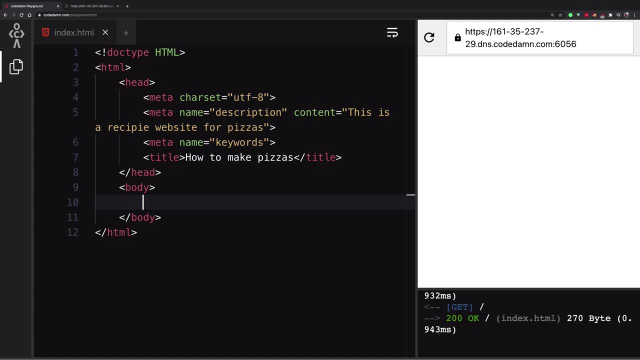 of bold underline italics and EM and strong and all that stuff, So don't really worry a lot about them, But I just thought you should know about all this stuff. So that's all for this video. I'm going to see you in the next one. 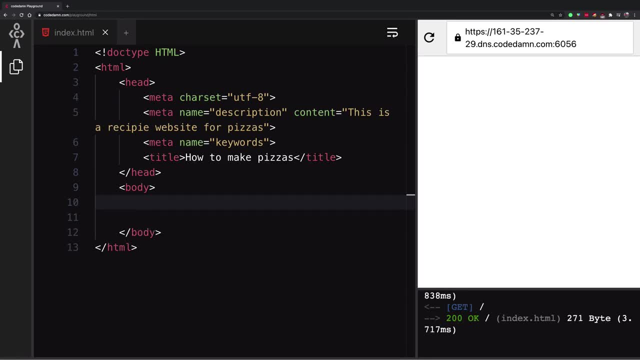 Hey everyone, welcome back, And in this video let's just discuss something about conditional comments in HTML. Now remember, before you watch this video, this is an old topic and you should never really use conditional comments. I'm just telling you this because if you see somewhere in any source code, you should. 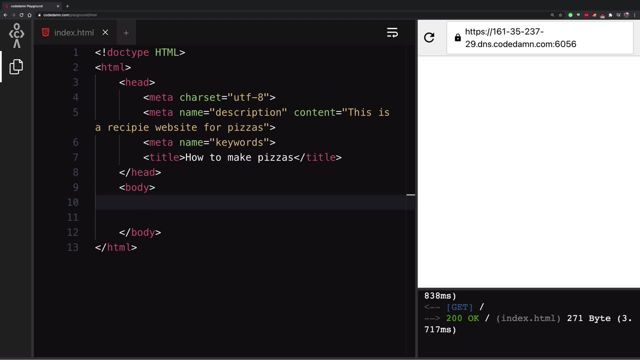 not be like scratching your head that what the hell does this even mean? So what conditional comments used to be in HTML? they are not really used at all now. is that with Internet Explorer you could sort of hack your way around to run certain 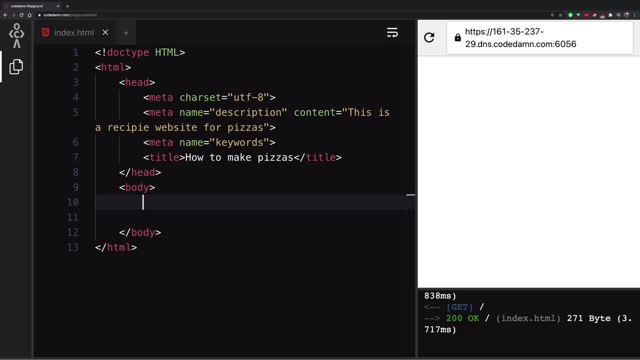 HTML code only if your browser is Internet Explorer in some way or another right Now. what does that mean? That means That IE, that is, Internet Explorer, shipped with certain hacks within the comments of HTML. You know you can start and end a comment like this and the comment usually should. 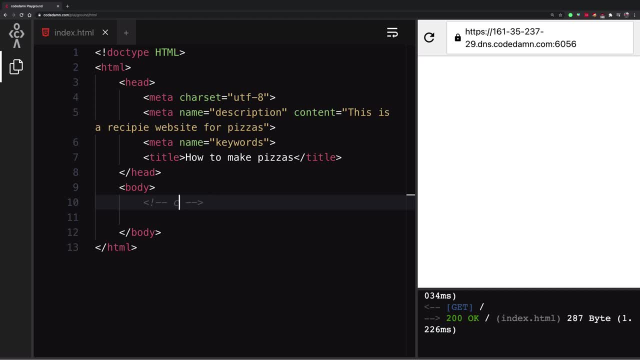 not be, like you know, passed at all by any sort of engine or anything, But what IE had was sort of a silly feature or I don't know why that was, Maybe because of compatibility reasons. but yeah, that existed right. 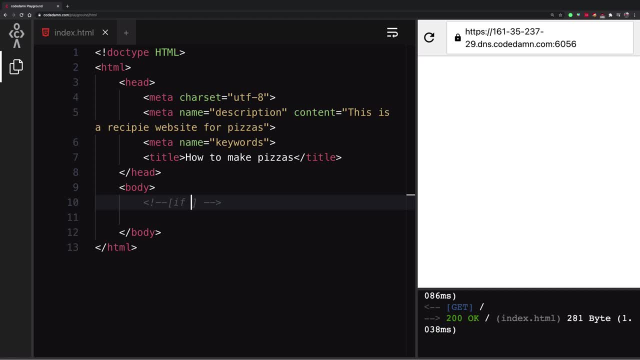 And how you could tap into that. And you would just say: if IE like this and you know you would not close this comment, right, So you will keep it like open, without the double dash. and then you'll something say something like this: why the F on you using Internet Explorer in 2021, right? 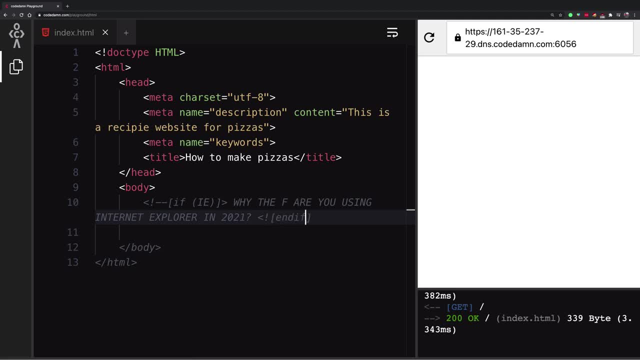 And then you would say something like: and, if I think I remember it correctly- I don't know about, I don't remember the syntax exactly, but it is probably something like this: So you can see nothing happens, Nothing appears on the page, really. 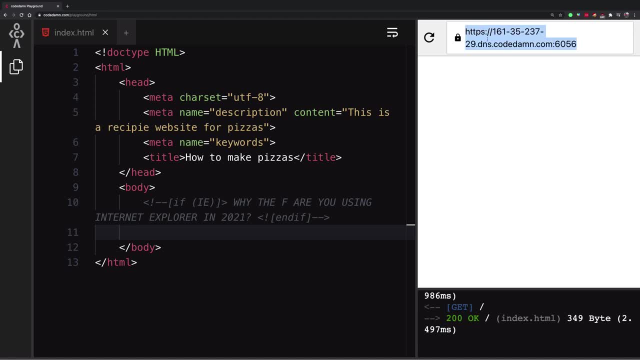 But if you were to take this URL right- And maybe if you're following this video right now, you're on your own playground- And if you take this URL, open an Internet Explorer- IE 8 or 9 or 10, and open that page. 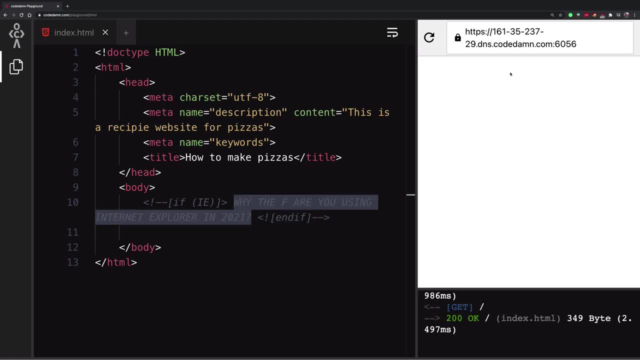 you would actually see this text on the screen. And if you take this URL, open an Internet Explorer- IE 8 or 9 or 10, and open that page, you would actually see this text on the screen, right? So that's that's. that's sort of like a hacky thing with Internet Explorers. 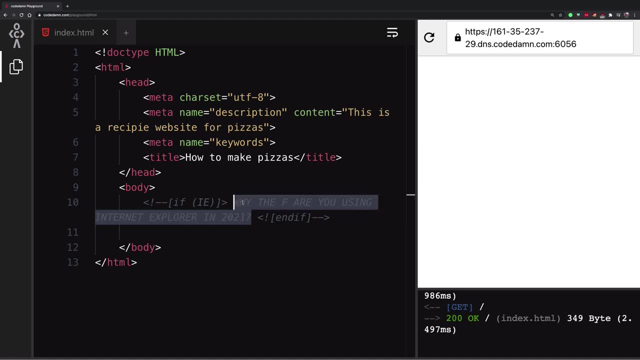 And how people used. it was like including a style sheet here, link real style sheet. you know it should have IE only, not CSS, right? So this way you could just target. you know you could actually target versions as well- IE 9, then you can have a block here for IE 8.. 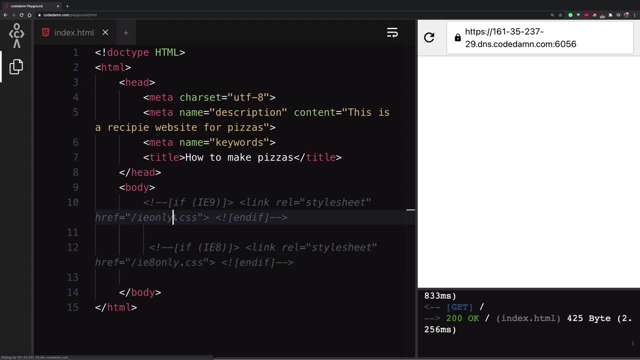 Then you can have IE 8 only, IE 9 only And on their respective versions. this would just work fine, But this is super hacky way of coding a web page, right, Because you don't really want your CSS to be browser dependent. 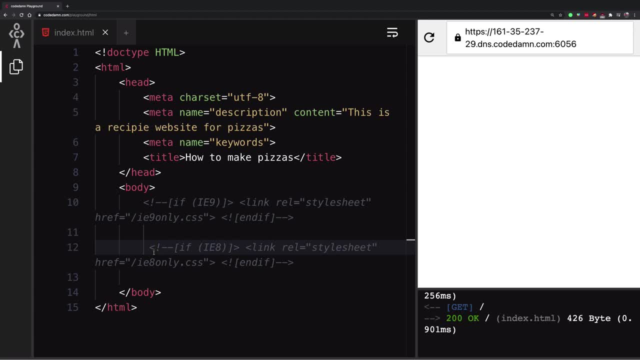 That's like you know. browsers in themselves have their own, different ways of handling CSS and HTML, And then you are specifically targeting browsers, and that too with browser numbers. So this is like an insane amount of developer work And technical burden, right? 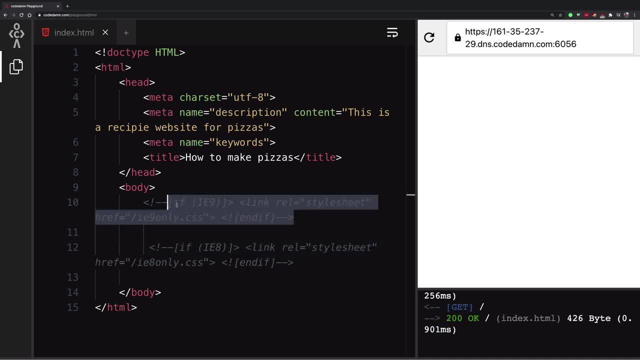 I'm just. I'm just telling you this because you should know, if you see any comment like this or any sort of close equivalent of this, that probably means that website really needs a redesign right in 2020 and 2021.. So yeah, that's pretty much it for conditional comments. you could probably, you know you. 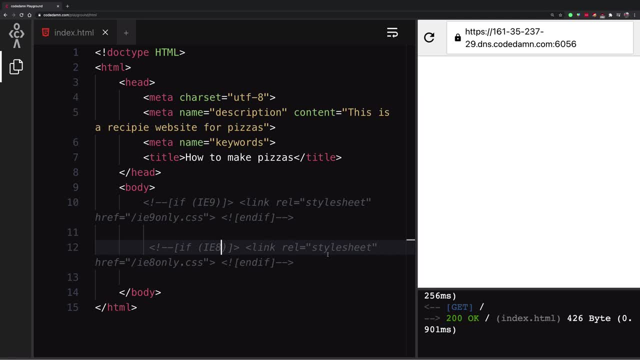 have a not IE sort of comments as well, But I'm not really gonna get into that because that's not really something you should know about anyway. But yeah, if you saw the syntax anywhere, just remember this video And just blow that source code up and code that CSS again or HTML again or whatever. 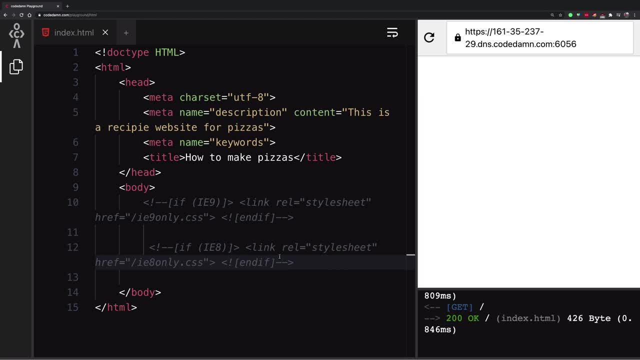 it is. So that's all for this video. I'm going to see you in the next one. Hey, everyone, welcome back. And in this video let's just go ahead and review something known as non breaking space, which might come handy sometime if you are just playing around with HTML. 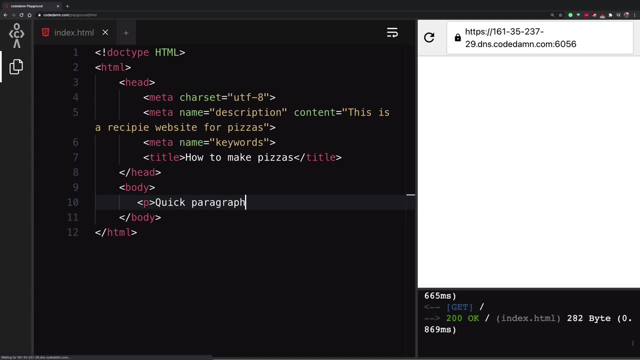 Let me just go ahead and add a quick paragraph right here And let's say I want to create another one And I want to say this: this paragraph has many spaces, right to see. I wrote a lot of spaces right here. even if I give it a lot of spaces, you're going to see that nothing. 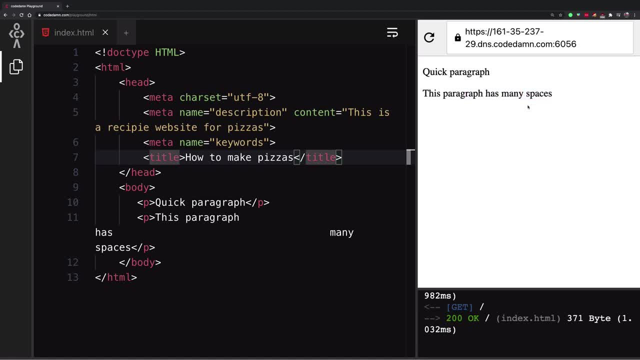 really happens. in the HTML output. you actually see that. well, it appears as if there is no space or there's just single space. right Now, HTML by default has the tendency to collapse, To collapse multiple spaces into one, And there is a way. there is an actual internal tag in define tag, which is known as pre tag. 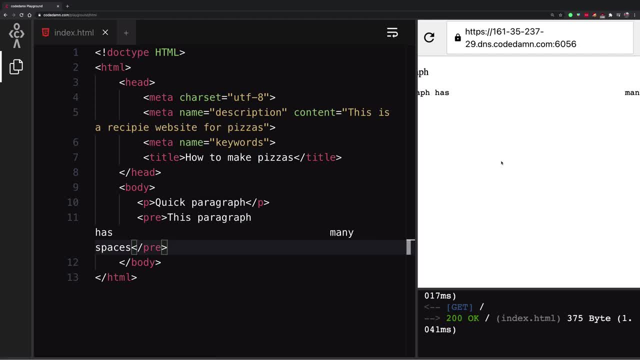 which preserves the space. So if I go ahead and scroll, you can see that it actually, you know, has a scroll bar, for you know now having so many spaces, But the idea is that a regular tag like P or div is just going to ignore these spaces. 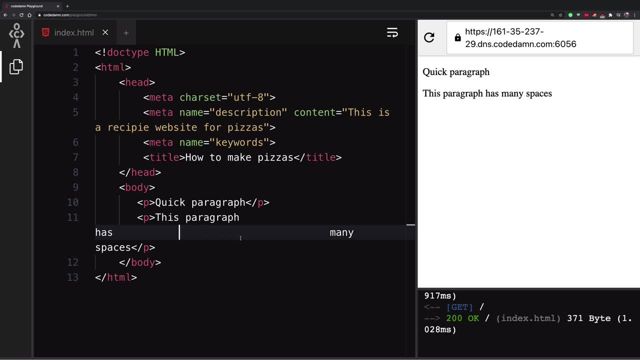 right Now. sometimes it's fine- I mean, most of the time That's fine, And other times when you really need to, just, you know, just value all the spaces and display them. you might go with options like three and everything. 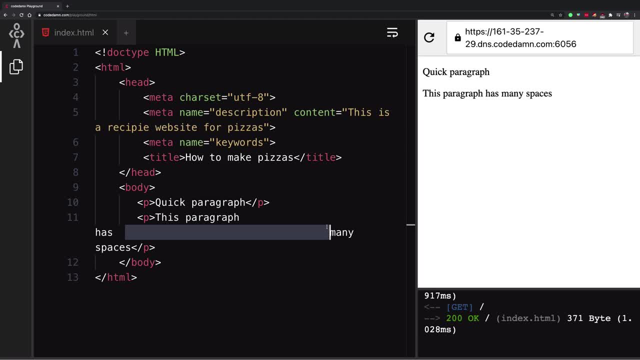 But there are times, I mean, you'll always face, always come up with those times, if you're a seasoned developer, when you just want to have a quick space without actually bothering anyone, right, Or maybe like just a little space. So for those times you have a special character known as non breaking space and HTML. how? 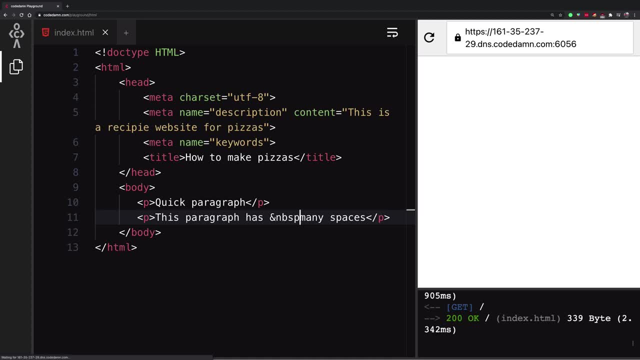 do you enter that? You use ampersand, write NBSP and a semicolon? This whole thing is super important. it should start with ampersand, it should be NBSP and it should contain semicolon right. Otherwise things will not work. 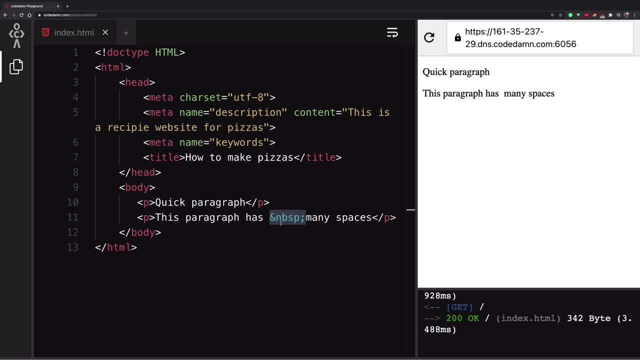 So this right here, what you're seeing is an HTML entity, right? I think I remember another one copy, for example, you see this copyright symbol. yes, you can go ahead and copy paste this right here and it will still appear like the same. 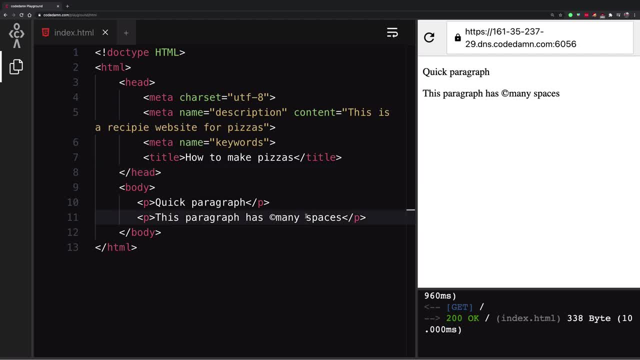 thanks to the UTF care set. But ideally, what should be your, you know, if you do not have that character on your keyboard, or maybe, like you know, if there's a- I don't know if there's, you know there's. 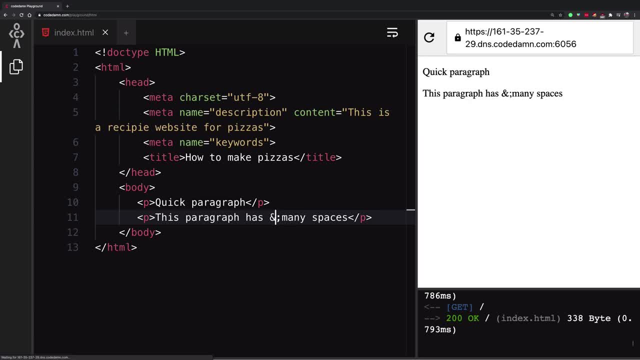 autocomplete: Wow, amazing. Let's see if we have greater than yes. So let's say, I want to say, for example, I want to say this text: P tag is an amazing tag, right, So I cannot do it now, right? 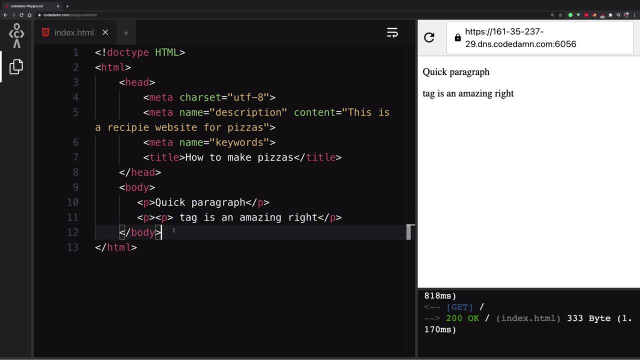 Because you know it treats the speed tag as an actual element. So how do you, how do I do this? Well, you convert these angular brackets into their equivalent HTML entities, And the way you do it is you write ampersand less than, ampersand greater than, and that's. 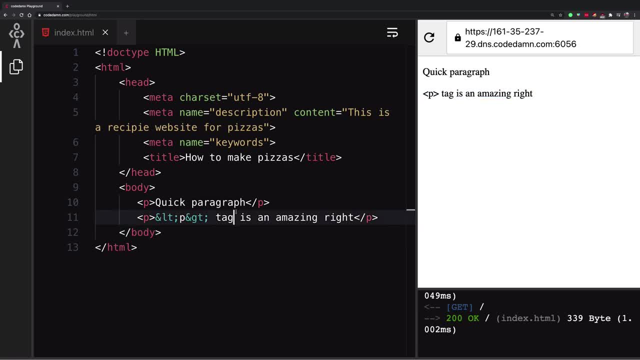 it. Now you can see P tag is an amazing tag right. Similarly, just like I said, let's say, if you want to have multiple spaces in between them, You can use NBSP, because if you do not, it will just collapse your white spaces. 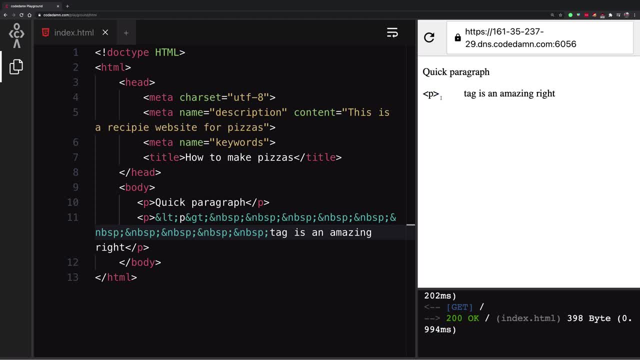 So now you can see that each individual space is a non breaking space. it does not really, you know, collapse into a single one, Because if you replace all these spaces with the all the spaces, that is the breaking space, you're going to see it. just, you know, does not work. 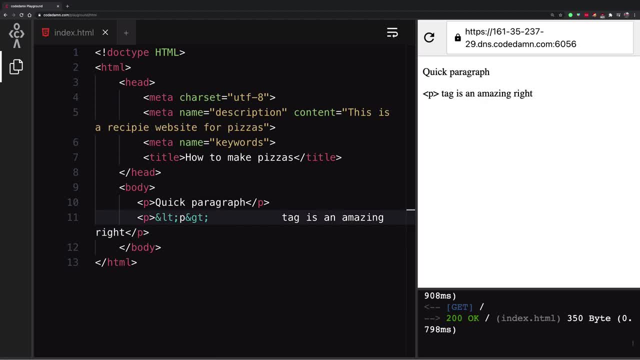 Similarly, you can probably play around more by just googling HTML five entities or HTML entities And you're going to have a lot, A lot more sort of entities available for you. you know all sorts of weird symbols. So yeah, that's pretty much. it a little introduction to what HTML entities are and what NBSP is. 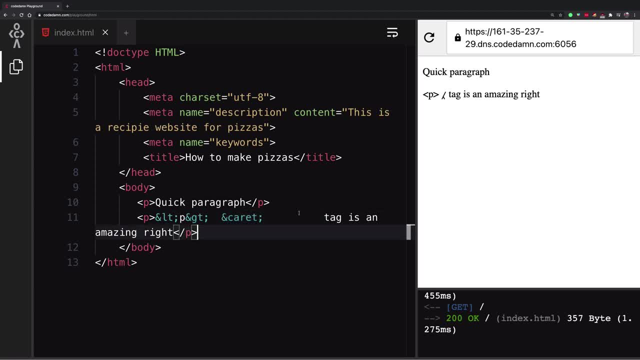 personally, I have used like NBSP more than anything else. So, yeah, that's that's why I wanted to. you wanted you to know about it. That's all for this video. I'm going to see you in the next one really soon. 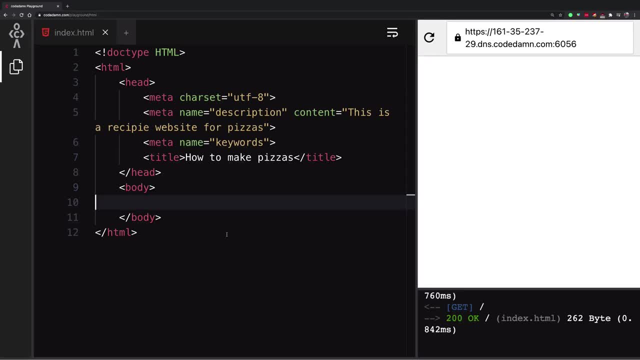 Hey everyone, Welcome back, And in this video let's just go ahead and take a look at some input values, basically all the common input values you're going to see, And, yeah, these are the typical values you're going to use in a, in a form, sort of interface. 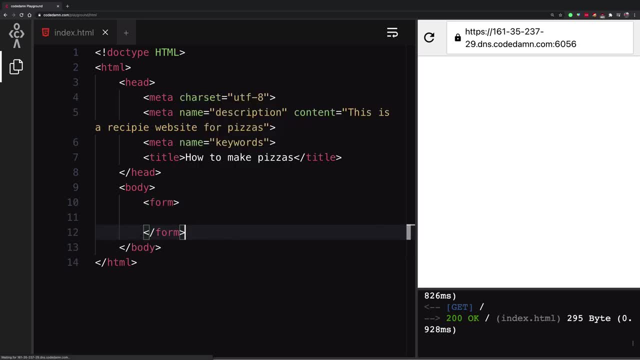 right. So you have, you have a form, And if you just go ahead and start writing these input boxes, input types, you're going to see a lot of different sort of things. So first things first. I'm going to start with input type text, because that is like: 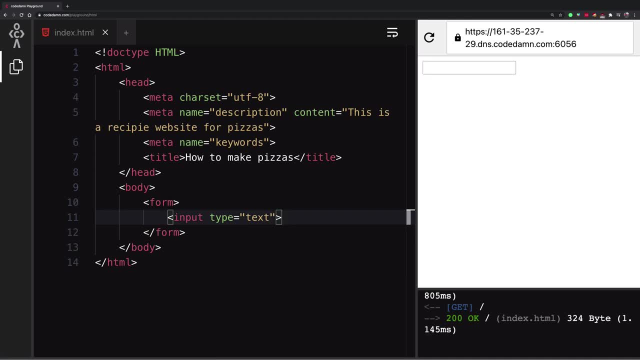 the most common Thing which you're going to use all the time, And you're going to see that it sort of creates this nice little area where you can just enter some text right now. this also comes with a lot of, you know, autocomplete and all that. 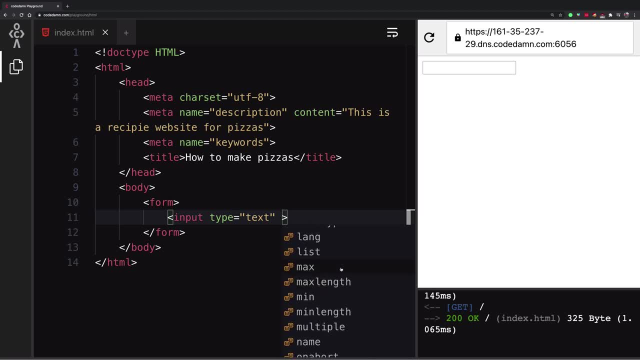 stuff And feel free to just go ahead and read about them. You know there are attributes like min length, max length, all this stuff, but this is more inclined towards form validation, which we'll quickly see in the next video. But let's say, if I want to have max length, 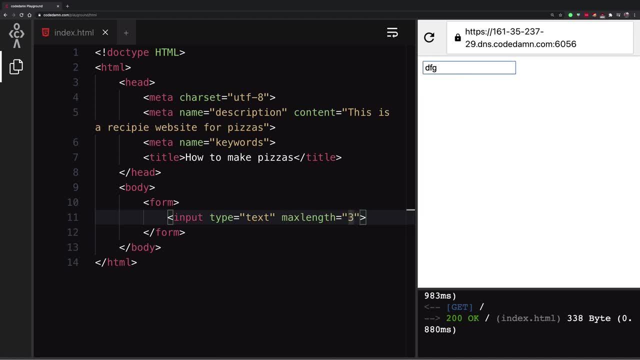 Of three. right now if I try to type, I cannot really type more characters than three, right? Even if I try to copy this URL and paste it right here, you're going to see it stops me at HTT. That's sort of like a little validation you can have from HTML five without actually just 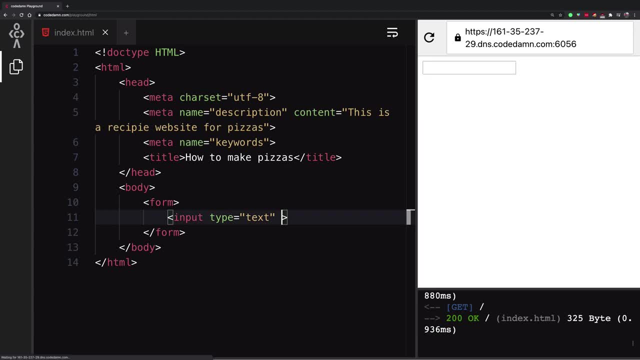 jumping into the JavaScript world, right? Then if you just go ahead and see min length, min length is probably going to fail if you try to submit the form, right. So we don't really submit the form yet, But you know, if you try to submit it it's going to fail. 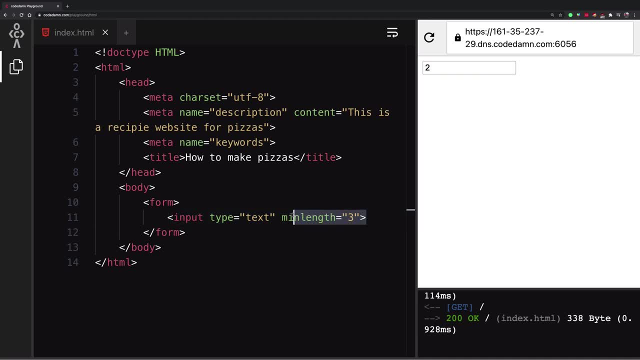 Right, If you try to submit it like on a two, it's just, it's just going to fail. So anyway, uh, we have this. then I don't know, there are like a million attributes you can play around with, but I'm just not gonna describe all of them, because that's. 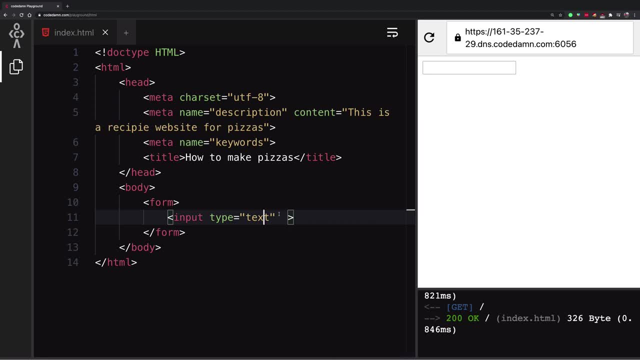 probably useless. You're not going to be using them all the time also. So anyway, this is our text attribute one year. One interesting one is a placeholder right. So placeholder sort of is the ghost text which will appear on your input fields. 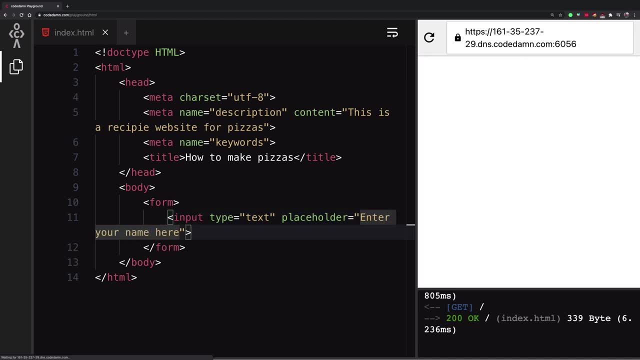 So I'm going to say: enter your Name here, right, And you can see this as the ghost text, right? It's not really a value I can. once I stopped writing over this, that text disappears, And once I remove this text, that text appears again. 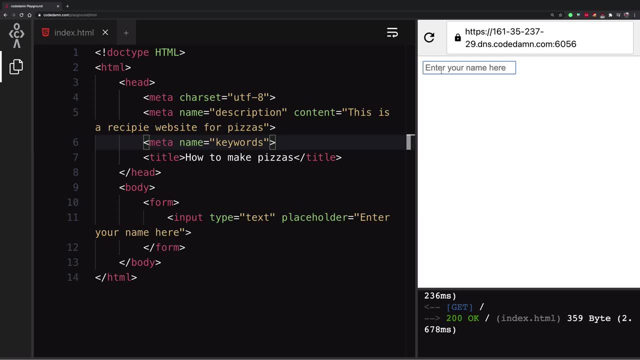 So it's pretty cool, right Just to convey information within your input field. So that's, that's one thing, And one. one cool thing about this is that it works with passwords as well. So if you have, for example, earlier we used to do like value as into your name here and 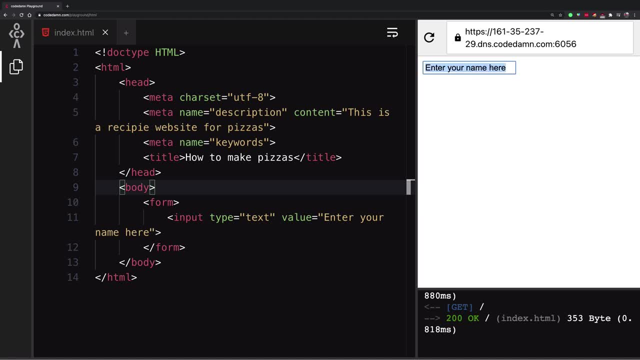 then when you click on it, We'll just remove it using JavaScript. but you know, value differs in the way that it is actually uh, the text which is present by default, placeholder is not just like we saw. the next thing: similar, similar to input type text is input type password- again, super. 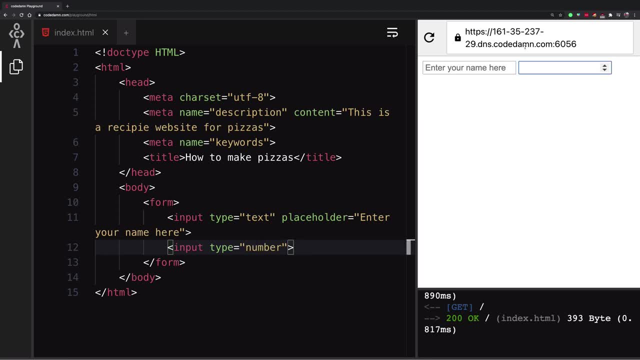 common to use. but you can see, right here you're going to really type just text. You see, once I copied this text, what it tried to do is it actually just copied only the Number bits, right? So you can see that this whole thing is a number, is also a number. 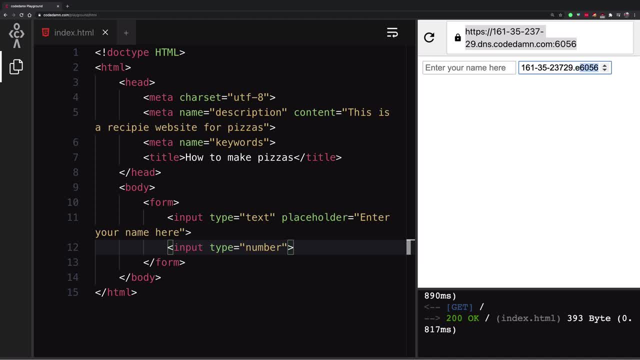 It's basically, you know, representing the power of 10 or something, but I don't know. but you can see that it's sort of like tried to copy only number and plus it gets these sort of increment and decrement for free from the browser itself. 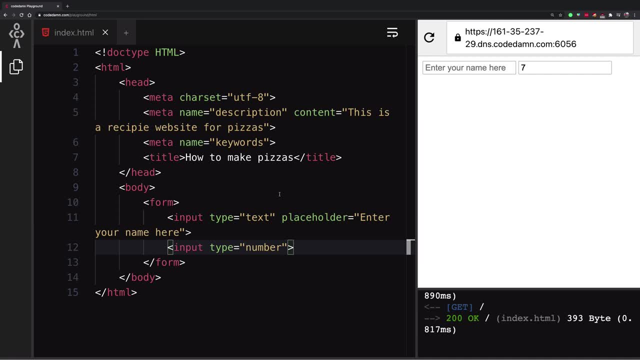 So that there's that right. So this is one thing. Next one is: uh, you have, let's see, input type file Which allows you to actually have, you know, this nice little interface from the browser itself. Now, this, all this stuff, depends on browser to browser, right? 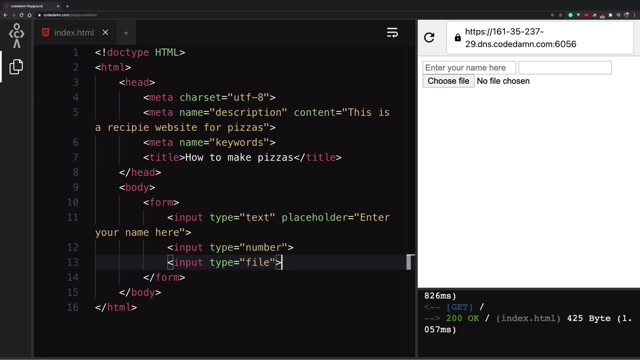 Some browsers might have a different sort of interface for picking up a file, but this thing just allows you. if you click on this, it will open the file explorer of your system And this will allow you to pick a file right- Super old, super common. 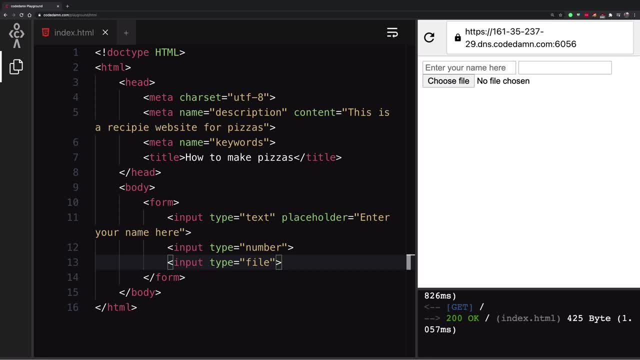 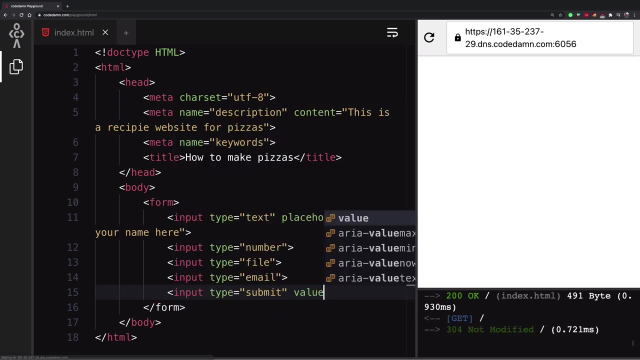 All the time we have been using as web developers. Next thing you could have is input type: email. And again, This is an HTML five sort of thing. Why? Because, uh, let's see. first of all, let me just add input type: summit, value, summit. 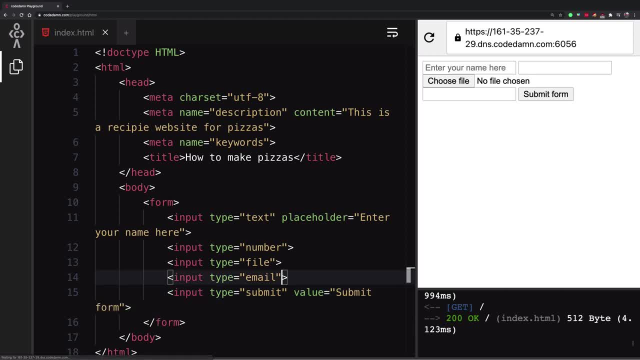 form right, And if I enter a required attribute here, that means this is required. Let's say, if I try to summit this, okay, Summit this. you can see that we get an error from the HTML five, That is, from the browser itself that please include an actor aid in the email address. 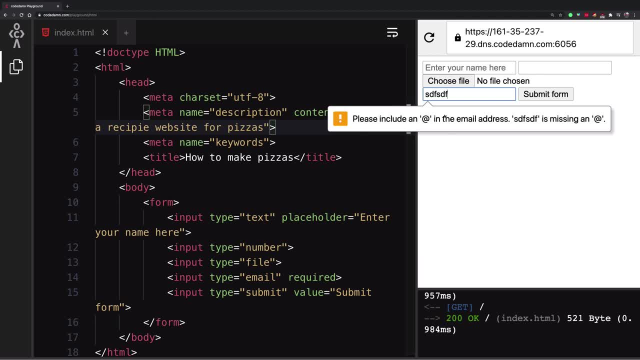 This value is missing an actor. So this is an inbuilt validation, uh, from the browser itself, from the HTML five interface itself. So this is sort of like where you would not want to use text over email, right, Because this is a much better option. 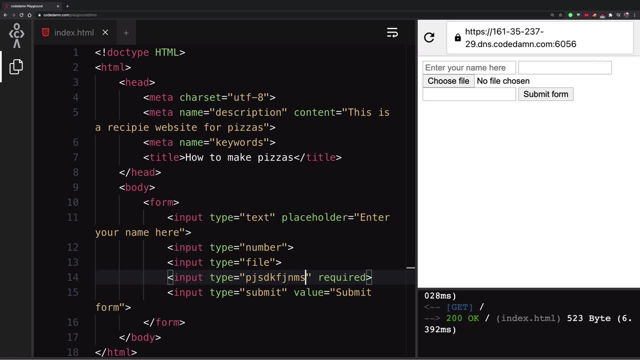 Similarly, this brings me to an important point is that, that is, if you have an invalid sort of attribute, by default it fallbacks to text always, So your text is like the sort of fallback. Okay, It will fall back for any, anything and everything which is invalid. 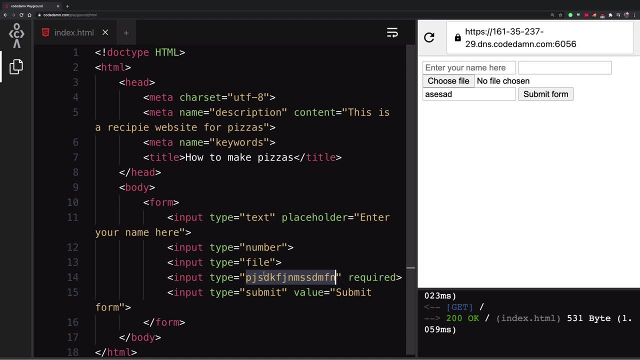 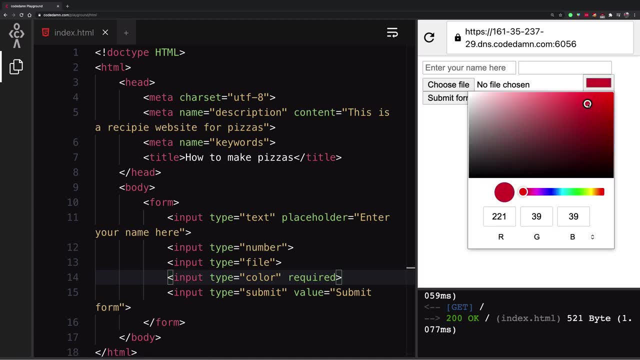 And this means this also means one thing that if a particular thing, let's say, uh, cutting it sort of thing, I think color is one, I don't know- Yeah, You can see that color sort of allows you to pick one color, which is a pretty cool. 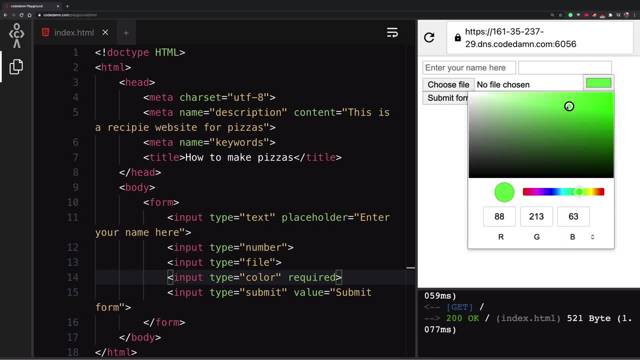 thing, if you ask me. So this color attribute right here, although it's pretty cool, but it might not be supported in all the browsers which you try to browse. So they will fall back to input type text, right? So this color attribute right here, although it's pretty cool, but it might not be supported. 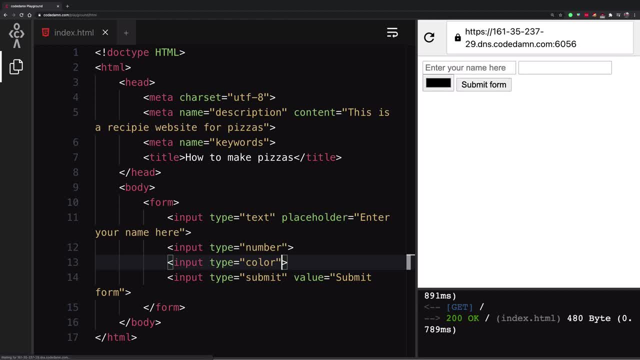 in all the browsers which you try to browse. So that's how it works. So anyway, moving on, what we can do next, what we can sort of like, discusses input type search. This is also pretty cool. I like this one. 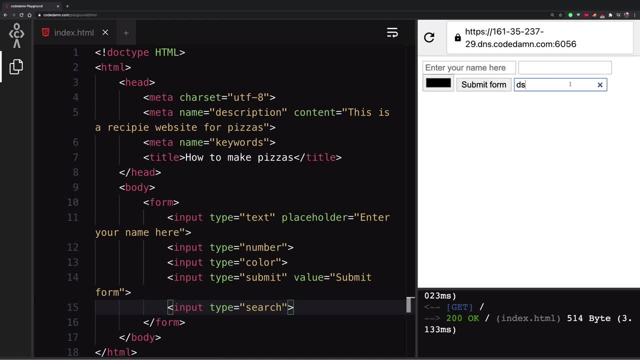 This is a pretty much input type text, but with a cross button. you see, when you type, it automatically gives you a cross button which, when you click on it, it clears the text. That's basically it. right, Pretty, You can just go ahead and achieve the same thing with a very small sort of JavaScript. 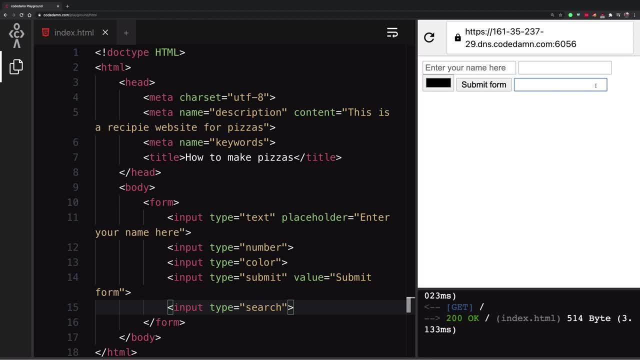 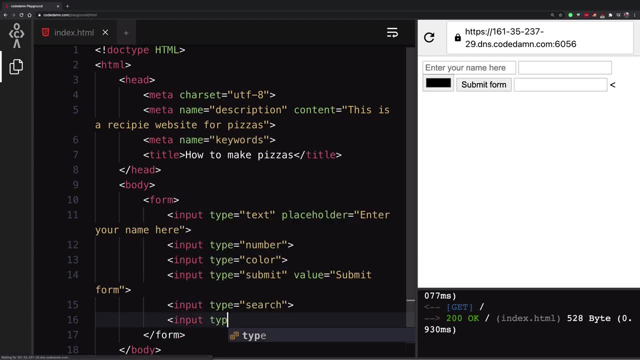 and CSS lines, But it's good to have sort of internal features like this also. So there's that. Then you also have input type range right, And once you do this, you can specify a min and max here, which makes much more sense. 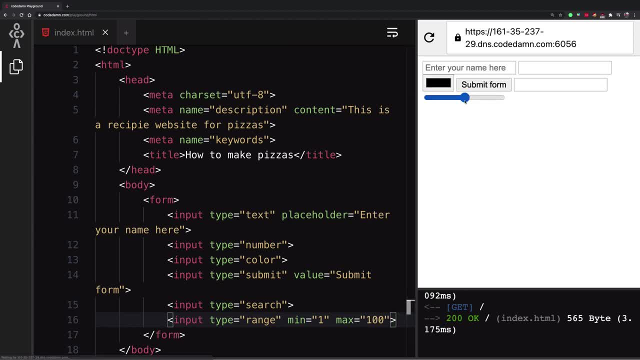 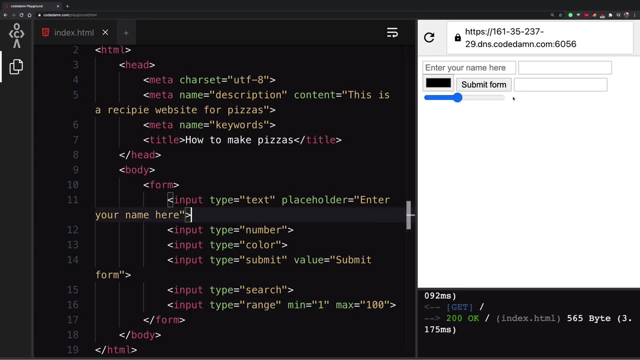 Minimum one, maximum hundred right, And once you do this it's sort of you know you're not really sure of what where the value is. You can add a little bit of JavaScript magic here to reflect the value, but I think you 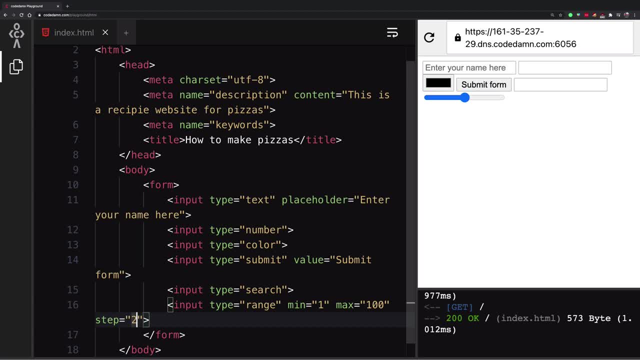 can also specify a step function- not really a function or value- step of two, right. So this increments and decrements in twos. So the minimum value that could be is two in this case, and maximum, or maybe like not really two but one, and maximum could be 99.. 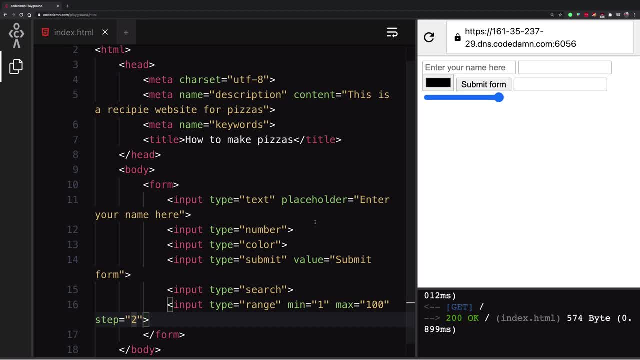 Why? Because you start from one all the way to 99.. If I probably just keep it like 30,, you're going to see how this differs. So you can see. now it just increases in chunks of 30, right, It starts with one. 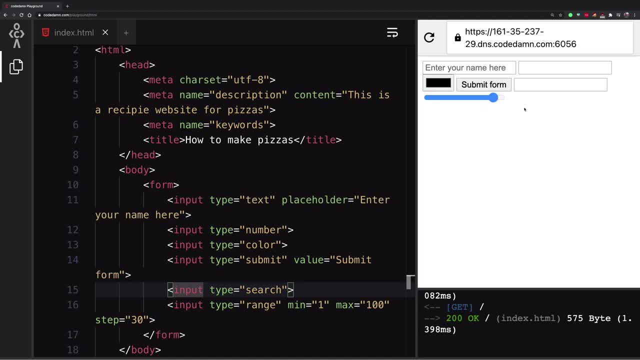 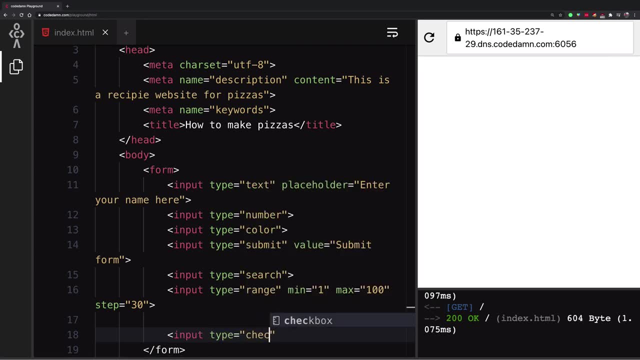 31,, 61,, 91.. That's it. You cannot really go further, So there's that. Another one is common input type checkbox, right? You know you might have seen this all the time. Do you agree to sell your data? 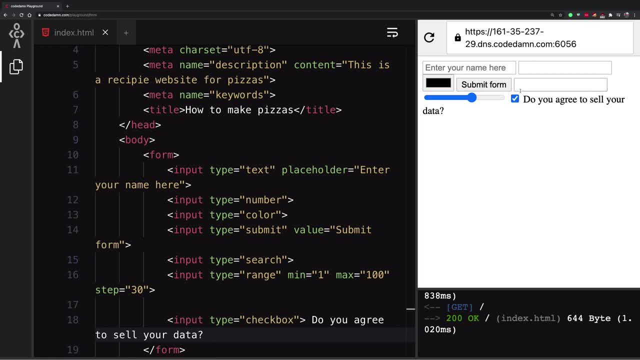 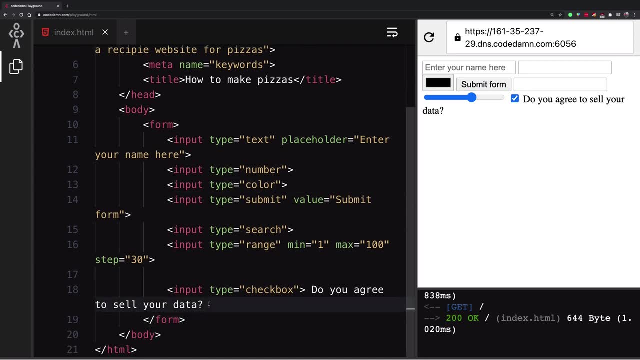 That's what Google asks you, right, When you sign up your account. you check this nicely and you click on summit. So that's how you create it for your own website as well. And yeah, that's pretty much it. I think I can just remember a couple of more input type: date, time or maybe like it was. 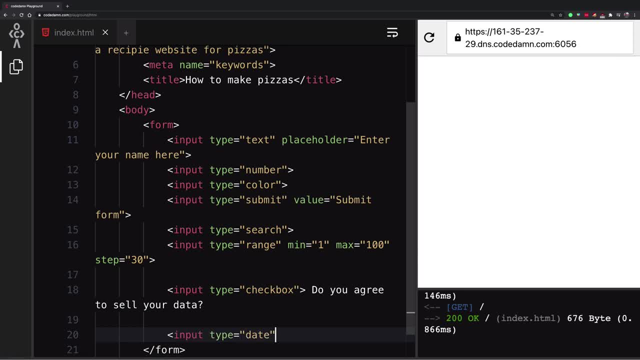 just date, I don't know. Input type: date. Once you do this, yep, You can see it has a nice interface for picking up a date and this is all provided from the browser itself, right? There's no JavaScript, no plugins at all, but again, it comes with a cost that different. 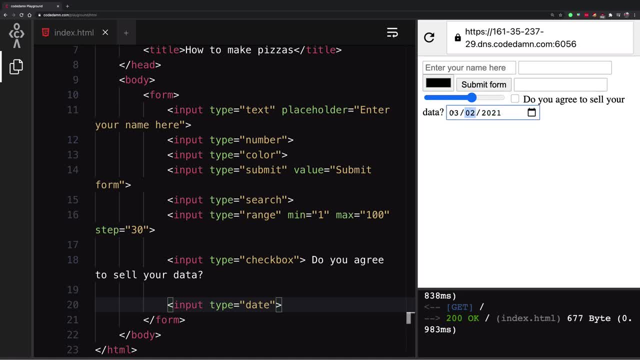 browsers will have different interfaces, So if you want consistency, then you might need to go for the JavaScript option. but yeah, the sort of really works without somebody just using JavaScript at all, which is also pretty cool. You also have a date time sort of thing, right? 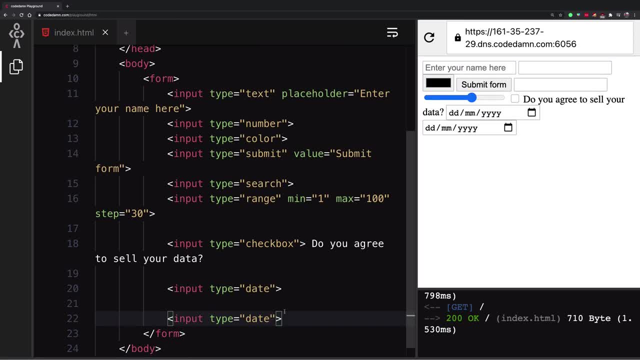 So if you just don't really want date time, you know date for the person. that used to be a date time, but you can see it is not deprecated. It's actually removed, not even deprecated. There's the state time, local thing, right. 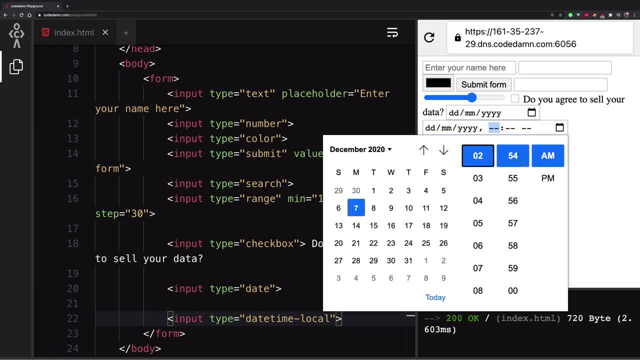 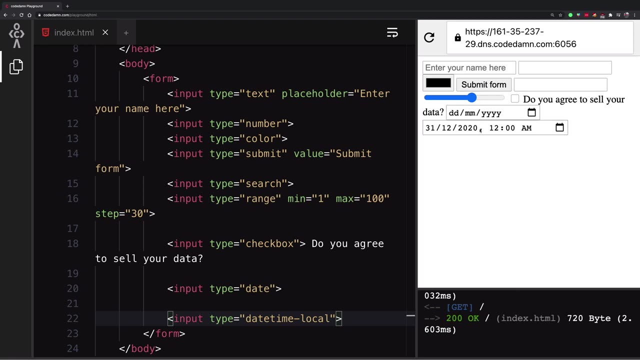 Which allows you to pick not only the date but also the time, So you can select. let's say, I don't know. Let's see: Okay, December 31st, 12 am, New year's time. Hopefully, everything would be fine in 2021. 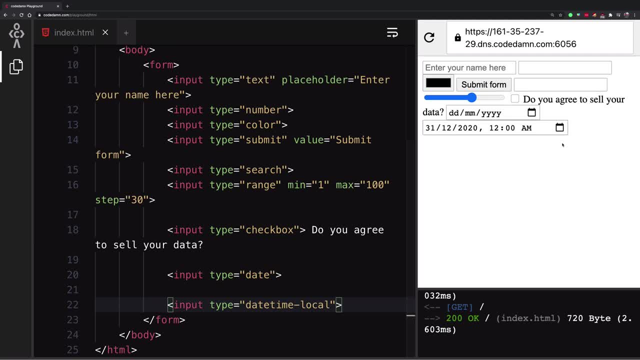 Let's assume and let's hope, And there we go. You can have a summit button and that will do the job. So, anyway, that's. that's another one in the bag. Another one which I can think of is probably input type button, right? 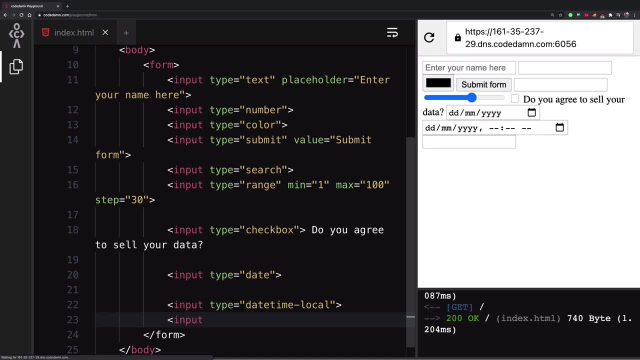 So, for example- I don't know, this might be just for fun or playing- I haven't really seen any use of input type button in the wild, but yeah, you could probably use it for loading data or something, but because there's already a button tag, that's. 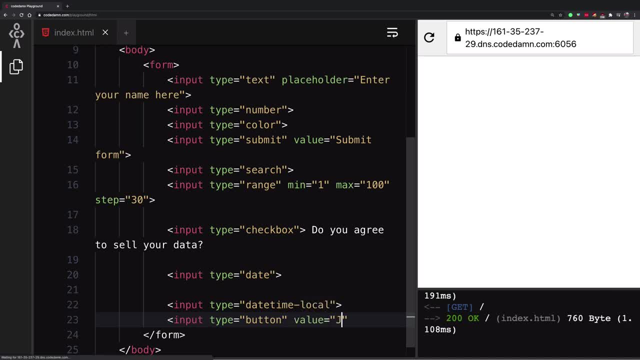 why. that's why I'm saying: but if you haven't put a button just for fun, you can have something like this and it'll just appear like a button, a regular button. You can just mess around with it. It will not summit the form, because summiting the form is the responsibility of input type. 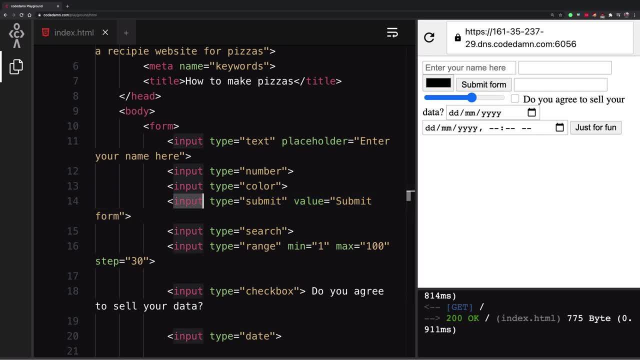 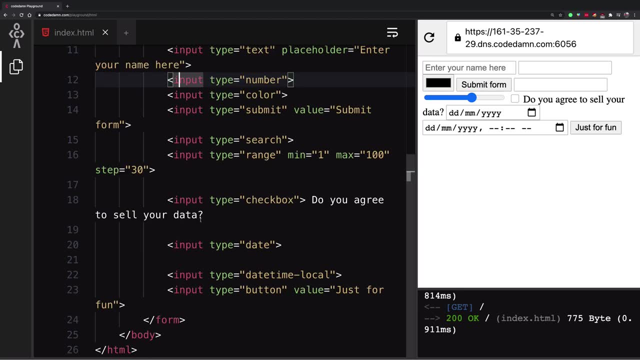 summit, which you already have, Right? So yeah, that's, that's pretty much it for, uh, this video. I think I have covered a lot of buttons and stuff. You have like one more thing to go. I would just say input type. 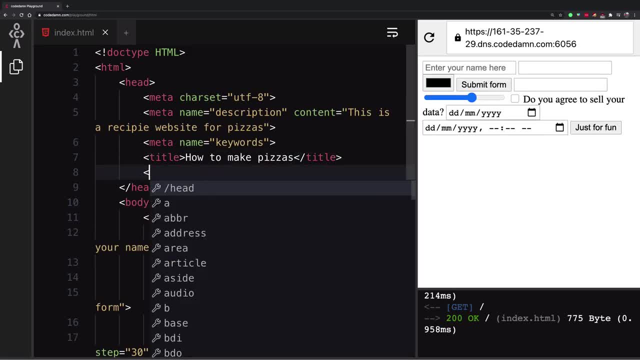 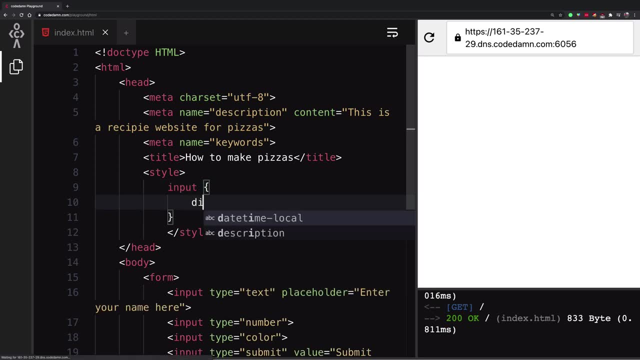 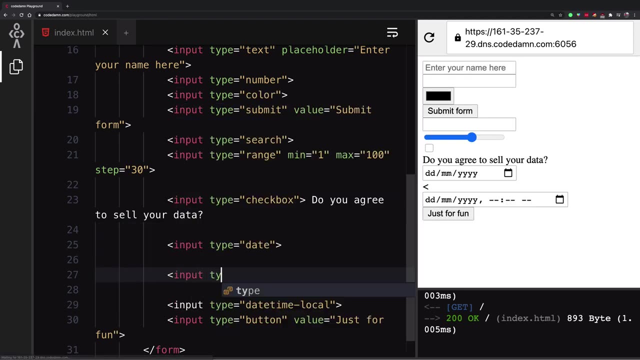 I'll just go ahead and, you know, make sure that all the inputs are block level so that we don't see them in line. So input display block: Nice and easy. And now I can just go ahead and add input type radio, also a fun and very common option. 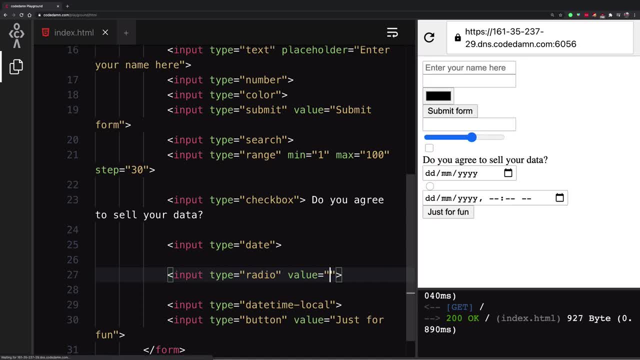 And I can say this is a value one, while this value would not really reflect on the page directly because you have to give it a label here, label one. but this has a fault because, you know, with input type radius, you will often see that you can only select one option. 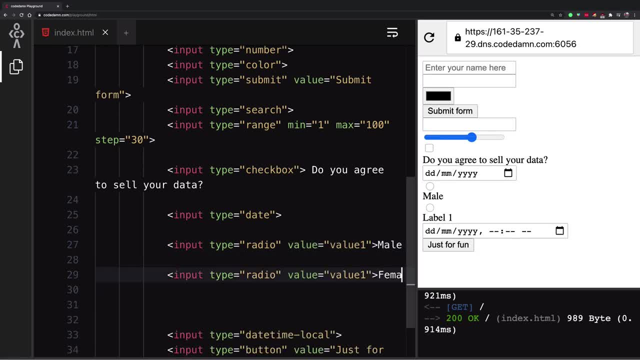 right. So if I'm asking you on gender- male or female- Yeah, So you have to select, like this one or this one, right So this, right now, it selects both. So we don't really want that to happen. So, in order to do that, how HTML works is how it can distinguish between, maybe like: 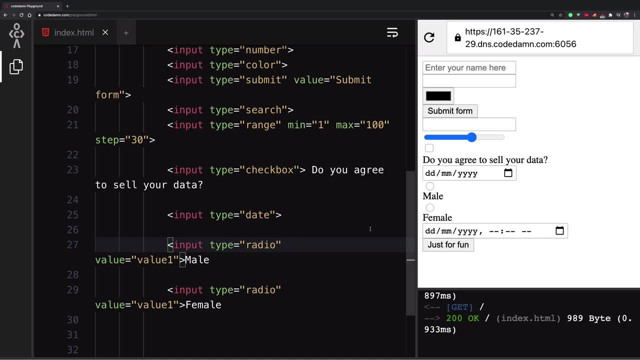 not really distinguished, but tell that: Hey, these are the part of the same group is using the name keyword So you can group them by saying gender right And name gender right here, Right, So you can now select this, this, you know now this. 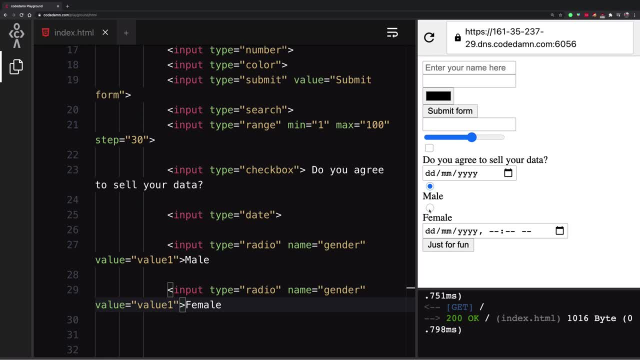 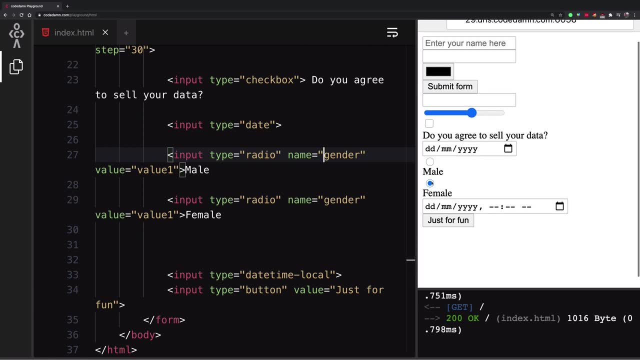 Right, You know now it does not allow you to select both of them. So there's that. So, yeah, that's, that's basically it. I guess nothing much into the input fields. You can pretty much create all sorts of forms and inputs and all that stuff just using these. 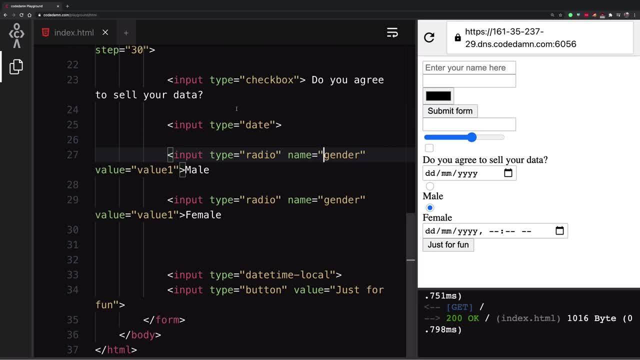 all these input fields. If you want to learn more, you can always head to MDN and Google stuff. but yeah, that's that's how much you would need eventually. That's all for this video. I'm going to see you in the next one. 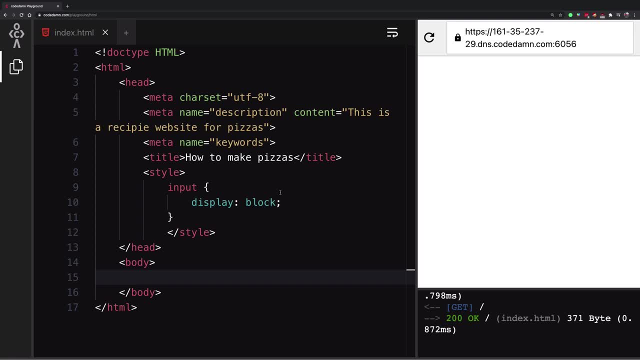 Hey everyone, Welcome back, And in this video let's just quickly go over through what an iframe is. Iframe is sort of a special tag in HTML and one of my favorites because it sort of allows you to, you know, explore your way into external web and actually provide interactivity from. 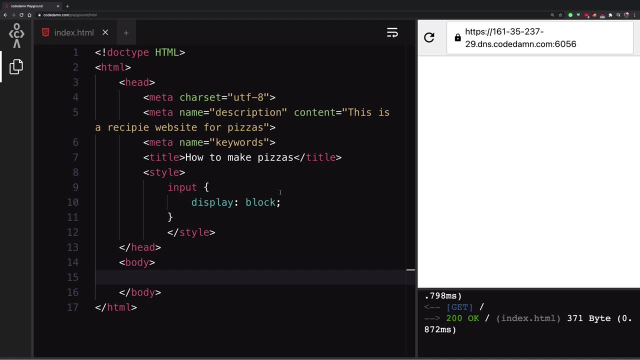 external websites without leaving your own websites. and hear me out, There's a big asterisk over there because not all websites- in fact most websites- don't allow this to happen. Let me tell you how this happens, first of all. So I'm going to have an iframe tag and I'm going to give it an SRC of, let's say, codedamcom. 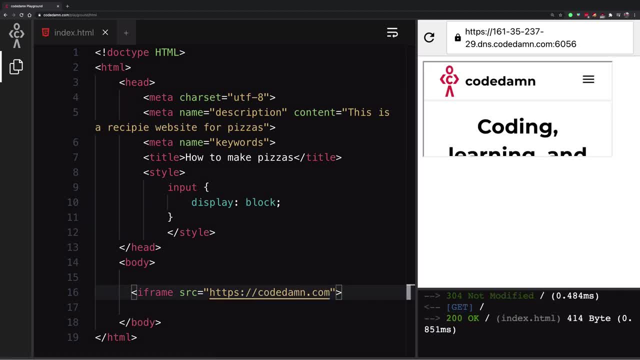 because I know it is not restricted as far as I remember right now. Yeah, So you can see this webpage. this 161, 35, whatever it is- is able to load codedamcom like this, And it sort of loads in the mobile preview because the iframe is a small. 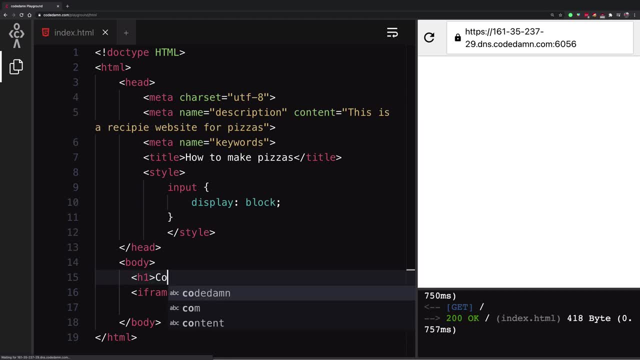 So what's happening here is, I can just go ahead and say codedamcom, Mobile version Right, And I could sort of like give you a look and feel of how this would behave in a mobile version Right. I can go ahead and say iframe width: width 300, height 300, and I'm going to say border. 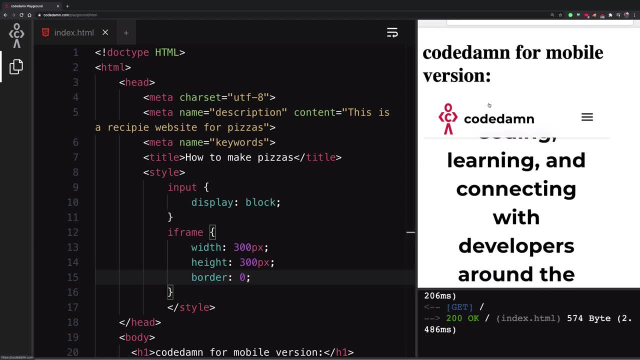 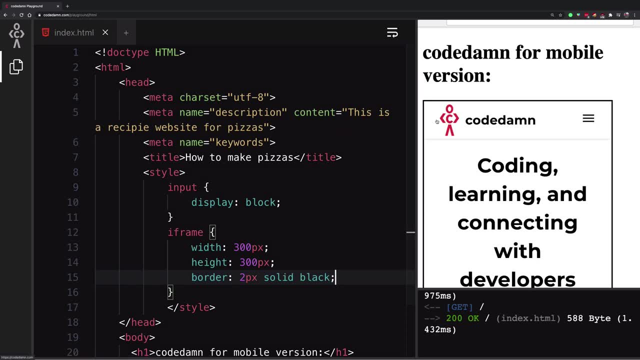 0, so that I just remove this thing Right. So now you can see it's sort of- or maybe like border 2 pixel, solid black, or if you are more creative, you can sort of have a form, A form like background. 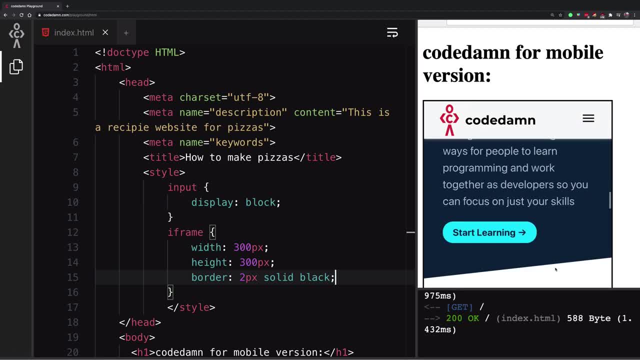 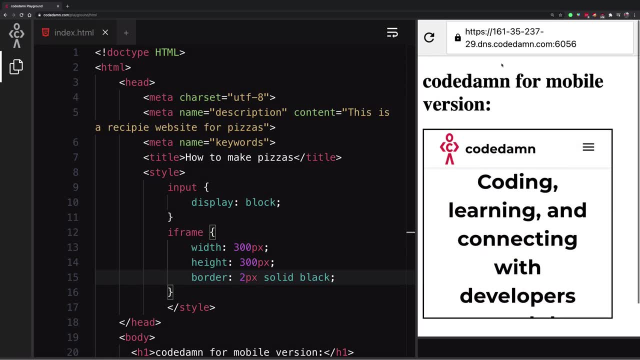 Right, So you would have a very nice interface, So you can sort of see, like, how this thing happens. Right, So I'm actually embedding a whole different domain inside another domain, Right? So yeah, that's, that's pretty cool actually. 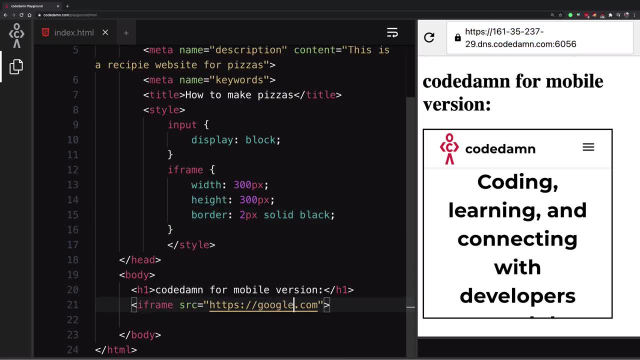 But you're going to see most websites like, for example, if I try to embed googlecom, you're going to see that you pretty much get nothing. And the reason for this is if I just go ahead and open this, Okay, So if I just go ahead and open this in a new tab and go to the console to see errors, you're 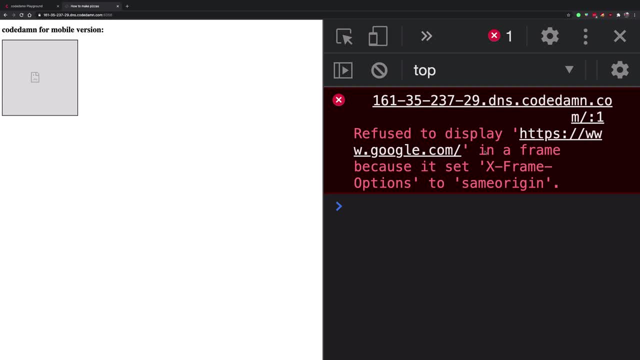 going to see that you get a refused to display googlecom in a frame because it's xframe or options are set to same origin. What this means in layman language is that Google says that I will not allow myself to be embedded into any website, except if it is coming from Google's domain itself. 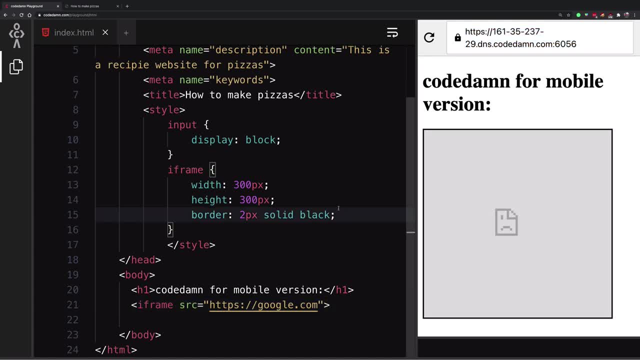 Right. So first of all I'll just- I'll just not really go into the security- implement implications of why websites don't really allow this, but you can think of, you know in this way that this, this sort of behavior, is not secure. 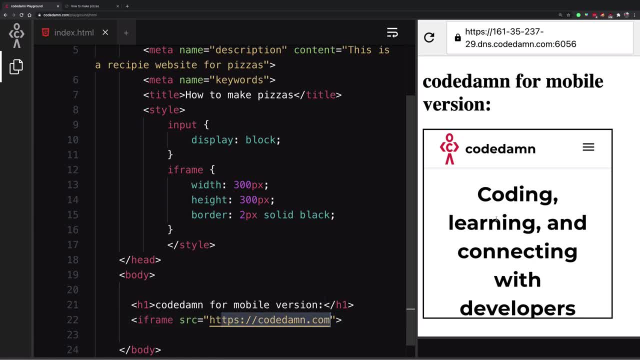 Even I should not really allow this to happen, but for now it sort of works. So if you're seeing this in future and go downcom does not work with iframe, you know why? Because I woke up one day and just just decided to make this as a security thing on go down. 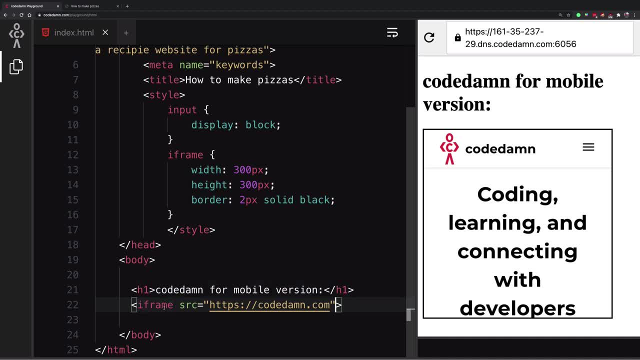 as well. But anyway, what iframe allows you to do- you might have seen now- is that it allows you to embed, embed different content altogether from another page itself, Right? So one very sort of example, very nice example of this, that if you want to embed a YouTube, 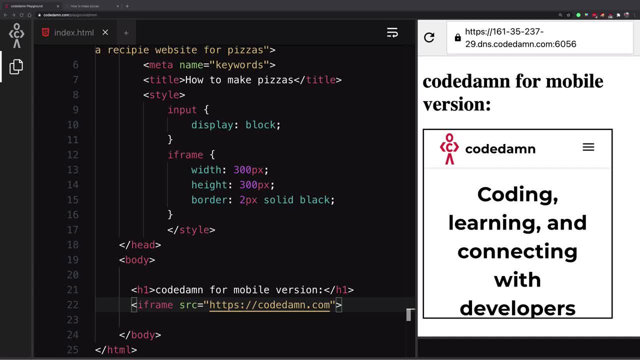 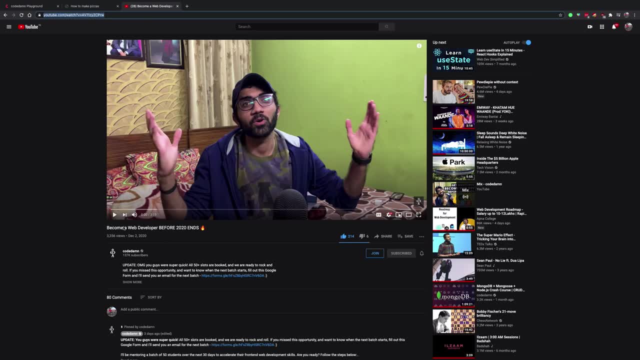 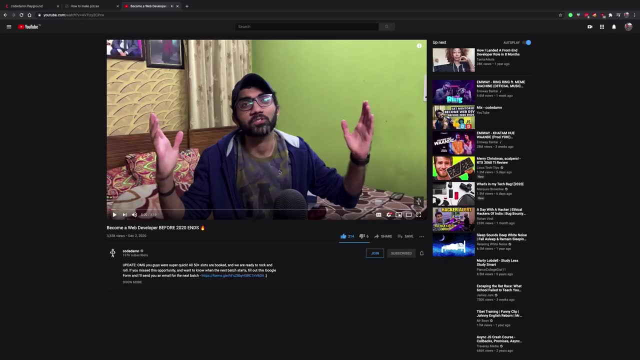 video. let me just show you a real simple YouTube video. Let's see if I can find any good. So this is my video from my YouTube channel code now and I'm just going to go ahead and embed this. not really like this actually. just go back and go to the share section and 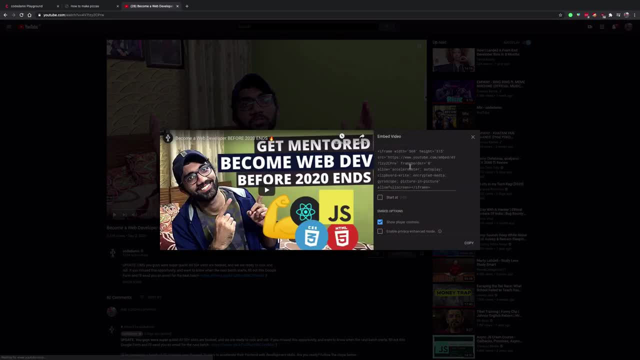 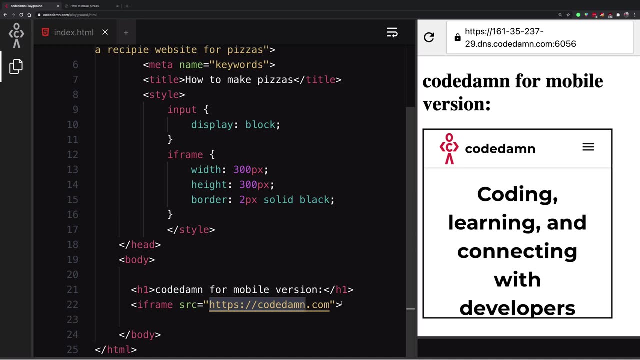 right here inside the embed. click on this and you can see YouTube actually gives you an iframe code. Again, you can see it's not really giving you any nasty scripts or anything, but it's actually giving you an iframe code with an SRC attribute, pointing to something like this: 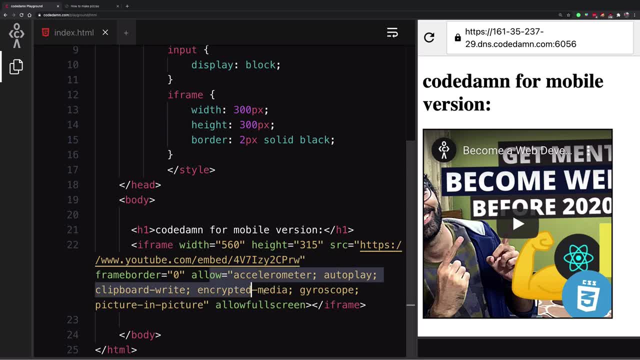 youtubecom embed in this and all the other stuff, right, So you can probably look up this if you want, Uh, but this just means, you know, having certain ABI accesses. but this means that now you have embedded a YouTube video nicely on your website. 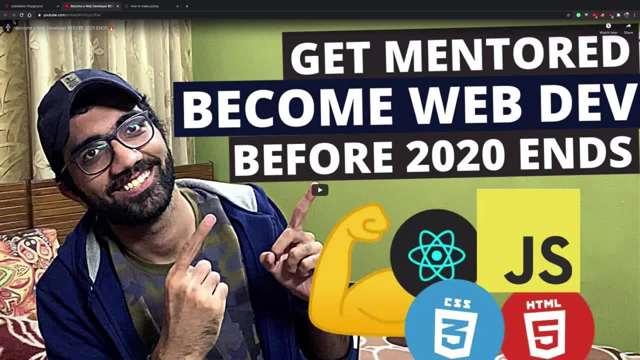 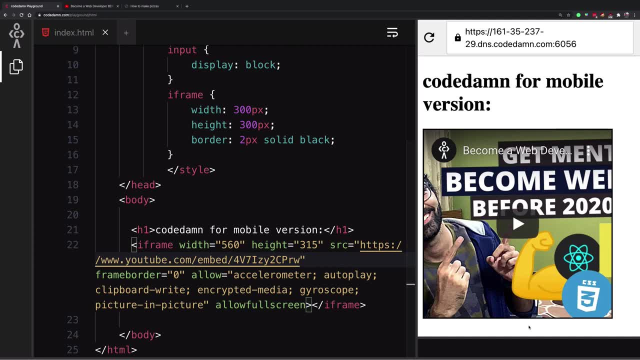 If you go ahead and open this URL in the new tab, you're going to see it sort of looks like the same way how this website, how this video was embedded, And that's why it appears like this right In the nice embedded form. 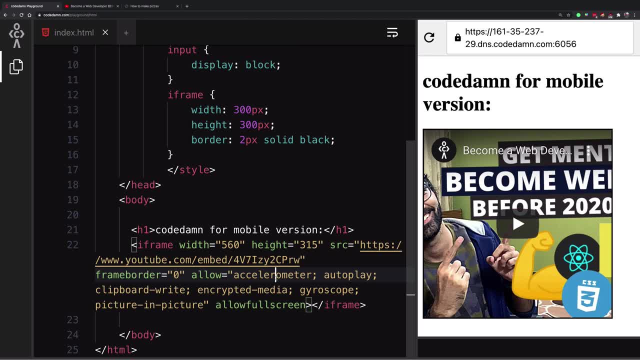 One thing you do have to remember is that don't really try to go ahead And I frame a lot of things. Why? Because you know it's not really something you should just be bothered about. If you're doing like five, 10 iframes, I'm talking about like a hundred or 200 iframes. 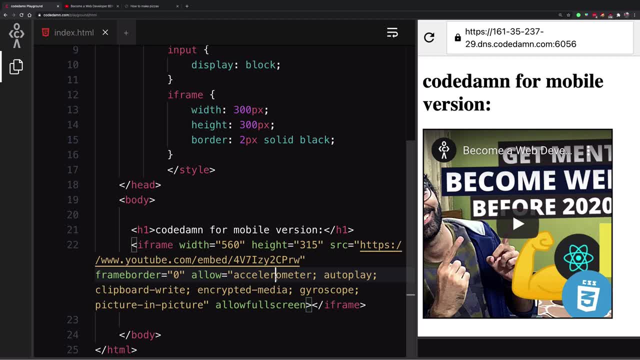 per web page, because when you do an iframe embed, the browser actually creates a sandbox environment for that particular page as well. So everything, um, in this uh URL is running in its own format, Sort of container. So you can think of: you know, this might be a bad analogy, but you can relate to it. 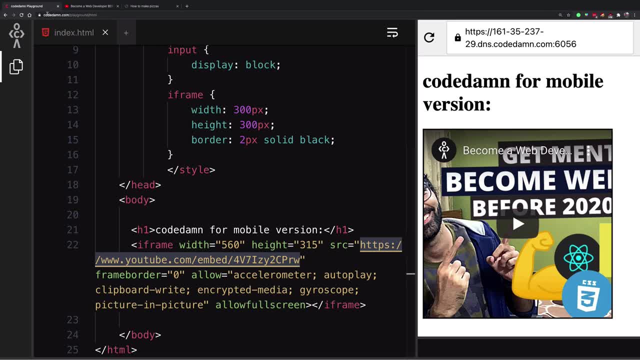 You can think of a single iframe as a single open tab, And we all know that if you try to open multiple tabs on Chrome or any browser, it's sort of like becomes very sluggish. So this is same thing with your website. because your website, every single iframe is running. 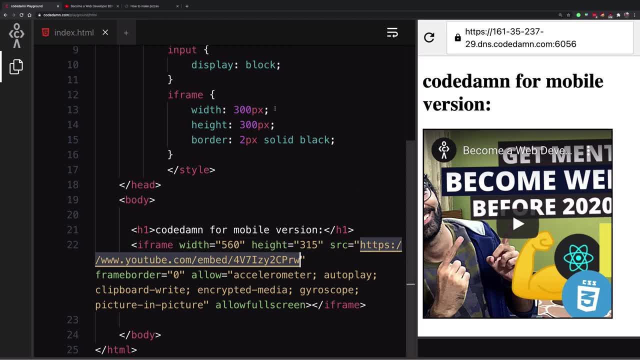 in a, in a sort of a sandbox, just like every single tab is. It would create performance issues real quick If you try to just go very convenient with the Iframe embed thing Right. So this is like something you should remember. 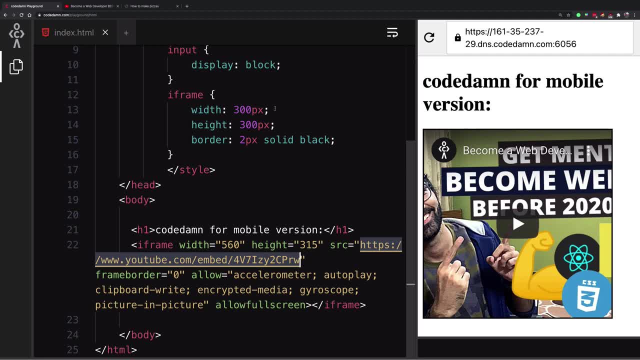 So yeah, that's pretty much it for iframes. So when you need them, you can use them, um, if the website owner allows. So yeah, very convenient. For example, right now I'm embedding the response of this domain as an iframe in this website. 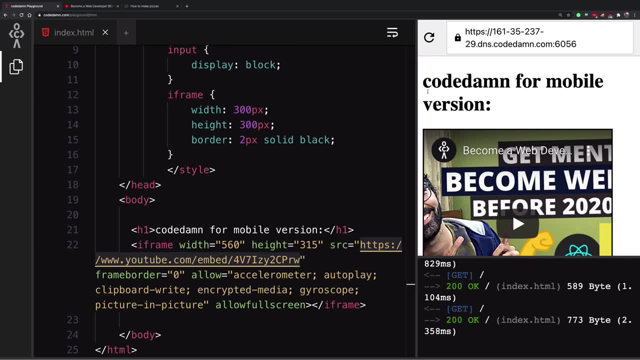 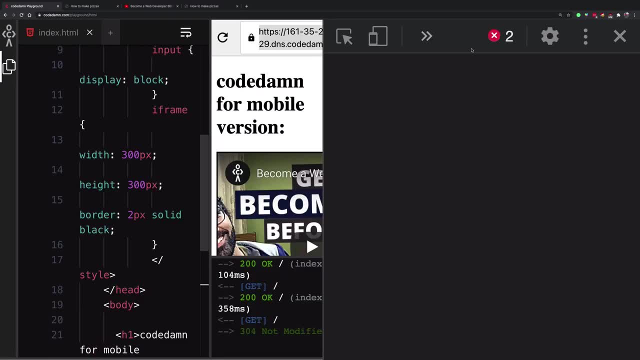 right. So the more you know how code dam works, So you can see this website. this response which you see is actually from this URL And if you just go ahead and try to take a peek into this, you could see right here. 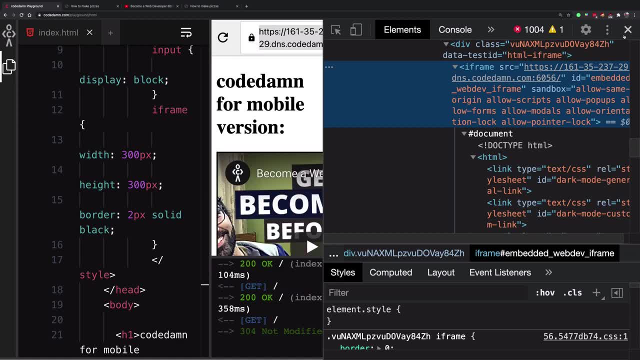 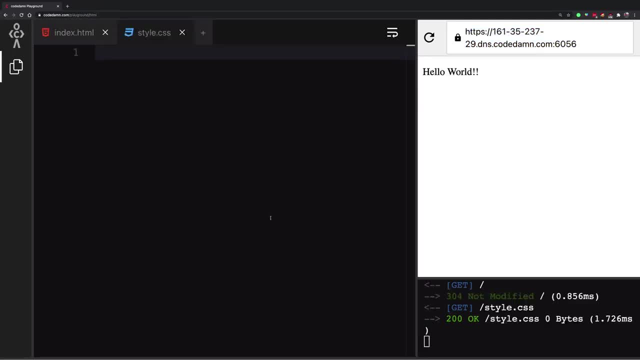 you would be able to see that this is an iframe, right? So that's how it works. So, yeah, that's pretty much it for this video. I'm going to see you in the next one really soon. Hey everyone, Welcome back to the advanced section of CSS. 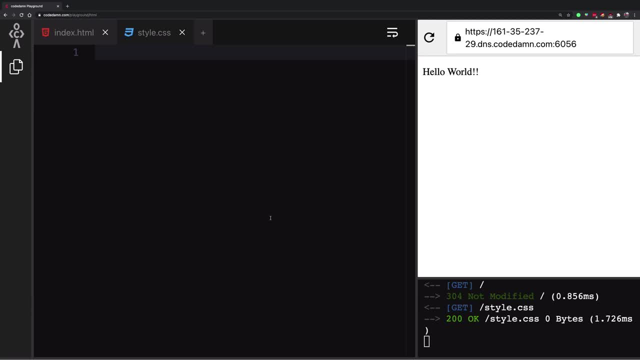 Now we're going to start with that. And in the last course, in the HTML CSS basics one, we discussed about CSS selectors, how you can select elements, How you can style them with certain properties. in this one, Let's just go ahead and start with some advanced things. 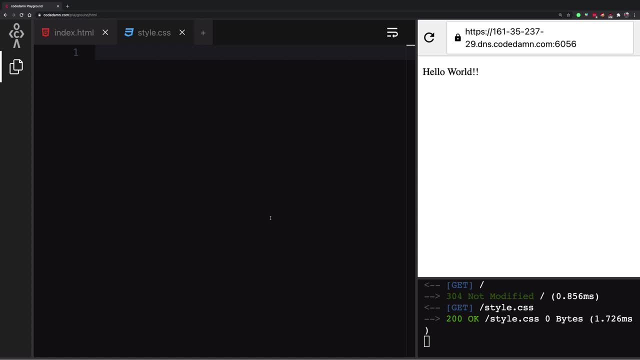 The first one being the specificity of a CSS selector. Let's just go ahead and create a style here, color red, And if we go to like the HTML document, you're going to see that we already have a P tag here and the style sheet link. 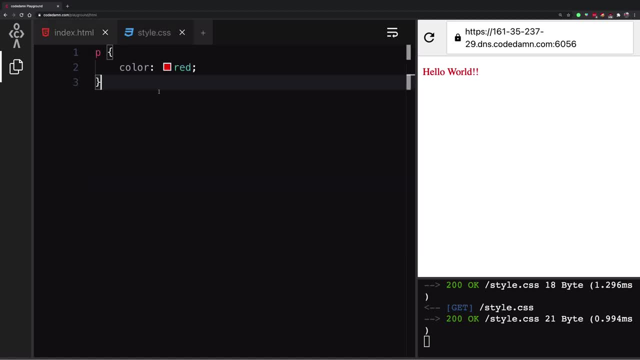 So that's fine. Now, in this case, I'm just going to go ahead and create another style, Let's say color blue in this case. So you can see that. So you can see, now it applied color blue right. Earlier it was color red. 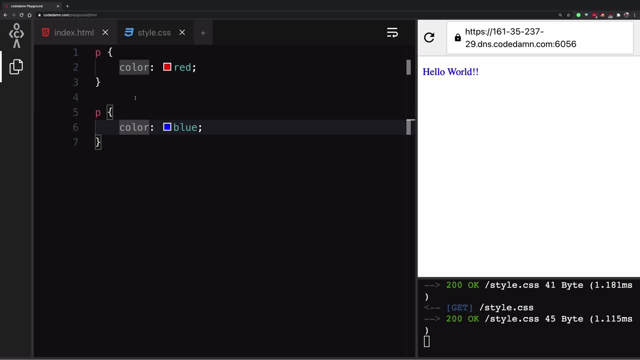 So how does CSS data mind? what to do? Is it, like you know, random? Is it like what is the order? So the first thing you have to remember is that every selector you use in CSS has a you can think of as a sort of a score, right? 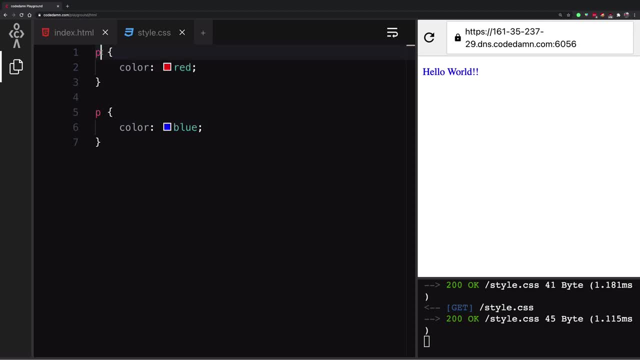 And every uh selector having a particular score. if that score is more than a competing selector for that particular particular element, then that style would be applied, For example. I'm going to leave this example for now. We're going to come to this later on. 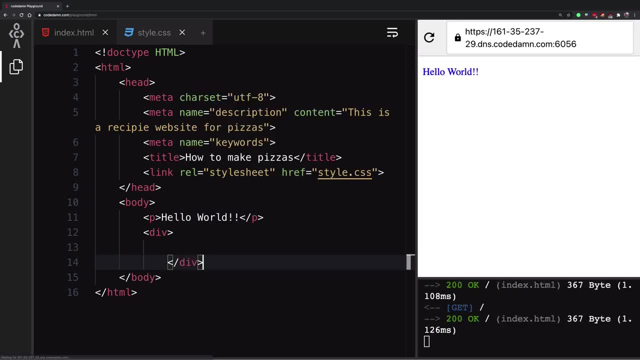 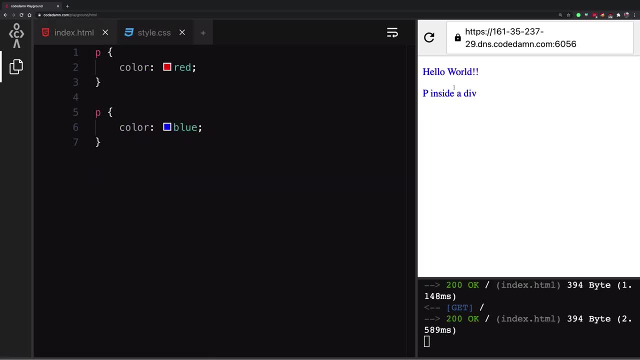 For example, let's just throw in a diff tag now and I'm going to say P inside a diff. right Now we can see both of them are blue at the moment, but the moment I change this to diff P, You're going to see. 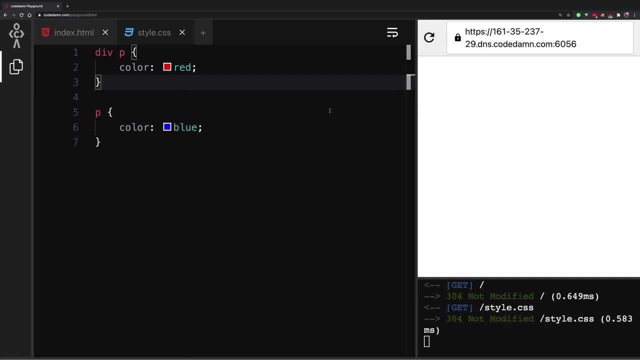 The first one Right here Don's actually red right, Even though we defined it above, and it's not not like you know, it's not, uh, sort of overridden by blue, which happened before, Right. So what's happening here? 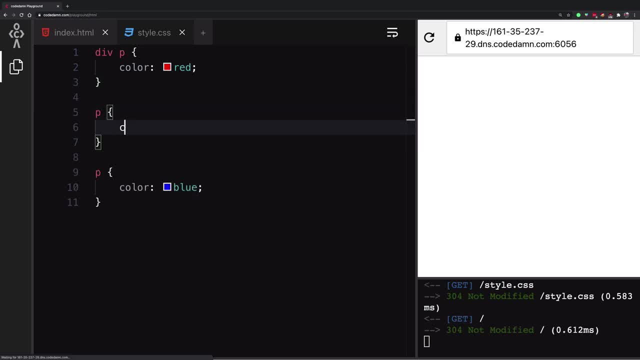 What's happening. Let me just go ahead and actually write a P color red here as well, just to make things clear, Right? So earlier we had this, Now we had this whole thing, but now this works. Okay, So we're going to write a P color red for the diff tag. 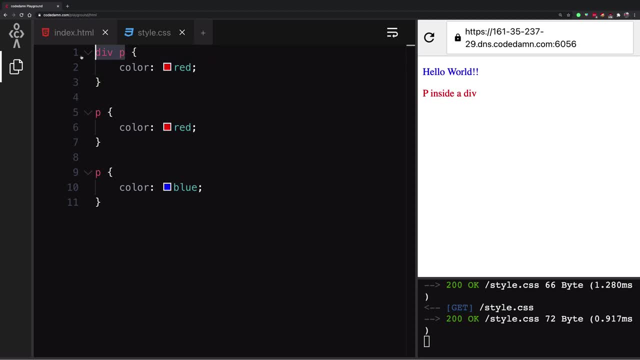 So the specificity of this selector right here, let's, let's just calculate that I'm going to have a comment specificity like this And the specificity for this selector is two. Why? Because it's a one plus one. I'm going to give it like this: 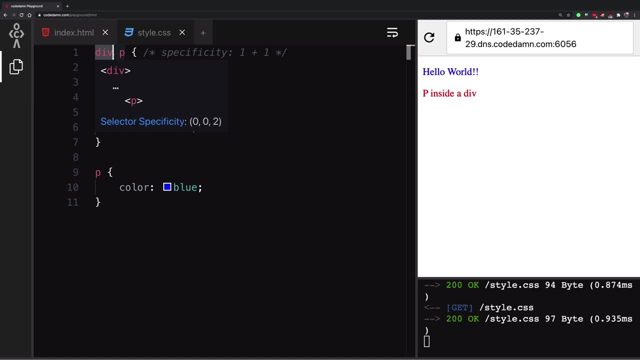 Every selector, every HTML element, as a, as a tag name. every tag name, rather, has selector one, It has a specificity of specificity of one. You can even see this thing in the, in the sort of- uh you know, sort of information. 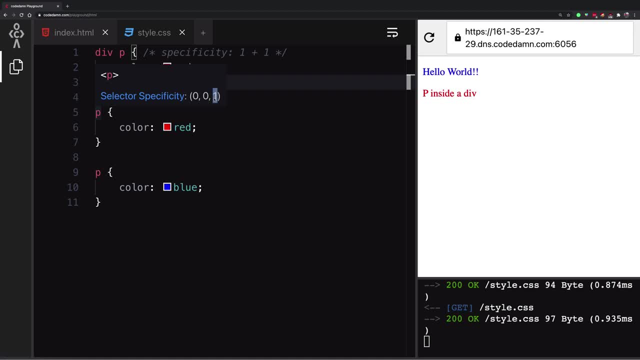 This right here. you can see if I hold over this. this has just a specificity of one. This right here has a specificity of two. So obviously this has more specificity than this one. That's why this style gets applied for the matching element. 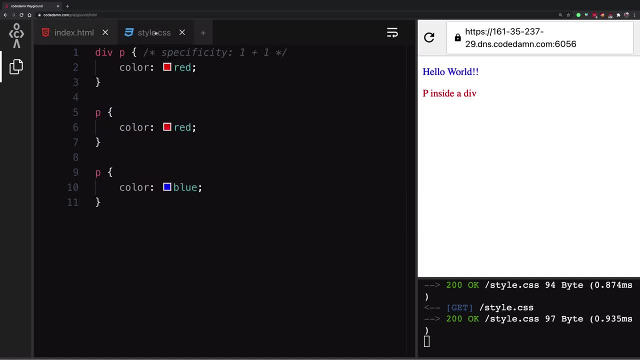 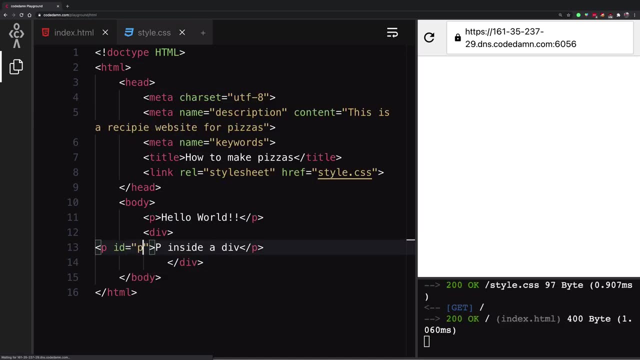 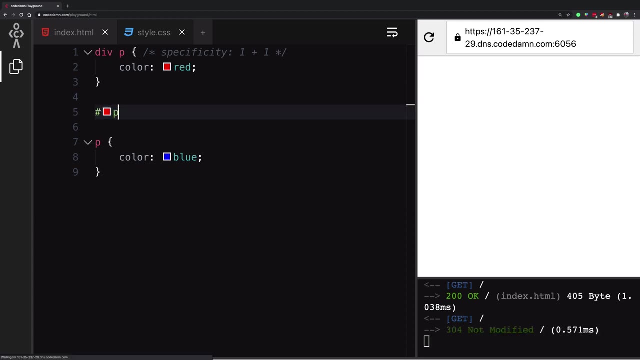 That is the P tag inside diff. Now, What about, Let's say, if I had an ID of P tag like this? Now, if I go ahead and give an ID of P tag and then say color green, what's going to happen? 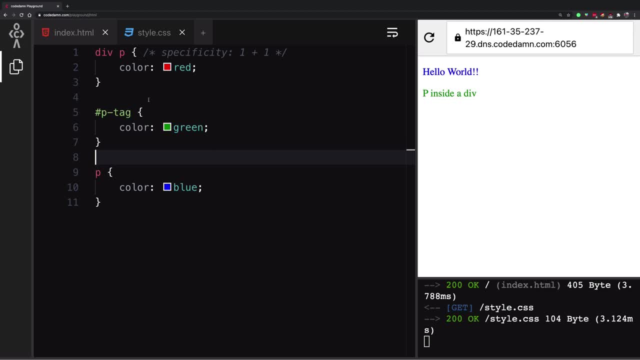 You can see it turns green right, Even though we have diff P of red, And if you hover over this, you can see it has a specificity of one zero zero. So what's happening here? What's happening here is you can think of, if you have an ID, then the specificity score. 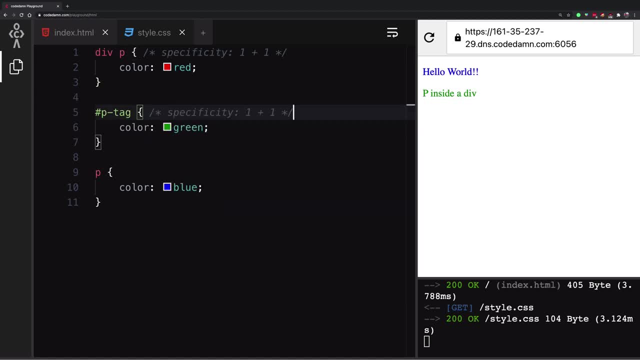 of an ID is hundred, right. So the specificity score of this thing right here is two, whereas for ID it is 100, right So it's. it's a massive jump in the specificity. So specificity just means that, Hey, how specific you are with your selector. 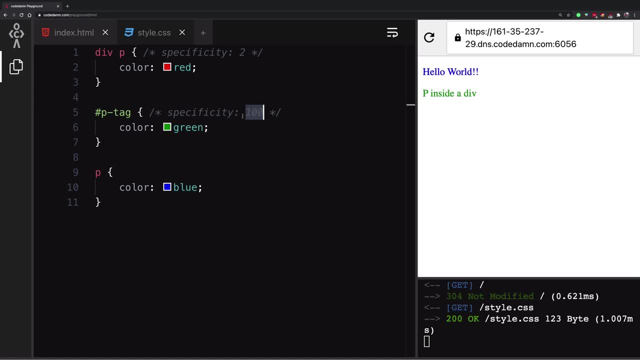 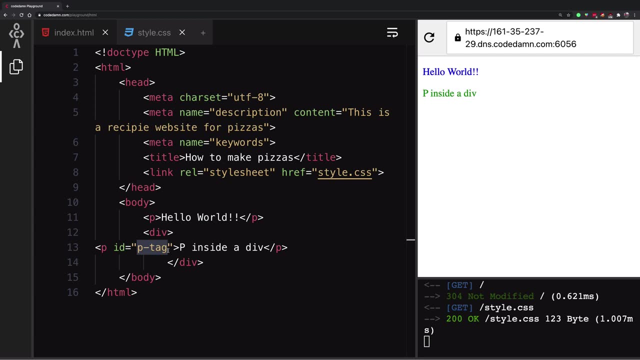 And the reason the IDs have a specific score of hundred is because there could be only one single ID on the whole page, right? So that means you're super specific on what element you're targeting, So you should always have a single ID on a specific page. 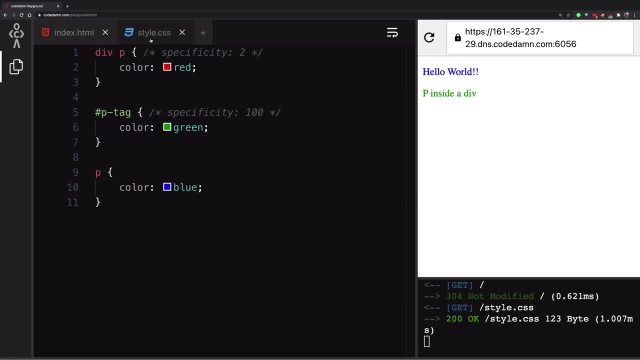 That's, that's how the semantics are laid down and the workings are laid down, And if you do not do, bad things would happen. But anyway, you can see it has a very high specificity. So, yeah, that's. that's basically one thing for specificity. 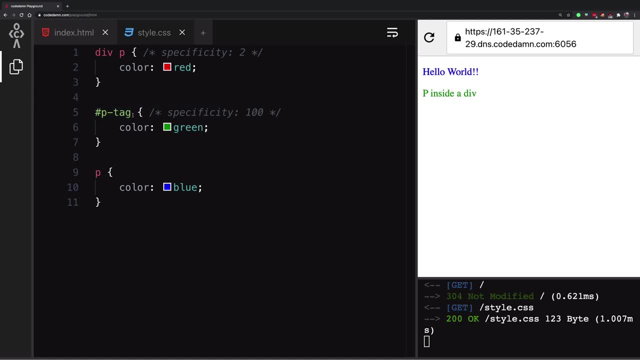 First of all. the next thing is: you can also have a class name, right? So if I have a- not really an ID, but a class of P tag, and if I go ahead and rename this like this, you're going to see the specific score of this right. here is 10, right. 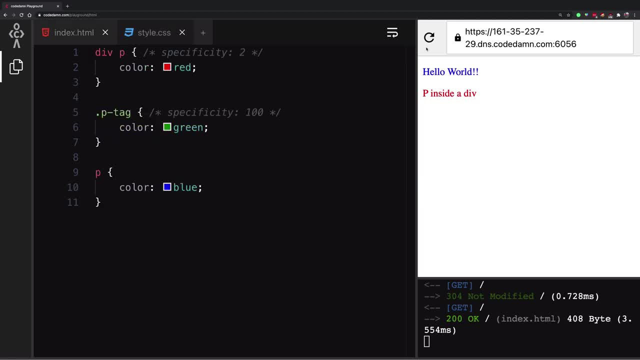 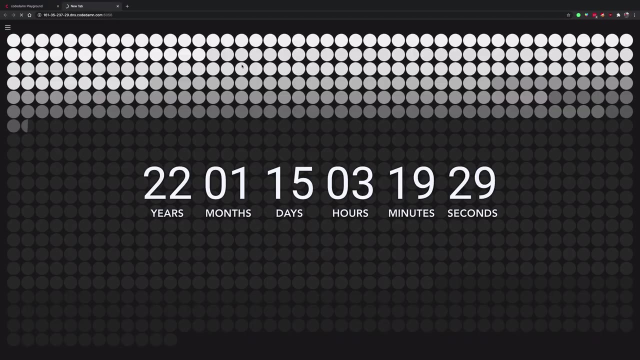 And we have a P tag class and let's see, we probably again had a little bit of caching issue. I don't know, Yep, Looks like caching issue, So let's just go ahead and open this in a new tab, rather- And now you can see that it's actually green, because you know, obviously this has a specific. 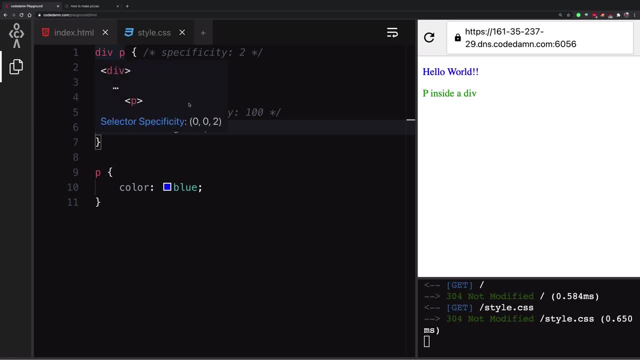 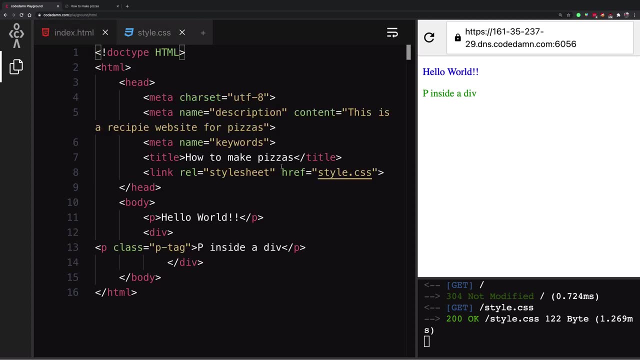 score of 10 and that specific score is still two, So this is going to win, right. So there's that. Um, yeah, so that's one thing. Another thing is that if you try to do something magical, like ID of P tag as well, 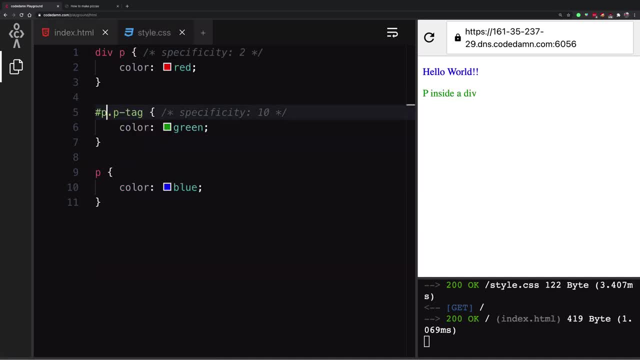 And if you try to chain these two, you can do that in CSS- that an ID of P tag and no space. remember no space, because if you give a space, that means that it is looking for that children inside the IDP tag. 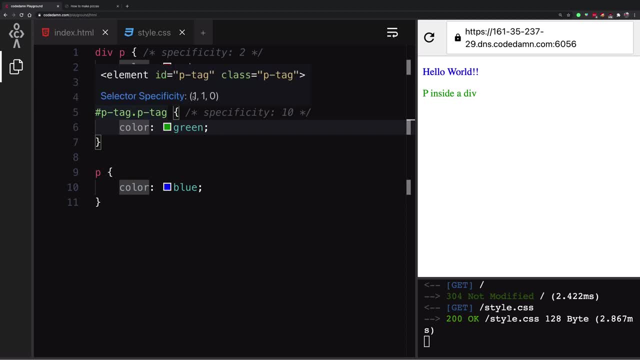 So right here you can see that this has a specificity score of 110,. just like you can see, the one hundred comes from the uh ID and the 10 comes from the class name. So there's that right. So, yeah, that's, that's uh. 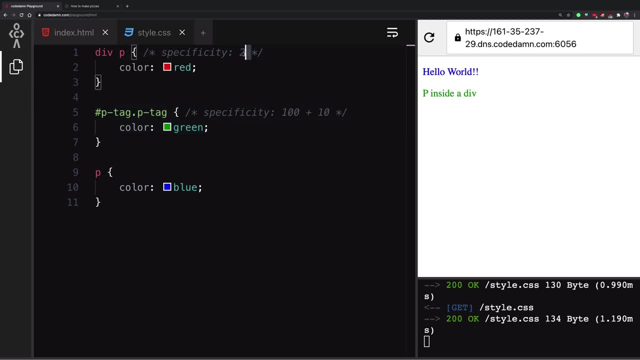 It's specific score, again much larger than two, So you're going to win. Now what you can do is probably nest more salad selectors, For example. if you're competing between these two elements, the way you can make this particular element win over everyone else is probably by throwing in more selectors like this right. 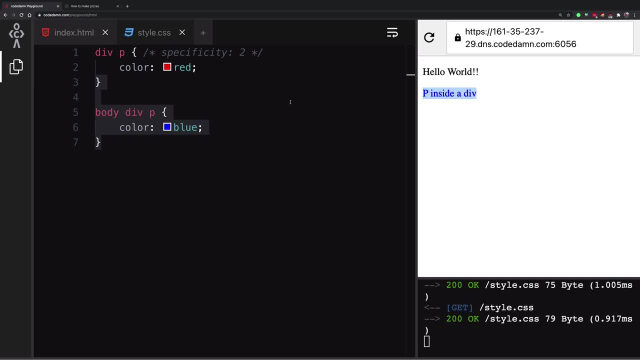 So you can now see the P inside. dev has a color of blue instead of red. So if you ever see that this is going to win, If you ever see that there are styles conflicting, that means you are applying something but something else is being shown. 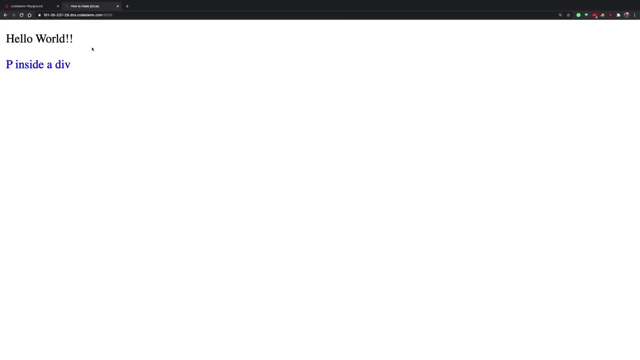 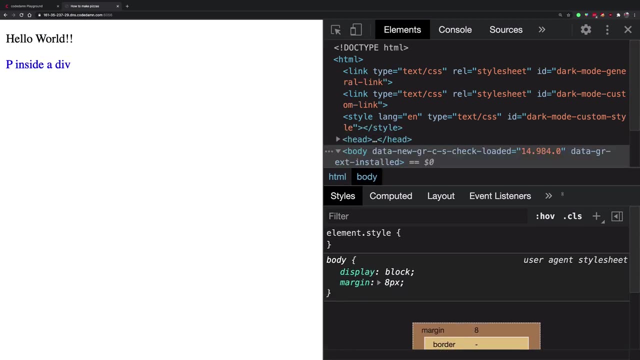 The first thing you should go do is go ahead and open that in the browser. Obviously, open your console. We're going to have a dedicated console. uh course on code dam, but don't worry about this. Just open that console. go to that element inside this elements tag. 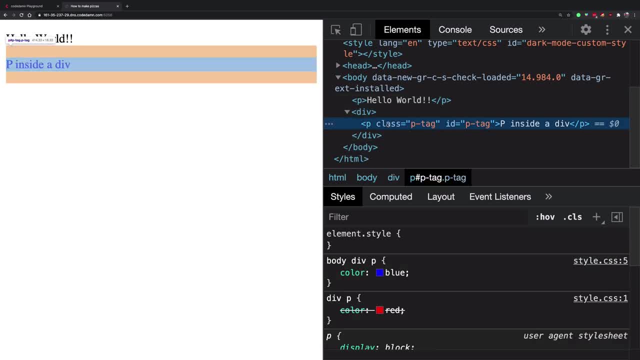 For example- this is the element I'm targeting- inside the dev tag And you can see right here we see a style which is crossed. So if your style is crossed, that process Probably means that another super style is overriding it, right? 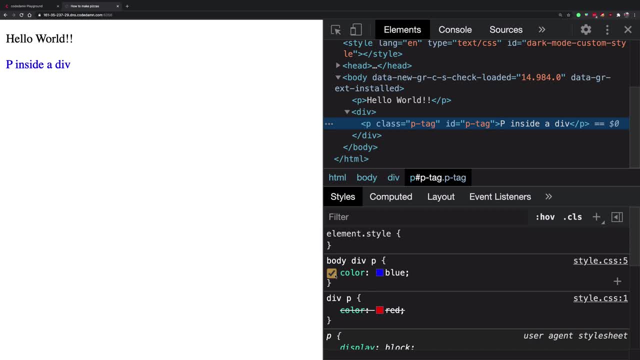 And you would probably be able to see it just above that. So if I go ahead and remove this, you can see. if the style was not present, then that would work, But if you, you know, just if you see they are stylus crossed, that means some other. 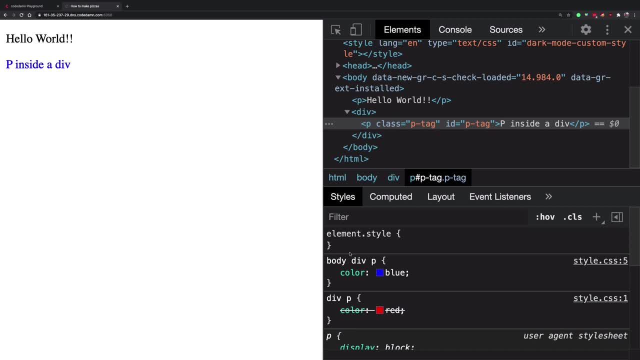 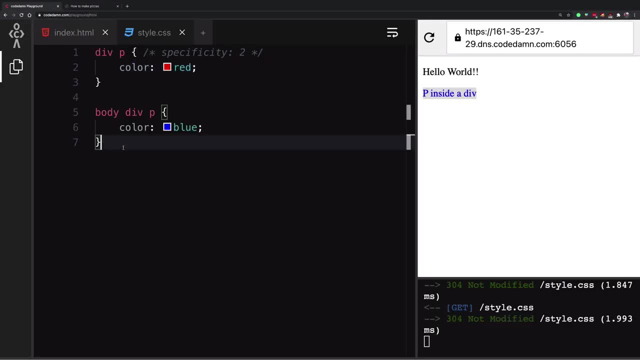 style is specificity. Some other style specificity is more than this one. That's why it, why it is overriding it right. So that's, that's a little bit course on specificity. coming to our first problem, That is, If you have a conflicting score of specificity, the style which is applied is the style which 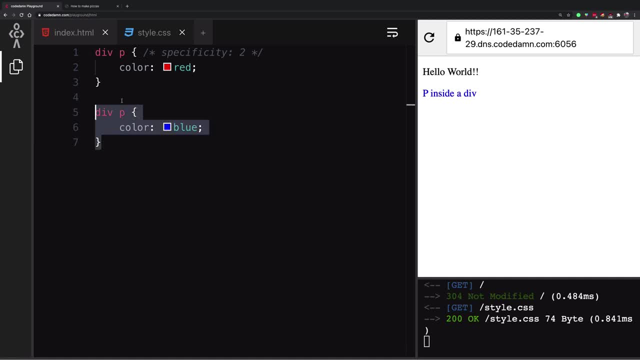 comes later, right, So this style comes later. That is why it is applied. If you just cut and paste this one, this would be applied, right? It's not a big deal, So that's that's. that's how it all works. 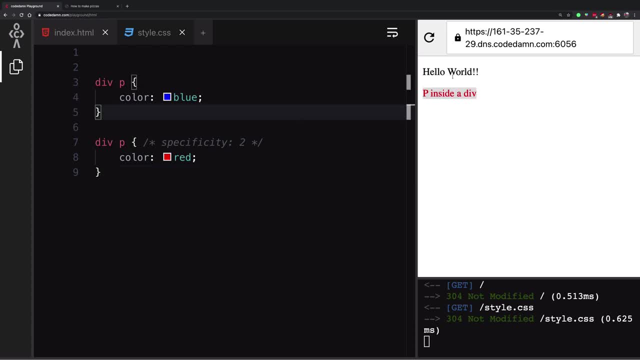 So yeah, I mean, that's that's pretty much it, How this specificity thing works in a nutshell. So, yeah, that's it for this video. I'm going to see you in the next one. I'm going to see you in the next one discussing more concepts about CSS. 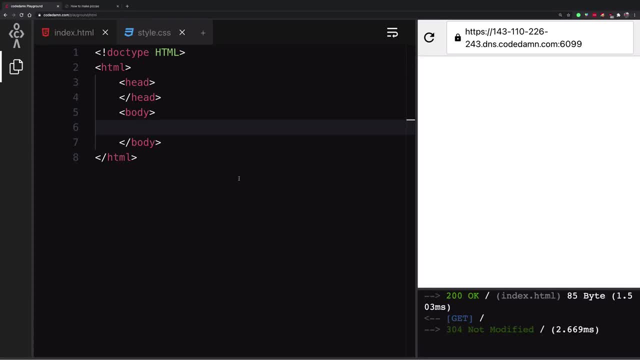 Hey everyone, welcome back, And in this video we will be discussing box model in CSS3, which is a super important concept overall. If you're learning about CSS3, this and layouts in CSS3 is probably like. I keep these two. 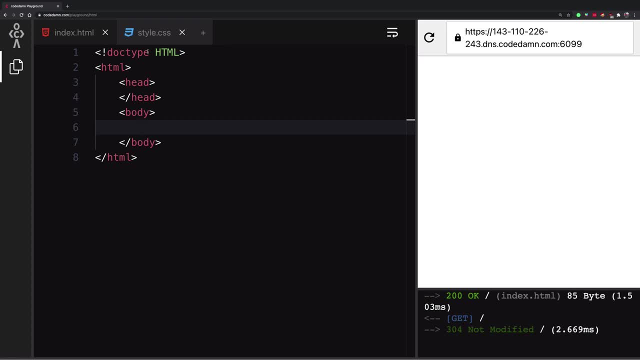 things at the top. Layouts basically means flexbox or grid systems, And if you're a 2015,, 2014,, 2013 guy, then floats also. So anyway, coming to what exactly is box model in CSS? Box model in CSS basically means how you kind of like display the element on the screen. 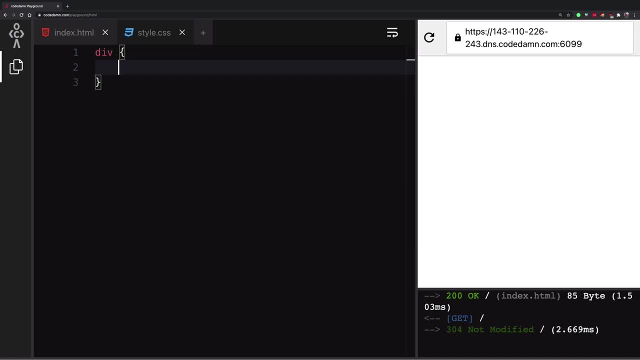 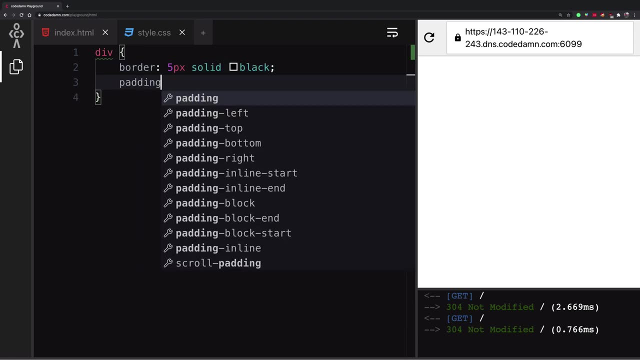 right And its properties. So let's start with a simple div tag. I'm going to give it this border of five pixel, solid black. I'm going to give this a padding of 10 pixel from every side. I'm going to give this a margin of 15 pixel. 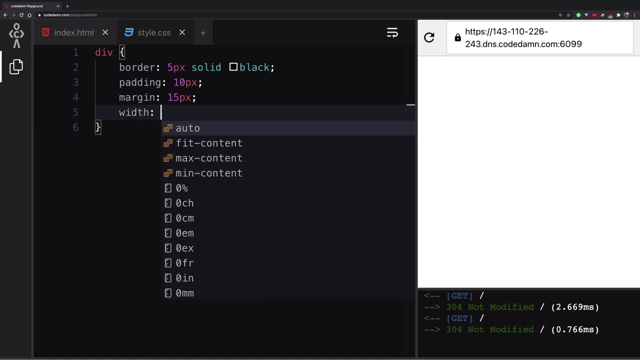 And I'm going to give this a width of 300 and a height of 300.. This is like gonna- or let's just give it a 400 height. This is going to like clear up everything in your mind, right? And I'm just also going to give this background color of, let's say, yellow, right. 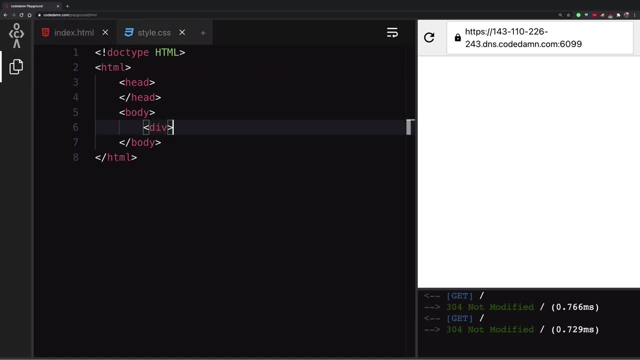 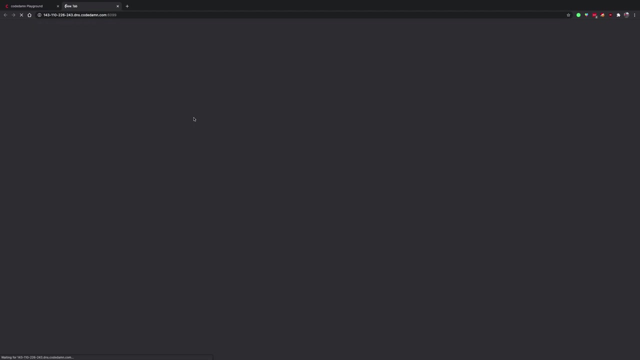 That's it, And we can just have a div of hello world right here with us, right? So this probably needs to also have a link: rel. Okay, Style sheet, href, stylecss, And there we go, right, So we have this, but I'm just going to open this in a new tab, right? 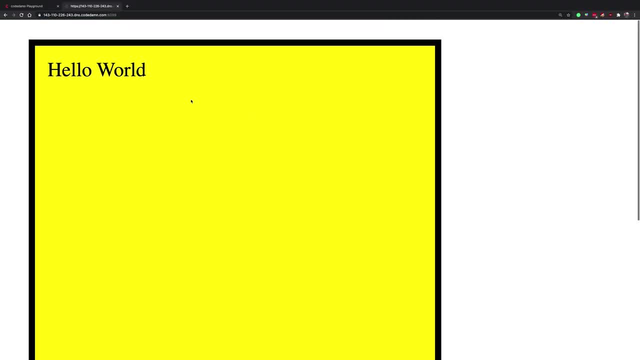 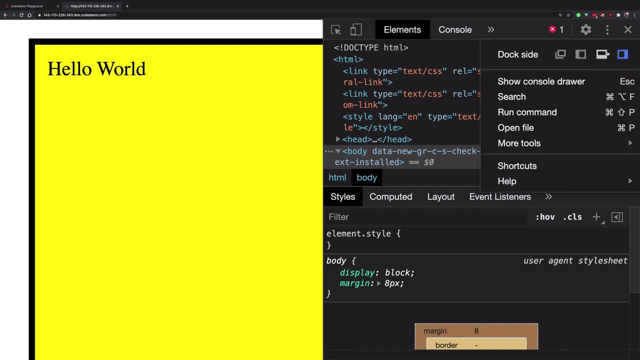 And right here we have a nice little div with us Hello world, with a background, with a border, all the good stuff. But let's just go ahead and take a deeper look. I'm going to go ahead and select this element right here. 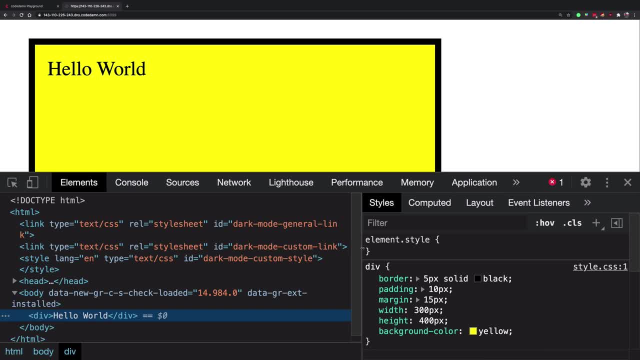 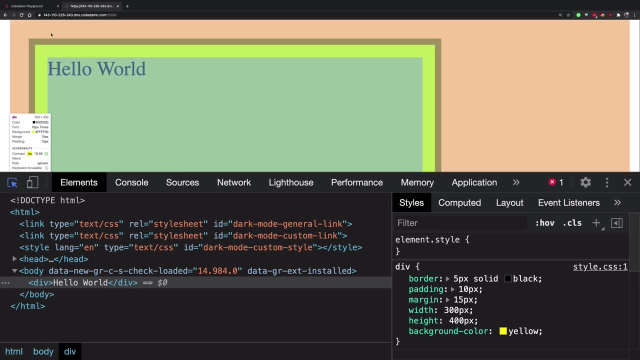 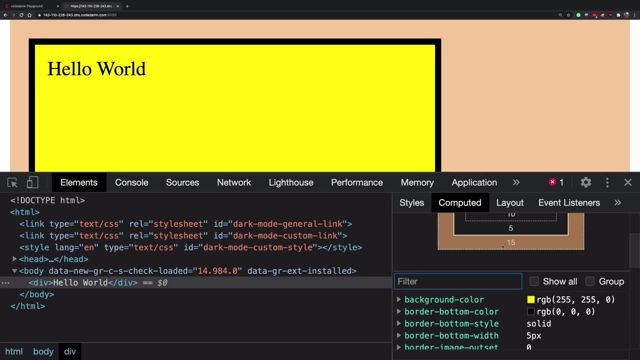 And div right here. Now pay close attention to what all you see on the screen. When I hover over this, you can see. or maybe when I click select this, you can see this box sort of thing appear, appearing right here. Now what this thing appears, I think I also have a right. 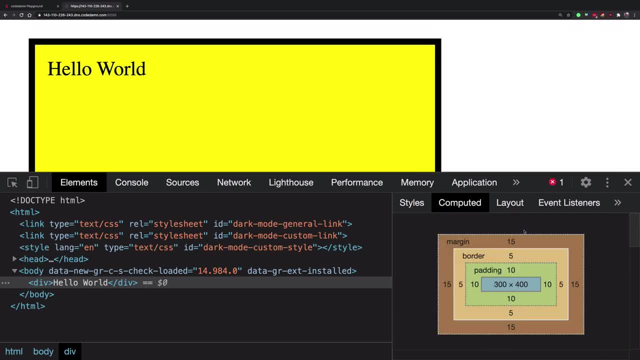 So we also have a sort of interface like this. So this is the box model of this particular element. You see, the width and height which I gave to it is the central content: Weight and height. So that is 300 cross 400, which you see right here is the, you know, is the width where. 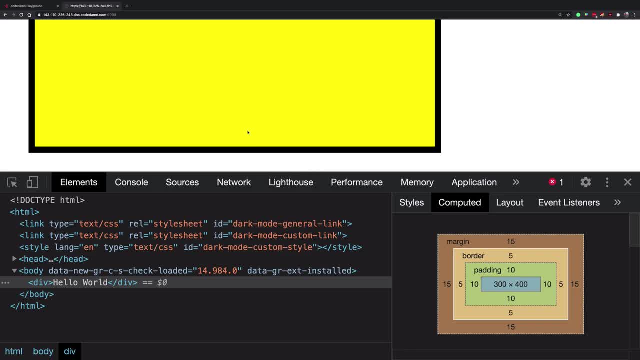 width and height where the content could live. Let me just go ahead and drop the height. Actually, it's, it's way too much. 300 cross hundred would be probably much better. right, Refresh, or maybe like 50 would also do refresh. 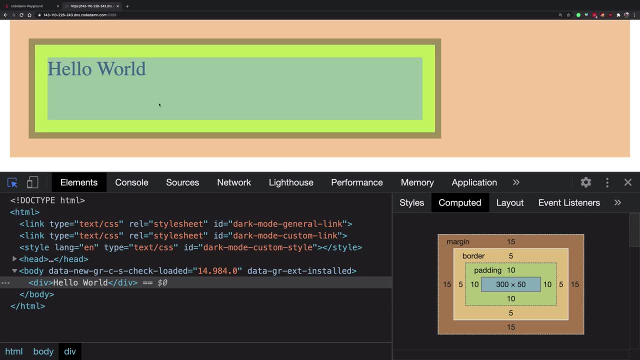 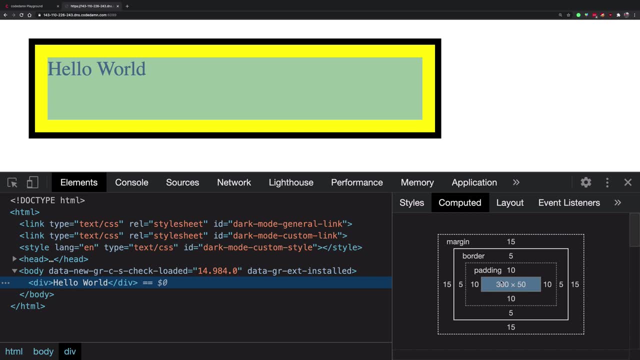 And there we go Right. So you can hover over this and go to compute it. You can see this: 300 cross 50 turns that region into a little bit blue. That means this is the region for the width and the height. The next thing is you have the innermost thing as the content. 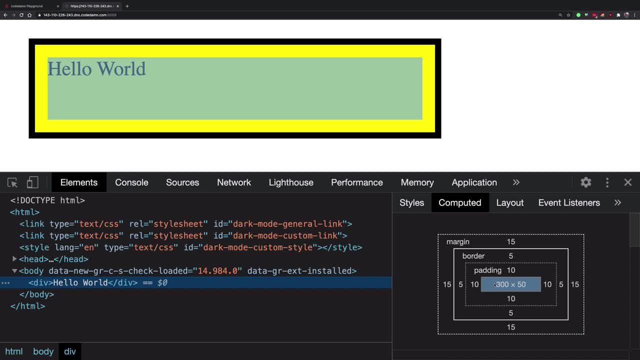 The next thing on the boundary is padding right, So your content is always surrounded by padding. Your padding is basically the amount of which you specify as how much distance do you want the elements content from the bottom? The outermost thing of an element is the border right. 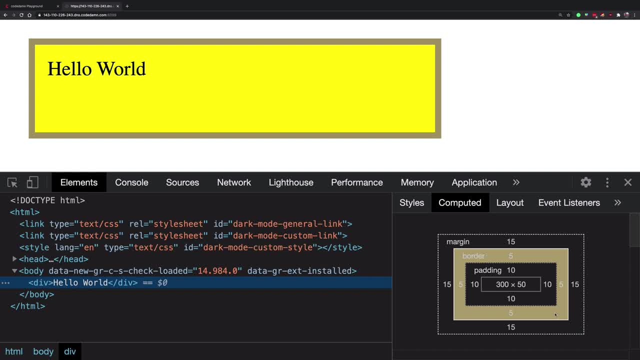 So the border right here defines the boundary of your element, And after boundary is margin. This margin right here means you know your distance from other elements or from the outside world. So this is, like you know, sort of the whole box model equation that you start from the content. 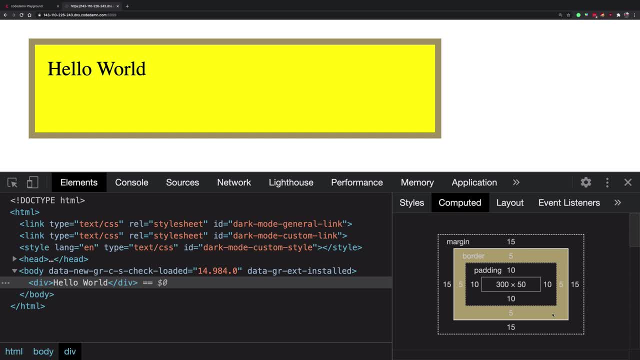 You add up the padding, You add up the border And then you get the full element right. So this is your full element on the screen. So if I have probably a click event listener or you know any sort of hover effect, 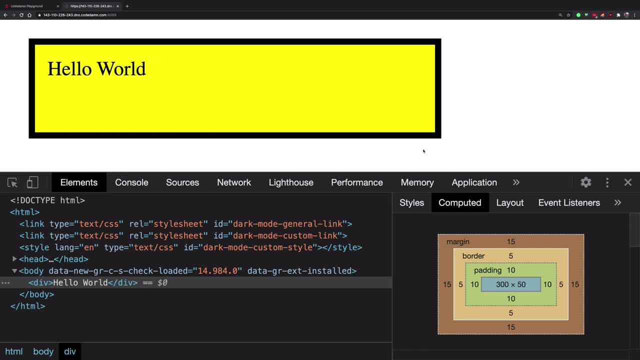 that would work, always work whenever I am at least on the border of the element, Not really on the margin on the border. So if you can see, you can observe a quick little thing here And that is that, even though I specified padding and border and all that stuff, 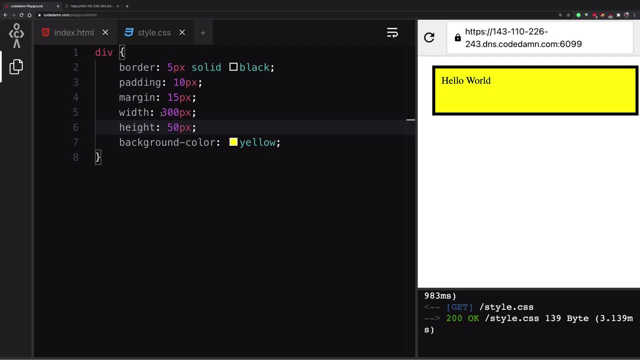 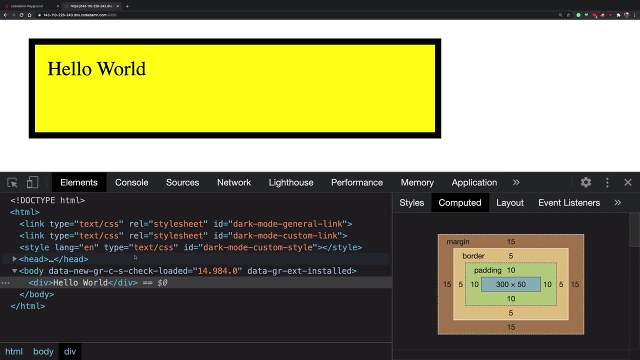 even though I specified the width and the height. the width and the height as 350, the original width and the original height is actually 330 by 80.. If you can zoom in a little right on the thing when I hover over this, 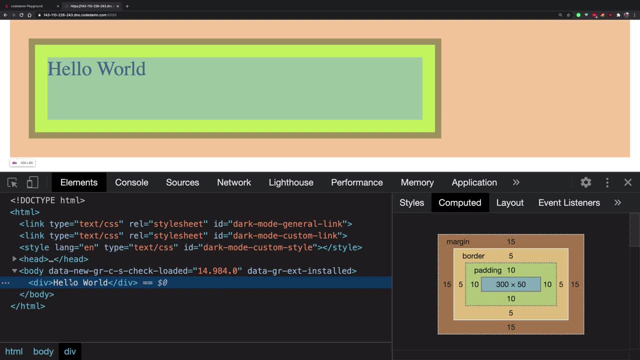 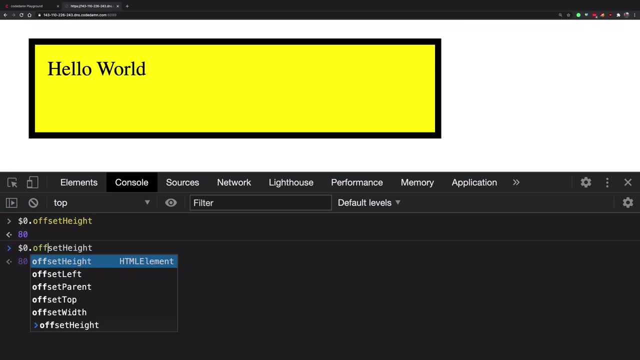 So if I hover over this you can see the original width and height of this element. Let me just go ahead and see if I can say: let's say offset width and offset height, width, right, So you can see the width and the height of this element is 330 by 80.. 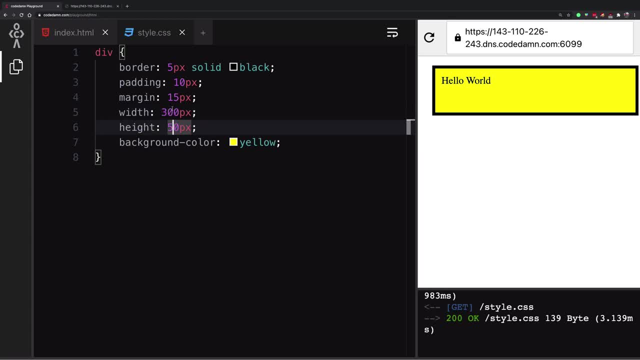 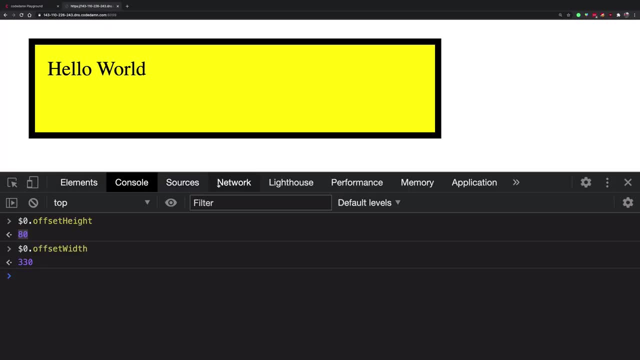 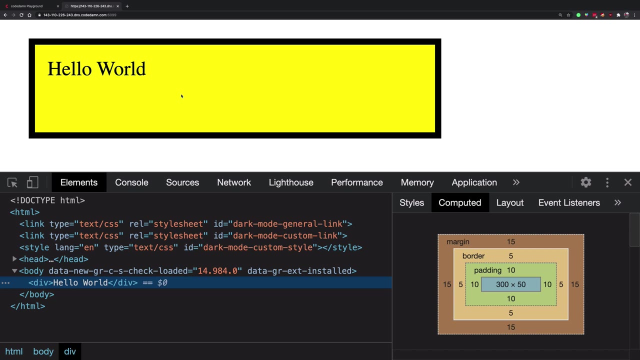 But I specified 300 by 500,, 300 by 50, right. So why did it not be that same? And the reason for this is that, by default, the CSS model which is applied in the browsers is not. you know what you would expect otherwise. 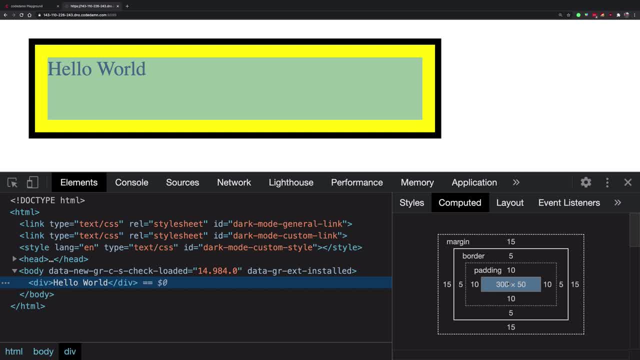 The model first of all has the content and the padding and the border as separate from the original width. So your original width is only applicable for the same width. The padding is the central content. However, if you want to change this behavior, you can do that. 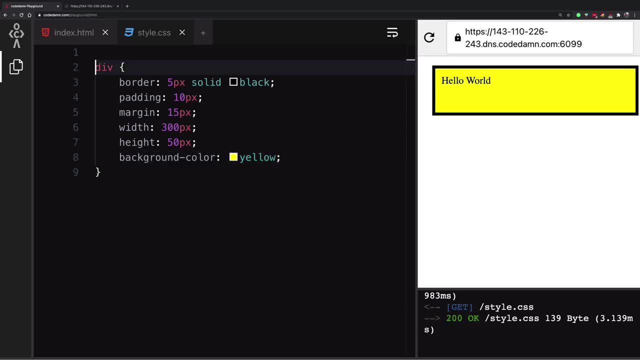 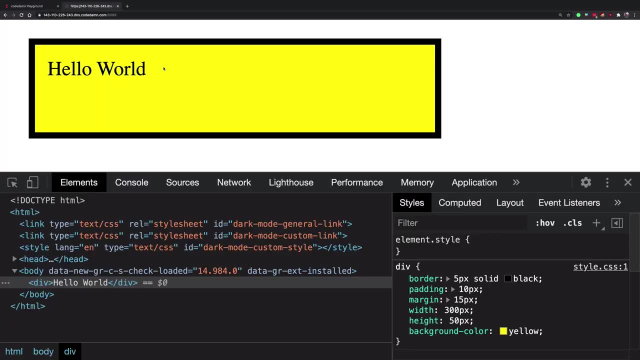 And the way you do that is you give every single element a box sizing of border box right Now. what this means is that once you have applied this and if you refresh, you can see the box sort of reduced in width and height. 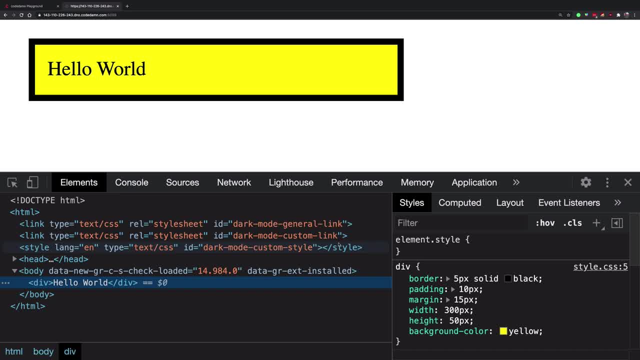 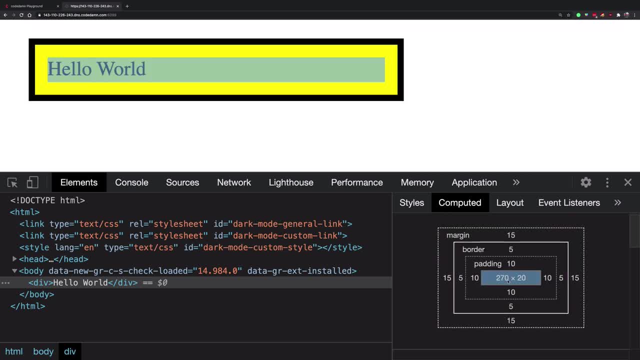 And the reason for this is because your width and height now include the padding as well. So what do I mean by that? If you go to compute it now, you can see your content automatically shrinks according to what it would make it suitable for the whole element to be 300 cross 50.. 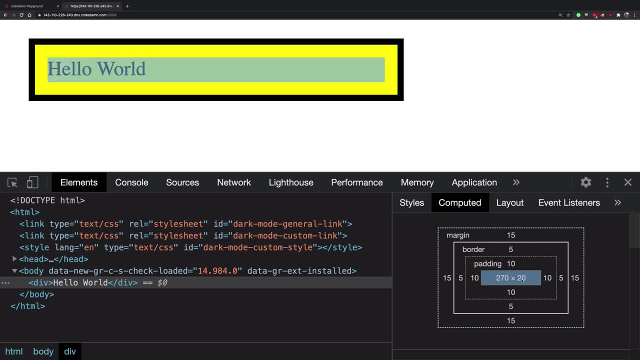 And in this way, CSS determines that, hey, its height, the content's height, should be 20, because we have a 10-10 padding, which makes it 40. And we have a 5-5 border, which will make it 50, right? 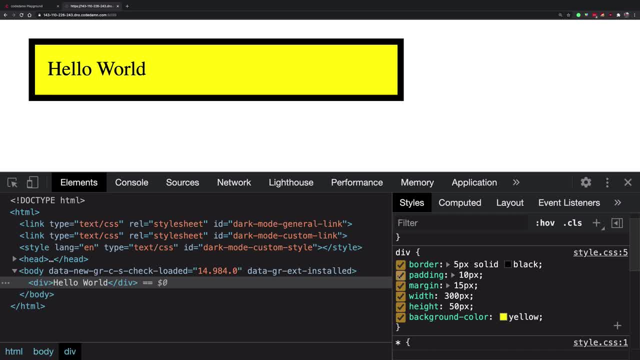 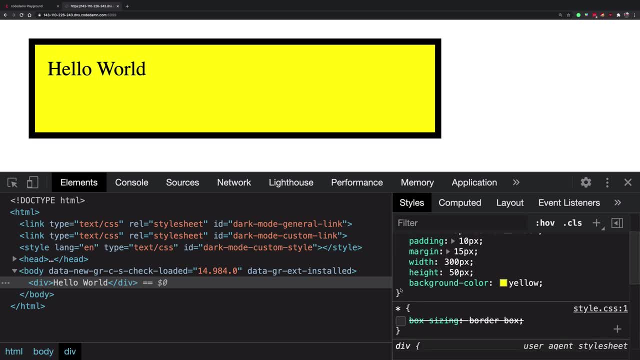 So if I go ahead and try to drop padding here, you're going to see there is no difference in the total width of the box. But if I remove the box sizing, border box, and now if I go ahead and drop padding, you're going to see there's a difference in the width and the height. 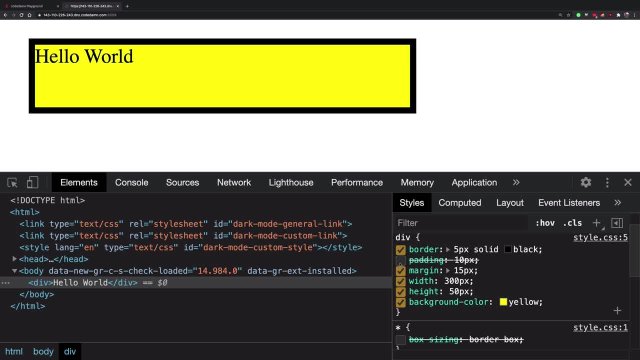 because in the last case the width and the height was independent from the padding. It was fixed, it was constant. But if you do not have box sizing, border box, then the width and the height depends on the padding and the border. If I enable this again, you can see this does not make a difference. 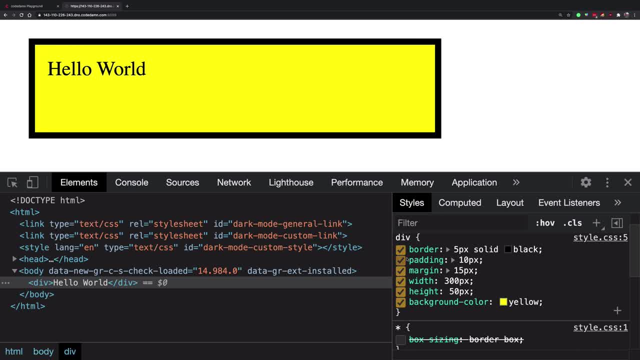 If I disable this, that is the content box. this makes a difference. So this is. these are like two models. By default, the content box is applied right, which you can see right here, But you can switch it to border box as well, and this would work fine. 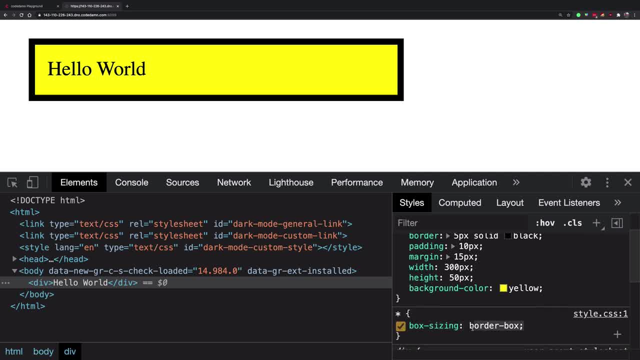 Personally, I really really like border box because it kind of like solves a lot of pain points which you might get because you now have more control over the width and the height of the element itself. But yeah, it's a personal choice, to be honest. 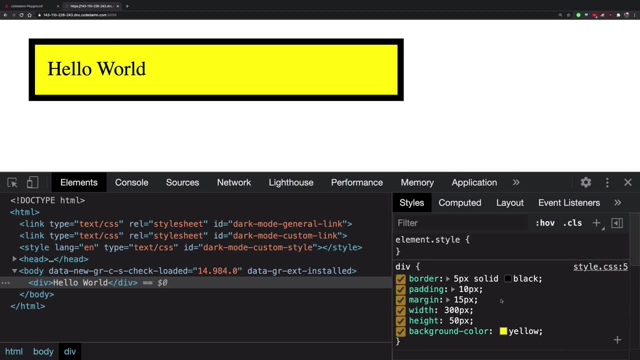 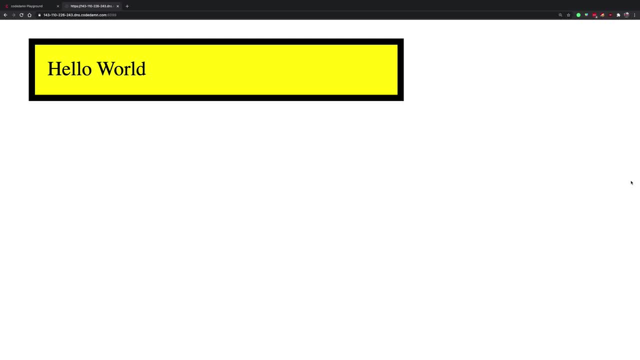 So yeah, that's pretty much it on the border box And content box and the box model of CSS. That's how things really work in CSS And if you know this- you probably are- you probably would be able to, you know- visualize margins and paddings in a much better way now. 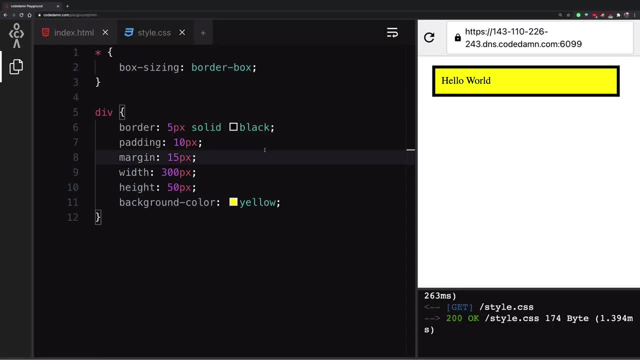 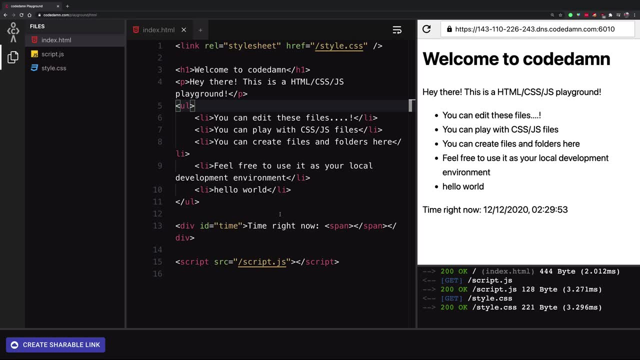 So, yeah, that's pretty much it for this video. I'm going to see you in the next one really soon. Hey, everyone. welcome back to another video in which I want to discuss about CSS variables, which is again something which is new in CSS. 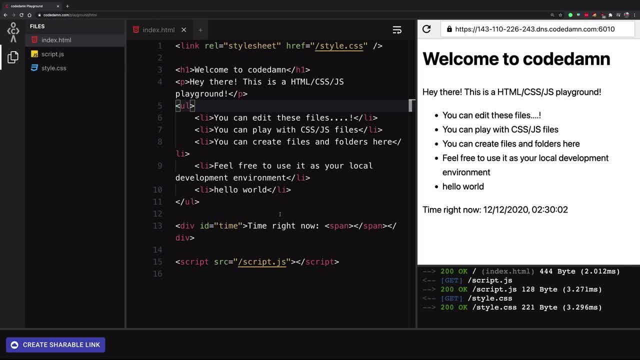 Now what this means is that you can to some degree, use variable like thing in CSS. That is, you can assign a value, you can change it using JavaScript- More on that later on, when we are learning JavaScript- But you can mess around with variables in CSS. 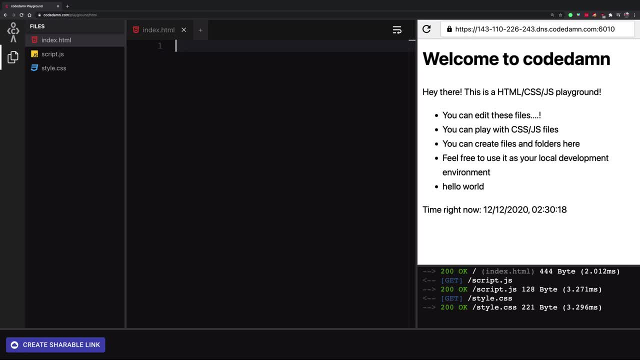 So what does this mean? Let's just go ahead and just create a very simple HTML document here, really quick HTML: head opening, head closed, body opening, Body closed. And I just have a, let's say, h1 tag saying hello world. 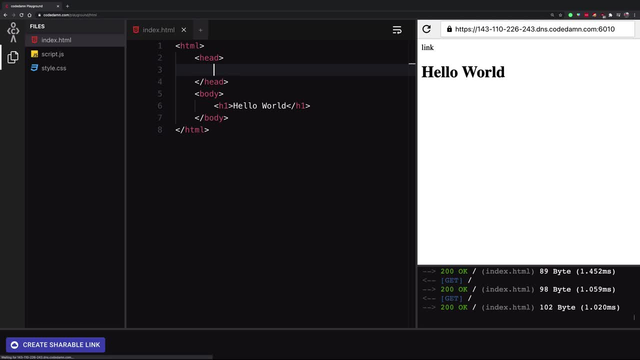 Right, We can also bring in a stylesheet which would be link rel. stylesheet, href, stylecss right, Which is at this file right here. So let's just open this And already in the stylesheet file we can see we have some content. 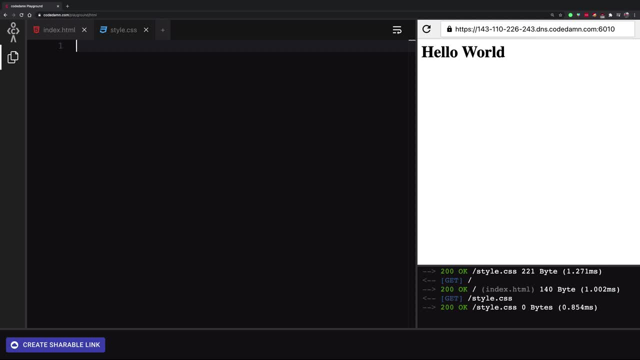 Let's just get rid of this. So what we can do next in order to create a variable, first of all, let's just go ahead and give a background, a body color of, let's say, yellow. Now what you can do in CSS is you can create variables, just like I said. 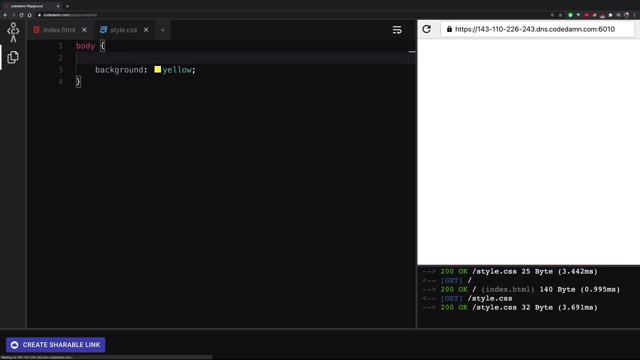 And the way you create variables is the way you write property names. However, there's a very important difference, and that is these variables name will start from two dashes. So whenever you write two dashes, whenever CSSC is two dashes, this means the name of the property now is not actually a. 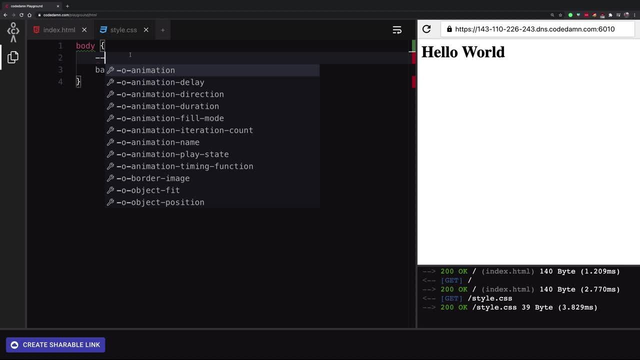 name of the property itself. but it is a variable. So let's say, I want to say BG color and I just want to give this as green, right? Let's see Now, this variable is defined. right, It is there. 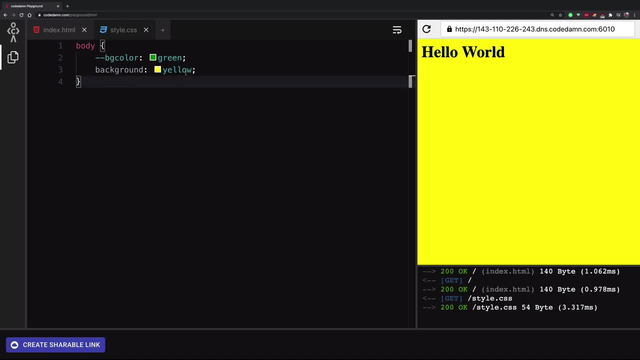 It contains the value green. It's all fine and good. However, in order to use this, what do you have to do? is you have to use the keyword var? Now, this is a sort of a function in CSS, which will expect the name of the variable. 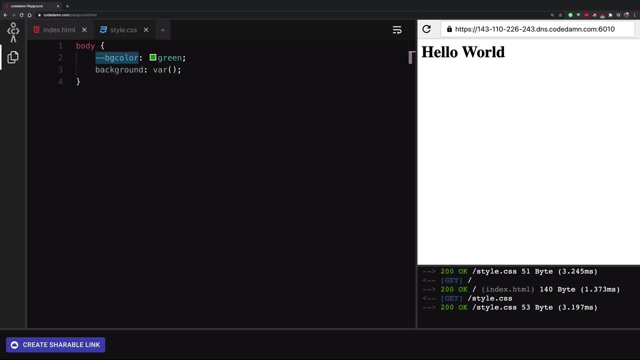 and it is like the full name. It's not, like you know, without dashes. you have to specify the full name. So you see, right now I created dash dash BG color as the green value property name and then I access that using var right. 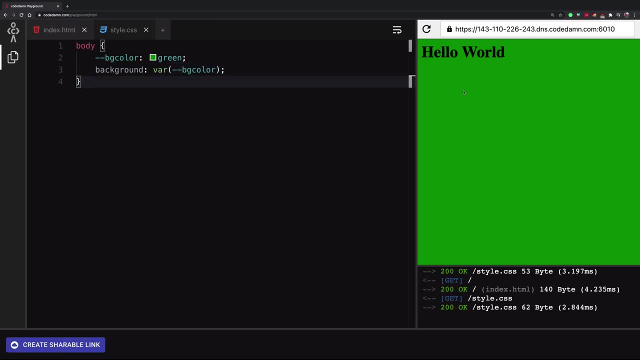 And you can see on the right, we actually see that the background turns green, So this is pretty cool. Now, one thing you have to be careful about when you're using CSS variables is that it follows a scoping mechanism. That means your variable is only applicable to the particular element on which you are. 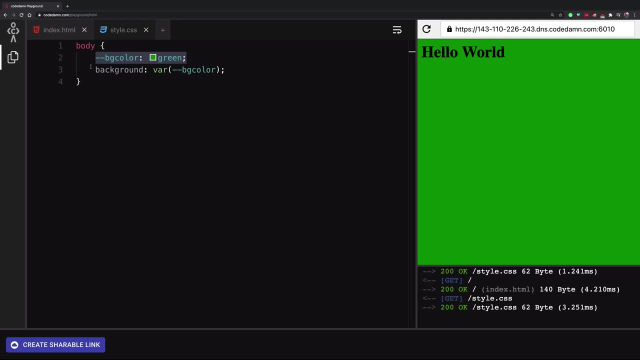 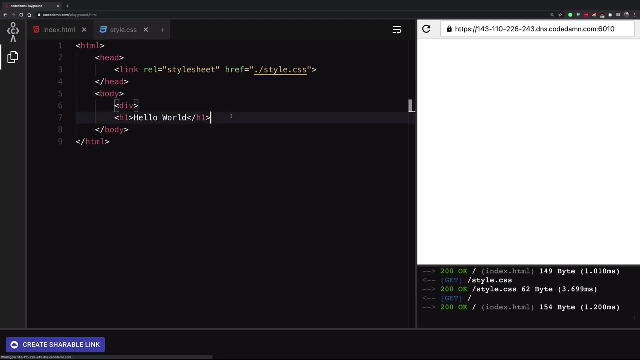 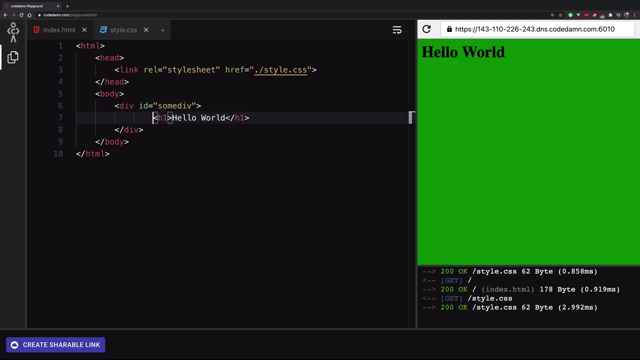 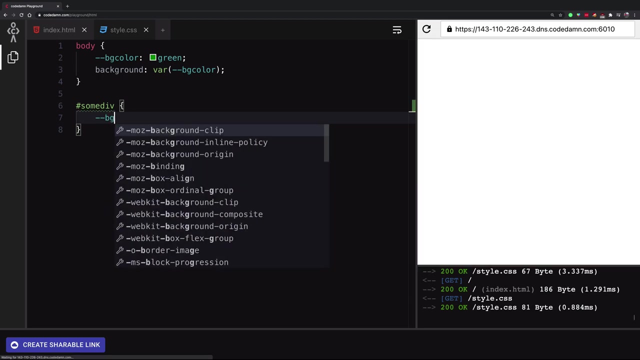 applied on which you have written the variable declaration on and the children. So that means you, let's say, if we have a div right here with a div ID of some div right, So if we have this div right here and if I go ahead and add a sum div and BG div to 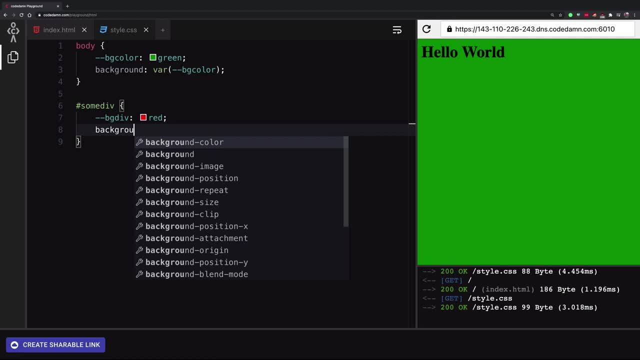 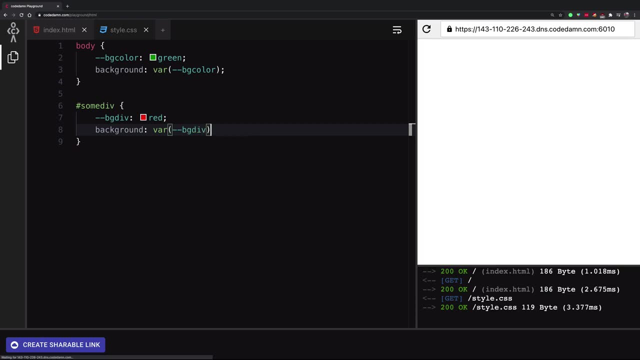 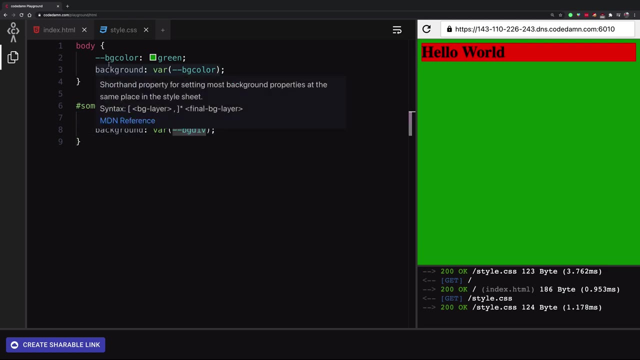 be, let's say, red. and now I give it a background of, let's say, var dash dash BG div. So this thing, right here, you can see it turns red. But this BG div variable is not accessible in body right. 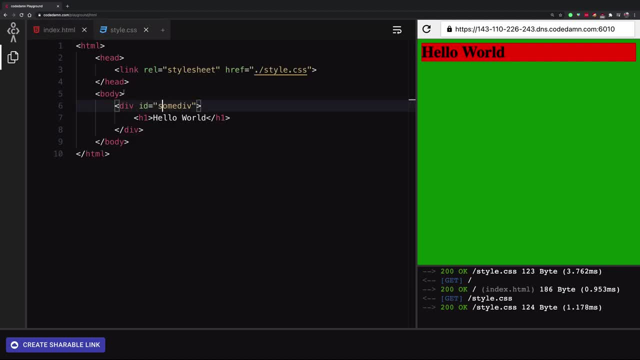 Why? Because some div is the child of body, or in other words, body is the parent of the sum div right. So parents cannot access the variables of children, but children can access variables of parent right. So you can use BG color right here. 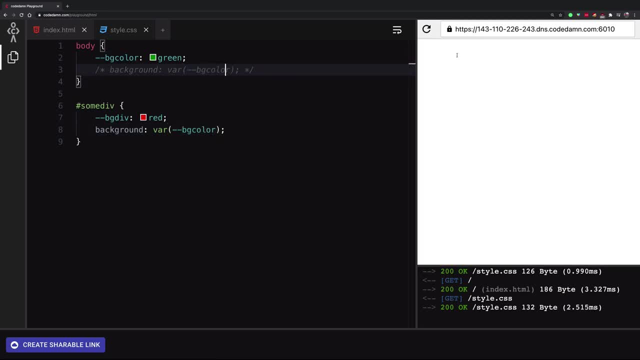 And if we just remove this, you're going to see that this in fact turns the div into green. So you can see this happens just fine. However, if you go ahead and try to use BG color, If you go ahead and try to use, let's say, BG div inside this one, 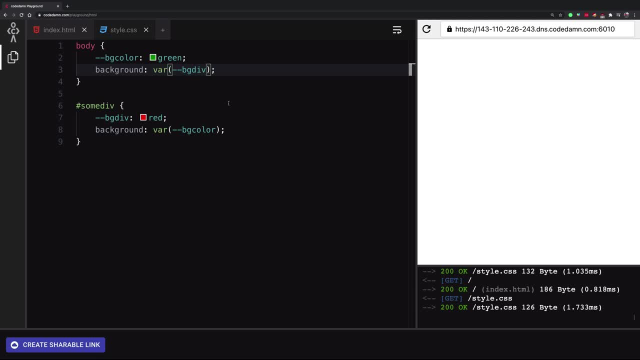 Nope, Nope, Like this. If you try to do something like this, this will not work. You know, you see, that the background did not apply because we cannot see any red. So you see that you cannot really transcend the variable sort of hierarchy in CSS. 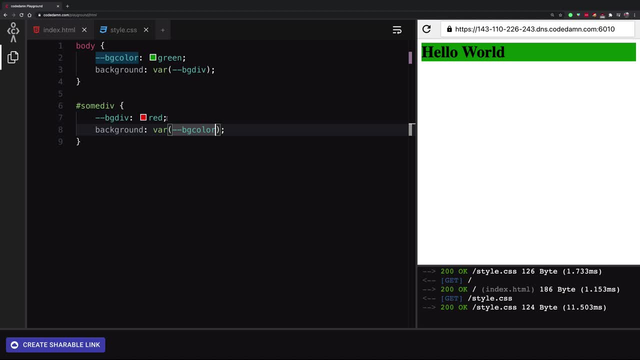 So most of the people who want to have a global sort of variable- what they can do is- you can be. by the time you would probably know that you know if you're applying any variable to body, it will be accessible to every everything. 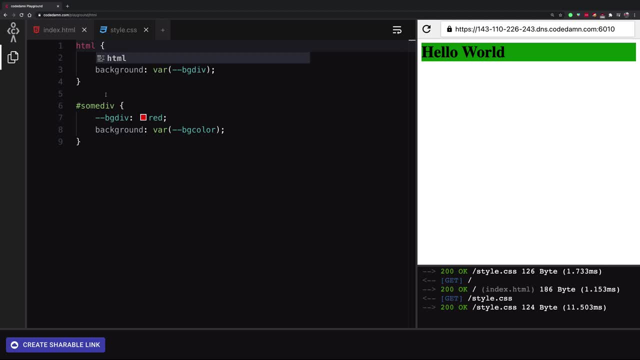 But sort of the convention is to apply it on HTML right Or to apply it on root, And root is just a pseudo selector. We'll discuss more on pseudo selectors when we in the next video- actually not really in JavaScript- series, So this is basically equivalent to HTML. 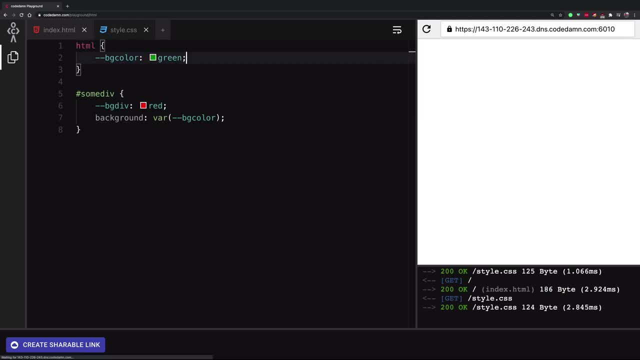 You can think of that. So once you apply all the variables- like on the HTML, HTML collector, HTML selector- Now you are free to go ahead and make use of them in different tags, right? So you can go ahead and say body and then background, BG, color, right? 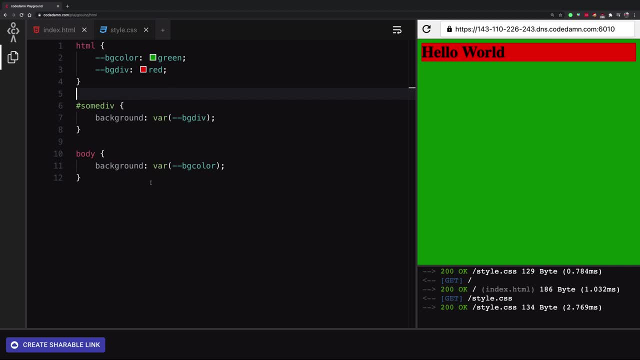 So that way it will just work fine. So this is how, in a nutshell, CSS variables work. There's one more thing with CSS variable, and that is you can specify a default value. By that what you mean is, let's say, if BG div was not set. 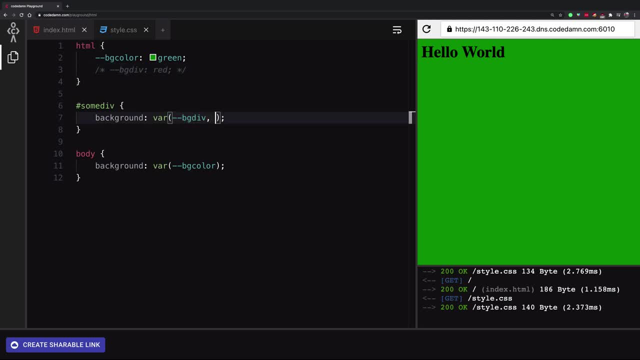 Right. So in that case, if BG div is not set, what I want to do is I want to say that the color should be yellow, Right? So this value, right here, you can see, it is basically the default fallback for the variable. 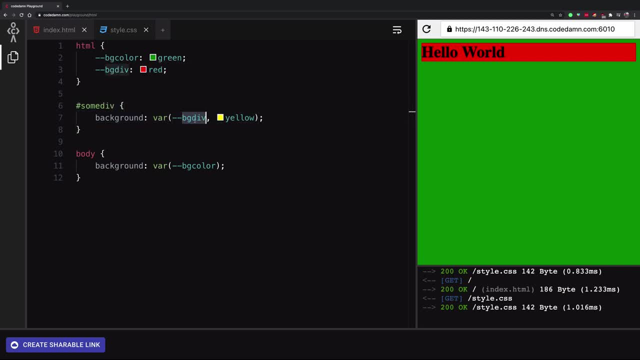 Right Now. one thing to remember again is that if the variable value itself is invalid, then the fallback does not get triggered, Right. So you could see that if the value instead of red is, let's say, one pixel, which is a, 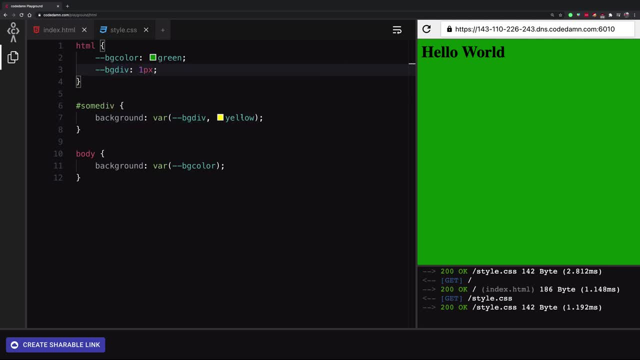 wrong sort of value for a background, then you can see we do not get yellow Right. It just does not work. So it does not work. Like you know, if the value is not working, then we just just fall back to default. 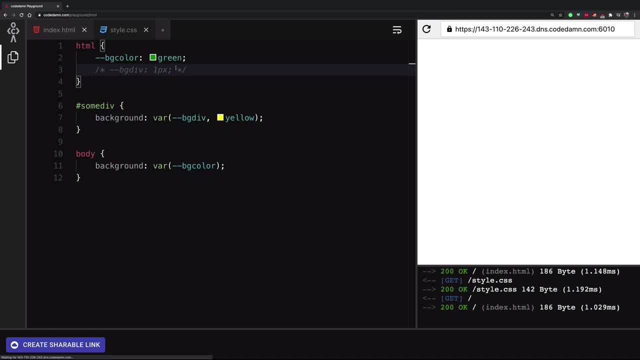 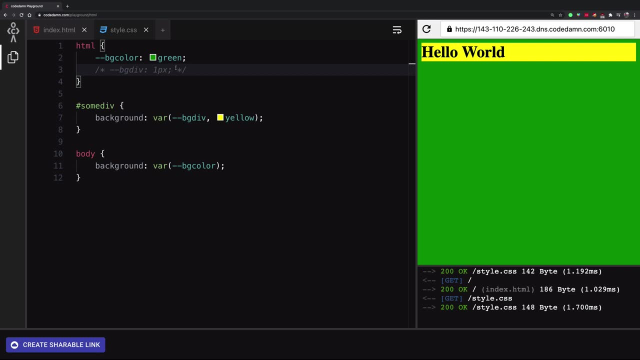 That is not happening here. It just happens if the variable is not set at all. That is the case. So yeah, that's pretty much it for this video. Just the takeaways are that if you want to create variables, you most likely want to. 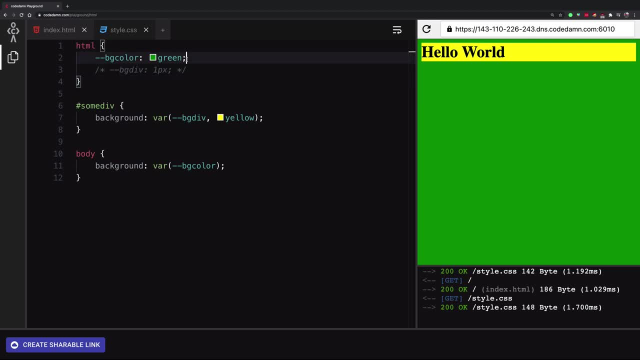 do them on the HTML, because in CSS you probably would keep the variable scope Global in most of the cases. If not, you can also have component level access of the variables. But that is sort of like an advanced use case, I would say. 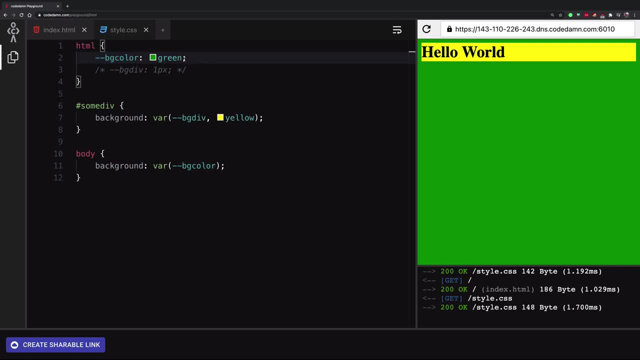 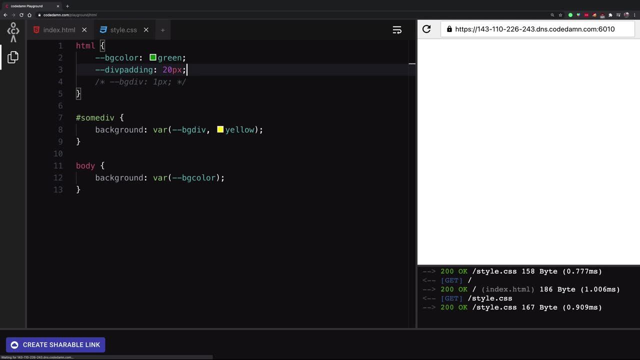 But you know you get the idea. So you can create as many variables as you want, assign them any value, Like, for example, you can say div padding and give it a value of 20 pixel, And now you can just apply this div padding to basically like padding. 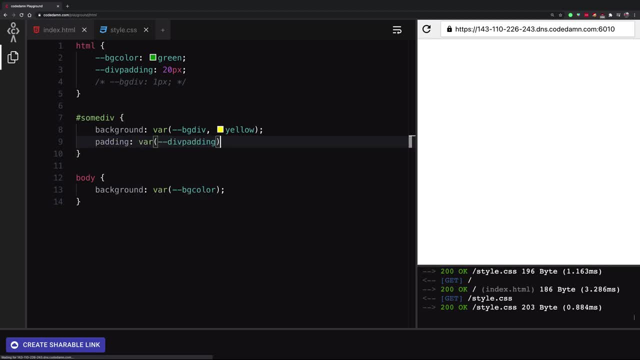 And then you can say what Div padding. And yeah, if you ever decide to like change your layouts or anything, you just have to change the value of a single variable. So that is pretty cool, if you ask me Right. So yeah, that's pretty much how it works. 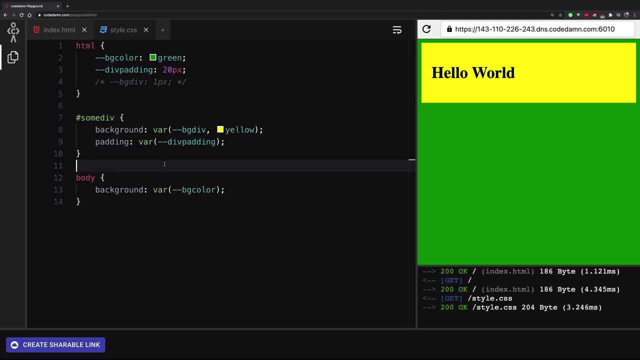 And that's all for this video. I'm going to see you in the next one really soon. So what is going on? everybody, Welcome back. And in this video I want to explain calc in CSS, and calc is another function in CSS. 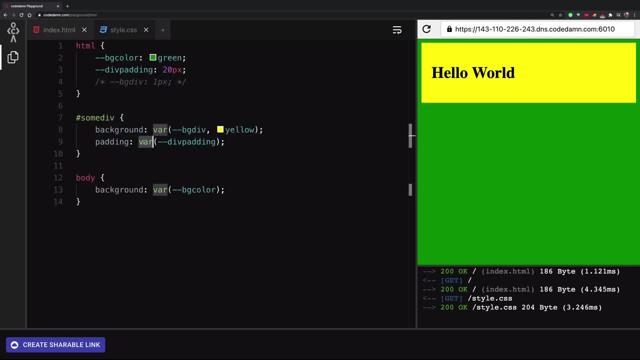 just like var was Right. So this function allows us to access the values of variables. Similarly, calc- if you can think about it from the name- allows you to have computations in CSS on the runtime, And that is again pretty cool feature because you can do pretty funky stuff with that. 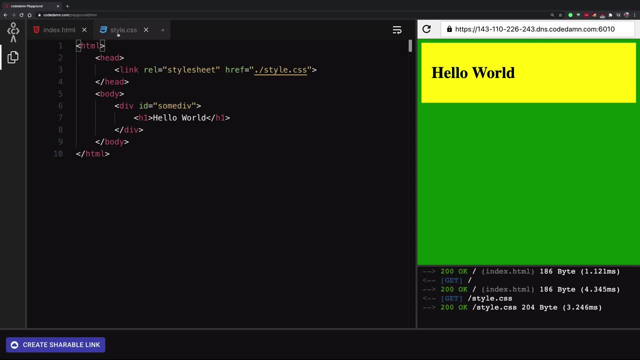 So let's just go ahead and take a look at how we can make this happen. We have an H1 on the page, So I'm going to give it an H1 right here And I'm going to say that the font size. 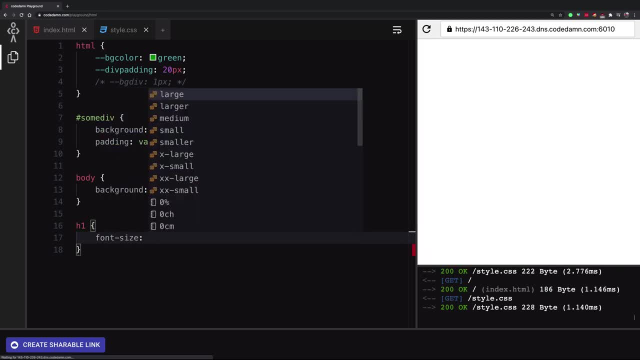 That the font size of this H1 is, let's say, 35 pixels, which is sort of not so, you know, exciting. Let's give it a 48, so that we can at least see that it's increasing, All right. 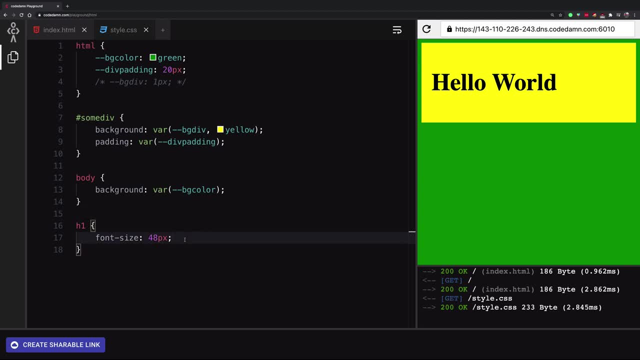 So this is that. But what you can do with calc is that? how about we try to set this as a dynamic value? Now, with calc, if I go ahead and do something like, hey, calculate this, Set this to, let's say, 32 pixels, but also add, I don't know like two view width to 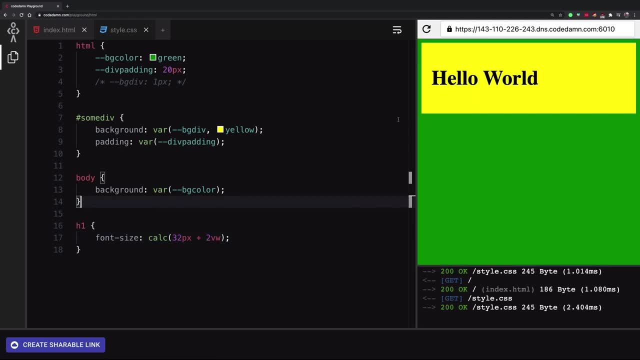 it. So now what's really happening is that if you scale up the screen, if you could observe, the font size is actually increasing. Let me just go ahead and push this factor to 10,, for example. Then it might be more observable. 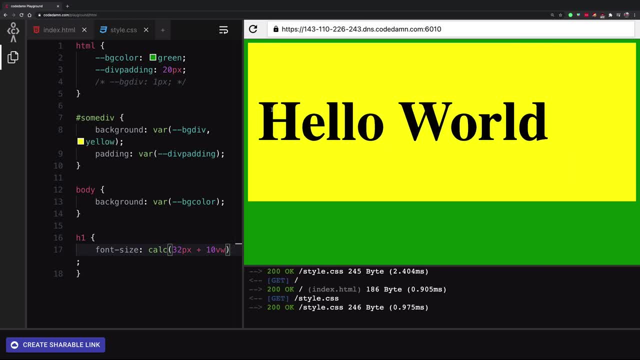 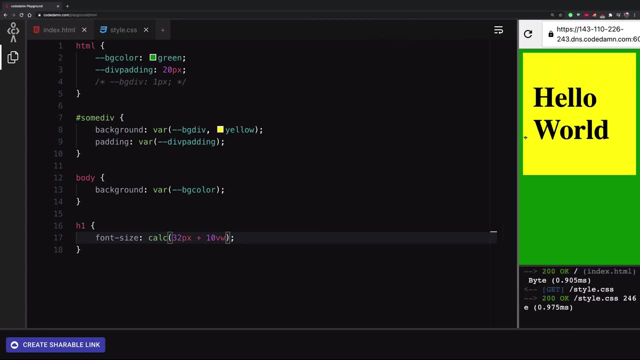 So if I increase the size of the screen, you could see that the text size increases, Right. And if I decrease the size of the screen, you can see the text size actually decreases. Now it does not really follow the sort of ratio of the screen width with the actual. 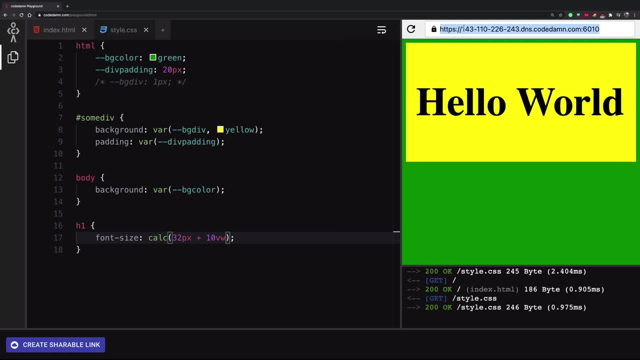 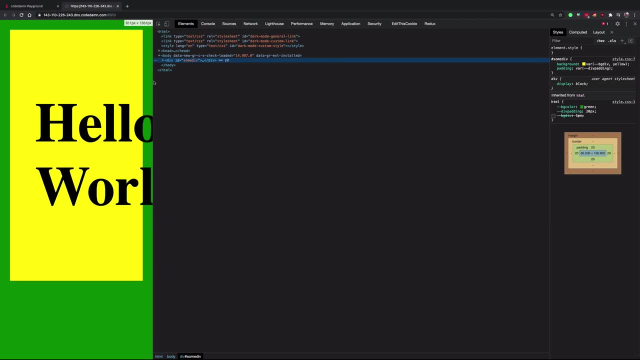 text. It should be, But you know, you get the idea. And now, if I go ahead and open this, actually in a new tab, what we're going to see is that I could pretty much do the similar thing here, Right? 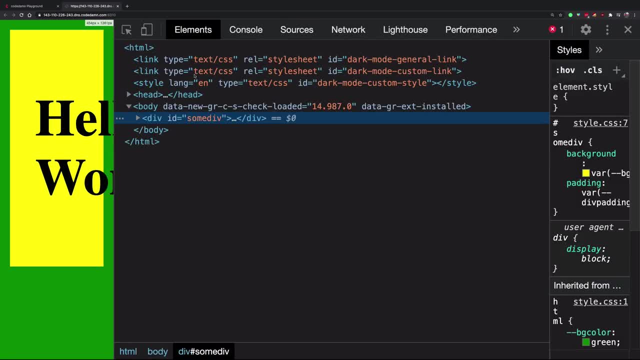 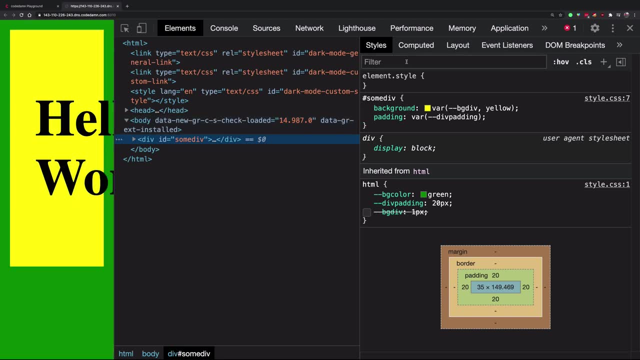 So it decreases, it increases And if you go ahead- and this is just a neat little trick, we'll discuss this more in the Chrome DevTools course, Which is again on the website itself, But if you go to the computed section, you're going to see not really computed. 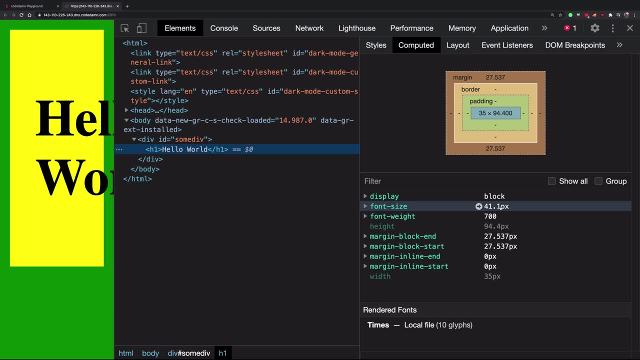 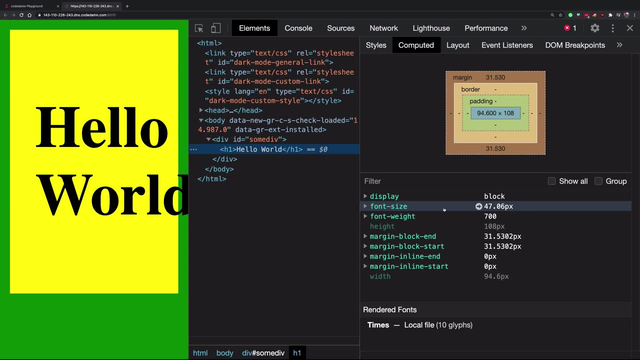 Yeah, So you're going to see the font size right here is 41.1 at the moment. Now, if I go ahead and increase this, you can see the font size changes dynamically. So you are actually computing it with the help of you know, two different units, which. 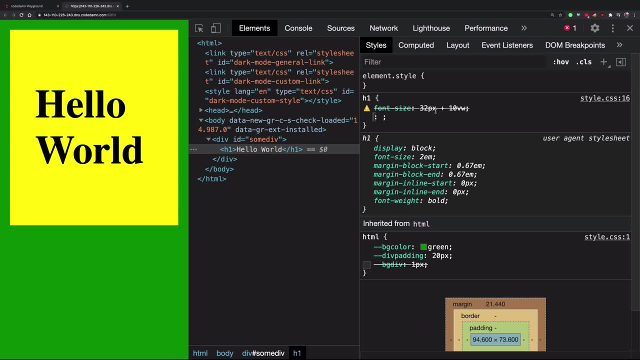 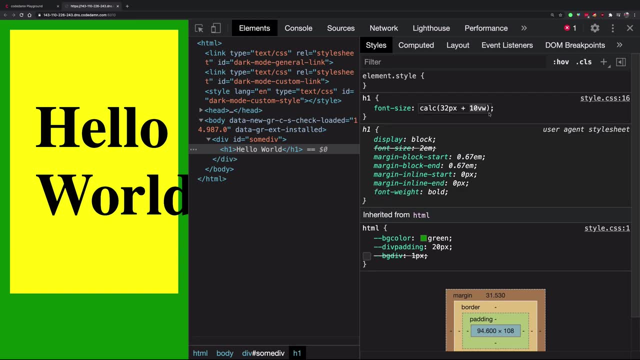 is not really possible if you are using something like this. It's just an invalid value. So calc allows you not only to do computations in the same unit. I mean you could technically do like 32 pixel plus 10 pixel, but it's not of any use if they 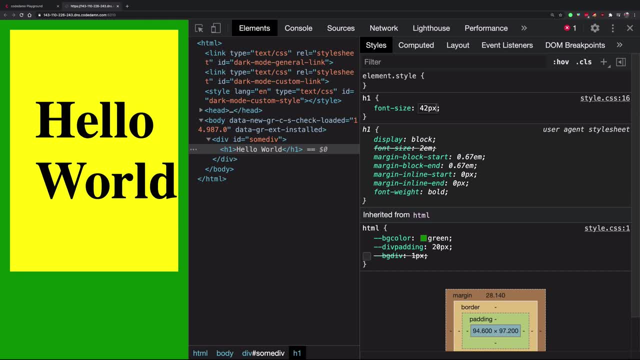 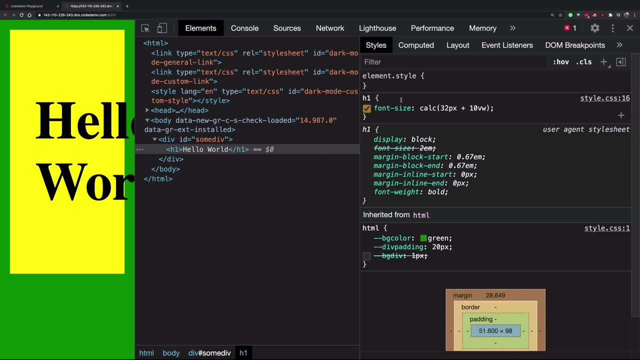 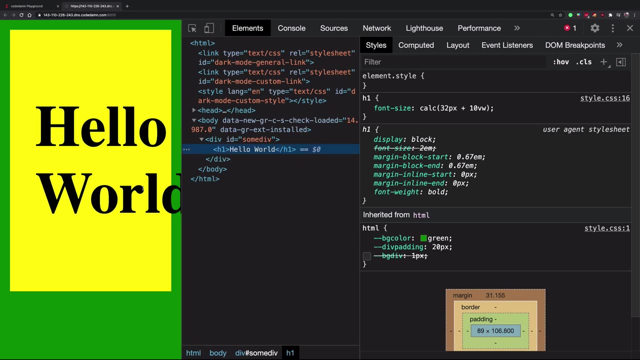 are in the same units, Right, Because then you could just probably write 42 pixels itself. You want to do calculations when there are different units involved. So anyway, you get the idea that you can use calc like this. Another thing which you can do with calc is that you can use them with variables. 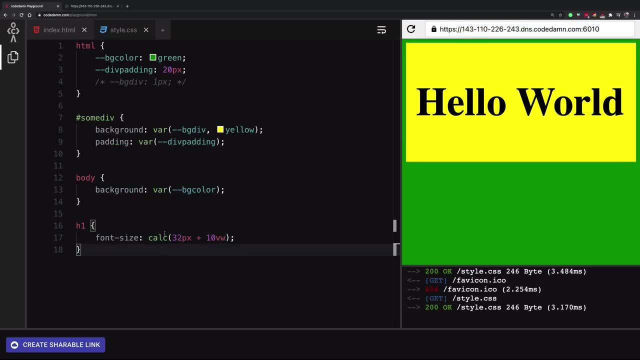 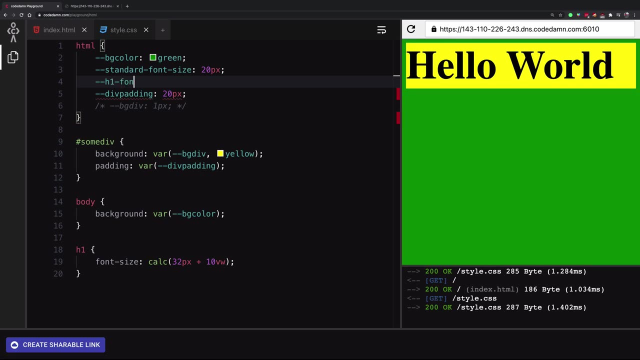 So what you can do is you can calculate. So what you can do is you can go ahead and say something like standard font size and give it like 20 pixel or something, And then you can put like h1 to be I don't know font size, to be like calc, then variable. 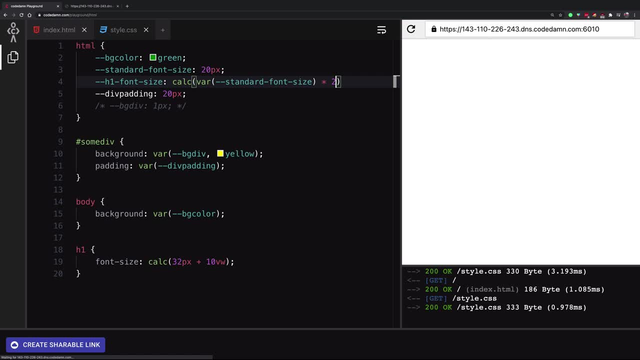 value of standard font size times two, Right? Or you know whatever you want. So now, if I go ahead and try to use this variable right here, what are you going to see is that this is actually 40 pixels, Right. 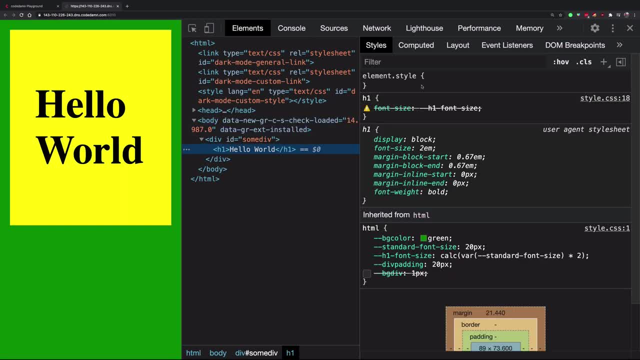 So if I go ahead and refresh this page, we're going to see that the h1 right here and actually you need to have one here, obviously, And there we go. So now, if I go ahead and take a look at computed, you're going to see the font size is 40 pixels. 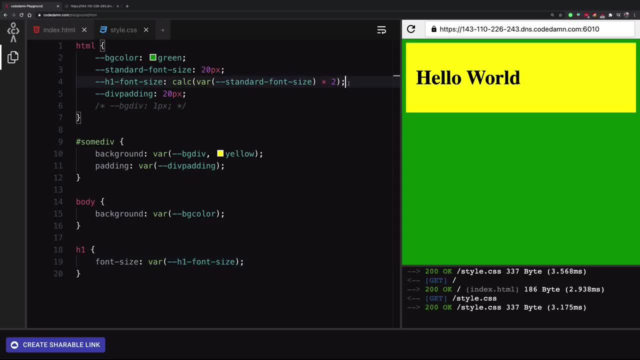 which is exactly what we observed, Right? So if you wanted to have like a P font size right here and give it like a 1.5 multiplication, then you can go ahead and give this to a body, Right? So, again, pretty pretty cool thing. 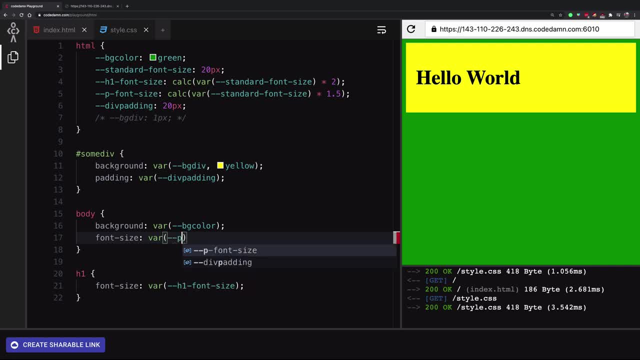 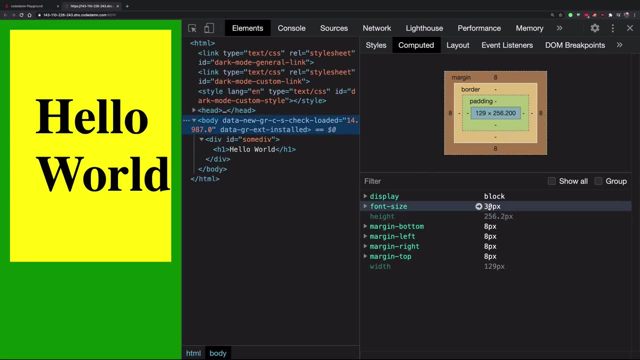 If you want to, like you know, control everything at a single place and, at the same time, just make your life much more easy. So now you can see that the body right here has a font size of 30 pixels, because you can see, 20 times 1.5 is obviously 30.. 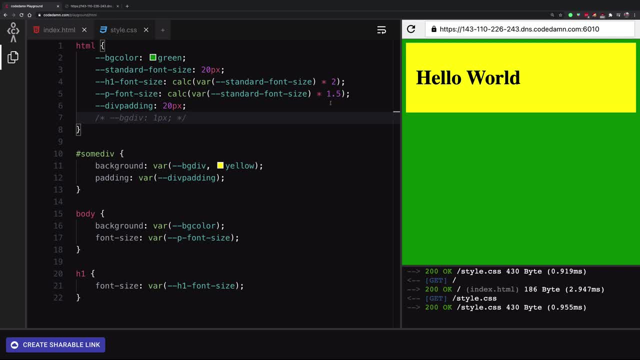 So that is that. So, yeah, I mean, it makes your life much more easy. You can also divide if you want, and division would also work fine. This just dropped it to 10 pixels, So you can go ahead and see now that if you see your h1 right here, it's actually 10 pixels. 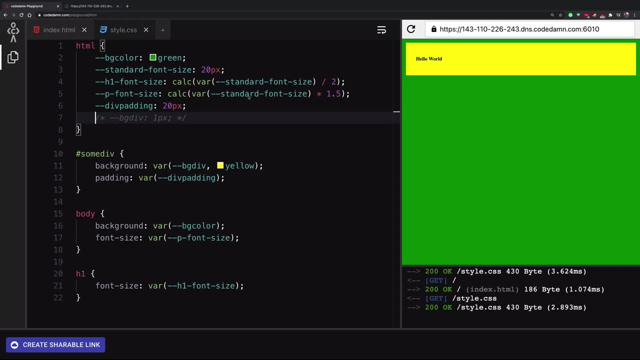 So there's that. One thing you have to pay close attention to is that when you are using addition and subtraction with calc, make sure you put a space in between. Let me just show you what I mean by that. So let's say I am having a calc of, let's say, 20 pixels. 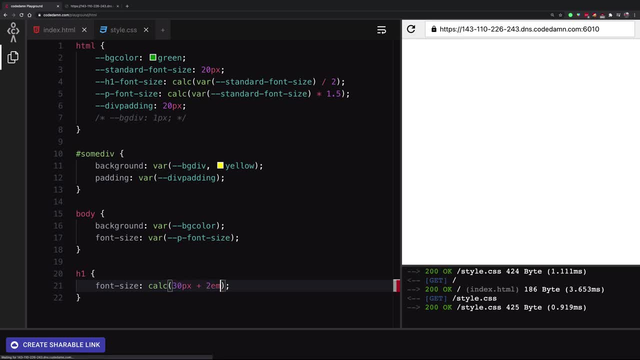 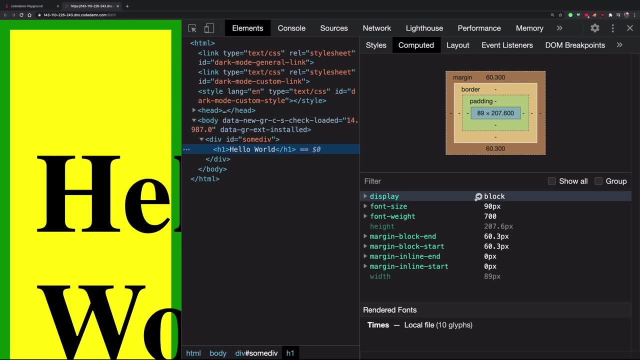 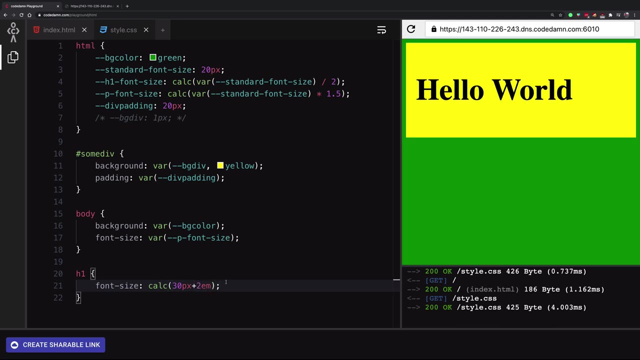 30 pixels plus 2em right as the units. So let me just go ahead and refresh this right here And you can see right here It works just fine. We get a 90 pixel output. Now, if I go ahead and just remove the space, sort of what's going to happen is that if 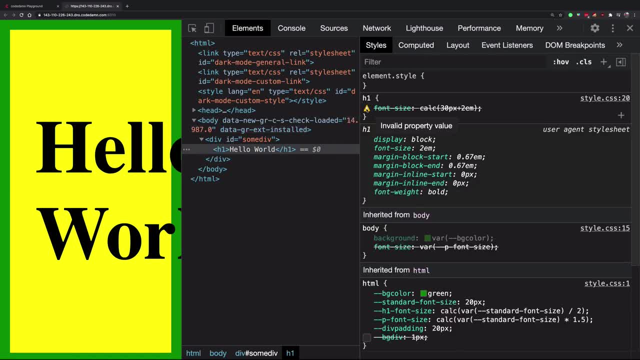 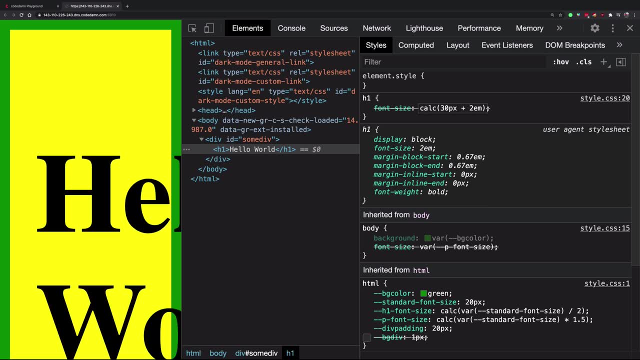 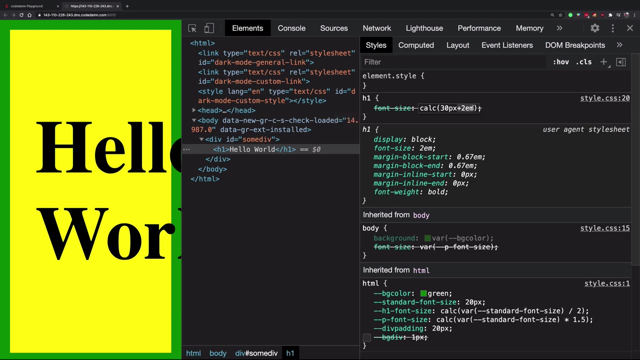 you go to the style, you're going to see that this is an invalid property value, And the reason for that is that addition and subtraction expects to be Separated by white space. Why? Because this gets translated as plus 2em. 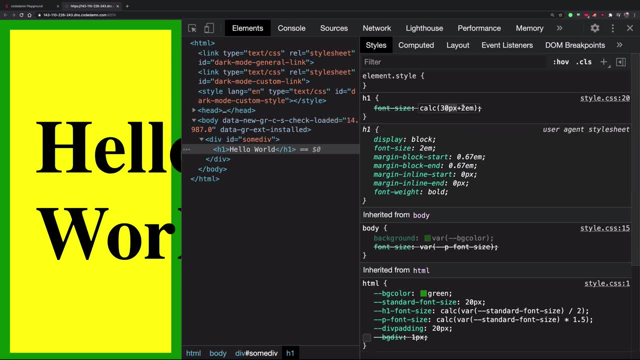 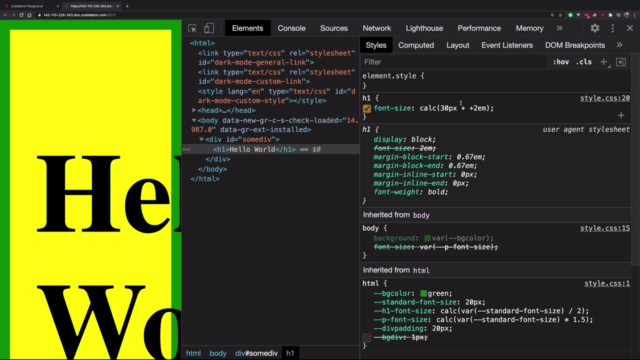 And that means there is no operator between 30 pixel and plus 2em, right, Oops. So if you go ahead and give it an another plus right here, then also it will work. Why? Because the earlier was sort of like equivalent to this right. 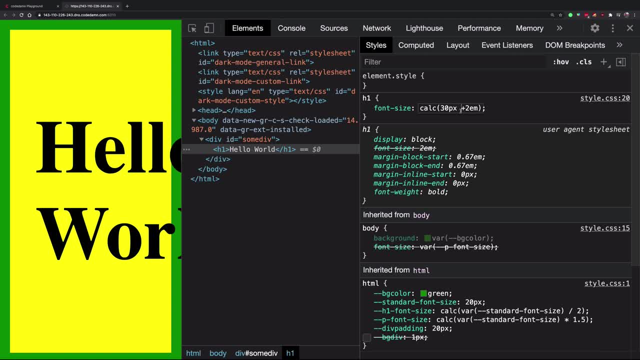 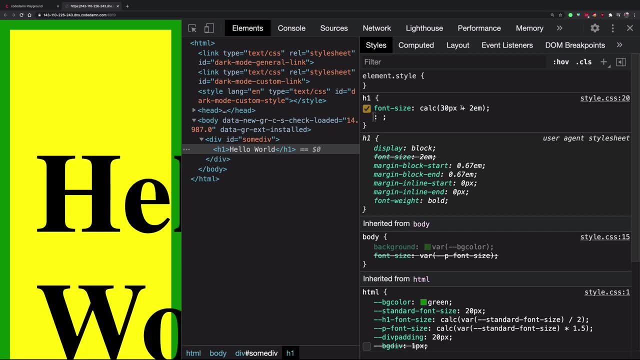 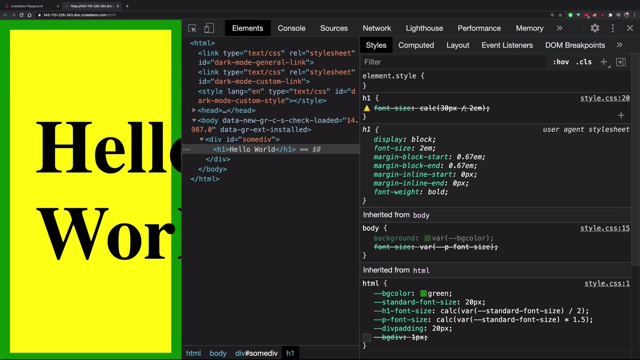 That means there is no operator between them. So you always want to give a space in front of and between Before, after the operator, And this is like, only valid and only required for plus and minus. It is not required for division, to be honest, 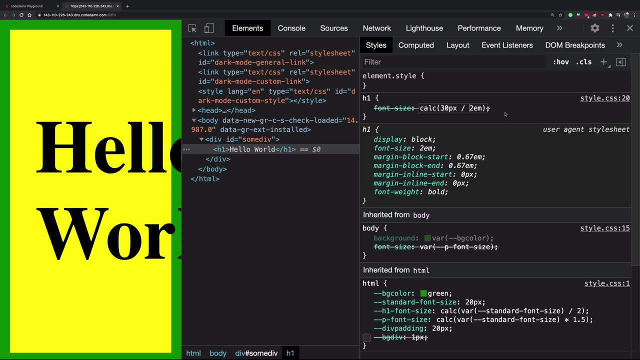 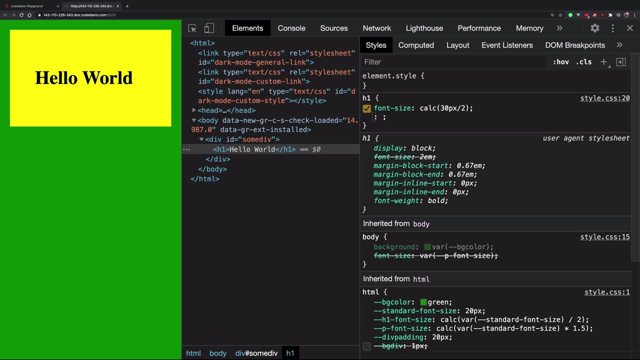 But it could sort of like be a good habit, right. So if you have like 30 pixel by 2 right here, if you just go ahead and you know, not give a space, it will still work. But it's just a good practice because you know it'll just make your CSS consistent. 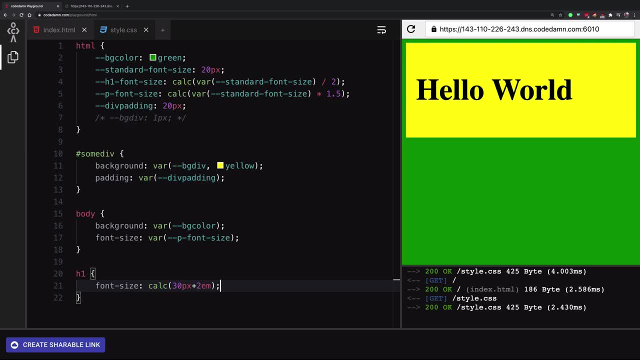 So there's that. So this is like one Another thing which I thought was important you guys should know. So yeah, that's pretty much it with calc. It's a super interesting property. You can hack your way around with widths and heights here and there. 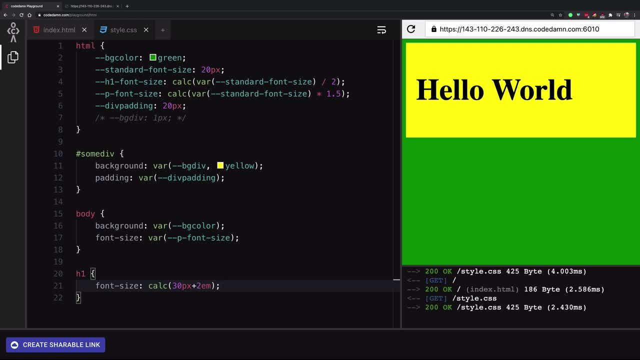 But yeah, if you're using it, I would say like, try to figure out the reason, because if it is a simple use case, like layouts or something, and if the layout is also, you know, very standard or typical, chances are you don't really need calc, right. 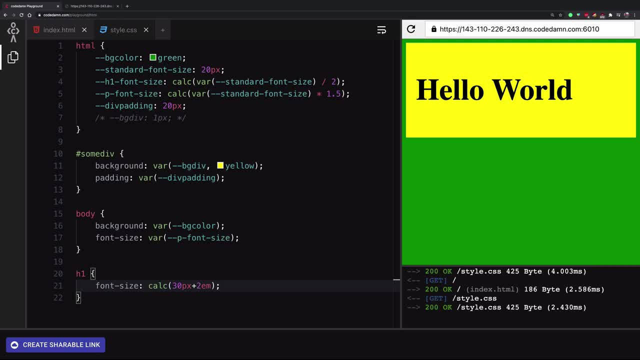 And if you are using it's fine. I mean, the support is quite good. The support is quite good right now, But yeah, it's still not 100% right. So, yeah, there's that, That's all. 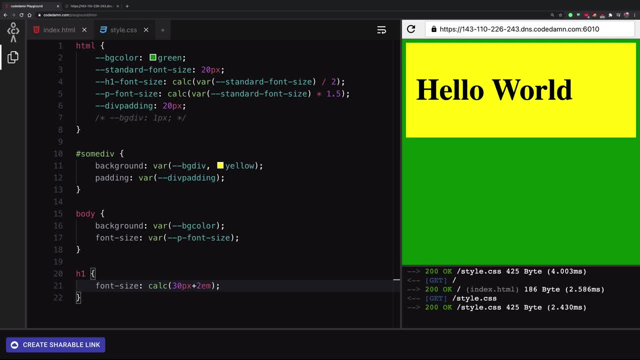 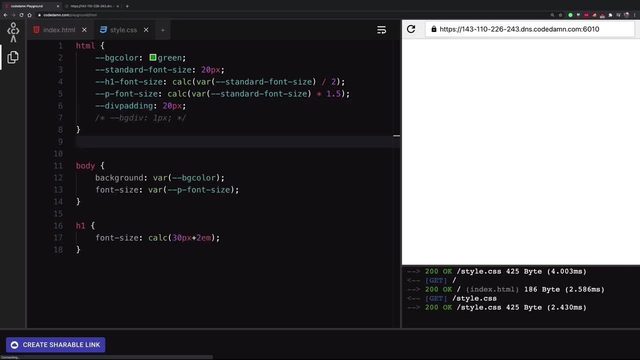 So that's all for this video. I'm going to see you in the next one really soon. Hey everyone, Welcome back, And in this video I'm going to go ahead and explain to you about CSS pseudo selectors. I think we touched a little bit on pseudo selectors in the basics course as well. 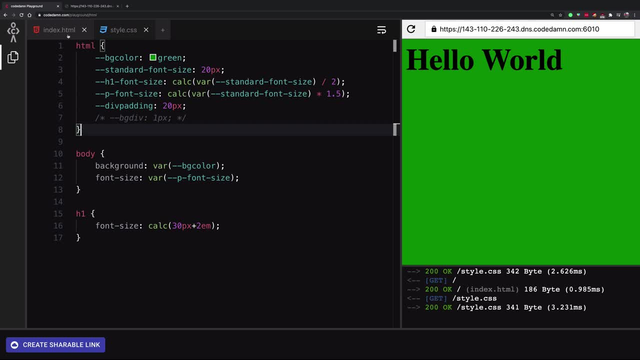 But let's just go ahead and formally look at that, because this is an important thing, right, And it is like one of the most used parts as well of CSS. So I'm going to go ahead and create a very simple page here. you know sort of like about: 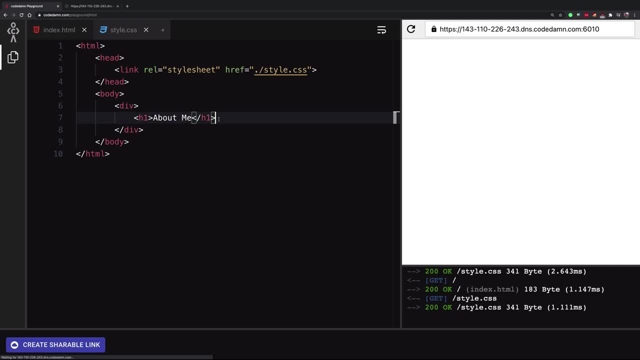 me And I'm not going to make use of any selectors right here, because pseudo selectors will cover that right. So I'm going to give it a paragraph. My name is Bold Mehul Mohan and I am the founder of CodeDamn right. 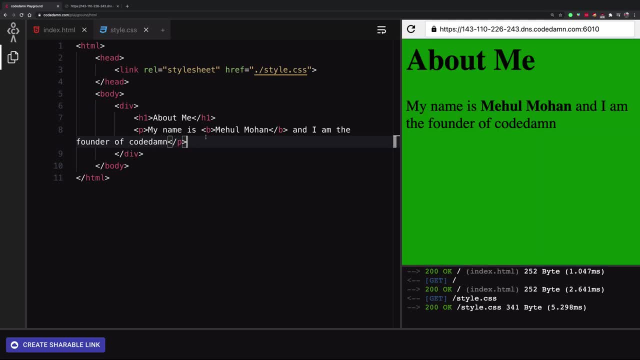 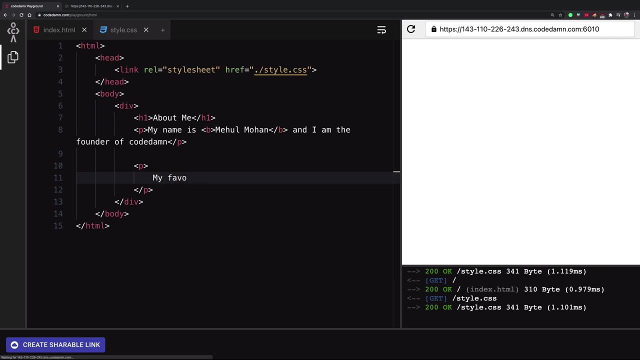 So this is a simple paragraph. Then I could probably go ahead and create a sort of- I don't know, let's say, another paragraph right here which contains my favorite F-O-U-R-I-T-E languages, And then I can create a UL right which consists of some LIs, HTML CSS. 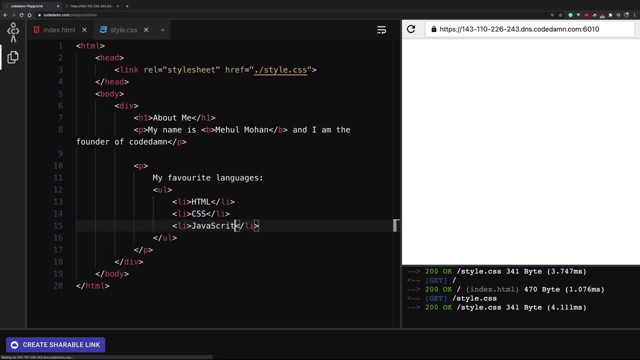 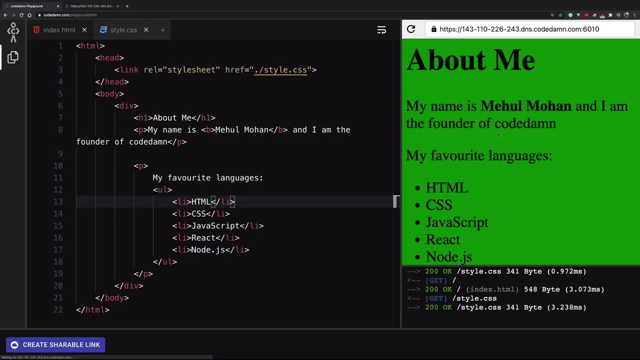 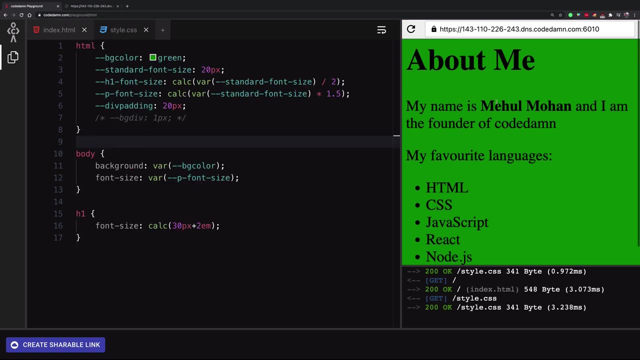 Then I could also have JavaScript here, Then I could also have React, Maybe like Nodejs, Something like this. So you know, you get the idea. So this is like a simple page for us. Now what I want to do is I want to add certain effects to this page, right? 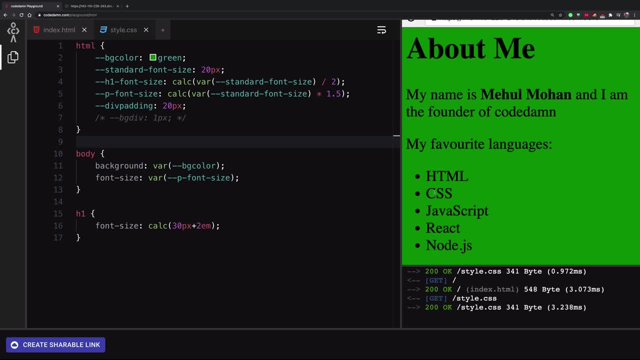 So if I'm- let's say, I'm- hovering over this, I want things to happen, And that is absolutely possible with CSS using something known as pseudo selectors. Now, pseudo selector means that that particular element would not really exist on the page. 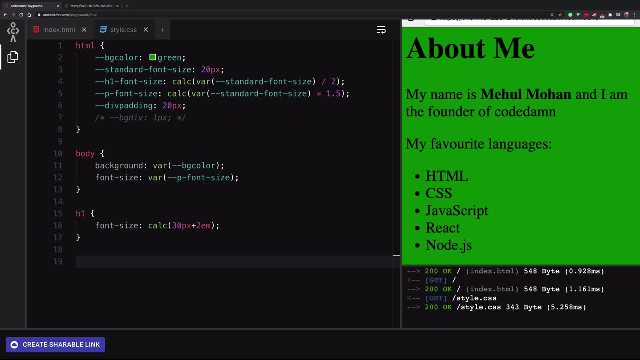 but either the state or, you know, with some user action or something happened which put that element into that particular state. right Now, let me just start with a very simple one, which you will be able to like visually see, and that is the hover selector. 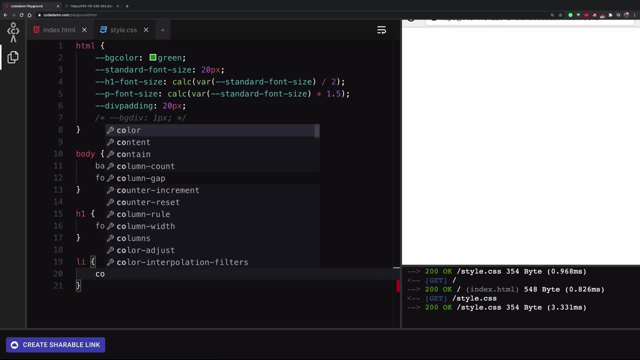 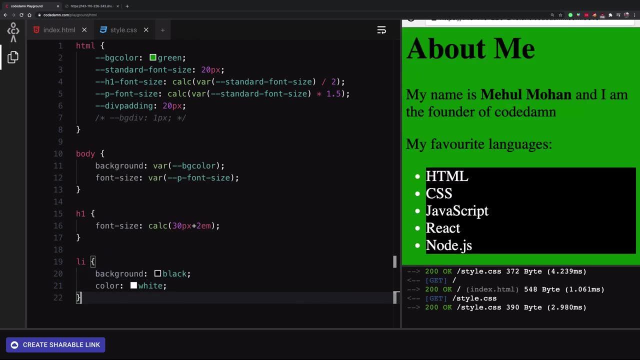 So what I'm going to do is I'm going to select Li and I'm going to say: hey, all of you have color background colors, So I'm black, white and color white. Simple enough. However, what I want to say that whenever I hover over these Li, I'm going to say Li. 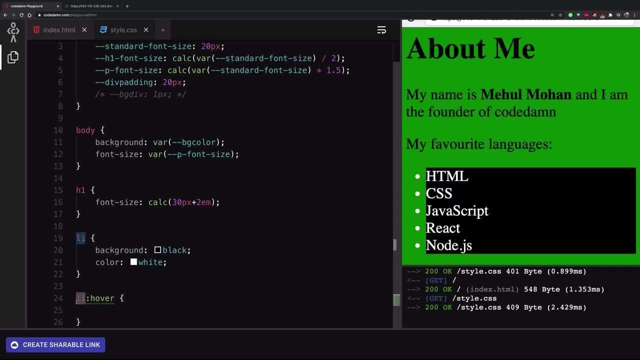 hover right. So what I did is I wrote the name of the selector and then I wrote: you know, colon, This colon right here is important- And then the name of the pseudo selector. In this case it's Li hover. 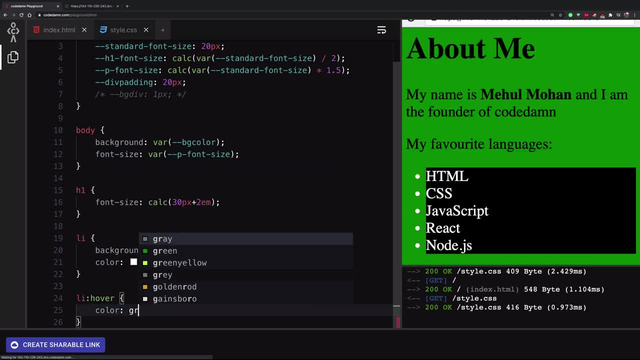 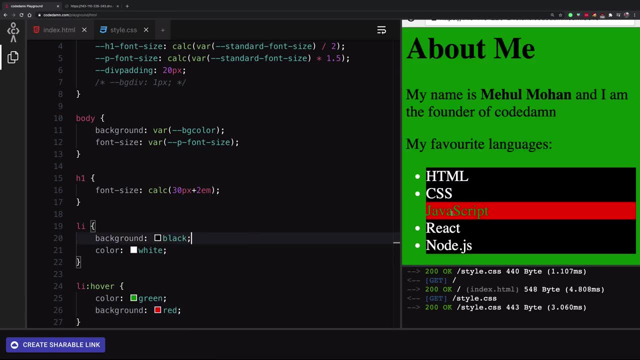 And I'm going to say, hey, once that happens, I'm going to have a color of green and background of red, Right. So now, if I go ahead and hover over this, you could see pretty much that we turn it into green and the bullet disappears because you know it matches the background color. 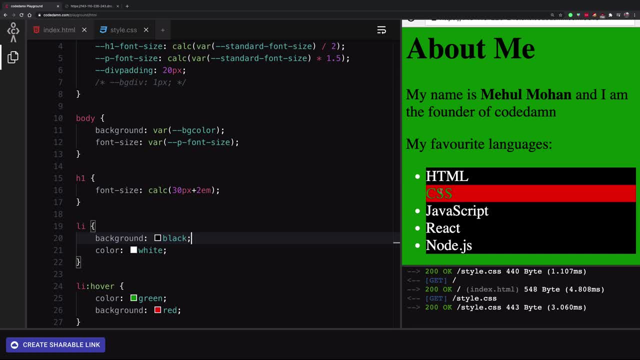 So that's why it happens And the background turns red for the Li right. So you can see that we have sort of added a little interactivity without using JavaScript at all. So that is why you know you can do a lot of stuff with CSS. 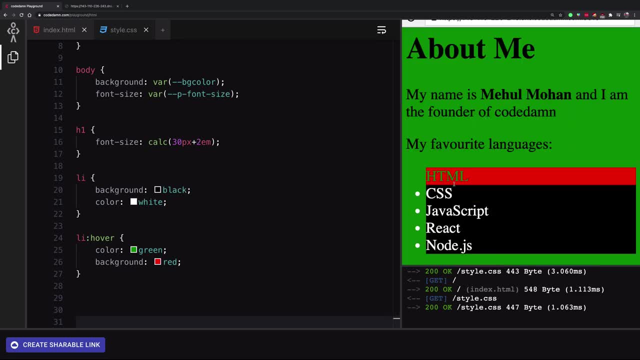 If you introduce animations and stuff, that becomes even more interesting. But this is like one pseudo selector which is, you can say, sort of a state based or, you know, user action based selector. The user did something which enabled that right. 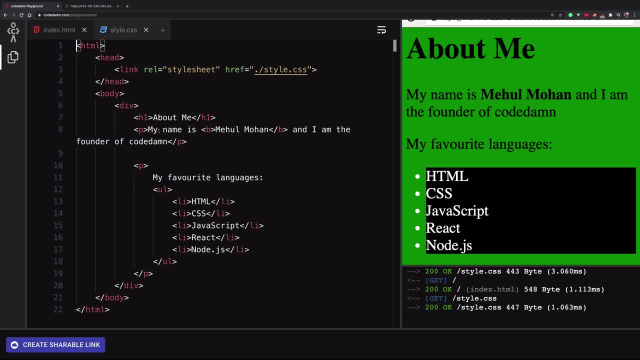 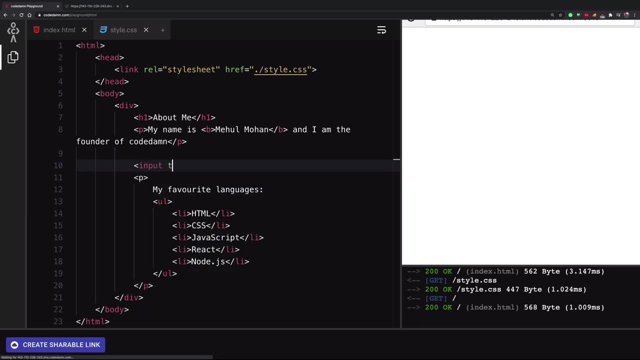 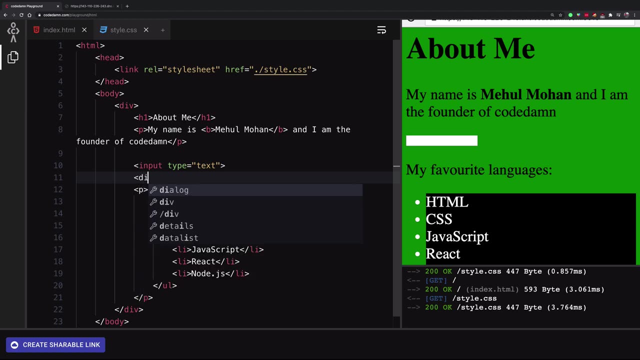 Then you have selectors for let's see, let's see if I can have a input field right here, input type text right. And now what I'm going to do is something interesting. I'm going to have a, let's say, dev ID banner. 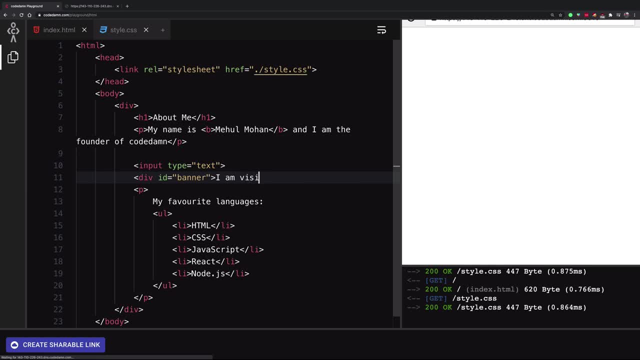 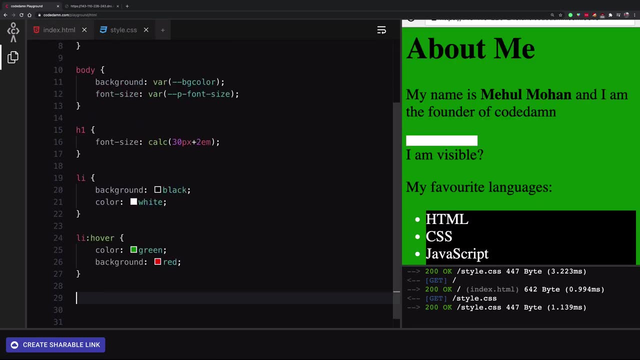 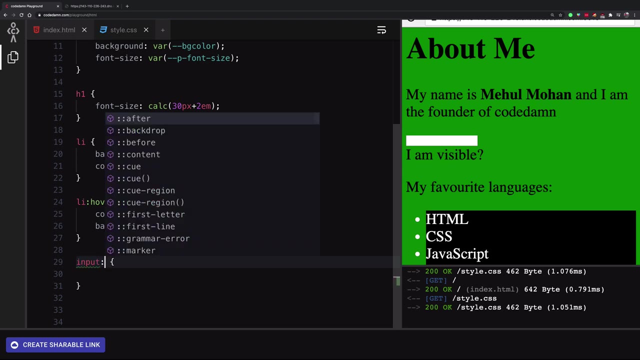 I am visible, right. So what I'm going to do is I'm going to go ahead right here and write input type text or just input, because we have a single field, And I'm going to say whenever I focus on this input again: see that this is a pseudo selector. 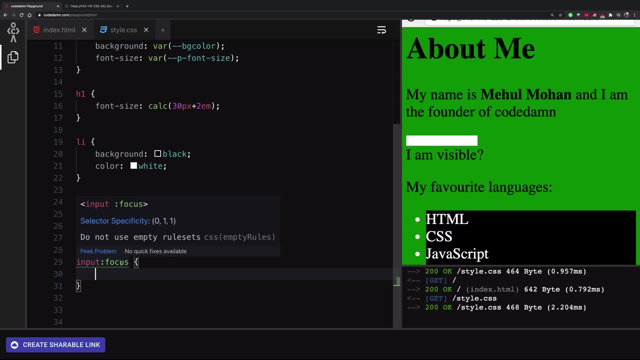 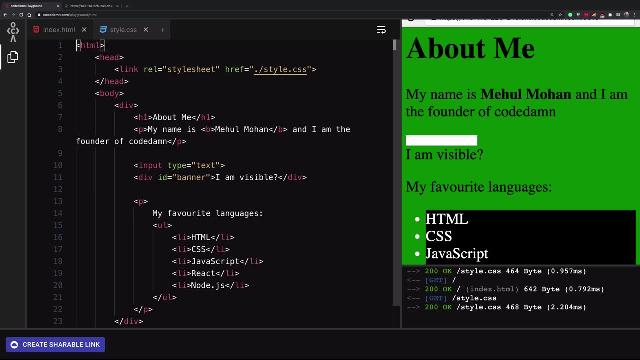 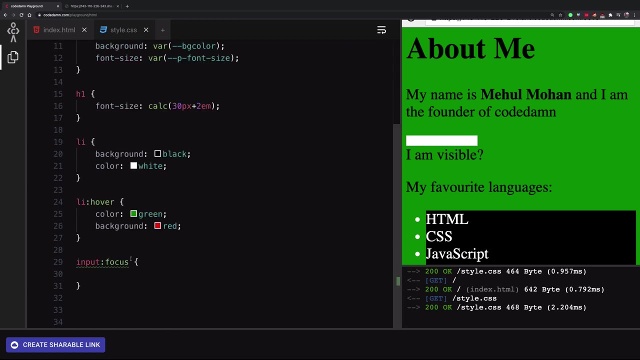 because it is state dependent. Whenever I focus on this input field, what I want to have is that I want this banner to be visible. Now, this is a sort of advanced use case. Hang up with me here. What's going to happen is how I select the sibling right. 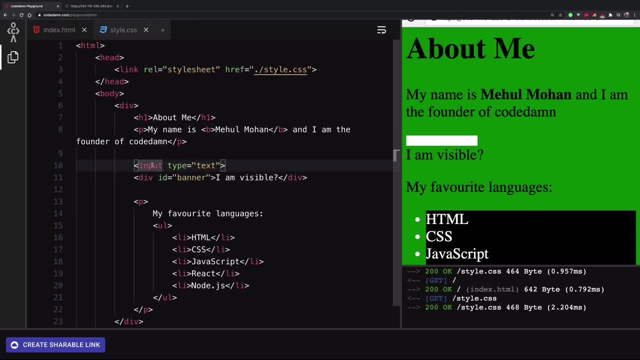 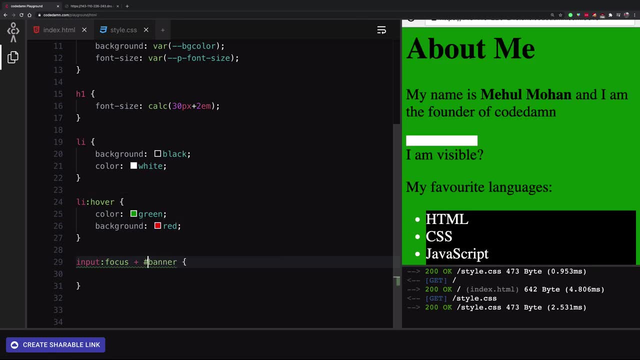 Because in this case, this banner is actually the sibling of this input field And the way to select sibling. if you did not know, it is using the plus symbol. So you know. hash banner Right. So you know, for example, if you have to select every li inside a ul, you're going. 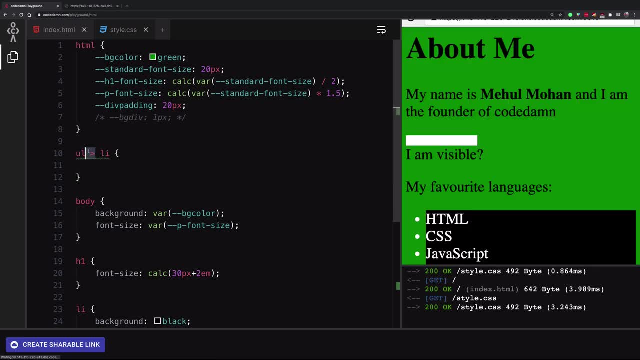 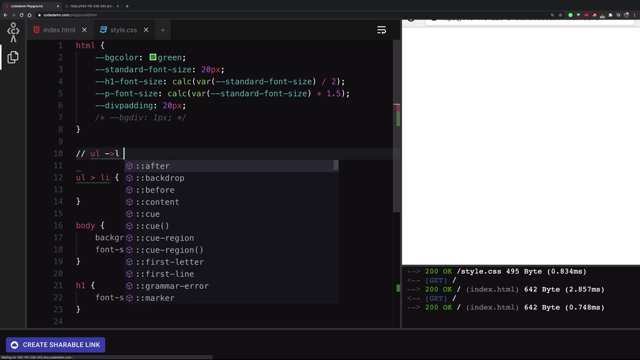 to do ul li. This means that the immediate child of ul, that is every li. So it will match a hierarchy which is something like ul and then li, But it will not match a hierarchy which is like ul and then div and then li. 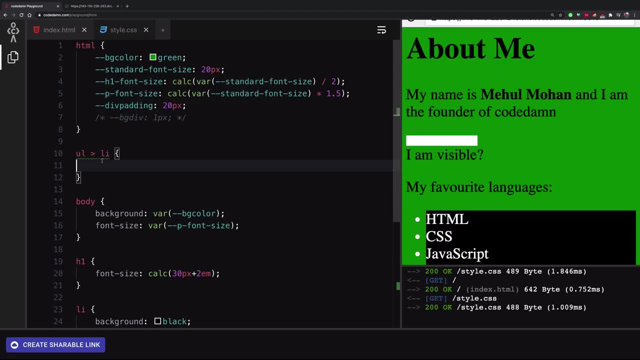 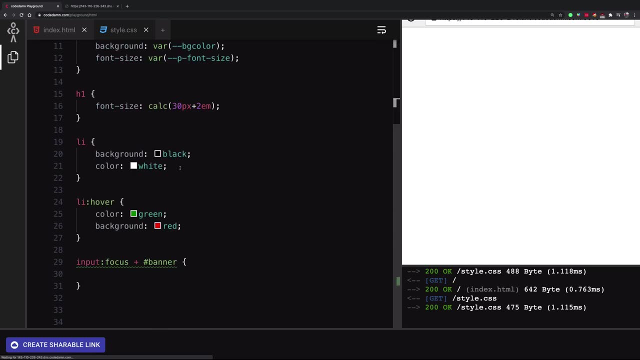 Right. So this is like one way of selecting immediate children. Using plus is another way of selecting sibling, Right? So, anyway, once we do this, you're going to see that I am just going to give this a display block. 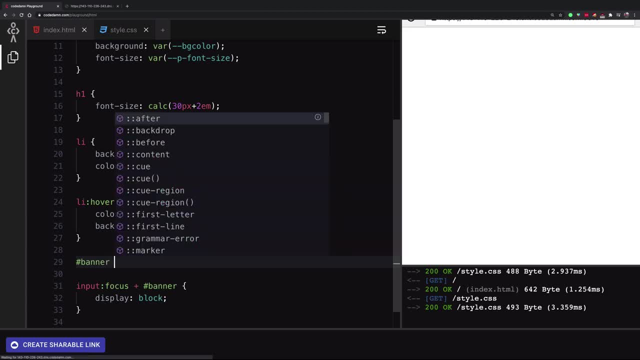 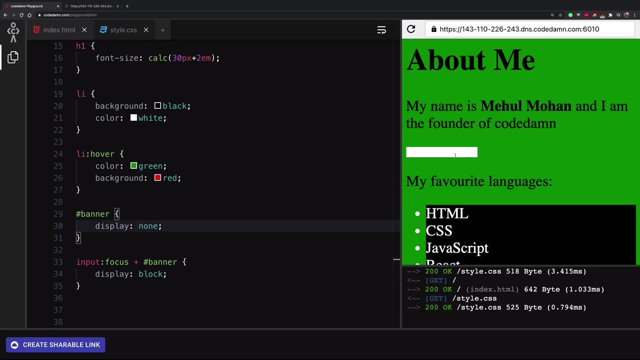 Right, And why I'm going to do that? Because on the banner, I'm going to give it a display, none. So what this means is you can see that there is no. I am visible on the screen at the moment And if I click on this, you can see I am visible, appears. 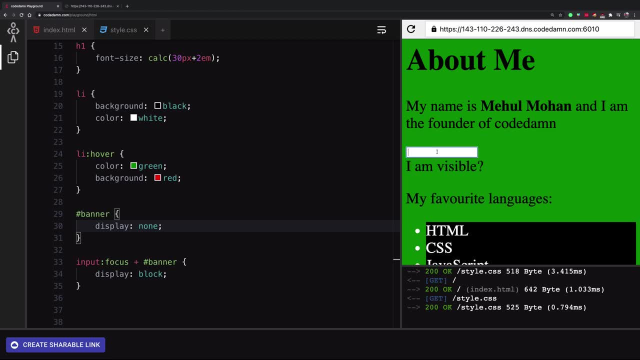 Right. So if I click out, it goes away. If I click in, it appears Why. Why does this work? It's because, by default, banner is display none And the moment I select this, this input focus event is activated. 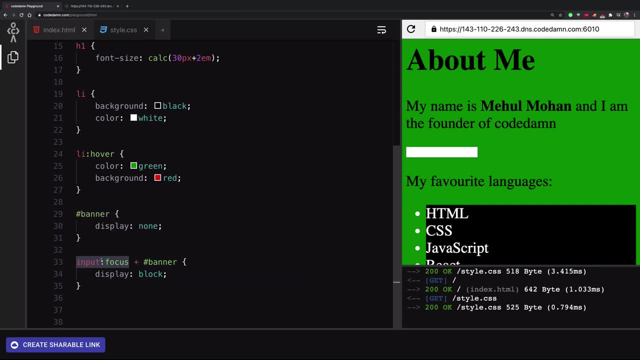 And it sees that, hey, whenever I have this input focus pseudo selector, which is currently, you know, present on the DOM, if you can just think about it in pseudo terms- that input focus element is now present on the DOM And the banner in front of it should be displayed. 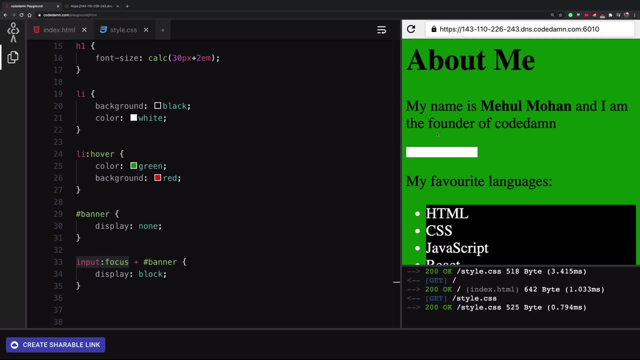 And if I click out input, focus pseudo element is now not present And the banner, you know, is sort of not there. So there's that. So it is again sort of like you can think of it's a user-based, action-based pseudo. 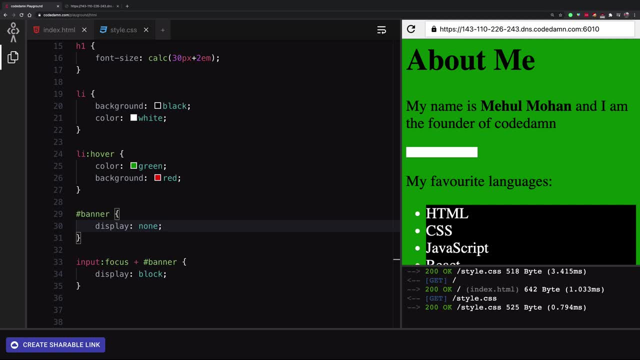 selector, And yeah, there's that. That's like one use case as well. If you want to have a little bit of interactivity with the visibility of the elements, you can go ahead and do that. However, another, which is like the most interesting use case of pseudo selector, according to: 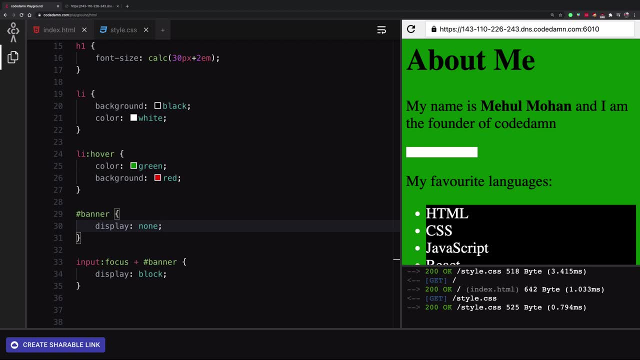 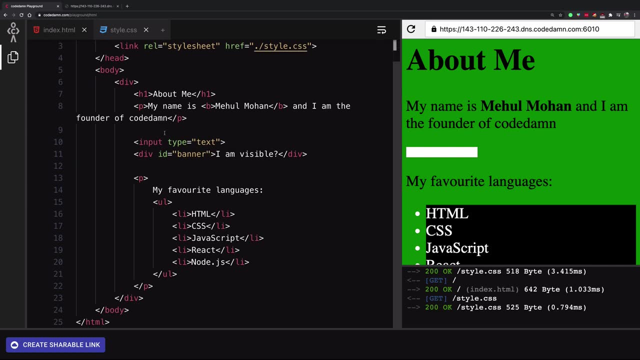 me is the nth child Right, And the nth child basically allows you to select elements which are not having any. you know they could have technically sort of a selector, But for example, let's say if I want to select only the third li in this ul list, how are 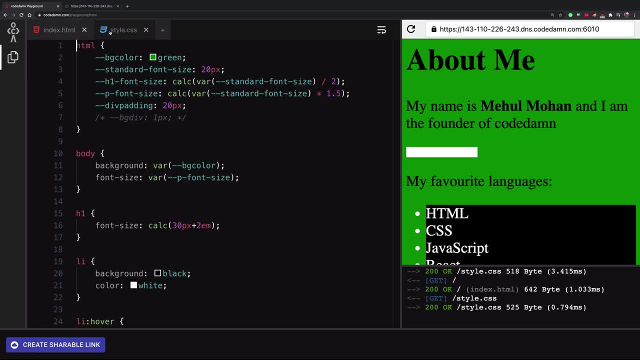 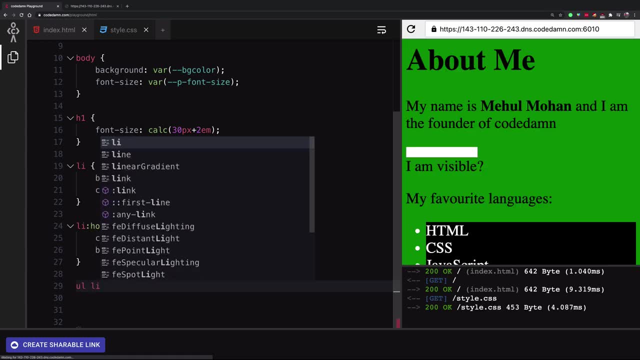 you going to do that? Well, you can technically say: you know, you can just go ahead. let's say, let's say I want to go ahead and select the third li, So you can say: this ul li selects every. let's just go ahead and work with this. 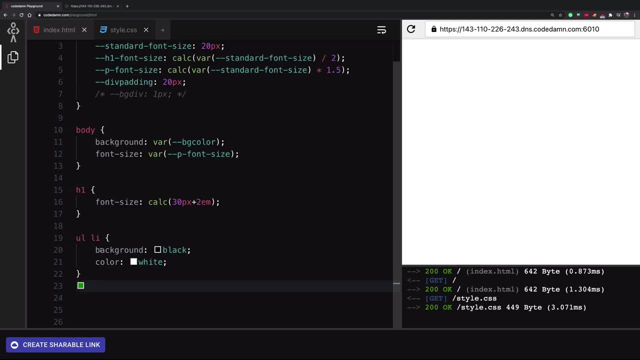 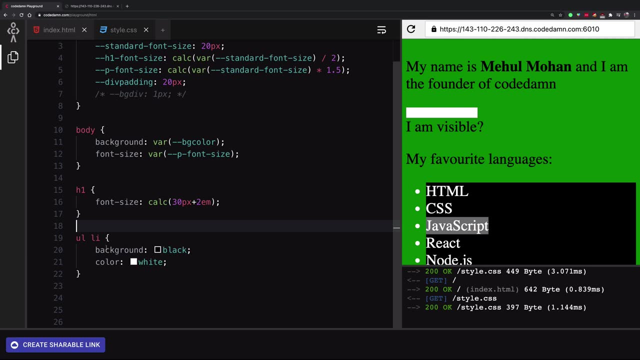 Ul li is going to select everything, and I'm going to remove this as well. So I don't want to do that. I only want to have the third, that is, the JavaScript, being selected. So you can- you know- do this just like, because you know, I told you how to do that. 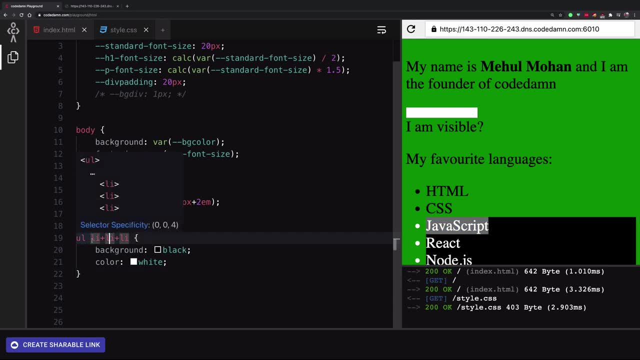 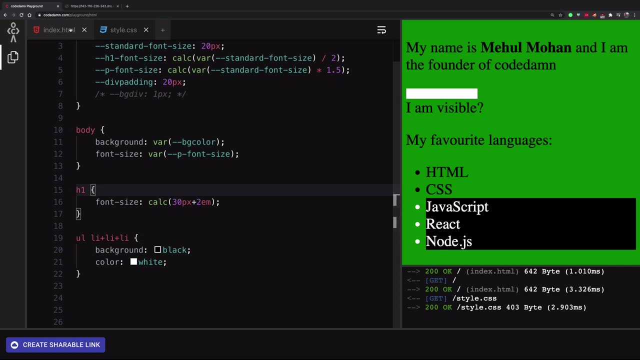 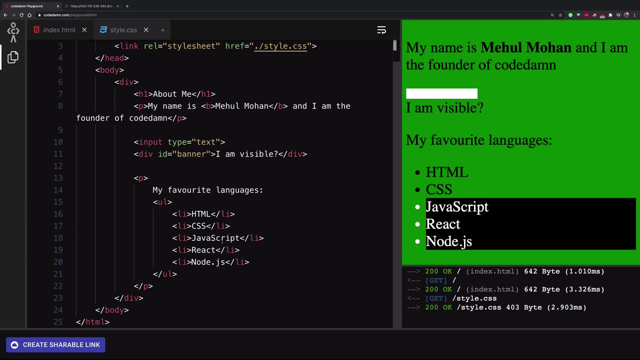 But you can see, it kind of does not work, because this li plus li plus li selects the last three. and the reason they select the last three, it's interesting, is because li plus li plus li means the li, which, the li, which is the sibling of li, which is the. 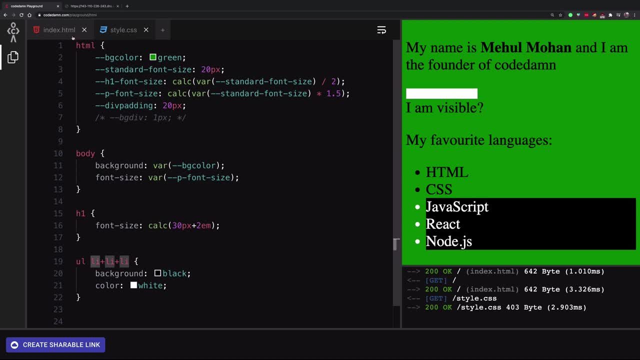 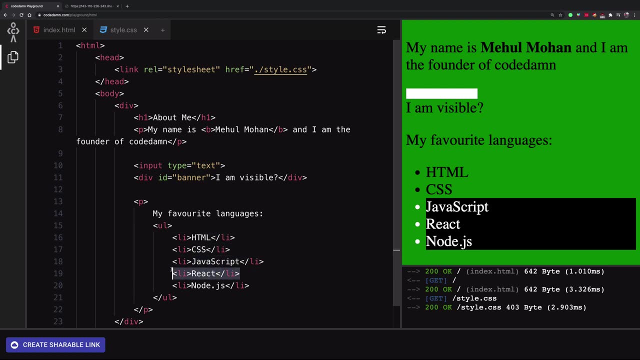 sibling of li right. So this constraint is fulfilled by the third one, because you know this is li plus li plus li. But this is also fulfilled by the fourth one, because you know this is li plus li plus li, and the fifth one and the sixth one. 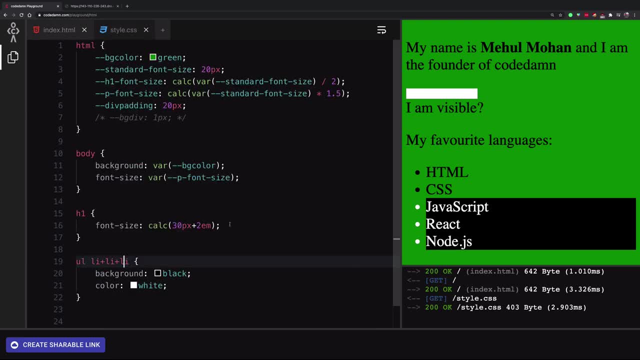 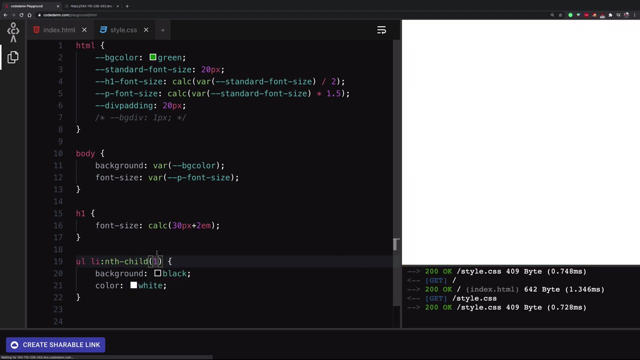 So you know this did not work pretty much and, to be honest, I cannot really think of a way to make it work without any class or id and without nth child. So I'm just going to explain nth child. So what nth child does is that if I go ahead and write nth child right here and write 1.. 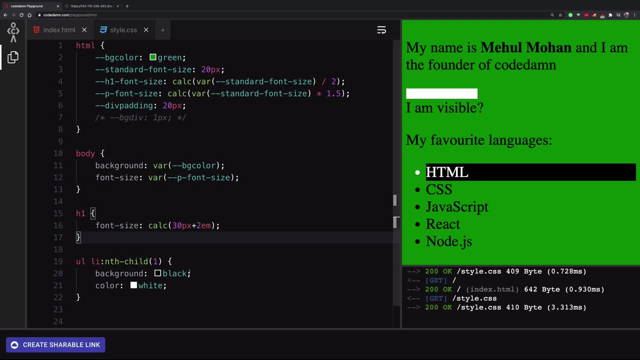 So let's see what happens. You can see that the HTML is selected. If I go ahead and write nth child 2, you're going to see CSS is selected. If I go ahead and write nth child 2, you're going to see CSS is selected. 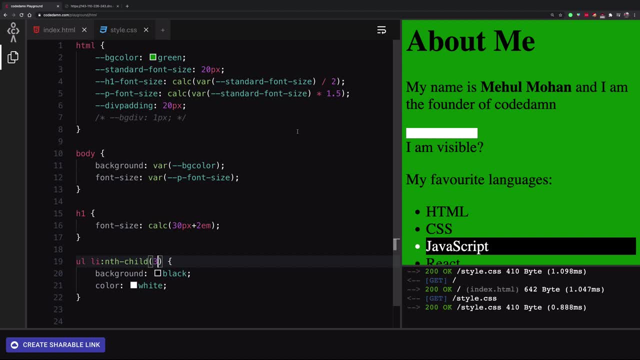 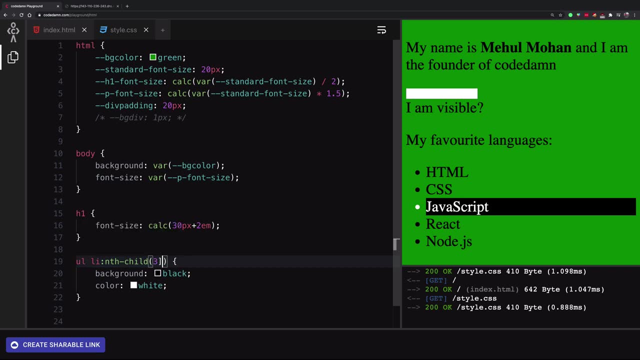 If I go ahead and write nth child 3,, JavaScript is selected. So I hope you get the pattern here. You can actually give it an index and remember this index is actually 1 based right. nth child 0 is nothing, right. 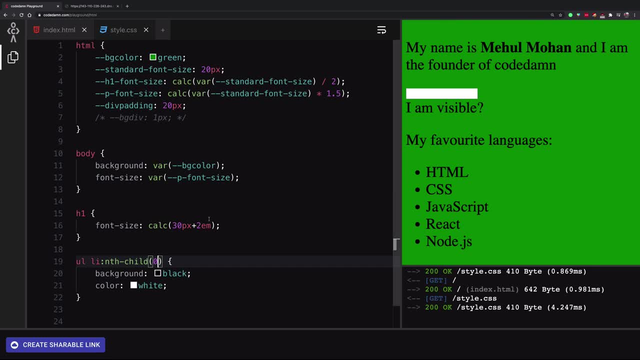 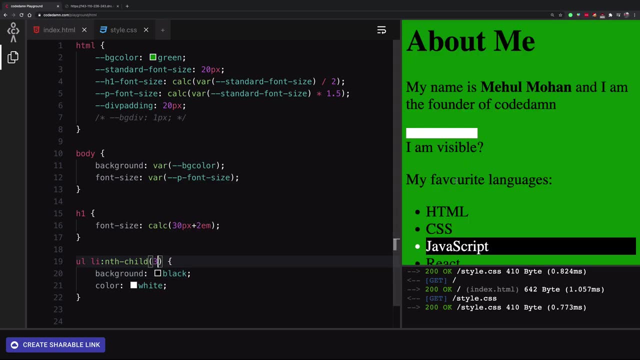 So nothing would be selected. So you have to remember that this index is 1 based and not 0 based, So you can give nth child 1,, 2,, 3,, 4, and it will just work, just like you know it. 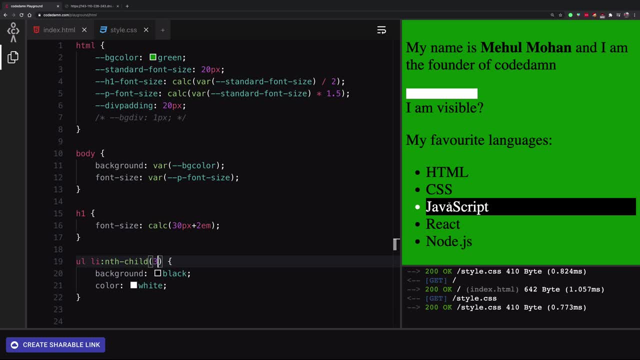 will just pinpoint, select that element. But things get very, very interesting with nth child. Why? Because you can sort of give it a dynamic input as well. What do I mean by that? Let me just go ahead and give it an nth child of 2n. 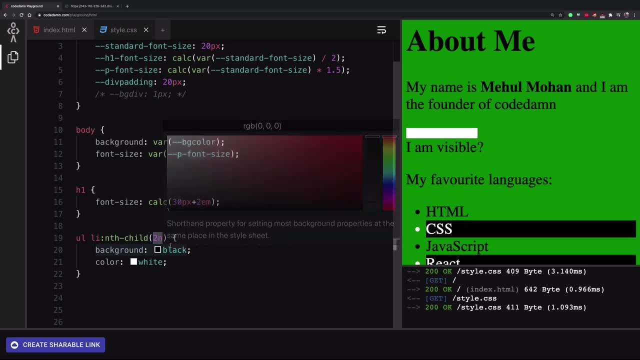 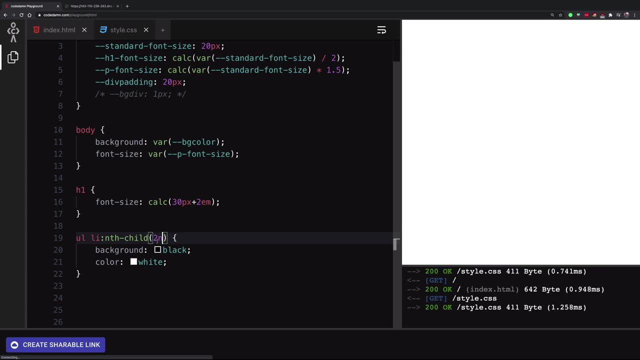 Now this is a special, you know. It's not like you can give anything except n. You cannot give like f or anything. It would not work. You have to use the variable name as 2n, right, Or not really 2n, just the n right here. 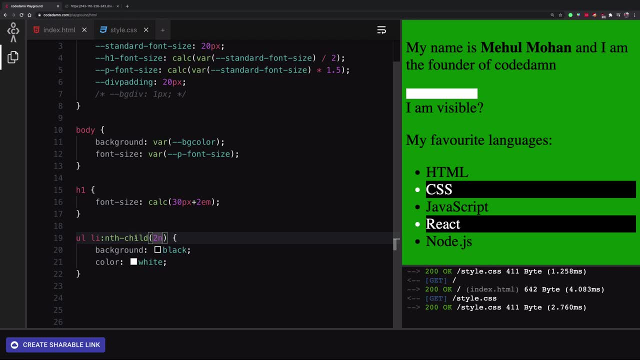 Now, what does this mean? This means that what CSS engine will do is that it will take this expression right here and it will start giving it values right. So if I write n, what's gonna happen? If I write n as 1, what's gonna happen? 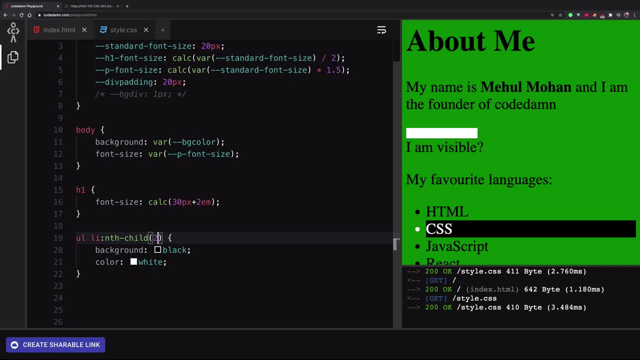 We're gonna get 2.. So CSS is selected. If I give n value of 2,, what's gonna happen is 2 times 2, 4.. So React is selected right. So if I give 2n, it's basically equivalent of writing ul nth child like this: 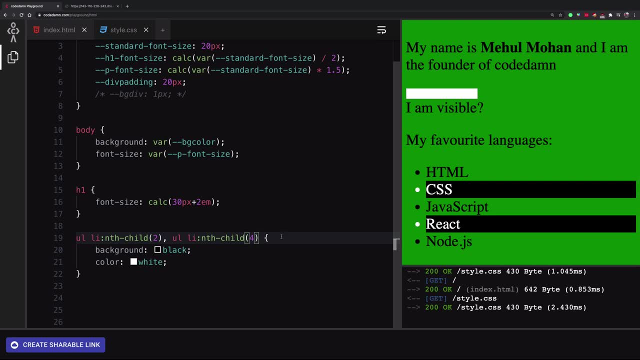 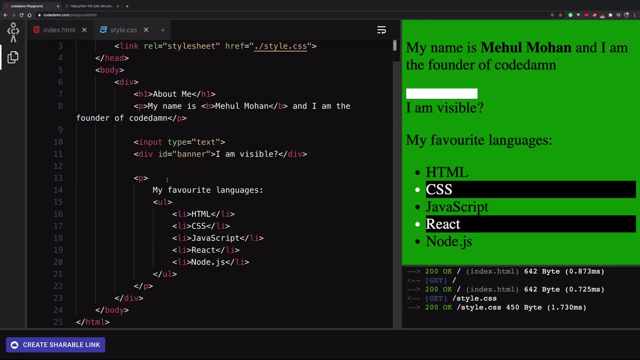 and then like this: right, And it is technically equivalent to. you know this as well, But you cannot really see it because there is no 6th element on the page. However, if there were, let's say, another node, js. 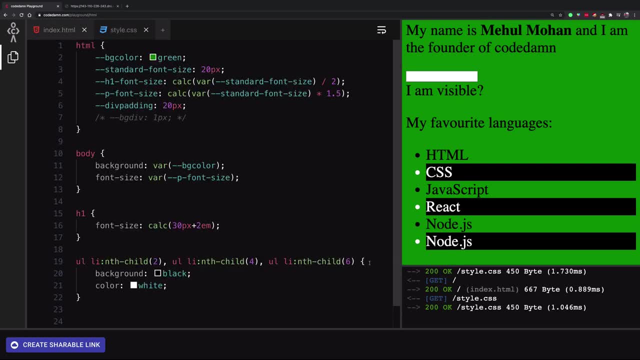 then we'll see the 6th element highlighted as well. But this approach, this approach right here, will fail with the 8th one. However, if you just write 2n, it's just gonna work fine, right? So it's just gonna work like this. 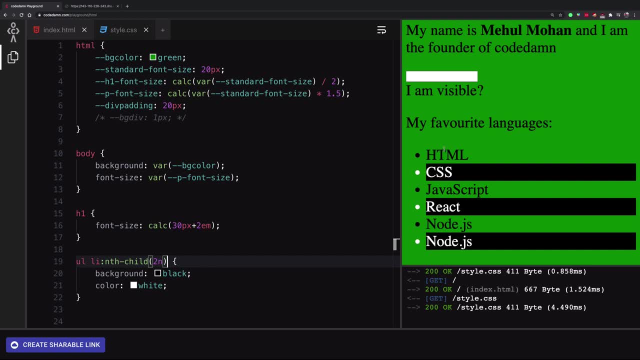 So 2,, 4,, 6,, 8, all the odd- not really odd even in this case- will be having background black and color white. This is also interesting because you can play a little math here as well. 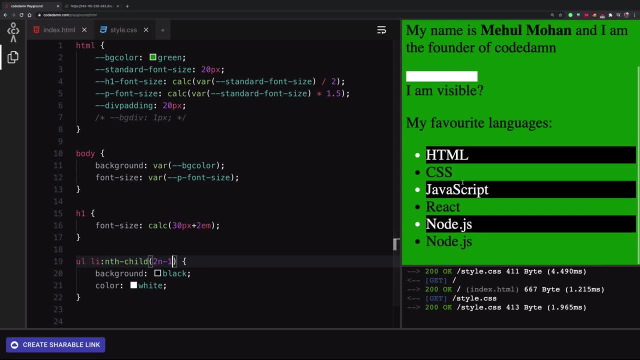 You can also subtract, So you can see that earlier we had all the odds, Now we have all the events. I spoke like in the reverse: Earlier we had all the events, Now we have all the odds. So you can see it starts with HTML JavaScript node. 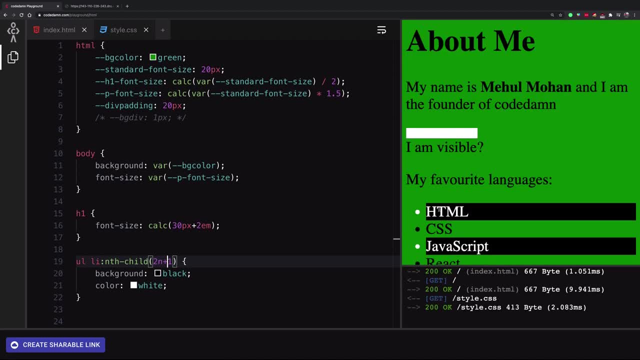 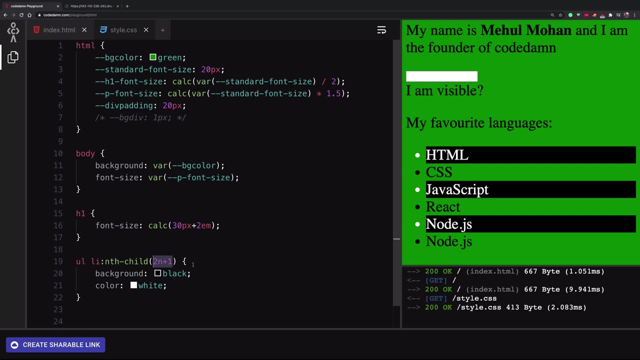 And you can also add to this stuff, right? So if you have done a little bit of you know algebra, you know that this is. this looks like sort of expression for all the you know odd natural numbers, right? 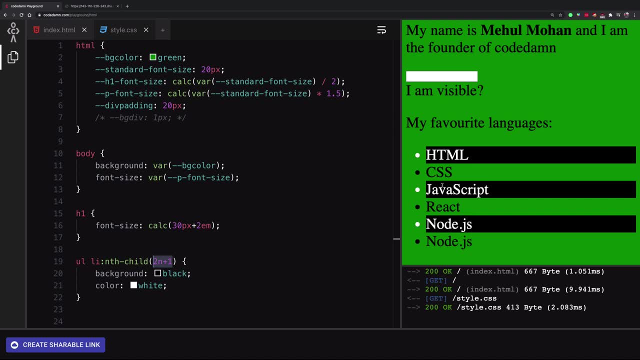 So 1,, 3,, 5, 7, 9.. That is why, if you were expecting that HTML will not be highlighted, you were wrong. right, Because this starts filling up with 0, right, So if you have a 2n minus 1 expression, 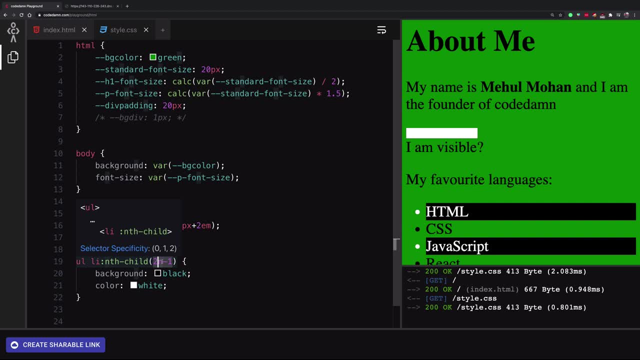 it will start n by putting it 0, right, So if you put n as 0, you're gonna get negative 1, which does not make sense. So it's just gonna skip that. So it's just gonna skip that. 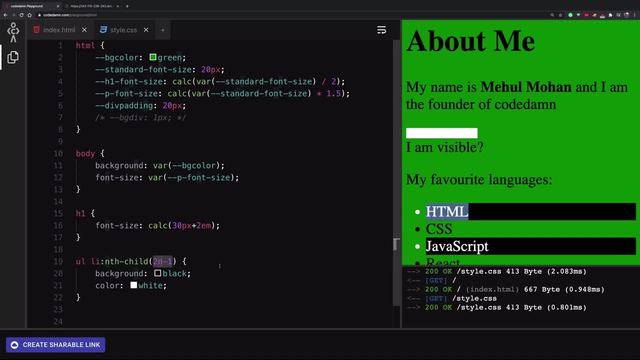 So if you put n as 1, it's gonna be 1.. That is why HTML is there. If you put n as 2, it's gonna be 2 times 2, 4 minus 1, 3.. 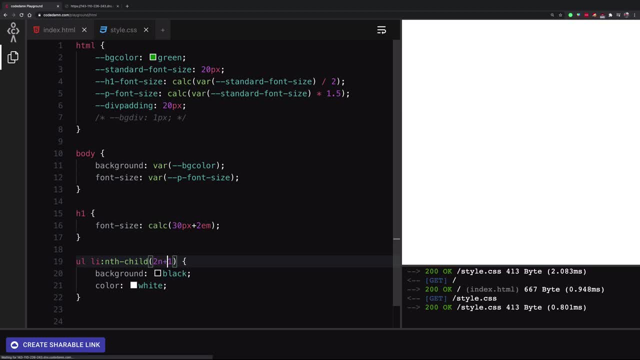 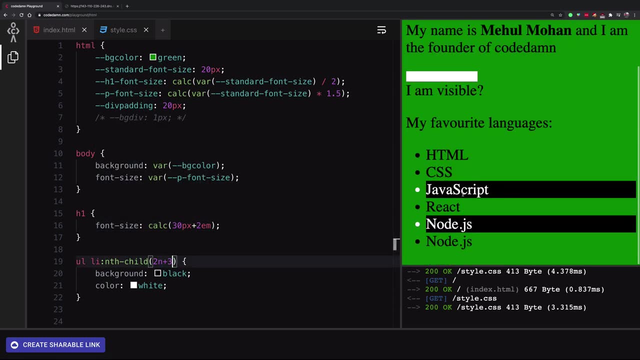 That's why JavaScript is there and so on. But with 2n plus 1, you already have. if you put 0, you have 1, right. However, if you do a 2n plus 3, you're gonna see that HTML is not covered now. 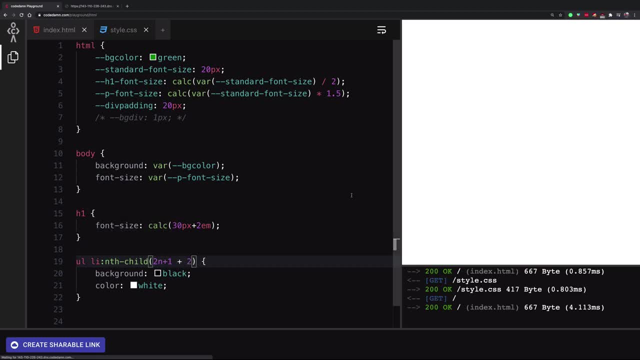 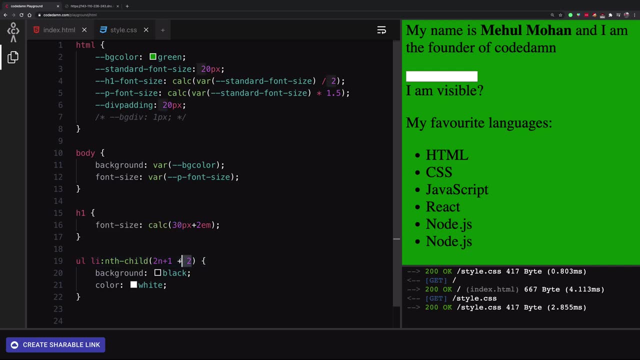 Why? Because this is technically 2n plus 1 plus 2, right, And you might see that this is. this is not like how calc. it's not as flexible as calc, So you can have only 2 expressions at the at the given time. 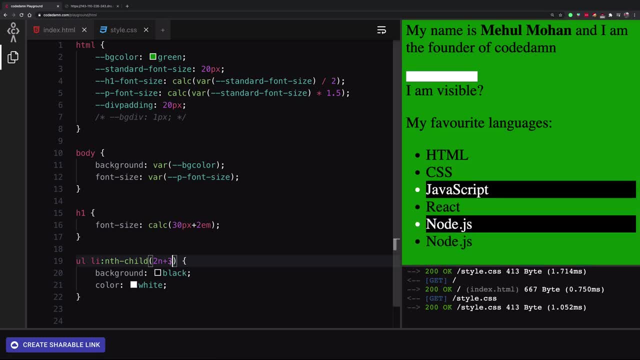 So you have to stick with 2n plus 3.. But what's happening here is that if you put 0 in this n, it actually has to start from 3, right? That is why it starts from 1,, 2,, 3.. 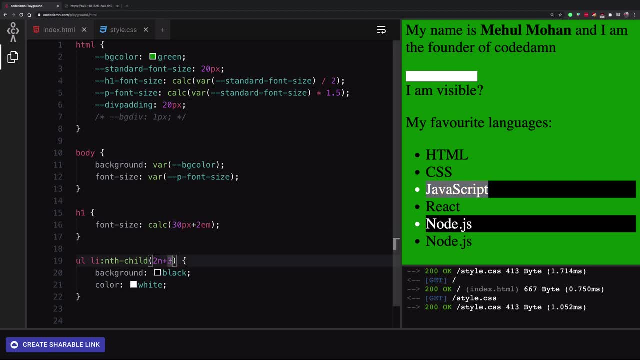 So this is like super cool and super important thing as well when you're working with CSS, If you want to target elements based on, you know, randomness, a little bit of randomness, or maybe like a pattern, if you want to have. 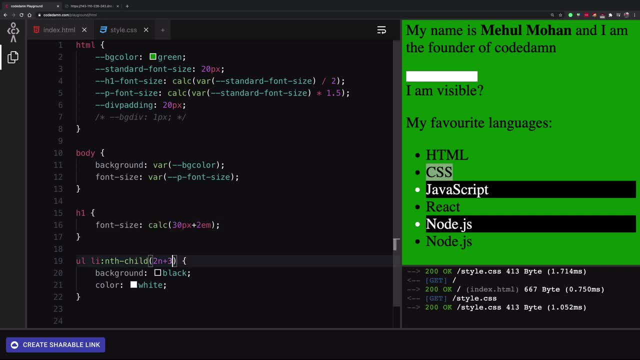 I don't know- a different effect on odd and even elements. you know, if you want to have a different effect on every third element, this is also possible. So there's that. That's how you do this using nth child right. 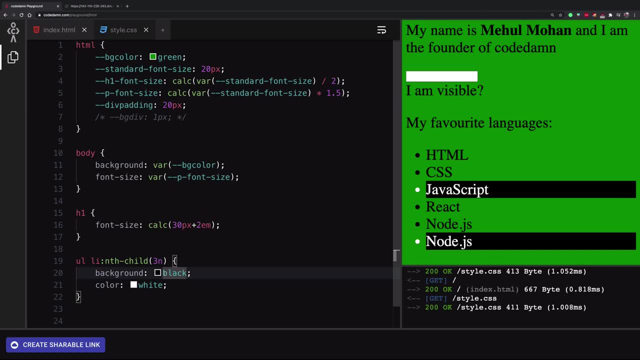 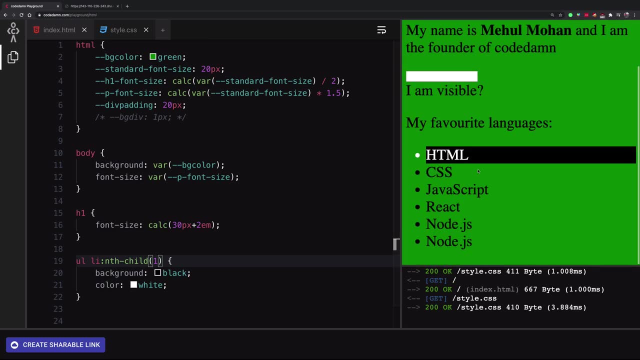 So with nth child there is actually a little bit of convenience and that is like. a lot of times people use nth child for targeting first element or maybe like last element as well. So how do you target like the last element? It's not really a sort of a way to target last element with nth child. 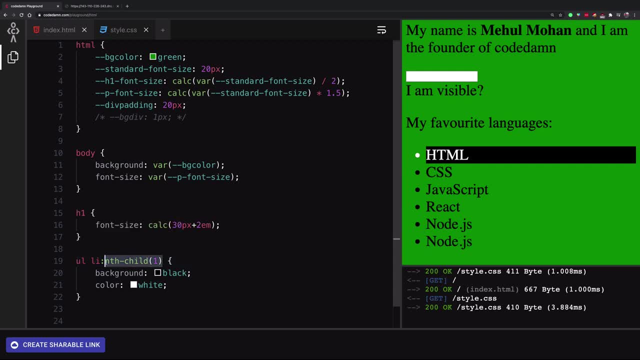 as far as I can remember. But what you can do is you can use some more pseudo selectors. The next one is going to be last child, So last child. just like the name says, it's going to target the last child of that particular selector. 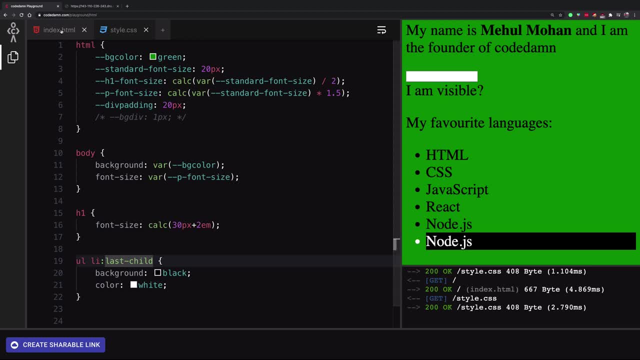 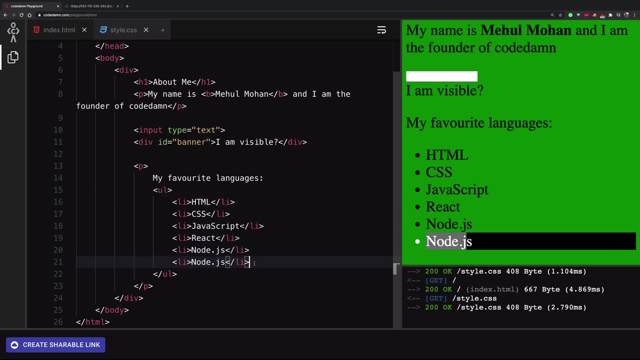 which you are targeting. This means now remember this does not mean that it will only target one single thing. It means that ul li matches all these li's and the last li in this one is this: However, if I sort of like duplicate this list, 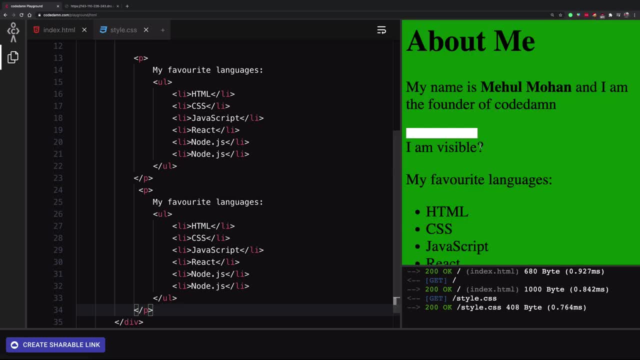 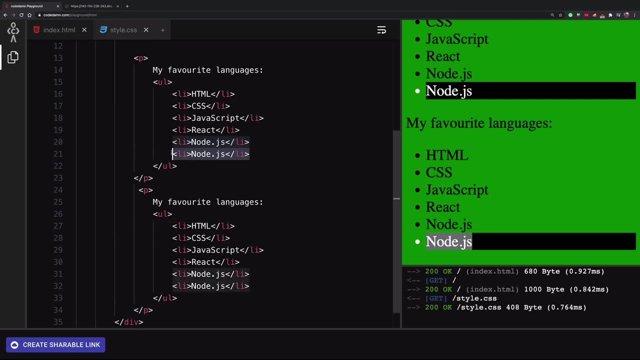 it will still target that thing, It will still target the other list, So it targets this one and it targets this one as well. right, It's not like a single selector base, It's just that in that particular selector itself, ul and li. 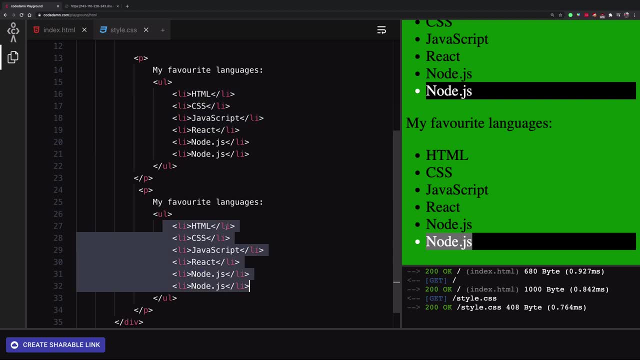 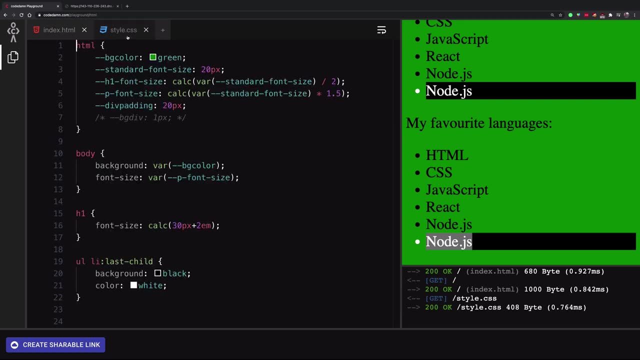 it has so many options. it has so many options and out of all these options, it's just going to target the last one And, obviously, if there is just a single option, it's just going to target that one. On a similar basis, you also have first child. 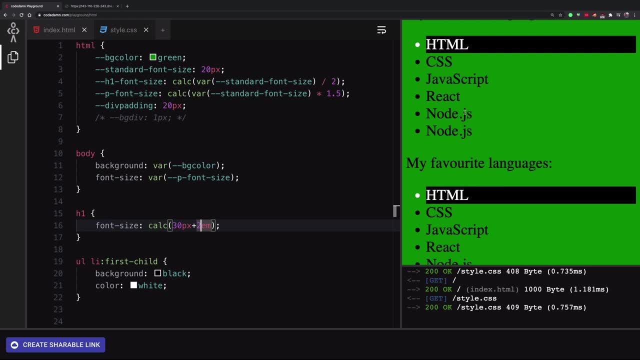 Right. So you have, you know the same behavior, and we already covered nth child. So there are a bunch of more CSS selectors. I'm not going to get into depth of every single one of them, because if you need them, you can sort of like use them. 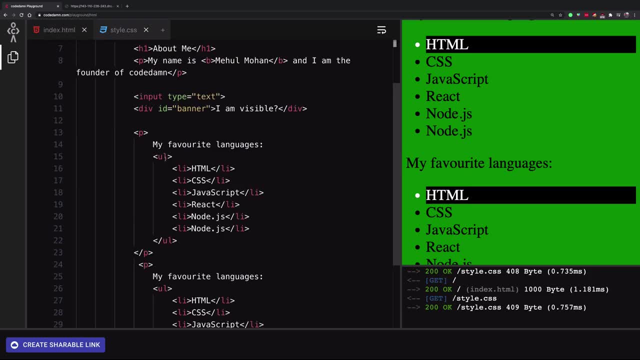 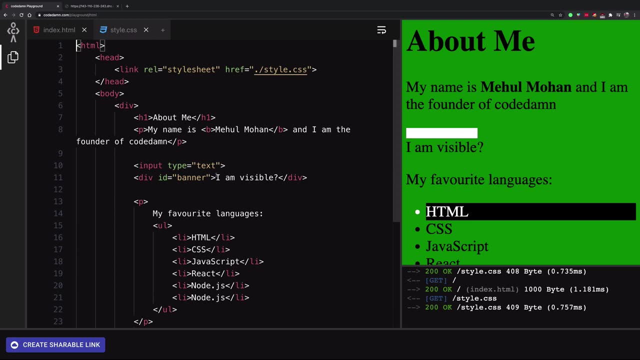 because you know, if you have like, for example, we can also discuss real quick with the input selectors a little bit Right. So we have an input field right here and, following the same sort of strategy for input, what we can say is that: 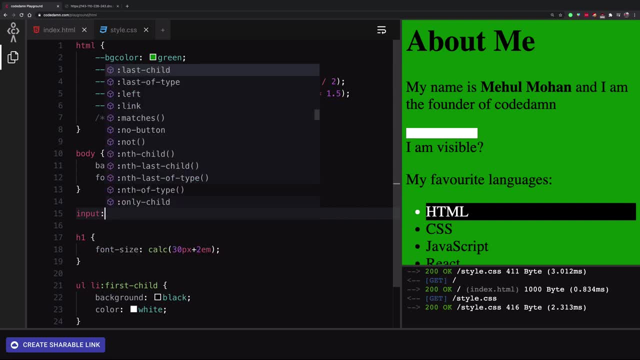 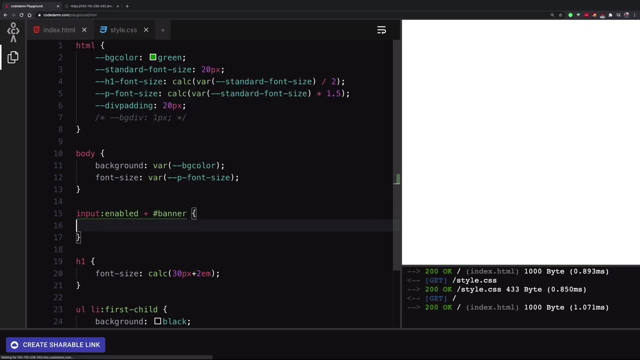 let's say, if input is- I don't know- enabled, let's see. And then, if I have a banner in front of it, I just want to display none Right, So you can see, right now the input is enabled. 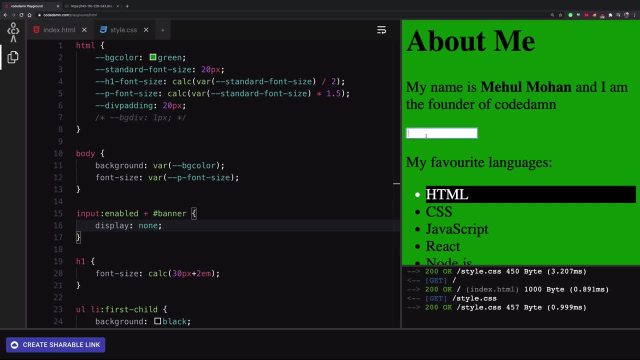 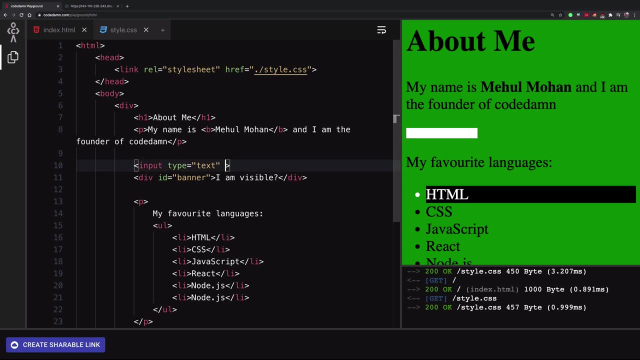 That is why the banner is not displayed. Let's assume that there was a button here which disables the input field, That is, you cannot really enter anything else. So if I add a disable, an enabled attribute to sort of mimic that behavior, 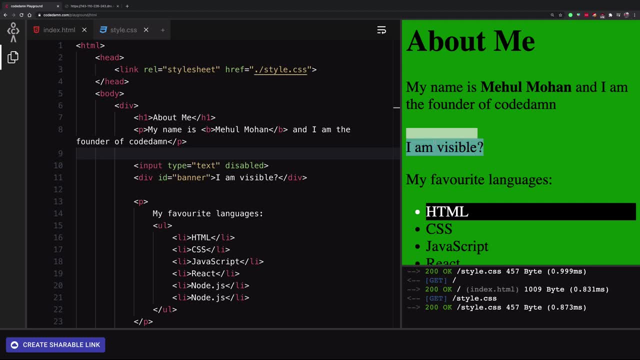 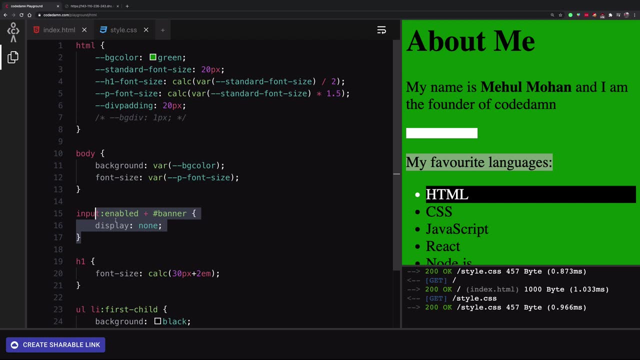 you can see now that because the input is disabled, now I am able to see the banner. If I remove this, I will not be able to see. I am visible. So again, this is also a sort of a pseudo selector. Now there exists a lot of pseudo selectors, you know. 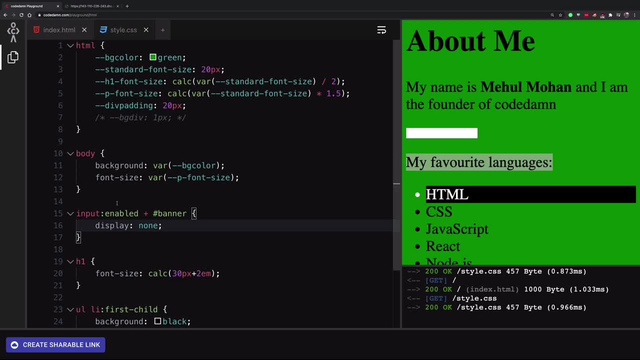 checked disabled blank pseudo selectors also there which we can probably show in a much better way. But blank would not work right now because it's an in-work progress, So it will land later on in the specification. If you are watching this video, try out blank and see if it works. 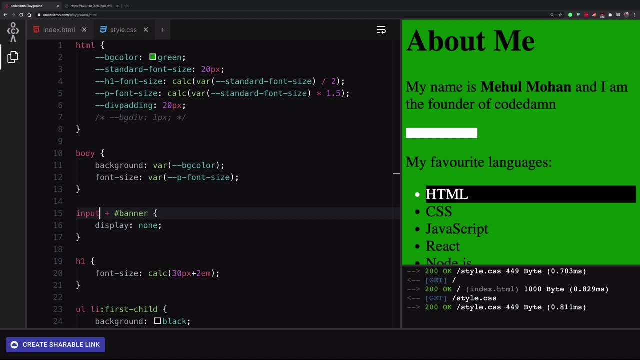 If it works, then you are from, you know, the distant future. But yeah, it does not work at the moment with browser, But it is definitely under the spec. So, yeah, there are other selectors as well. You are free to take a look at all of them if you want. 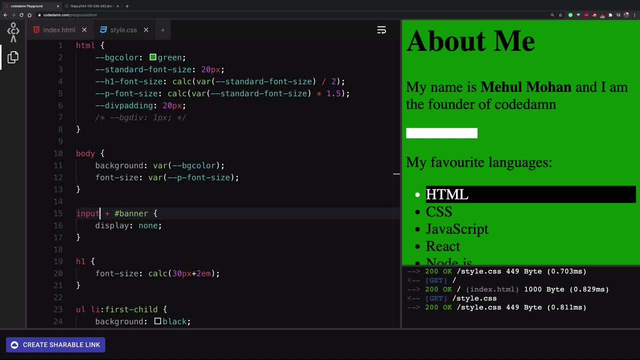 But that's pretty much what you would need in a nutshell when you are starting off. So that is all for this video And I am going to see you in the next one. Hey, everyone, welcome back. And in this video we are going to be taking a look at. 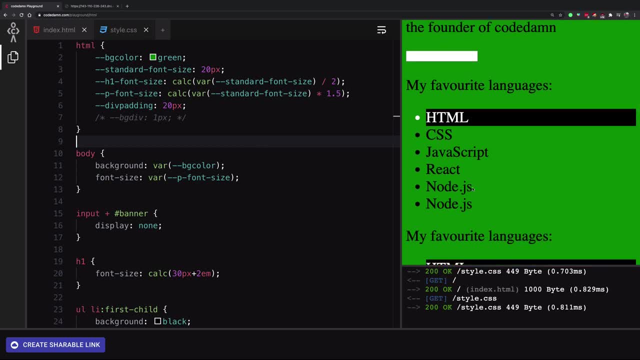 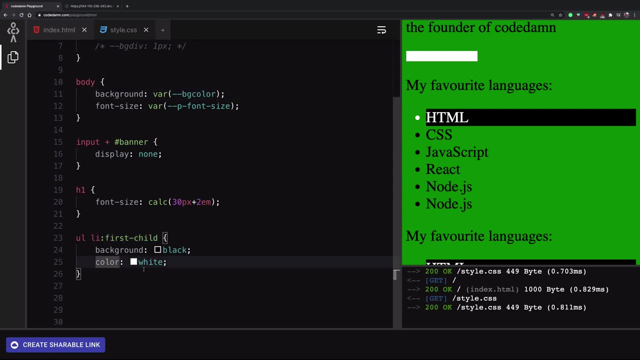 something super interesting with CSS, and that is the presence of pseudo elements. right? So so far we have been using pseudo selectors, nth child and all that stuff- But actually CSS brings in pseudo elements as well. What does that mean? You know, pseudo stands for fake. 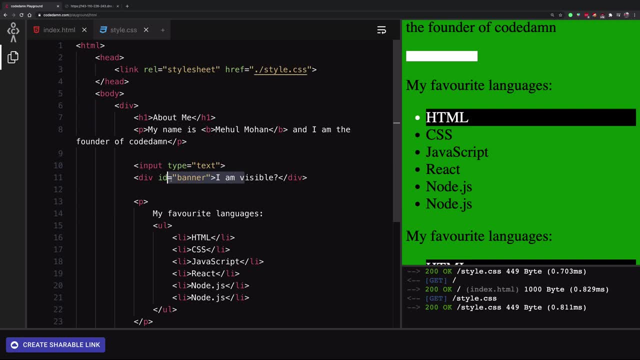 and element is basically: you know what you are writing on the screen, right? So what does it really mean to be a fake element? Well, firstly, realize that this is just going to work with the elements which have an opening and a closing tag, right? 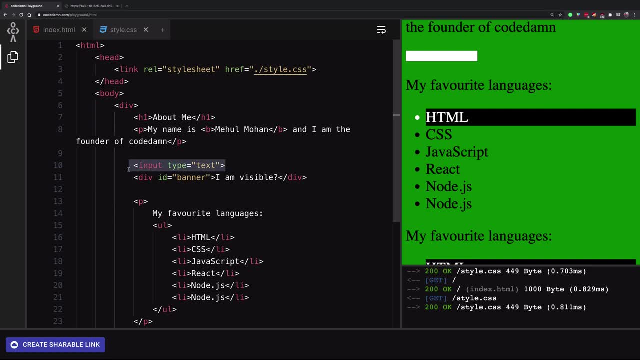 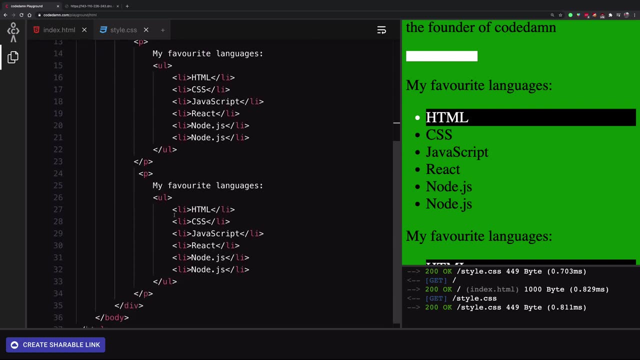 By this what I mean. it will not work with this strategy which we will be discussing. It will not work with input, It will not work with IMG, It will not work with- you know, pretty much like HR or BR or any tag which is self-closing. 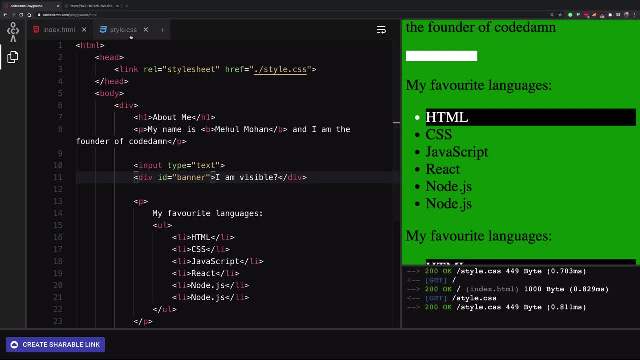 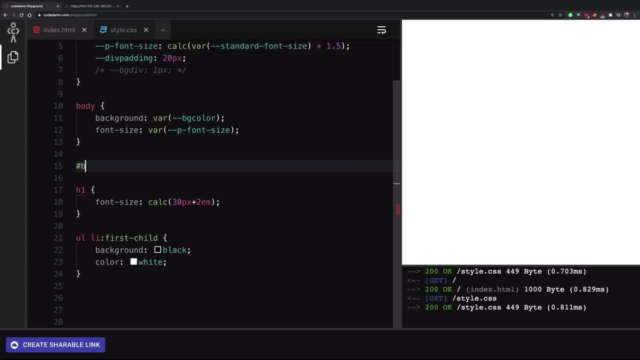 So, with that being said, what I want to do is I want to jump into my style sheet and let's take example of this banner itself. So I am going to have a banner here. I am going to give it a color of purple. 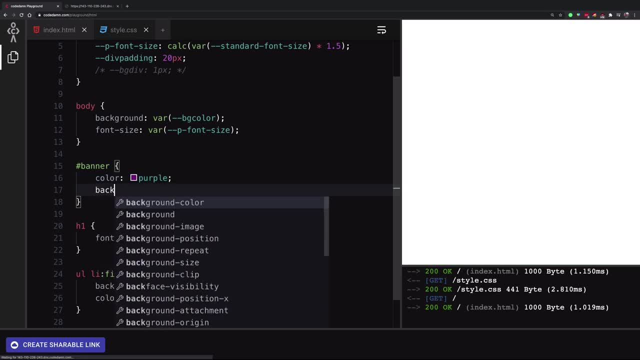 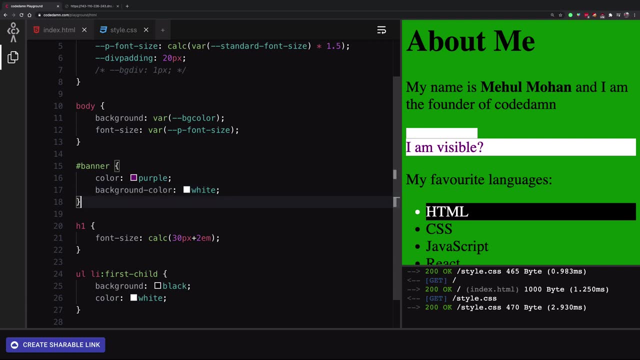 Let's hope that is visible, sort of Give it a background of white, Why not? Right. and now what I want to do is I want to add pseudo elements to it. Now, how do you add pseudo elements? or sort of, how do you target pseudo elements? 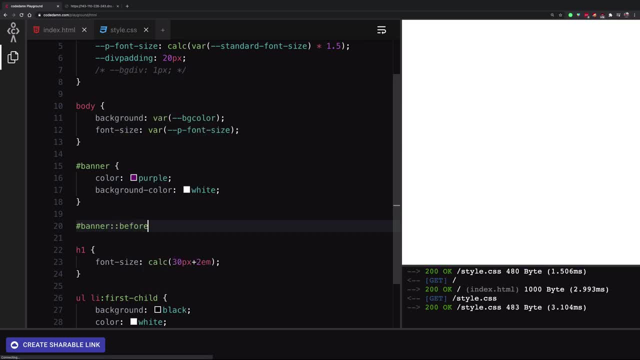 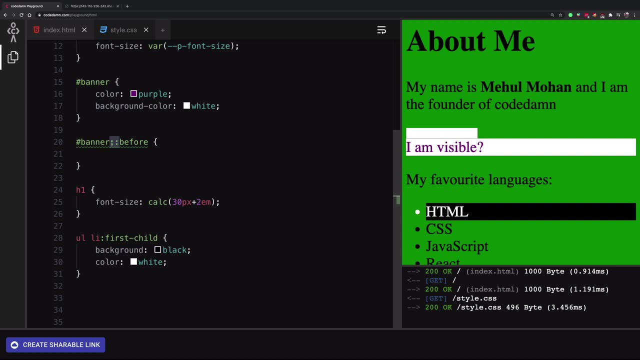 You say banner before right, And yeah, one quick thing, one very quick thing. I think I missed it. You might see that some selectors use this double notation of double columns. Some might use single one, right? So what is the difference? 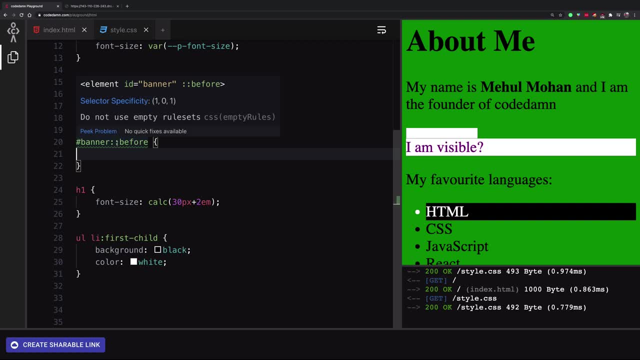 Well, remember that, first of all, when you are using double, whenever you are using double, a single is also valid, but not the other way around. For example, a double on this is not valid Right. It is also, it only. 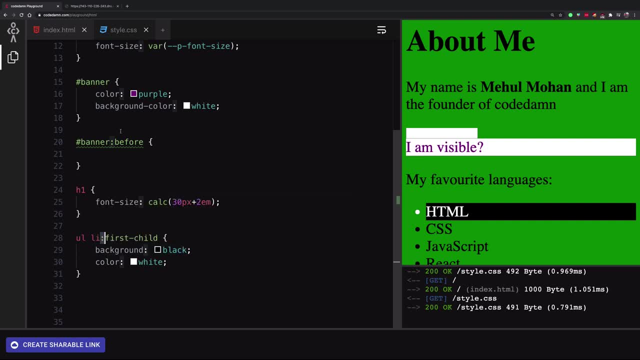 the single column is only valid here. Now, then why do we use double at all? Well, we use double to denote that the selector which we are using now is pseudo element, not a pseudo selector. Why, what do we mean by that? 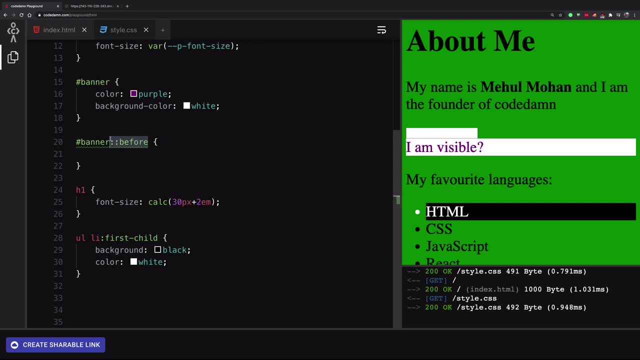 That means that this is actually sort of targeting a DOM element on the page itself. You know it's not really a DOM element, That's why the name is pseudo, But it will behave like one, So let's just go ahead and give it a content property. 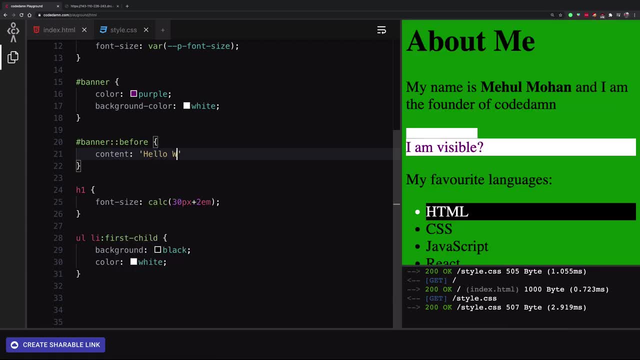 I'm gonna explain now. Let's say: hello, world Right. And what we did is we just wrote a string right here and magically it appears on the screen. Wow, I mean, we did not know that we can actually write with CSS now. 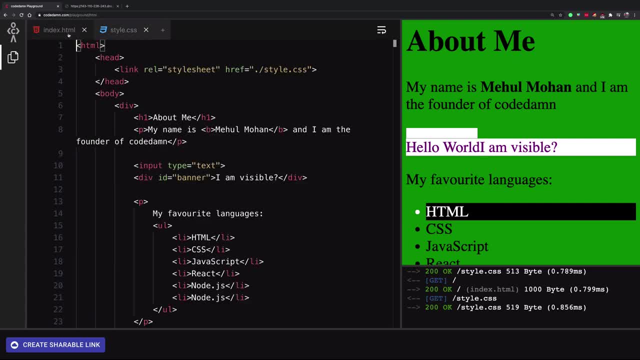 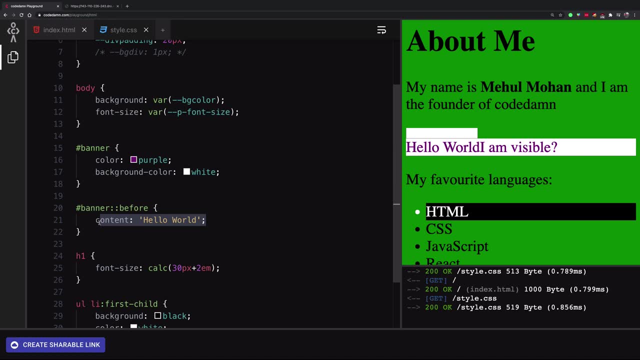 did we? Because, you know, we always assume that HTML is the one which shows the text and CSS is the one which, you know, programs all the colors and layouts and all that stuff. But it is actually possible to write with CSS as well. 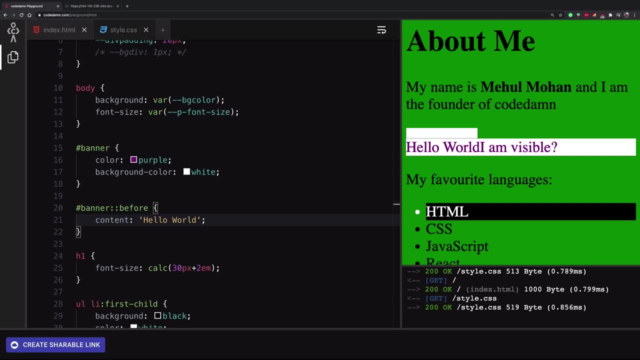 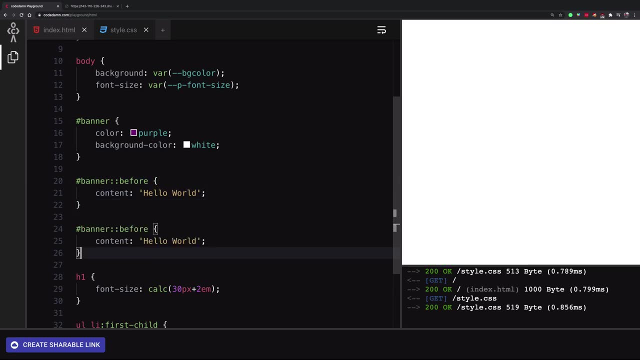 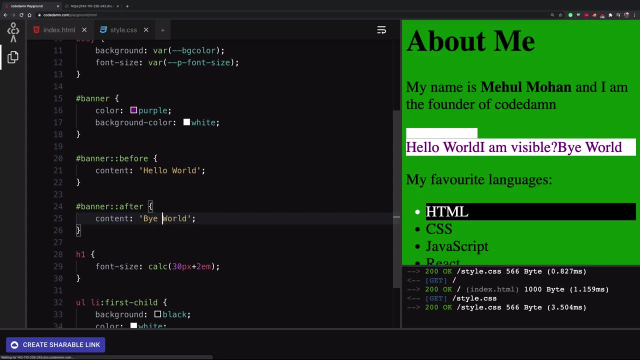 So this is like one way of writing with CSS right. Another thing which I can tell you is that before also exists. there's an after pseudo selector, which also exists. So if you go ahead and write after here, you can say: by world right. 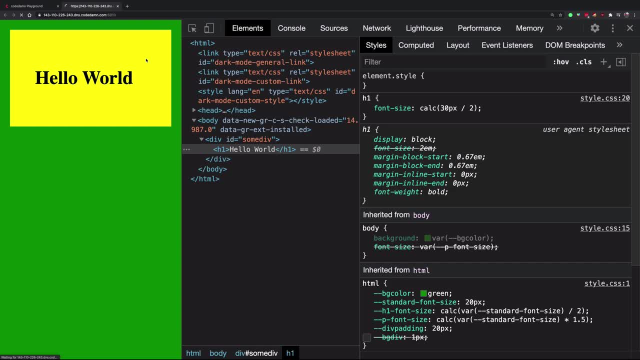 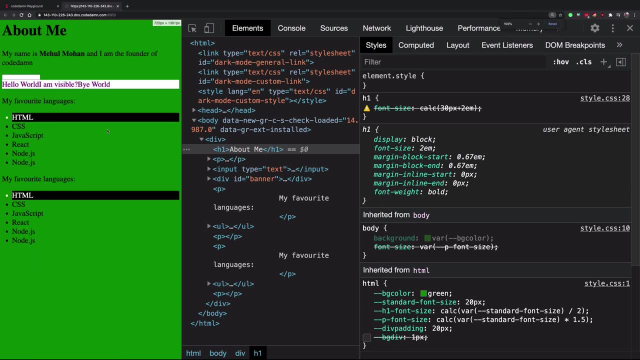 So there's that. So if I go ahead and open this new tab and refresh this and if we go down right here, I think we are zoomed in a lot on this page, Yep. So if I go ahead and select this, hello world, and by world. 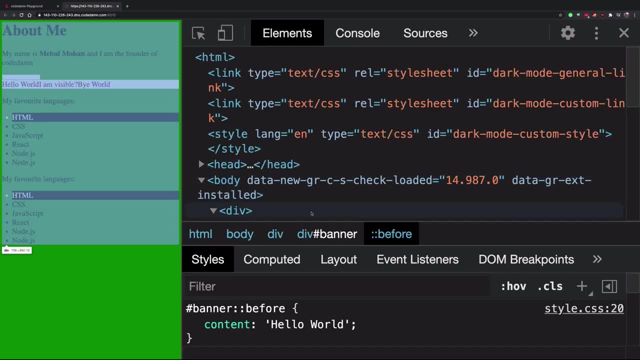 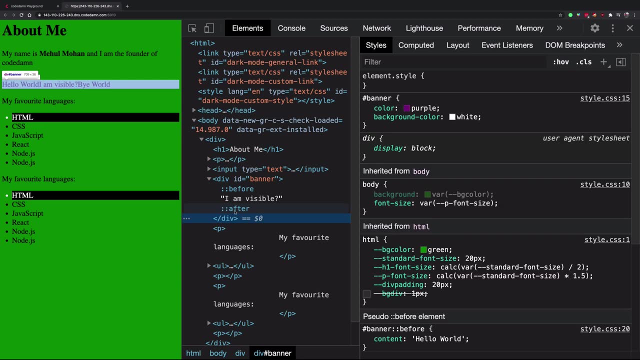 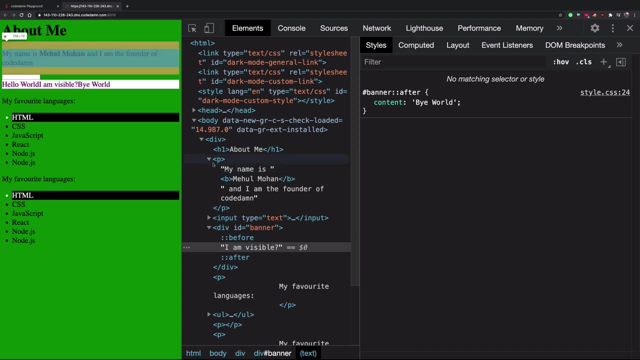 you can see right here, you can actually see in the DOM inspector, there is this before and after element which you can now actually select. right, But you would not see these elements in, you know, in regular tags by default, unless you do not create them. 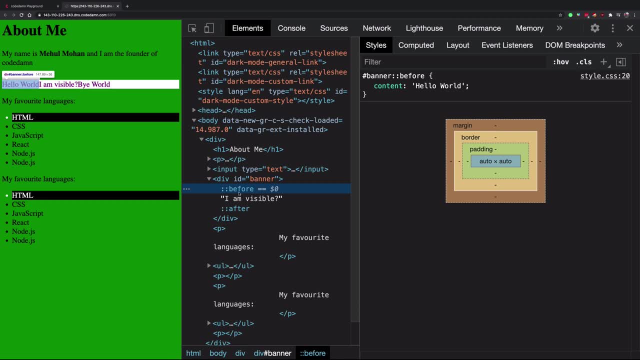 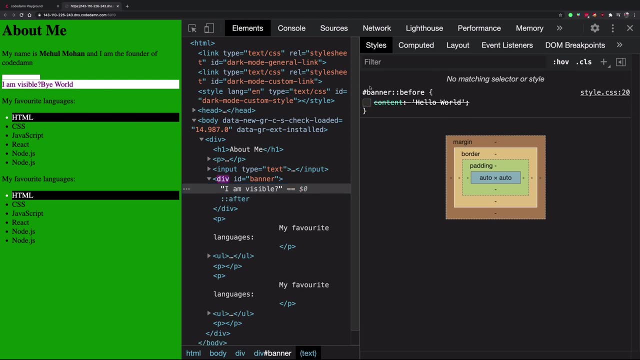 And these elements, interestingly enough, will only and only appear as long as you have the content property. If I remove this content property, you can see the element not only just goes away, but it is not only visible, it is not also visible on the screen. 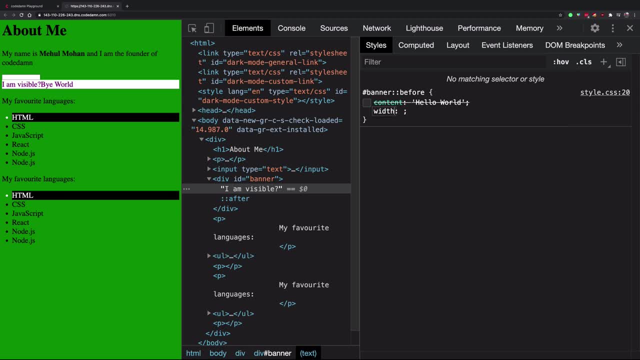 So I can go ahead and give it a width of 200 pixel, height of 200 pixel background- oops, height of 200 pixel background of red. Okay, it does not work, Let's just go ahead and do it here. 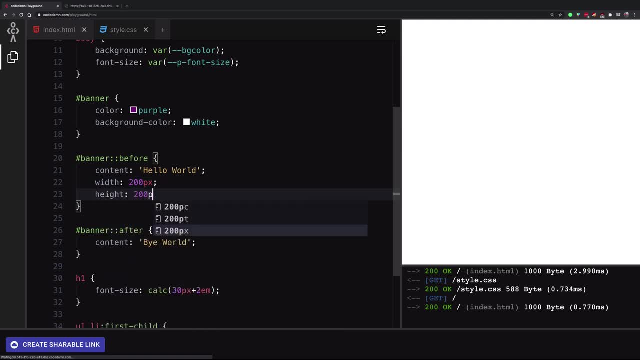 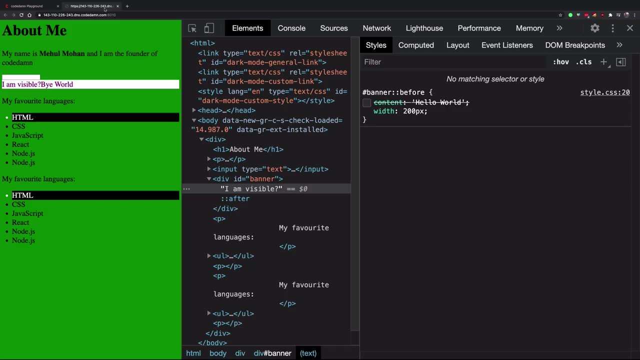 Width of 200 pixel. height of 200 pixel. background of red. You know I can do all that stuff, but it will not appear on the page, you know, if you do not give it a content right As soon as you remove that content. 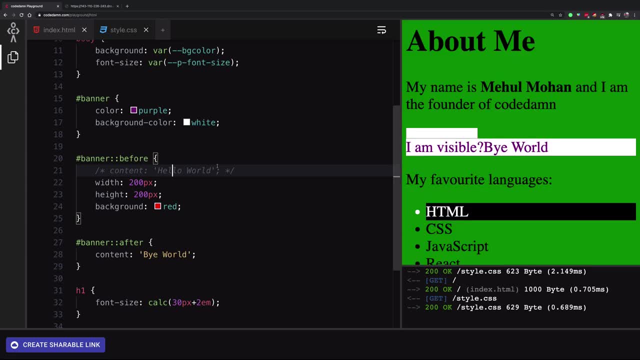 it disappears. If I remove this, it's gonna disappear, even if you give a display block right. Display block right here. It will not appear as long as you do not give it a content attribute, content property. So there's that right. 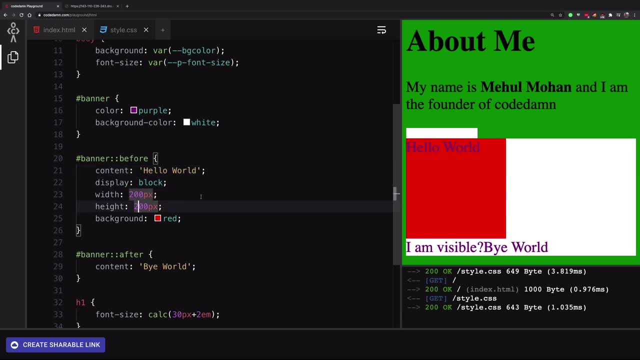 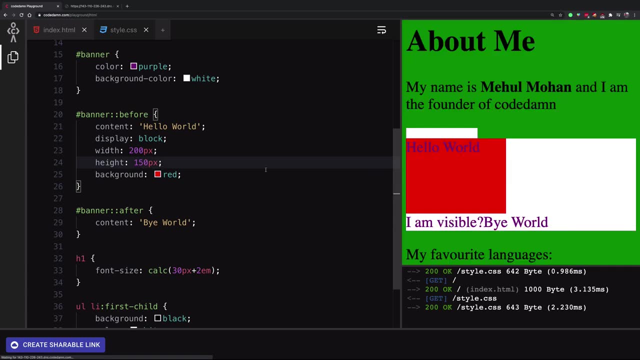 Now, once you have given it a display block, width and height, it sort of like behaves like a similar element. right, You can resize it, you can, you know, have fun with it, But obviously you know it's still not a part of DOM, right? 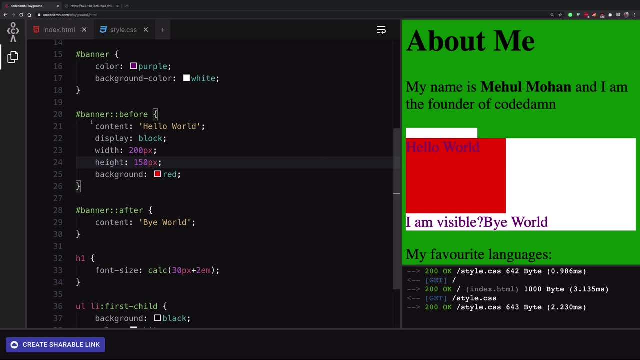 It's not a part of DOM. That means you cannot reach this element from the JavaScript world. This is an important thing. You cannot ever reach pseudo-selectors from JavaScript world, So that is like one thing to keep in mind, right. 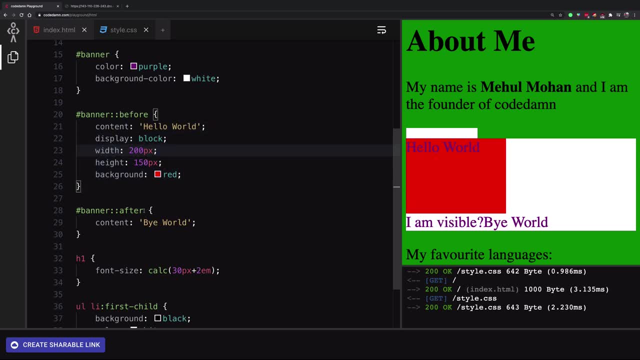 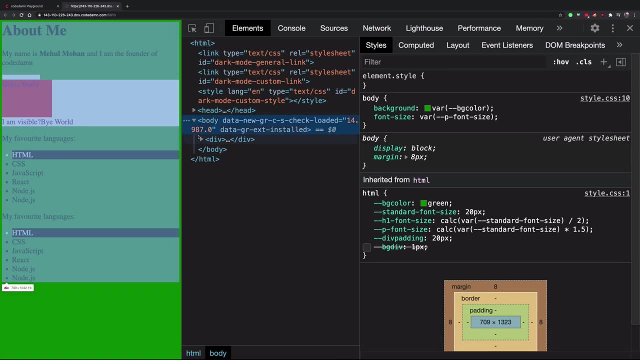 So this is like: before is a pseudo-selector, after is also a pseudo-selector which gets injected. just you know, if I refresh this page So you can see right here if I go ahead and target this hello world. 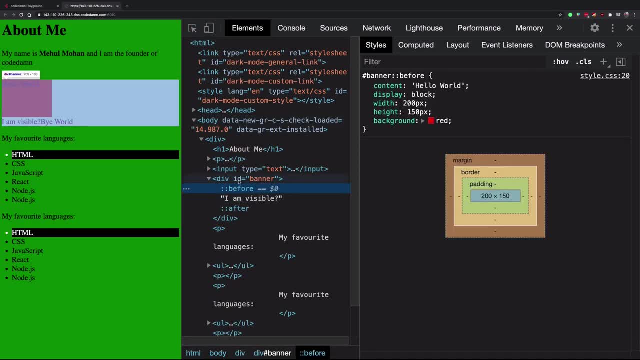 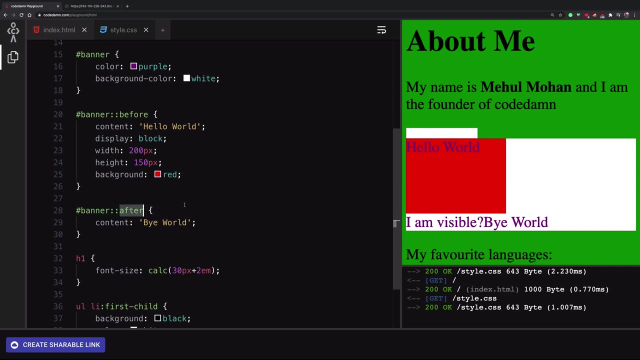 before gets injected: just as soon as we enter the element. and after gets injected, just before the element ends, Right? So there's that. There are multiple other, you know selectors which are pseudo-elements, right? Remember, these two columns means pseudo-elements. 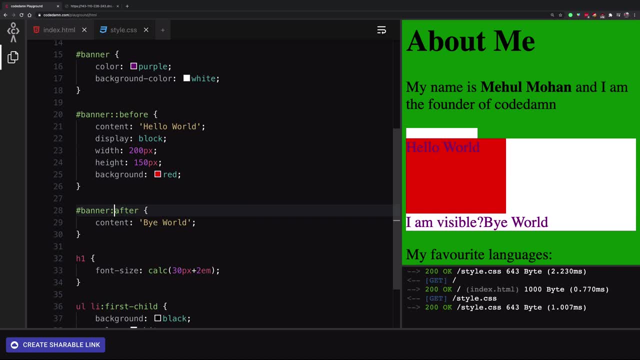 one column means pseudo-selector. These things still work because of compatibility reasons, you know, but you should always use double columns right here just to denote that, hey, that this is actually a pseudo-element, not a pseudo-selector. This is not a pseudo-selector, right. 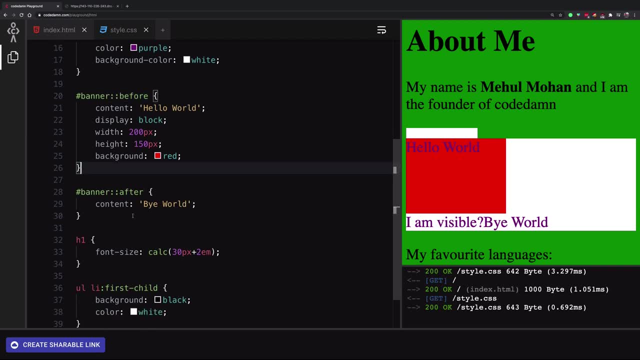 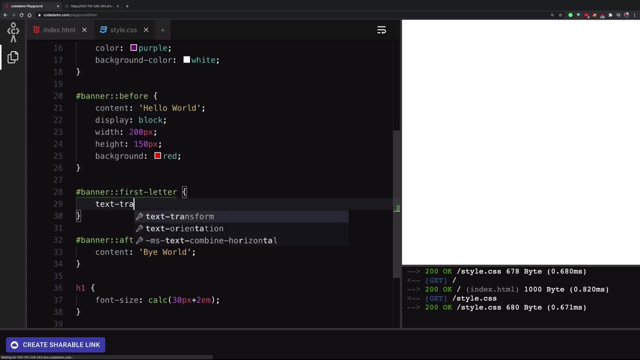 This is a pseudo-element you're targeting. Similarly, let's just go ahead and write banner and I'm gonna give this one a first letter right, Interestingly enough, and I'm gonna give this a text transform of lowercase. You can see that the hello worlds of 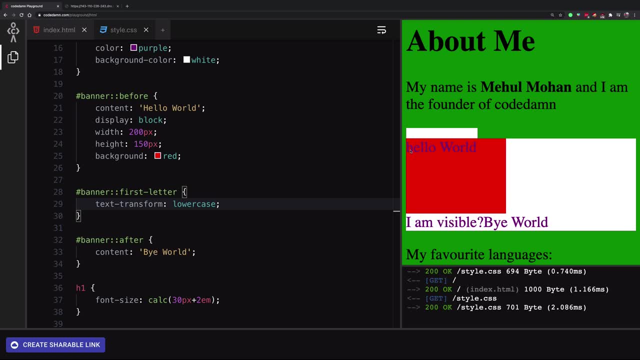 the edge of the hello world suddenly turned lowercase. Now, if I go ahead and give it a you know oops, if I go ahead and turn this all hello world so that it's much more clear, you can see that the edge is small. 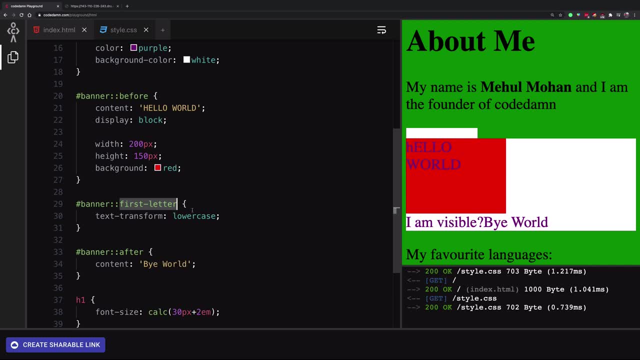 Why? Because I said the first letter of the element, the banner, should be lowercase right And I can also have a first line right here which is just gonna target the whole thing. If we did not have, like you know, 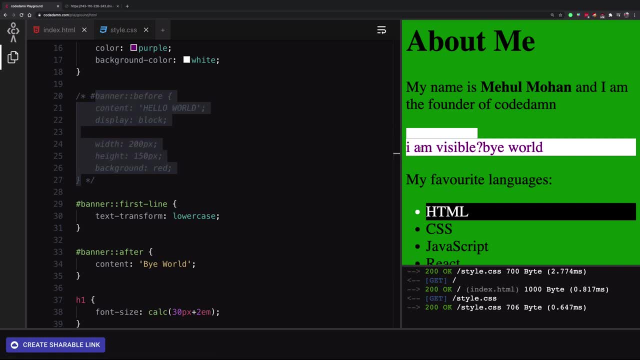 this before, then you're gonna see that it actually impacts the you know element itself. So there's that. So this is like. this is like how it works. There's one more interesting thing I would just like to discuss before we wrap up this video. 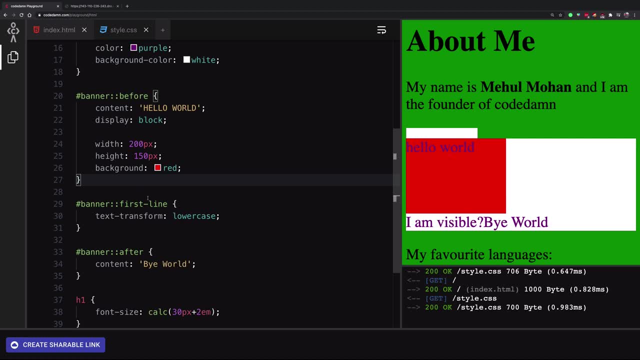 and that is, there is actually a way to add, you know, selectors on pseudo elements, And what do I mean by that? Let's see, Let's say, if you want to have a hover effect on the pseudo element, then what you might think. 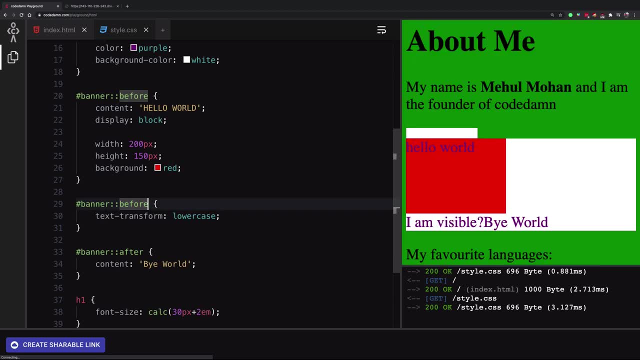 of doing is something like: hey, I have the banner before selector and when I hover over this, what should happen is that the text transform lowercase, which is fine, But if you check this out, it will not work. Why? Because you know. 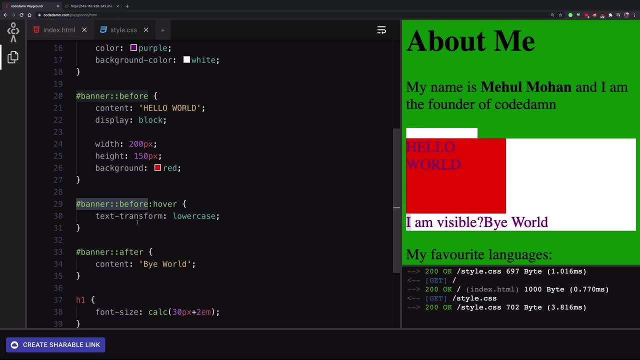 you're targeting an element which does not exist on the DOM tree. But what you can do is you can go ahead and hover. you can get the state first and then you can say, once I hover over this, the before state of this. 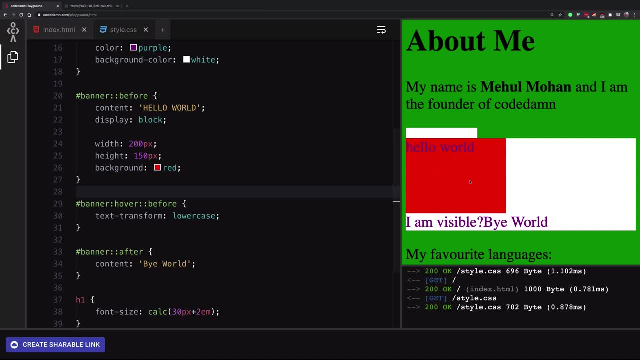 is gonna be you know lowercase And I know it sounds stupid that you know this one works, the other one does not work. But yeah, I mean, if you want to target pseudo selectors, just sort of like try to put the. 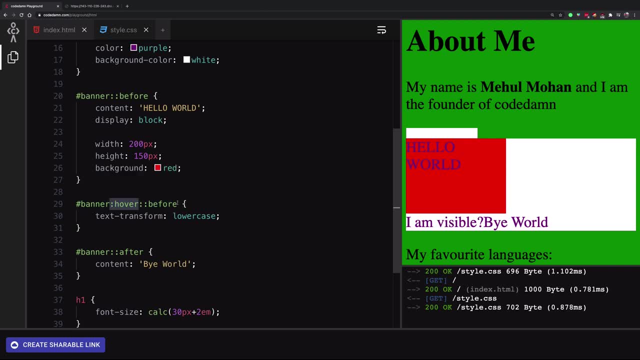 the pseudo. if you want to target the pseudo elements, try to put the pseudo selector before Right. So similarly, you can go ahead and let's see if we have- I don't know- banner hover, first letter as the pseudo selector. 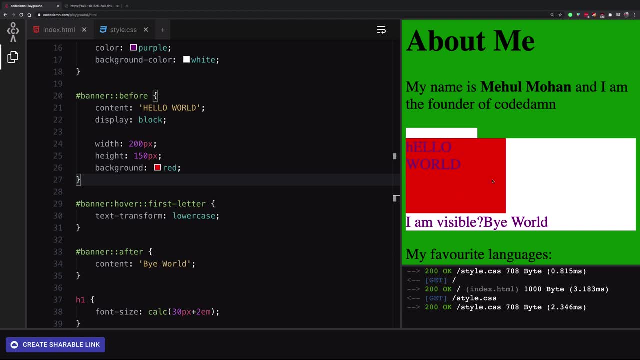 then also this will just work right. So no need of having any JavaScript or anything if you just want to have these simple effects. So this is how you know this. all sorts of works out. So so far you have seen that there are two sorts of selectors. 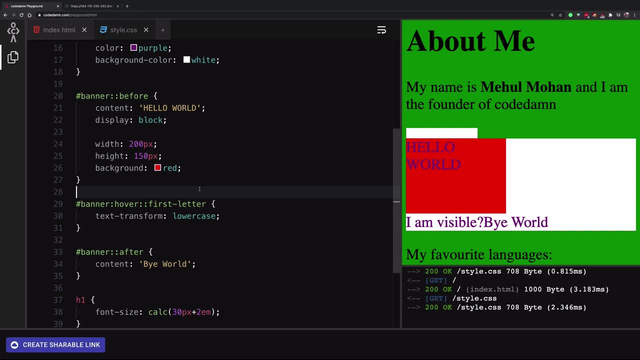 The first one is actually pseudo selectors. the second one is actually pseudo elements. Pseudo elements consist of: before, after first letter, first sentence, first line. actually not first letter, first sentence, But but yeah, there might be a couple more. 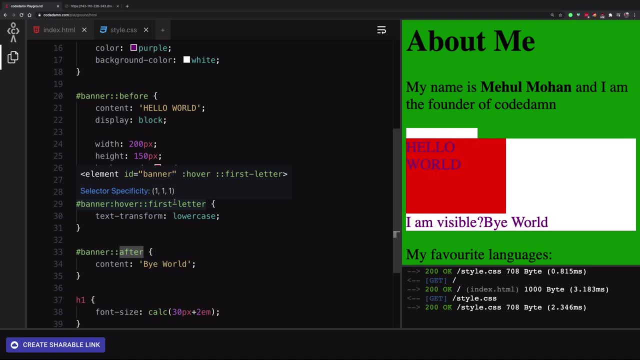 couple or so. but you know, you get the idea. That's how, that's how you use pseudo elements and pseudo selectors. So yeah, that's pretty much it for this video. In the next one I'm going to cover an ATTR attribute. 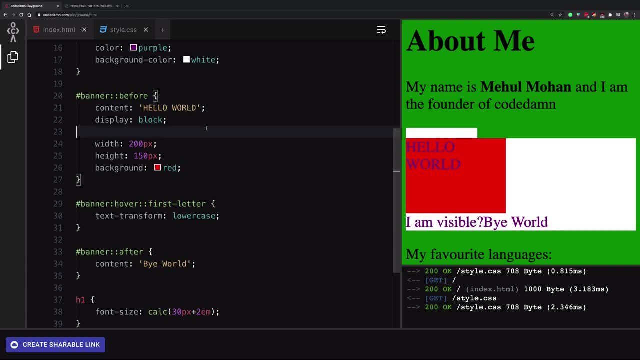 which is an interesting property, which sort of links your CSS with HTML world. So yeah, that's pretty much it for this video. I'm going to see you in the next one. Everyone, welcome back. In this video we're going to be taking a look at ATTR. 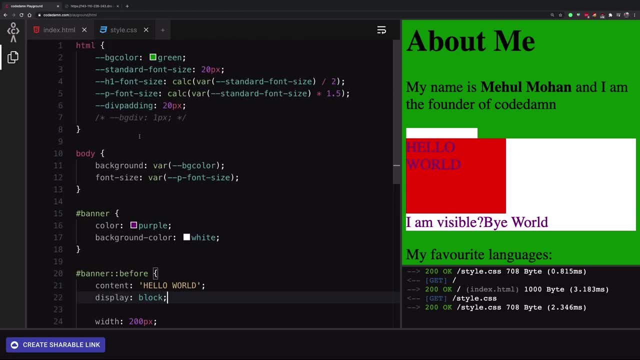 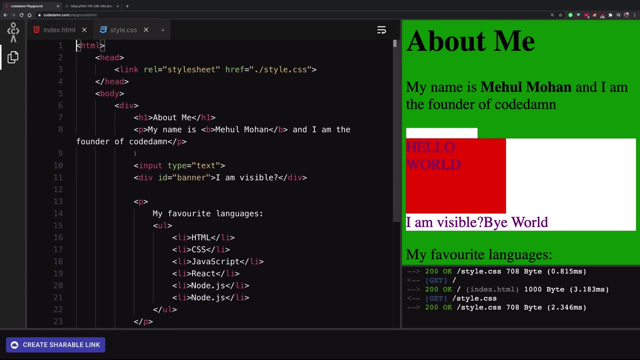 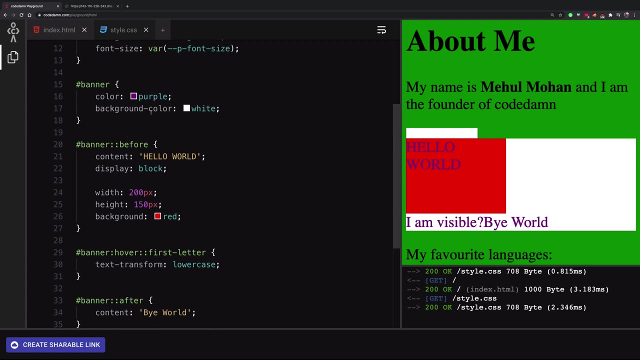 That is the attribute function in CSS. Yes, yet another function after war and calc, and you know that stuff. So let's just go ahead and take a look at what this ATTR means. So, first of all, realize that this content right here is actually a string. 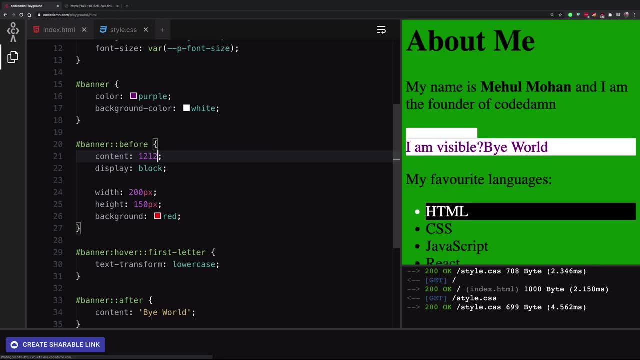 right, So that is pretty cool. You cannot have a number right here. It will not work. You have to have a string, irrespective of you know, even if that's a number. So content property right here always expects a arbitrary string. 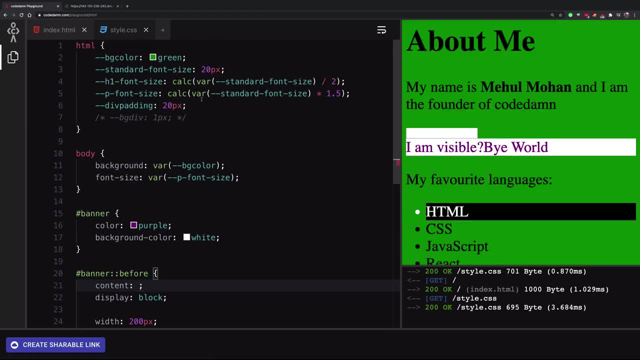 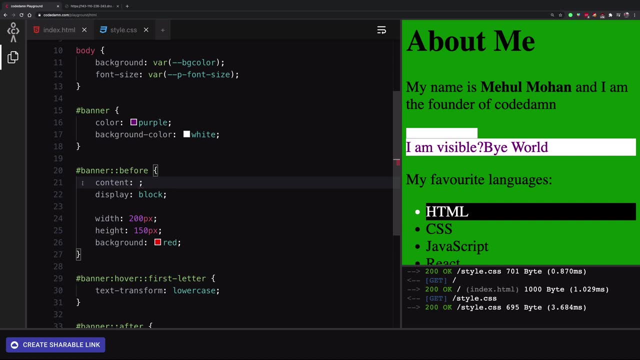 Number two is that sure, you can use variables here, That will just be fine, but you can actually use attributes from HTML element, the element which you're targeting directly. Now, what do we mean by that? You can go ahead and say ATTR, right here. 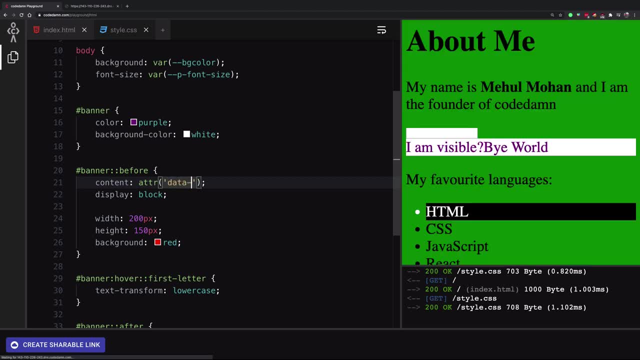 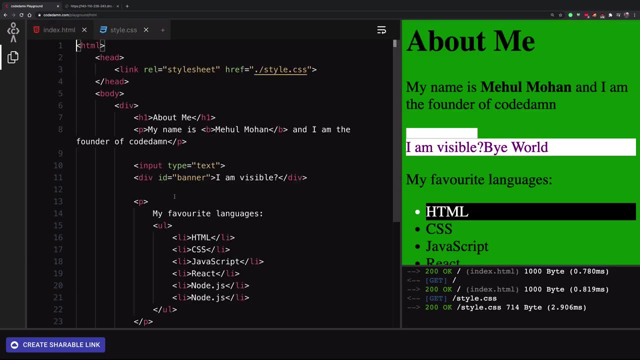 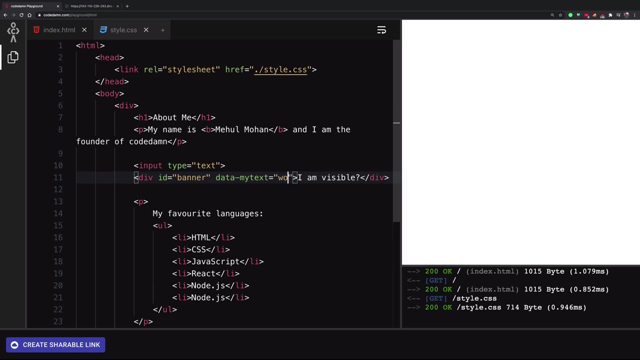 and you can say something like data my, my text, something like this. Now, what does this mean? is that if I go ahead and on the banner, if I create an attribute, data my text, and if I give it, wow, 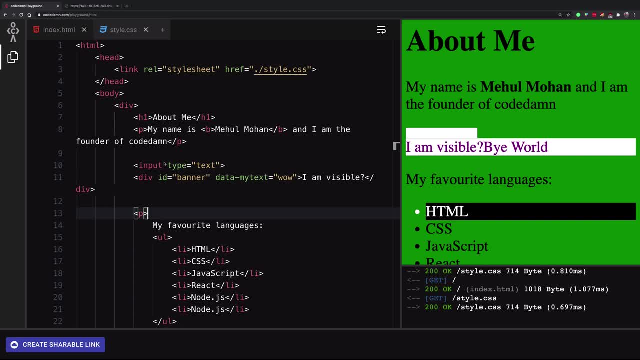 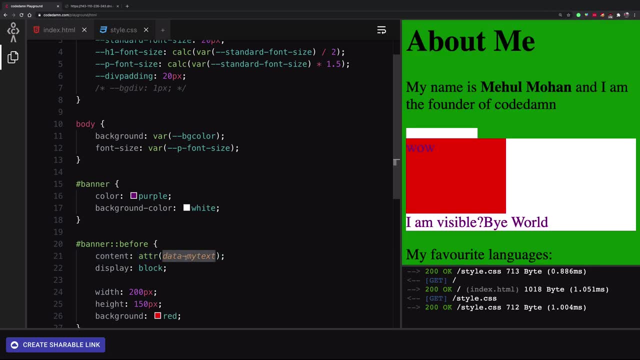 you're going to see and nothing appears, because this should not be in quotes. This attribute name should be in, you know, without quotes. So this right here you can see, gives you wow inside the red rectangle right. 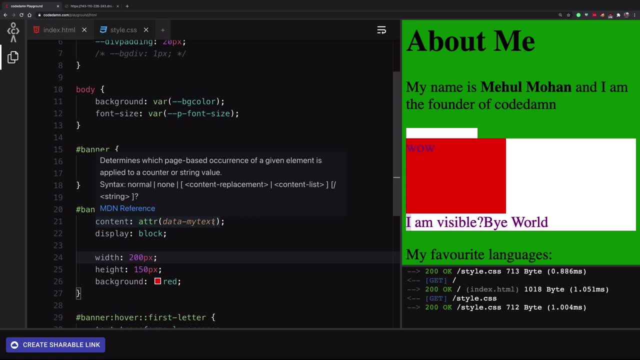 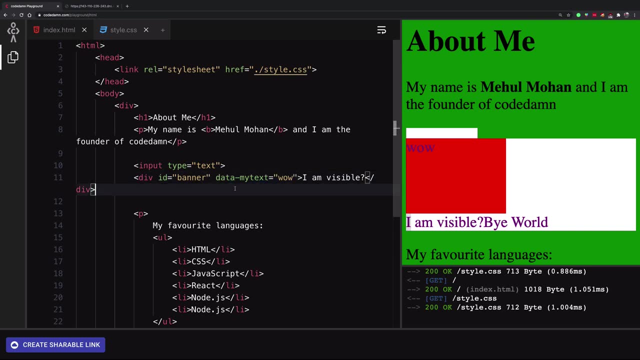 Because because of this thing. but what's the point to note here is that you have picked up the value of an attribute which should technically not be visible on the page, because you know you should know that data dash anything is like a wild card sort of given to you for putting in random amount of data in HTML. 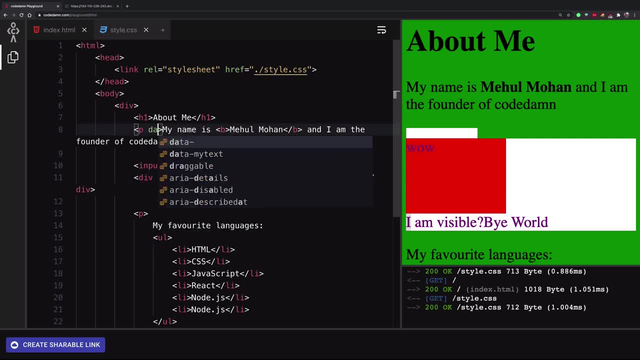 right. You can basically go ahead on any tag, put out data, something else and something value, and this will not reflect on the HTML page. It's sort of like a metadata placeholder for every single element, right? So you could pretty much put in anything right here. 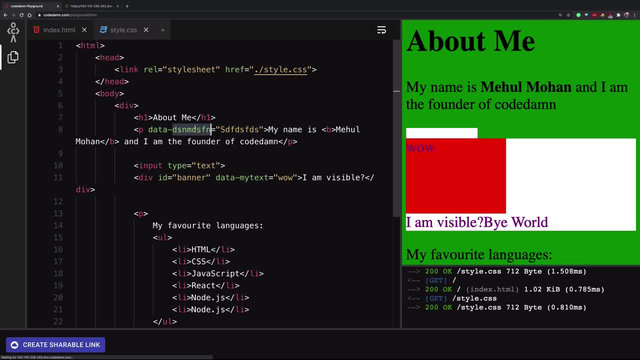 you know, given that it's a valid attribute name and he'll just work fine. But with CSS you can sort of extract up these values right here. And it's not just you know, it's not just data, My text. 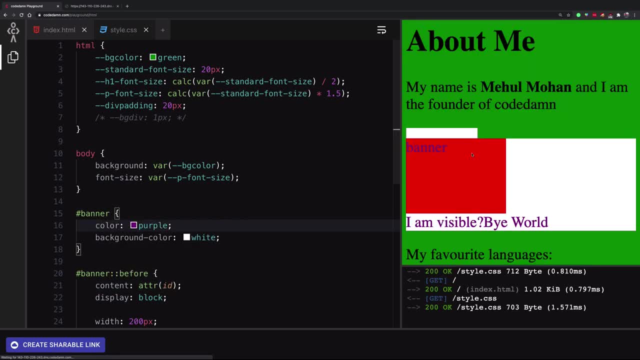 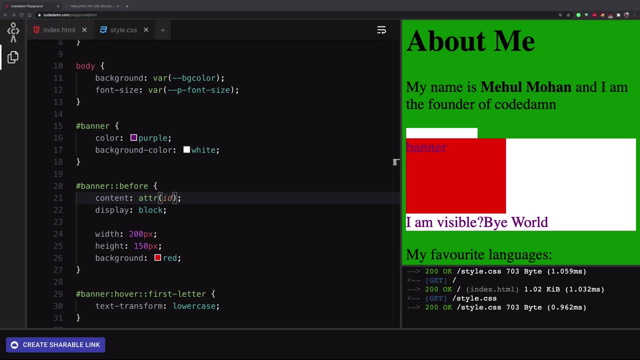 you can pretty much have an ID attribute right here which is just going to reflect the banner right, The ID of the element is banner. So the attribute function right here- you see, actually in CSS for would ideally support a fallback version, just like war supports. 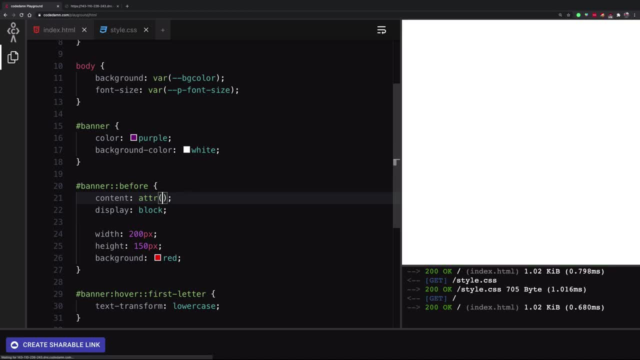 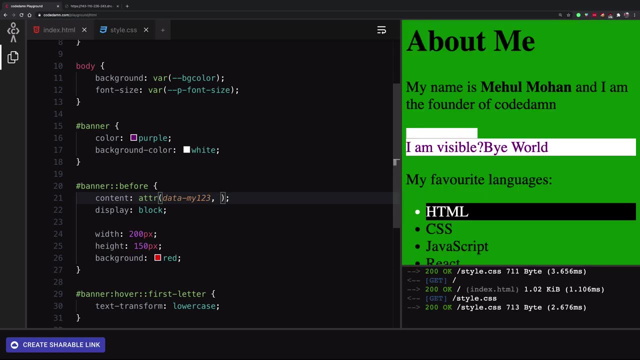 right. So if you have, you know, an attribute which does not exist, like data, my one, two, three or whatever, then if the value does not exist, you could technically go ahead and write Hey, here, and the value would appear. 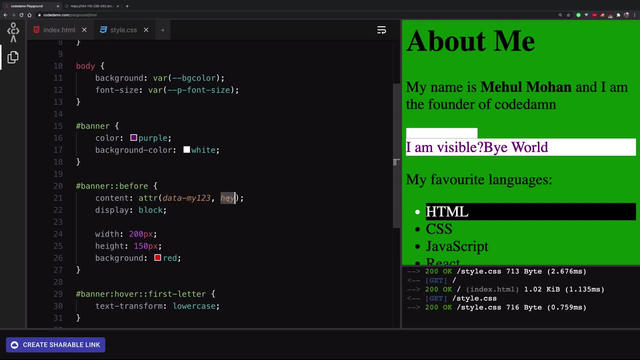 right. So this is a CSS for specification and it does not exist in CSS three. So there's that. But anyway, as of now, you can go ahead and plug in the attributes and we'll just work out of the box. So 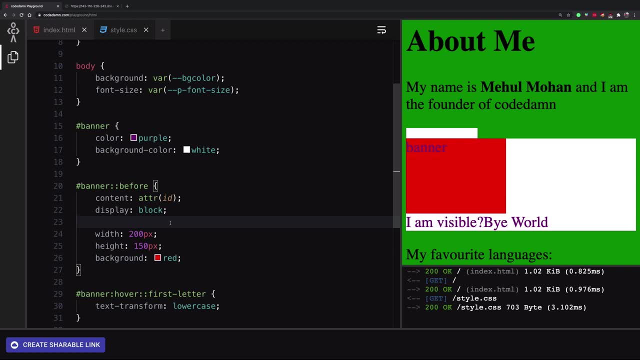 yeah, that's pretty much it for this video. Hope you enjoyed it. I'm going to see you in the next one really soon. Hey, everyone, welcome back. And then this video. I want to just go ahead and take a look at some advanced CSS selectors. 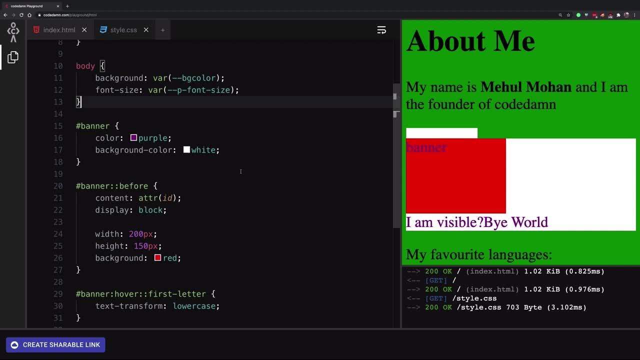 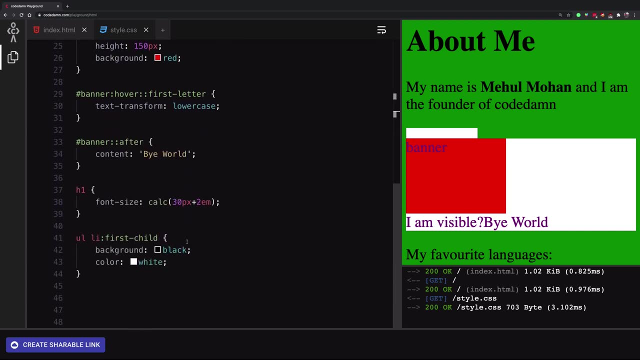 And we'll just go ahead and take a look at all CSS selectors, as a matter of fact, which are most common, And as well as covered the advanced ones, because I think I did not cover it very well in the basics course. So anyway, 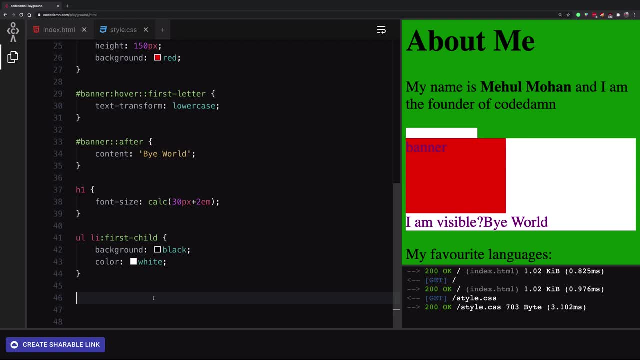 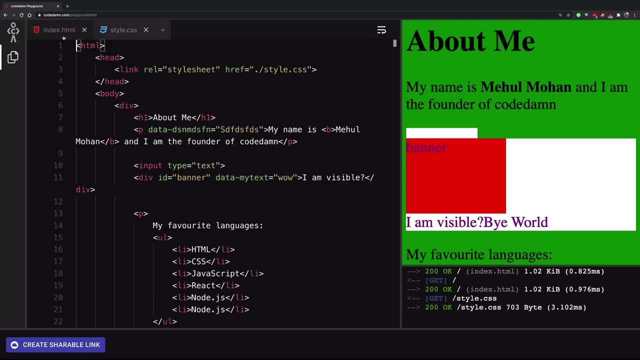 let's just go ahead and start with the advanced ones And we can just cover out the late, the basics one, later on as well. So I'm going to start off with the sibling selector only, right, Something which we discussed, So you can see right here. 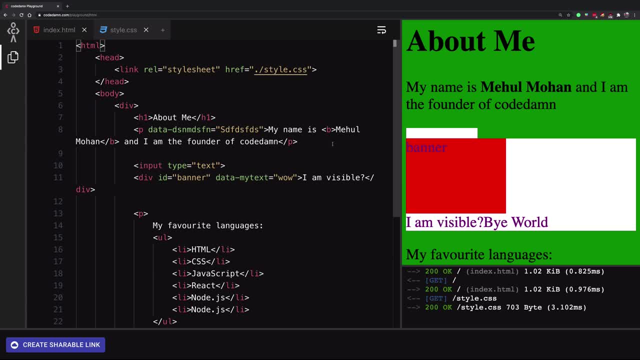 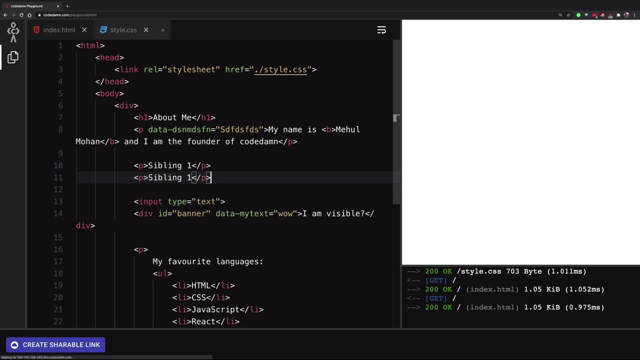 if you want to target immediate siblings, what we can go ahead and do is: I can just go ahead and create two siblings here: Sibling one. let's go ahead and create three instead. Sibling one, sibling two, sibling three- right. 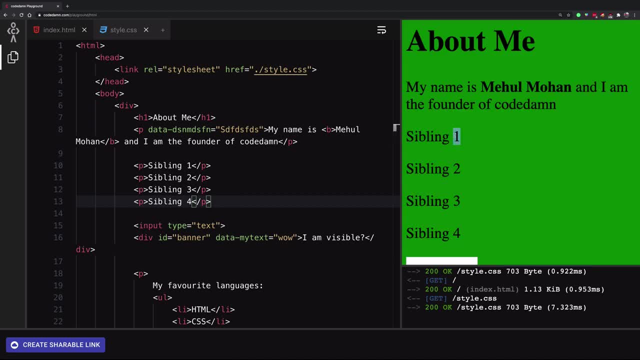 Or maybe like why not four Anyway? so you can see, right here we have four P tags which are siblings. And what do you mean by sibling? That means they are the same order in the hierarchy, right In this case. 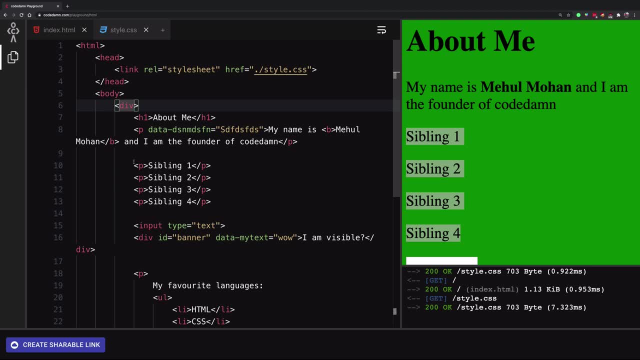 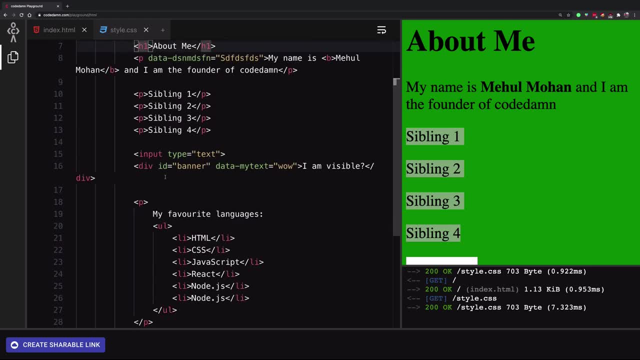 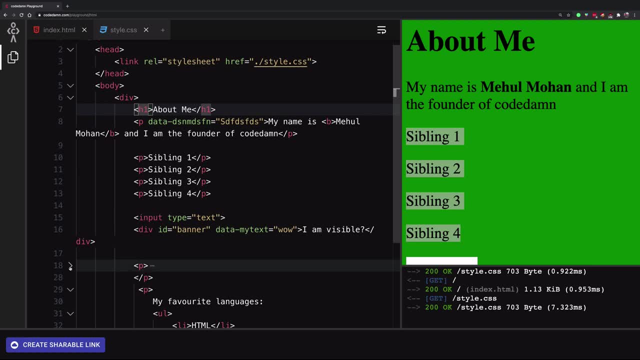 but there's that. But anyway, you can think of this P right here, all these P's to be siblings of H1. And similarly each and everything. So for now, we're just going to keep our focus on these four. 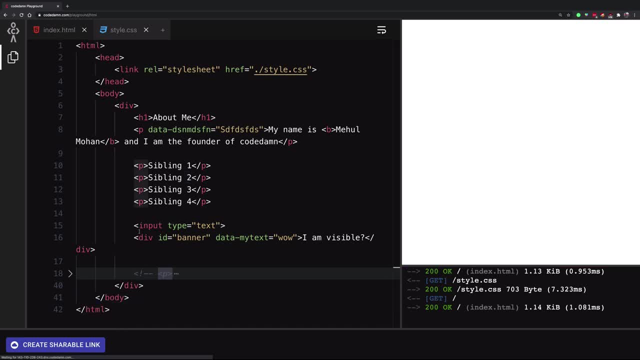 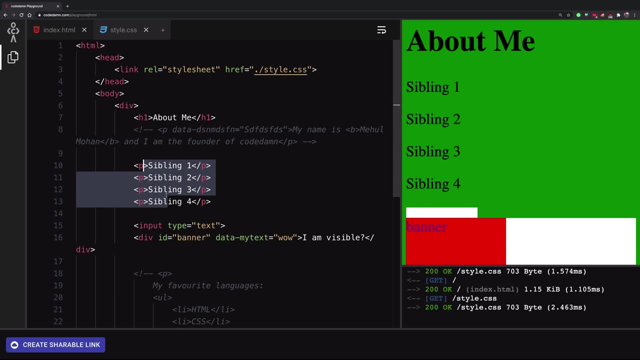 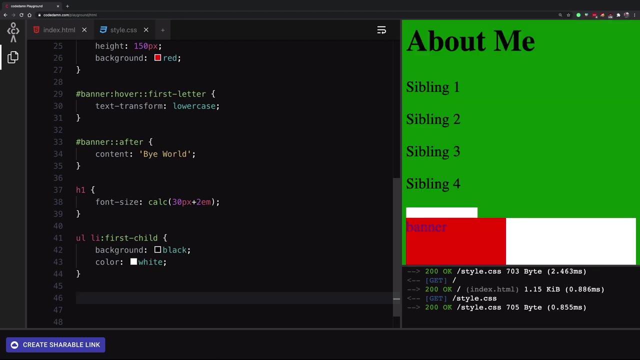 right, We're going to move or probably like comment out these guys right, So that they don't really bug us. So I'm going to also comment out this one. So we just have you know P tags as siblings. So what you can do is you can go ahead and select siblings using immediate siblings. 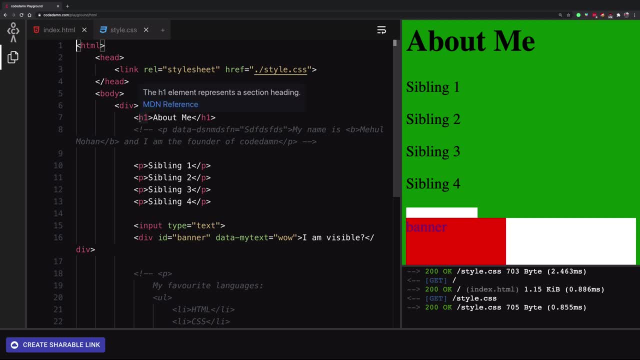 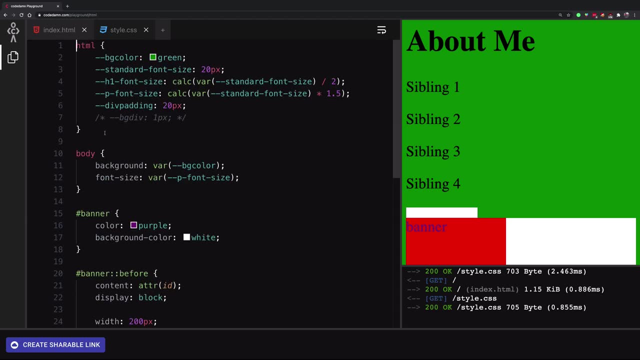 using the plus symbol. What this means is that, Hey, let's say, if I want to select the immediate sibling of this H1, which is P, what I can do is I can go ahead and say H1 plus P is color as blue, or background color as blue, or whatever. 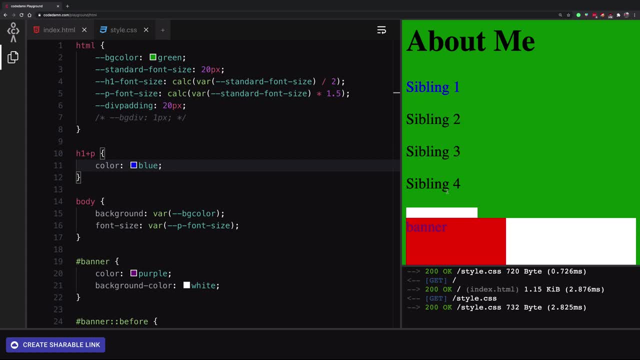 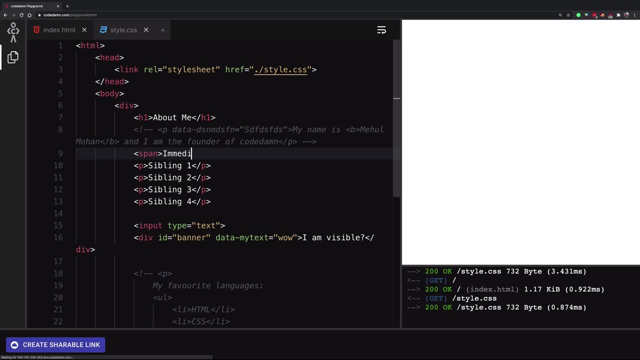 I can see this: one turns blue but the others do not. Why? Because this plus right here denotes the immediate sibling, right. That means this P should be the immediate sibling. However, if we have another span, let's say as an immediate sibling. 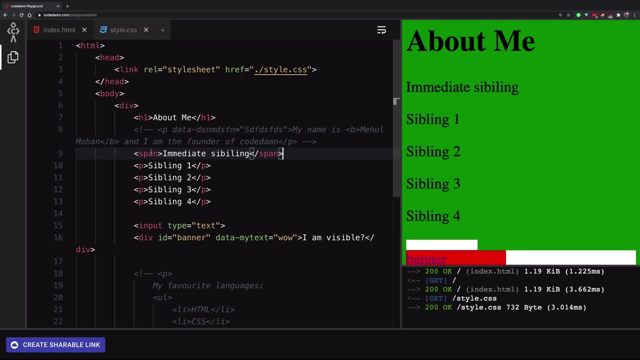 then that span would not get any style. Why? Because, first of all, that is not a P tag And this P will also not get any style, which it got earlier. Why? Because this is not an immediate sibling. However, if I move this at one place up, 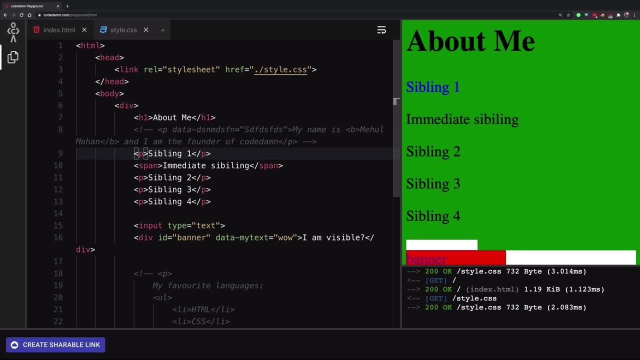 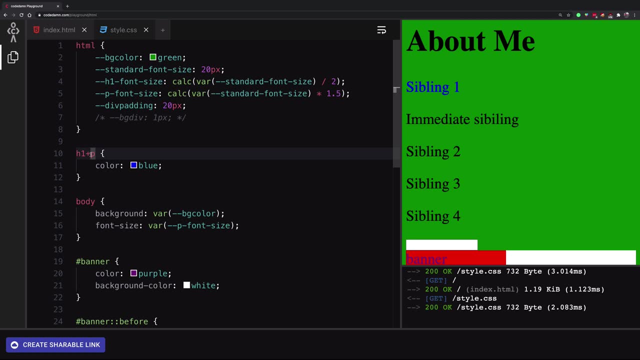 you know, things get blue again. So there's that. Now there is another sort of way to select sibling, And that is you know far away siblings and you know sort of like all siblings as well, And that is with the tilde sign. 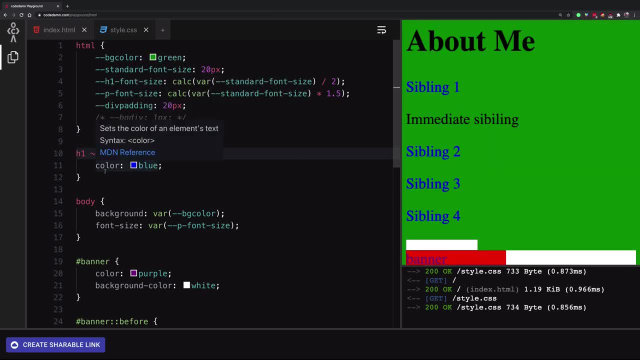 right, Which is above, which is on the left of the one key. So once you do this, this means that, okay, I want to select all the P's which are siblings of each one. Does not matter if they are immediate. 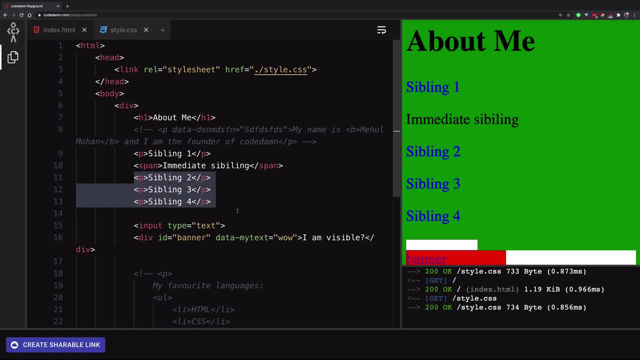 you know, in this case this one, or does not matter. if they are far enough, It'll just go ahead and select all the siblings, right? But remember, obviously remember, that is it's not selecting any children or parent or any sort of thing. 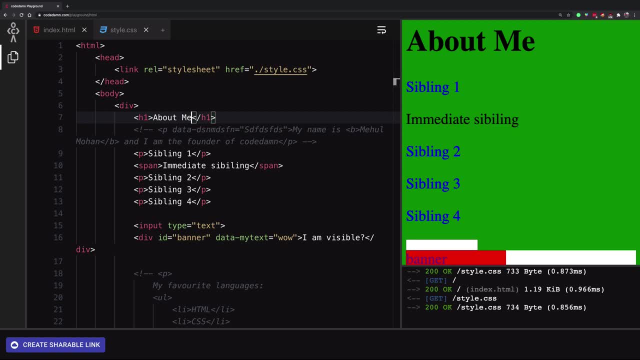 It's just the sibling stuff. So this is how you work with siblings in CSS. Just to revise: plus is, for you know, selecting the immediate sibling, and the tilde sign is for selecting far away siblings as well. Now the next one is the direct child of the element. 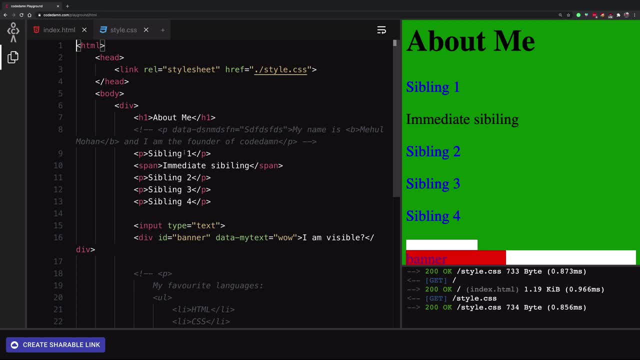 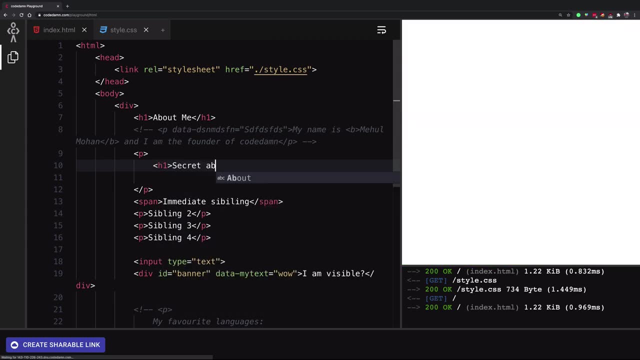 Now, what does this mean? Let's say, if I have a P tag with a sibling, or maybe like, like. let's say, if I have an H one right here, which is a secret about me. So if you have something like this, 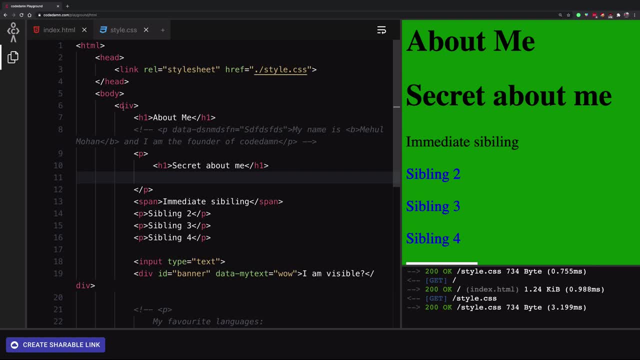 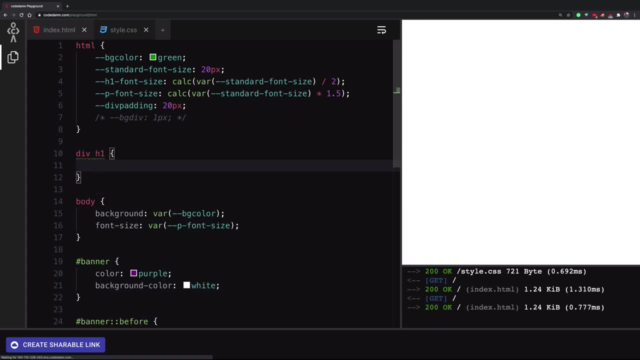 what we can do is I have this div tag and this H one, right? So I'm going to go ahead and get rid of this and I'm going to write div H one and I'm going to say text decoration underline, right, Which is just going to underline this text. 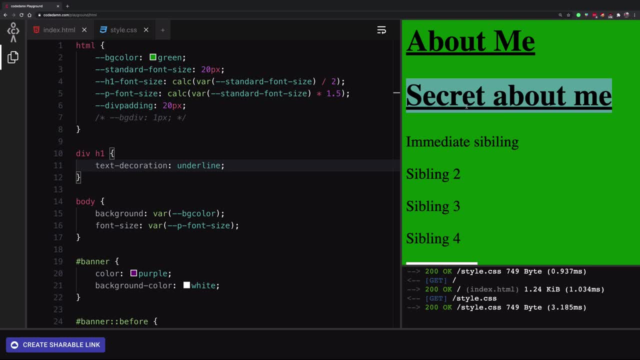 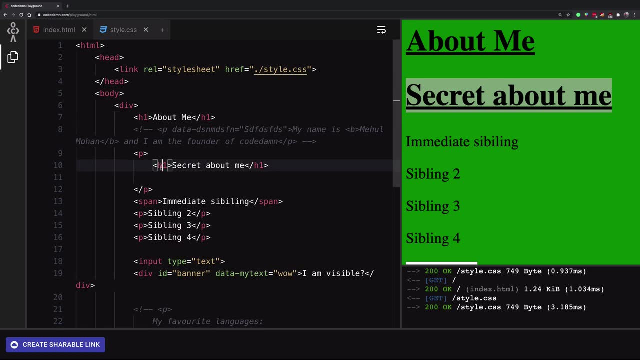 So you see, in this case both about me and secret about me gets underlined. Why? Because, well, this div and H one targets both of these tags, this one as well as this one. But what if I only want to target elements? 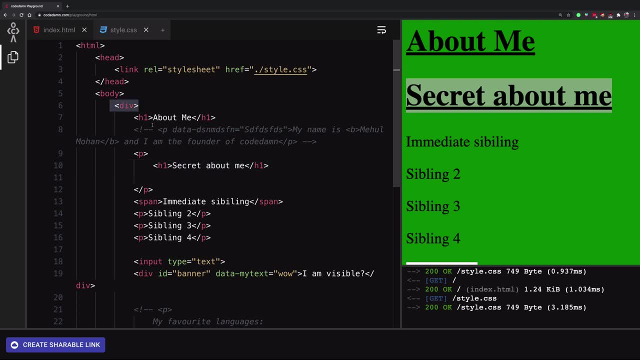 which are direct children of div, Now realize that in this case the parent of this H one is div. but the parent of this H one is not div. Div is the grandparent of this H one. The parent of this H one is this P tag. 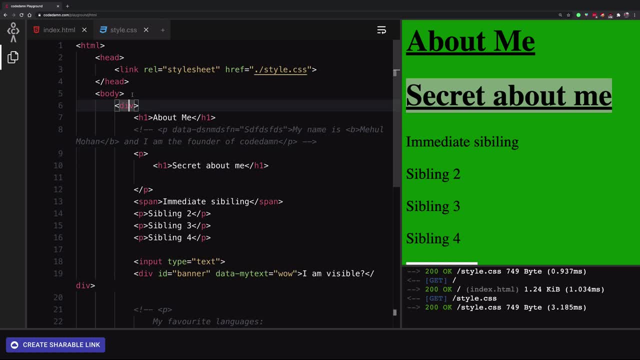 right. So if this div, which is like the sort of grandparent of this H one, if this div only wants to target its children, but not any other hierarchy down the line, then you can go ahead and use uh sort of 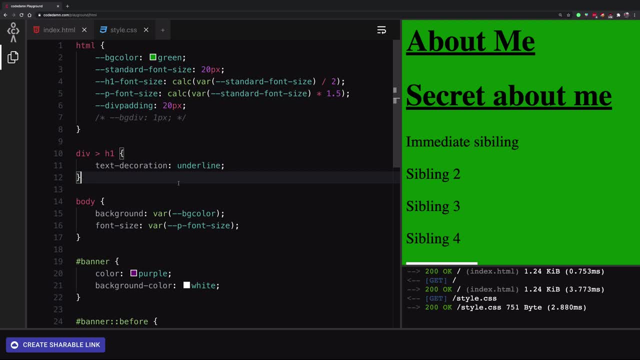 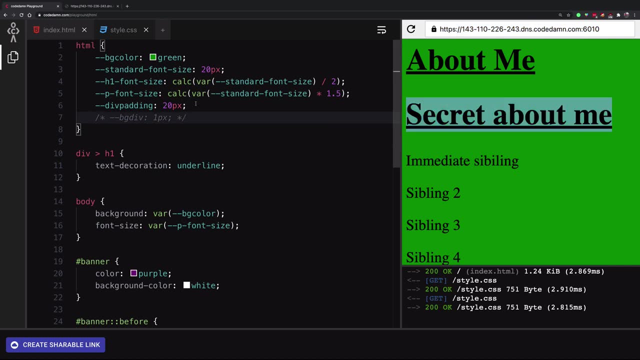 you know this, this bracket, right Angular bracket- And once you do this, what's going to happen? And it looks like we okay, And it looks like the thing is broken, or you know, it seems like the thing is not working. 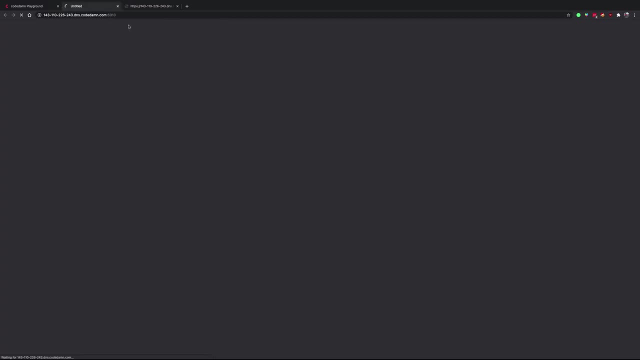 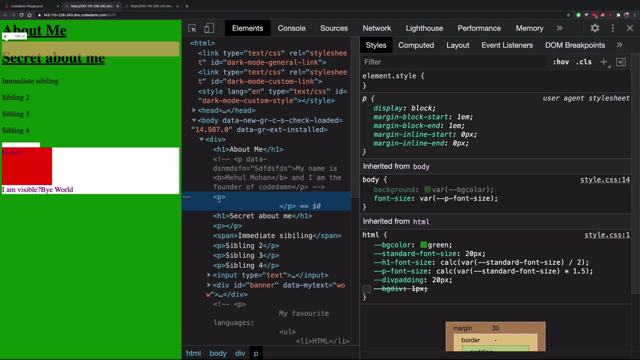 And the reason for this I'll tell you. if you go ahead and visit this page right here, if you go to inspect, you're going to see that the Dom which is computed by the browser is sort of different. That P has thrown away the H one. 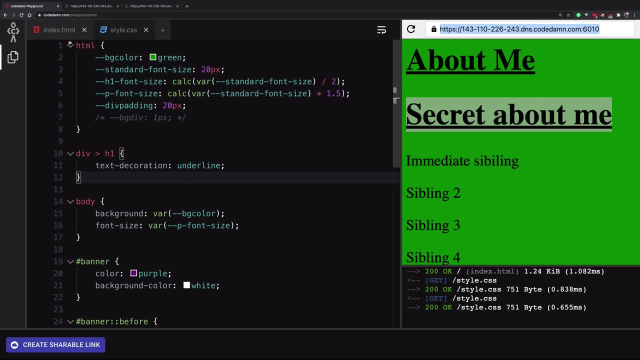 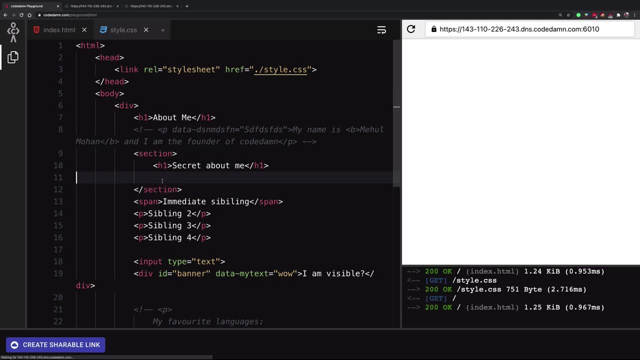 And the reason for this is because, by semantics, P is not allowed to contain an H one tag. So instead of P, let's just go ahead and throw a section here, right? So if we have a section now, you can see that our style just works fine, as expected. 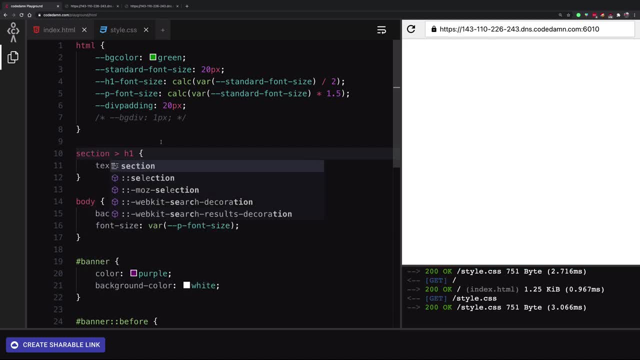 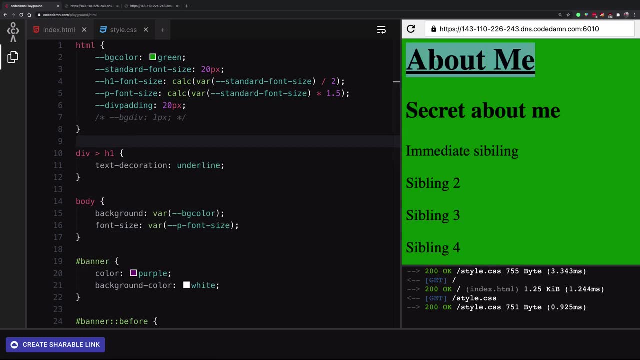 right. Similarly, if you have a section H, one like this, then only this one gets covered. on this one, obviously, but in this case, uh, only this one gets covered. However, if you just go ahead and just to reiterate, 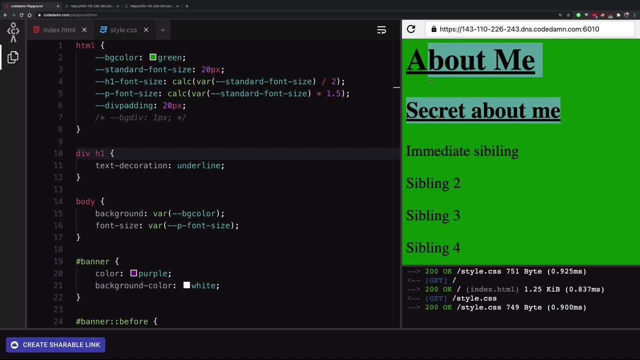 if you go ahead and just do div H one, then both of them will be covered to any depth or any hierarchy. So there's that. that is sort of like another selector you can think of Um. the next one, I would say, are pretty much the general selectors. 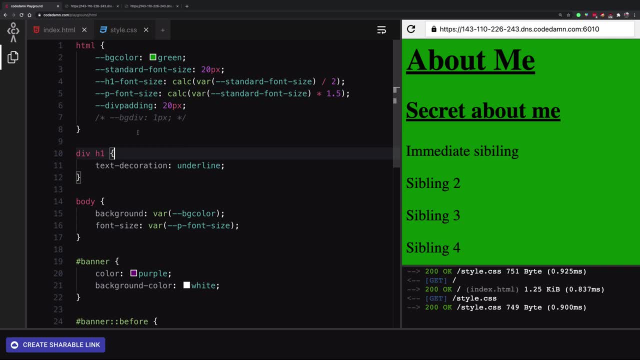 which you have worked on. There's another one I could just- probably just you know- throw it out there for you, And that is the star selector. The star selector basically matches every single element, right, If you use it on a. 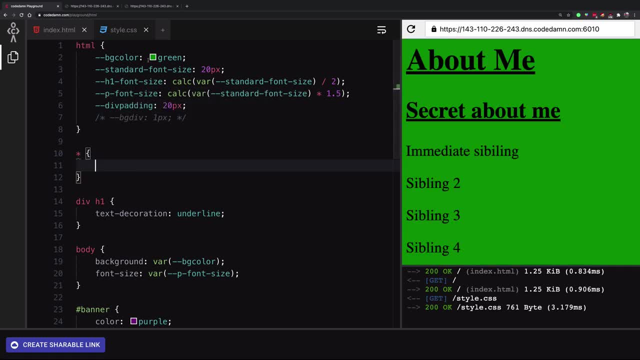 on a you know scope. this literally means like every single element on your page. So if I go ahead and give it a color of white and if I disclose it like this, I think I did not discuss important right on the CSS specificity video. 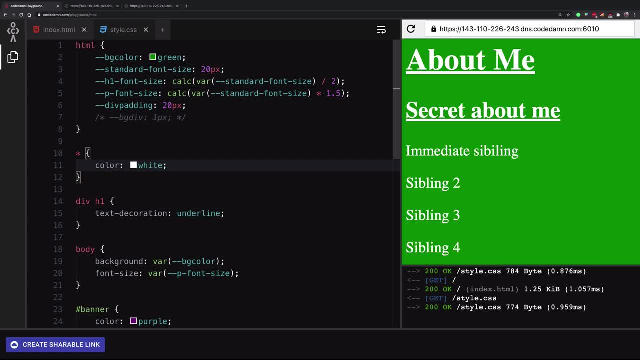 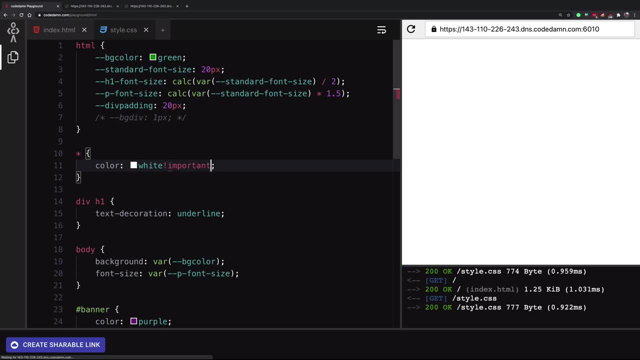 but yeah, let's just go ahead and make another one for that. But anyway, color white. right here you can see every single element turned white. right, If you just force, give it a color you know with important, that will actually turn every literally everything. 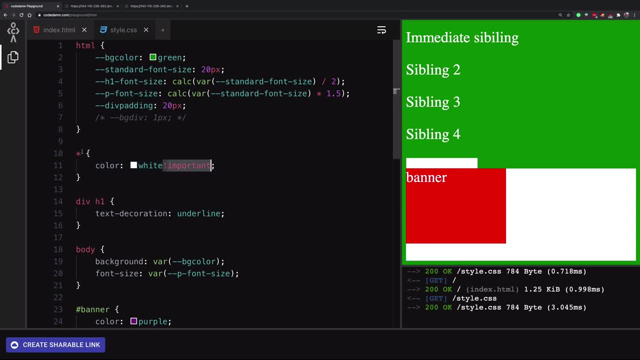 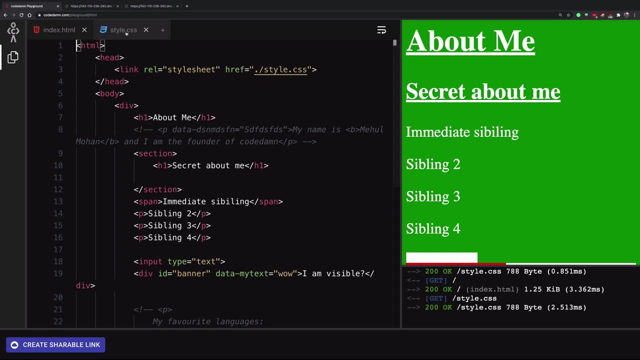 even the pseudo elements and all that stuff. So this is that if you want to only div, div to only convert, so you can do pretty much not really div, because that is like the main child. If you want to have like section, for example, 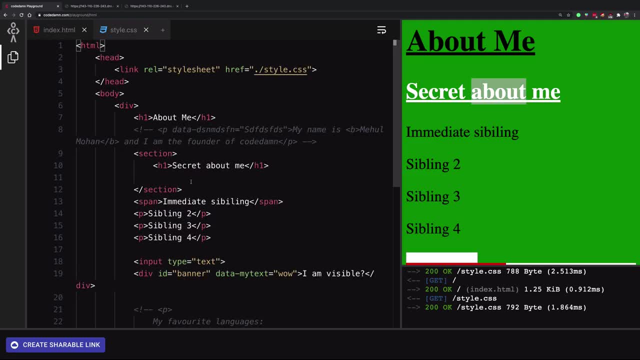 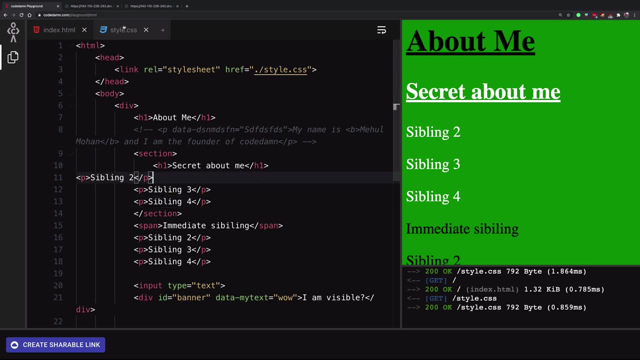 so there's that. you can see the H one gets converted. If it had contained, like you know, some more stuff, it will also get converted right. So the difference between just doing section of color white and section star of color white is important. 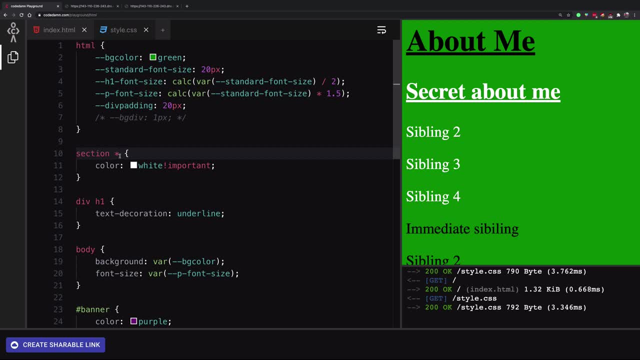 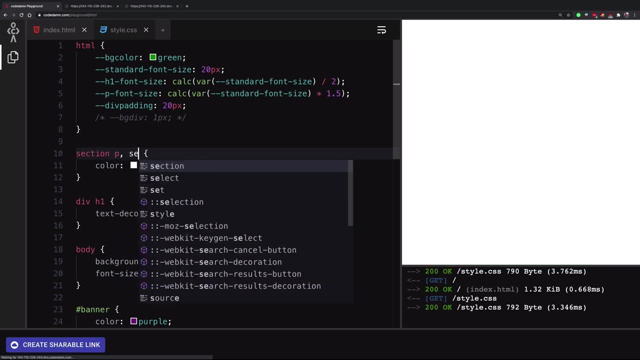 right And it is important to understand as well. Right here, what's happening is that you are selecting individual elements, as if you are writing section P, section H, one and you know just all the elements all the way. However, if you 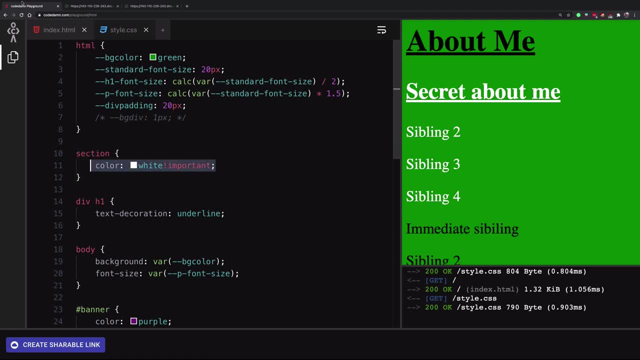 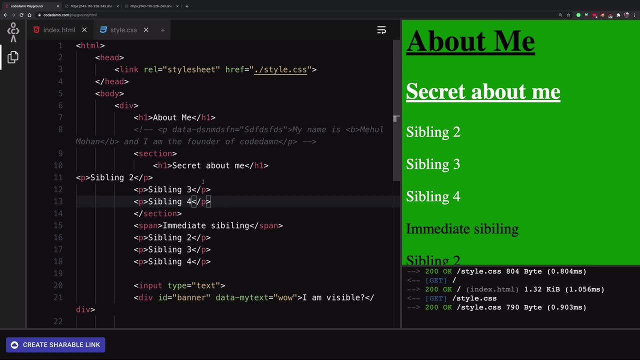 when you do section, what happens is that this property right here is applied to this element and the elements always have a tendency to borrow certain properties from parents, like color, font size, all that stuff, if that is not explicitly set right. 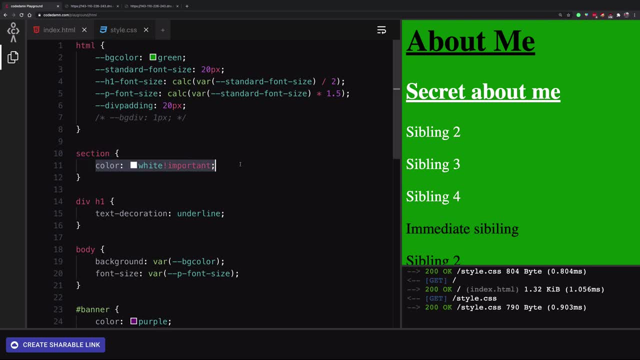 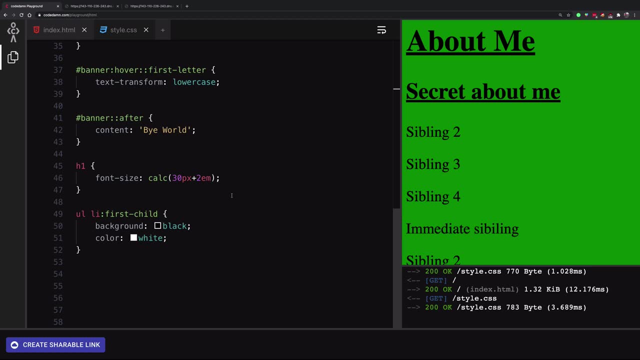 So let me just show you a quick example of this. If I have a section, I have a font size of, let's say, 30 pixel, then you're going to see that nothing changes. I guess, Nope. Anyway, you're going to see that nothing really happens because they already have their own defined font sizes. 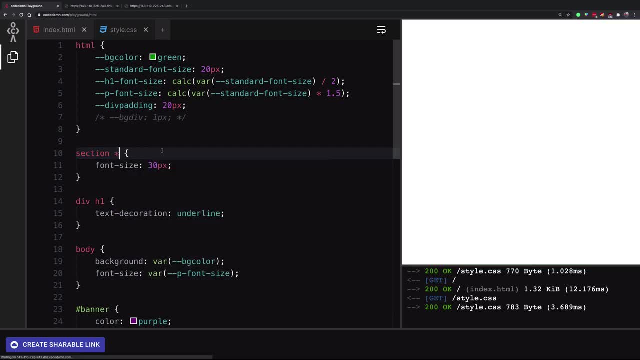 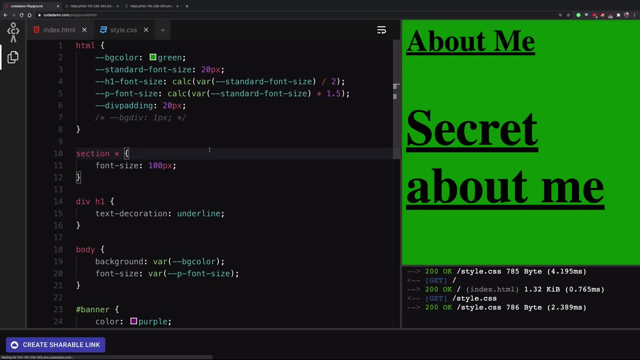 right, So they do not need to borrow from parent. However, if you do section start, you're going to see that everything becomes 30 pixels, Or let me just go ahead and make it 100 pixels. It's crazy big. So that's how we can see it. 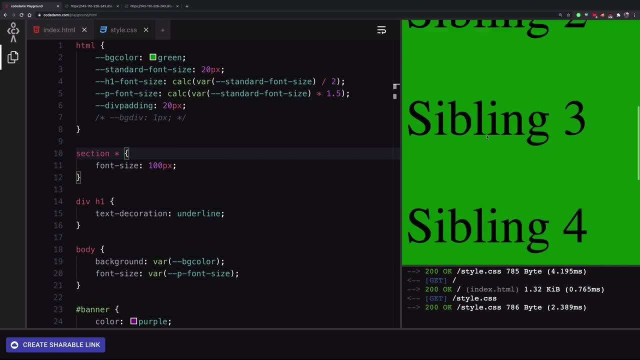 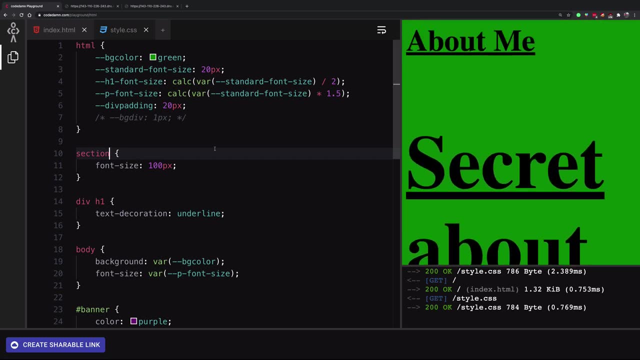 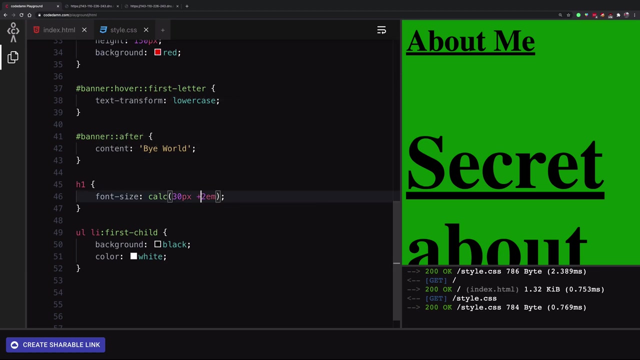 right. So now we have seen everything becomes 100 pixel, But with section alone. you know, things become 100 pixel, But if I go ahead and okay, well, that happens because we do not have a font size specified for each one. 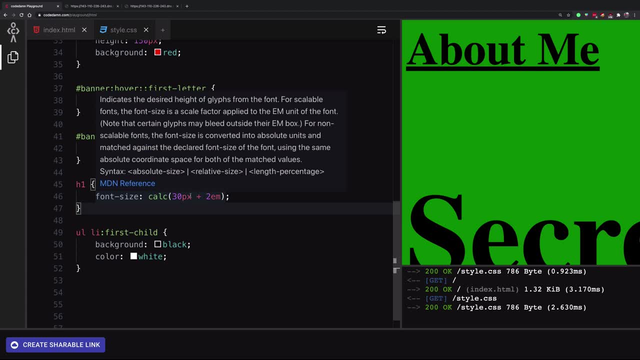 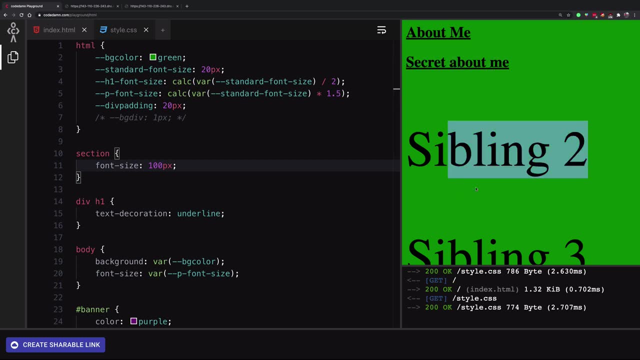 That was a wrong size. So you can see now if I have a, let's say, font size of 30 pixels for each one, you can see the H1, does not inherit the font size but the P tags do, because 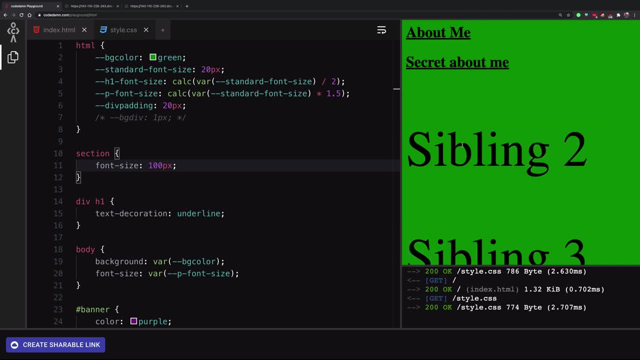 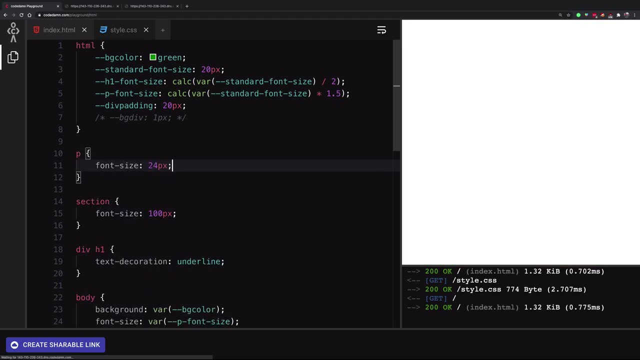 you know they are actually not having any font size, But if you go ahead and if you give a P of font size of 24 pixels as well, then you're going to see nobody inherits. However, now, if you give a section start, 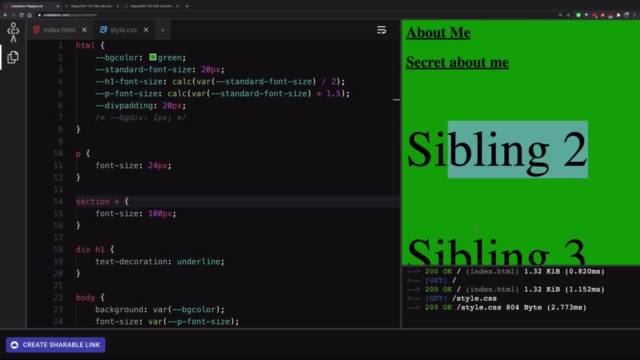 people start inheriting because you know this. this means literally every single element, And the reason this is this is not inheriting- is because of the specification. Now, if you go ahead and refresh this, you're going to see on here. 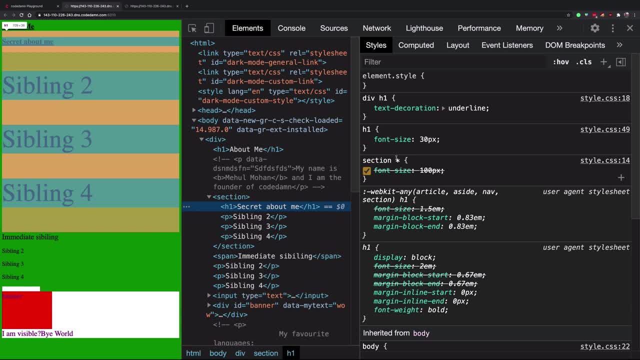 you're going to see, the start has a very low specificity right, And that gets canceled out. However, if you remove this, then you're going to see that it actually inherits, But anyway, that's. that's like the crux of it. 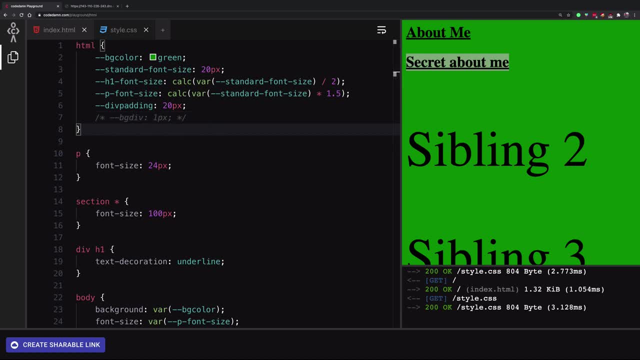 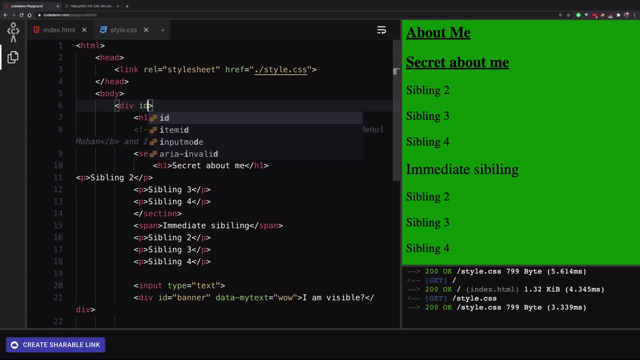 So yeah, that is again a start- is a special selector. Then, apart from this, we have IDs. I hope you all know about this ID. for example, all I can give this a div ID, all We then target this particular element. 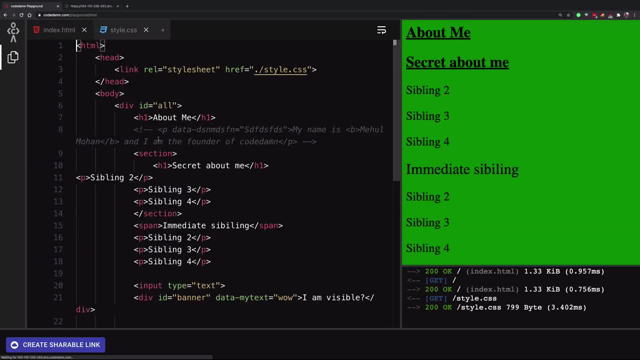 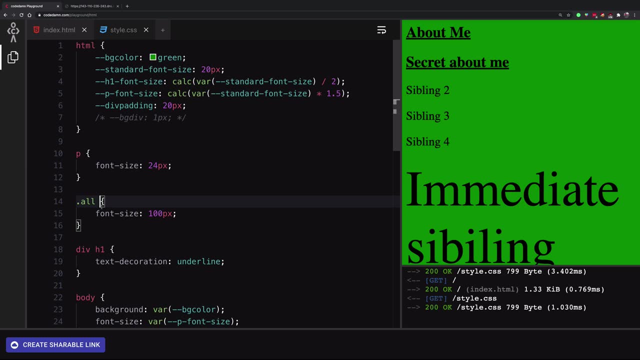 right Like this. We also have classes dot all. You can give it a class of all, and that is one and the same thing. The only difference between IDs and classes is that ID should be unique on a single page, whereas class could repeat. 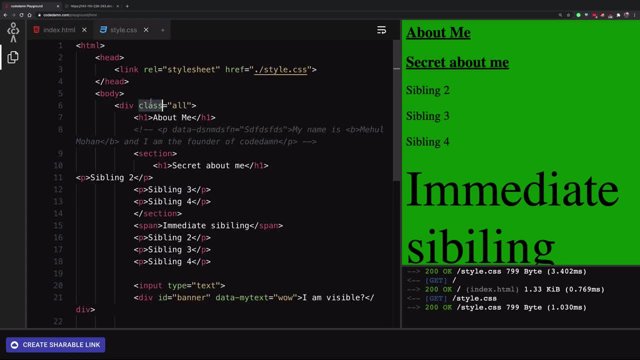 right, So you can make use of this class for some other div as well, But if you have given an ID of all, then well, technically, nobody's stopping you to reuse this. but you should never, ever reuse this, because it will create a ton of headache for you. 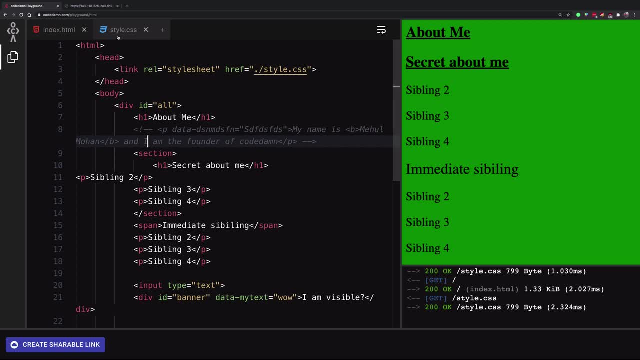 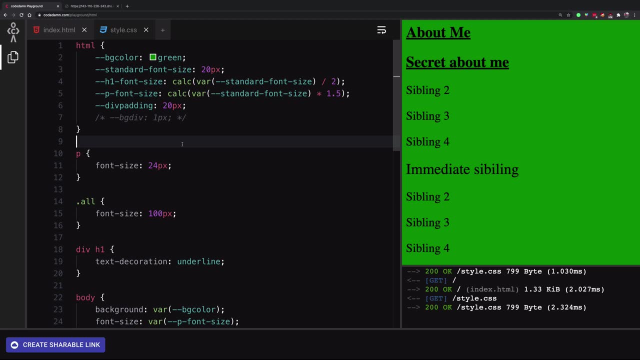 if you do So. yeah, that's pretty much it for the CSS selectors video. Hope you enjoyed it. That is all for this video and I'm going to see you in the next one. Hey, everyone, welcome back And in this video. 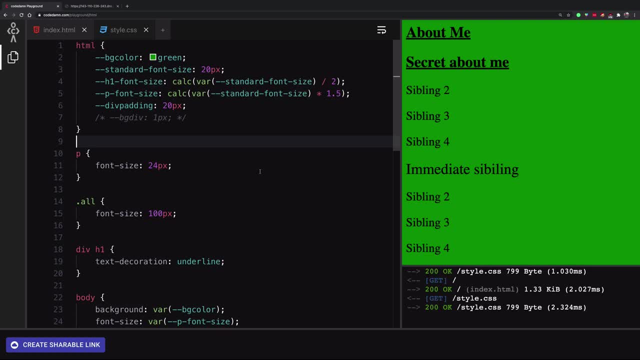 we're going to be taking a look at attribute CSS selector, And the reason I wanted to do a separate video for this is because attribute CSS selector can have a sort of a- you know a detailed explanation. And why? Because it consists of a lot of things. 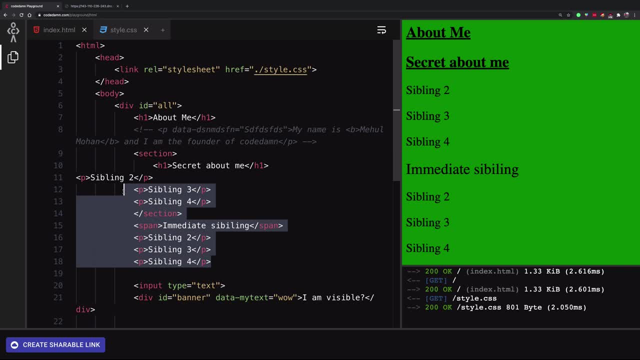 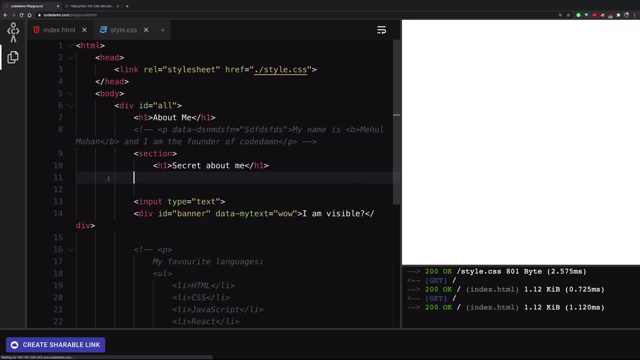 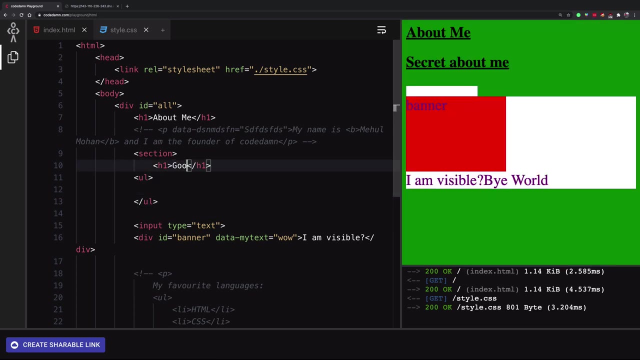 So, first things first, let me just go ahead and remove this and I'm going to add- let's say, um, I don't know, Let's just go ahead and create a list again of food. So I'm going to have something like food. 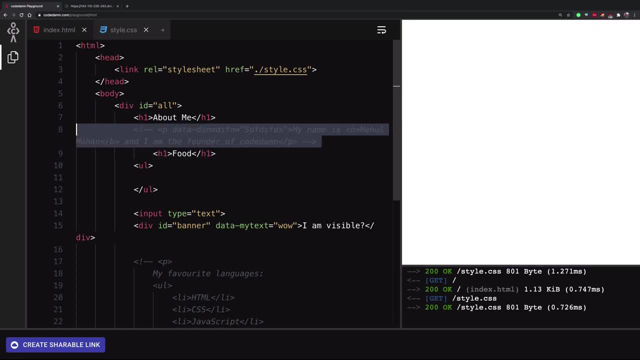 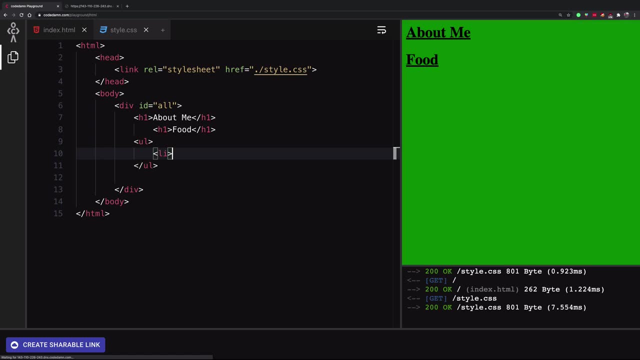 not good but food, And let's just go ahead and remove this. I guess we can just go ahead and remove all of this stuff And once you're left with this, I'm going to have an li, let's say pizza. 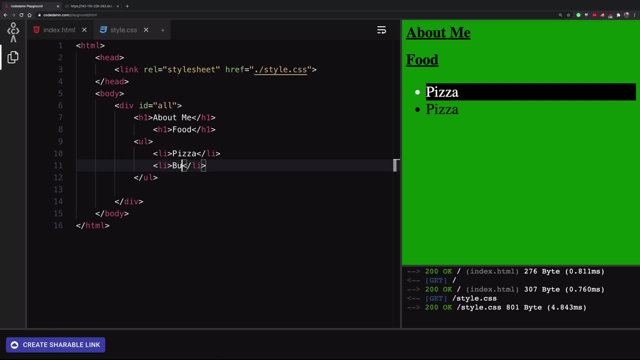 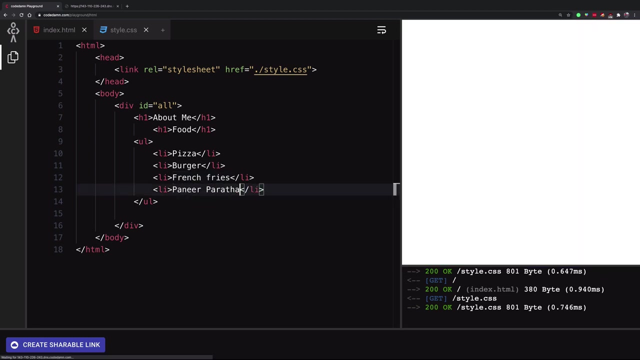 I'm going to have a li of, let's say, burger And what else? French fries And, let's say, paneer paratha. Why not? Because you're watching an Indian tutorial. So, anyway, this is a list of four foods. 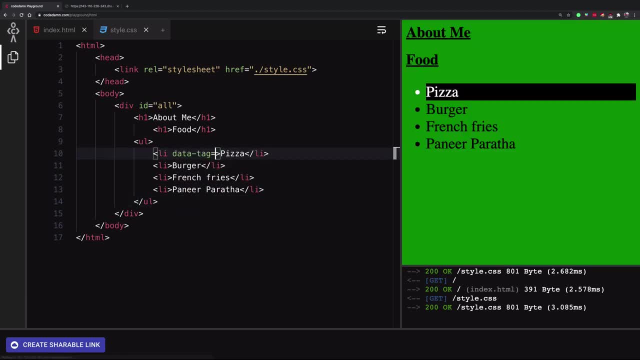 And what I'm going to do next is just going to give a data tag attribute of, let's say, of: um, let's see good spicy and I don't know, Let's see, That will probably not a good example. 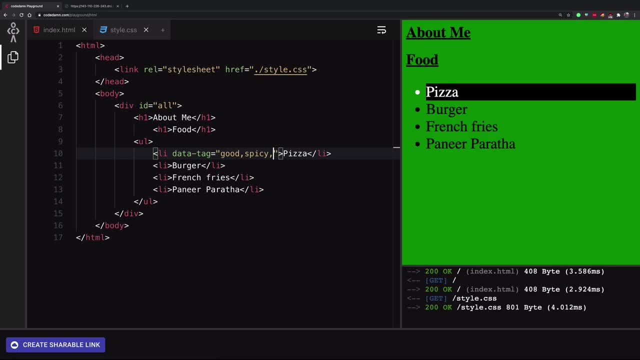 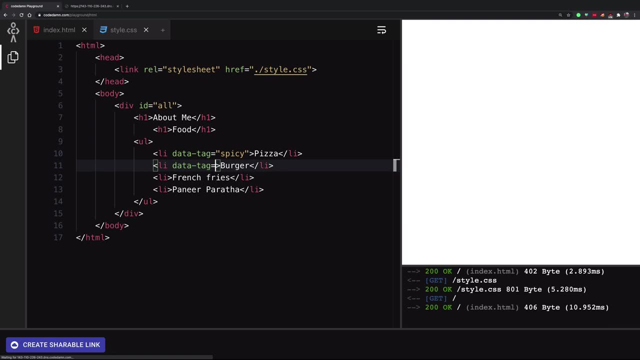 So let's just start with a spicy, or you know the variance of what I like: Huge or big data tag, lot data tag, let's say moms, right, So I'm going to give a data tag. 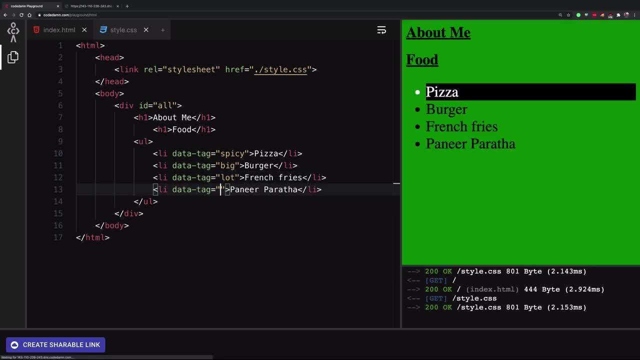 let's say, moms, right? So this means now we have these sort of selectors, these sort of attributes for these elements, and now we can target them- not only the- on the basis of. you know, just the order. 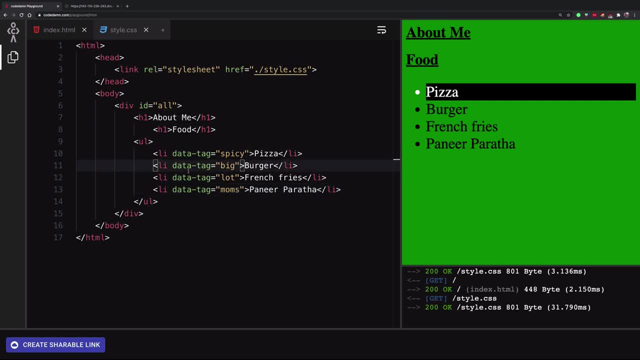 with NH, child and all that stuff, we can actually target them on the value of these selectors. And how we do that is we do that with the help of attribute selectors. So let's just go ahead and first of all get rid of this. 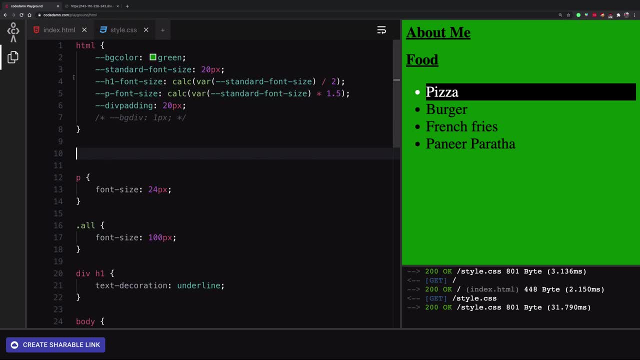 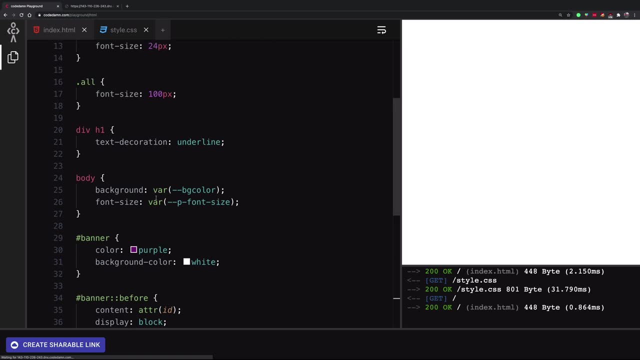 all this LI styling because we don't really want to, you know, get rid of this, all this LI styling, because we don't really want it to bother. So I want to give UL LI. 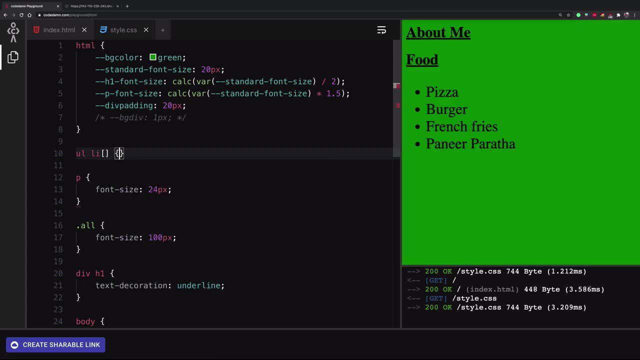 and now I want to give an attribute selector, and the way you give an attribute selector is you use these two square brackets and you write the name of the attribute- In this case it is data tag- and then an equal to symbol. 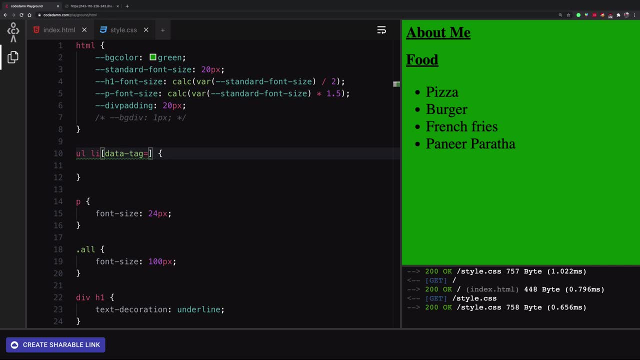 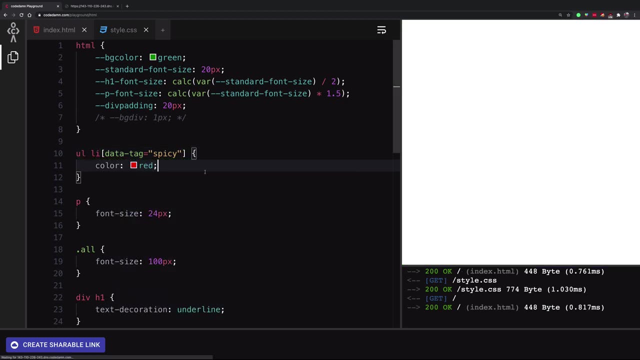 and you know you want to target the value which you want. So, in our case, is spicy, right. And now, if I go ahead and give it a color of red, you're going to see that the spicy 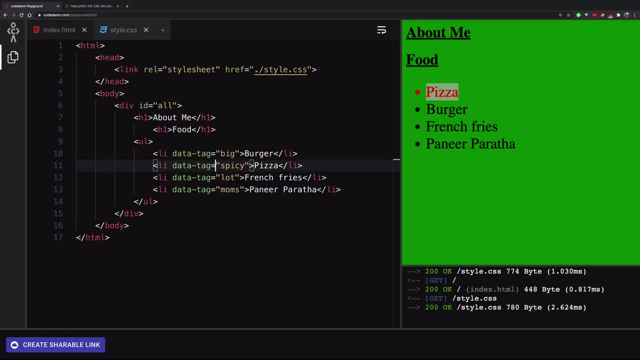 which is just the pizza turns red. And this is again independent of the order. you can move it down, you can move it up, because it is actually target, targeting on the basis of the value: exact value match. 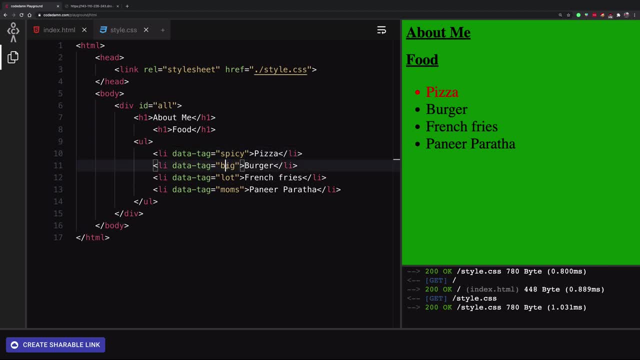 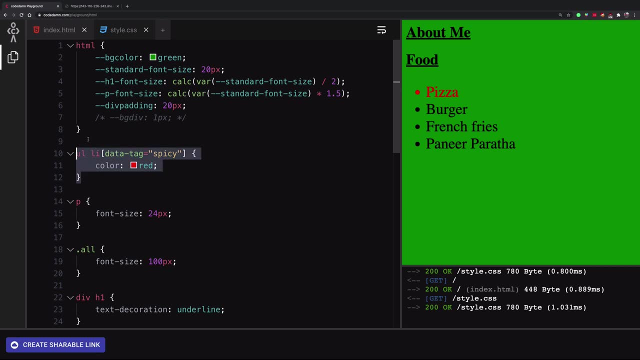 This is why you know it. it sort of works like this: independent of the order, You can also go ahead and do something like data tag. that's it. What this means is that just go ahead and find. 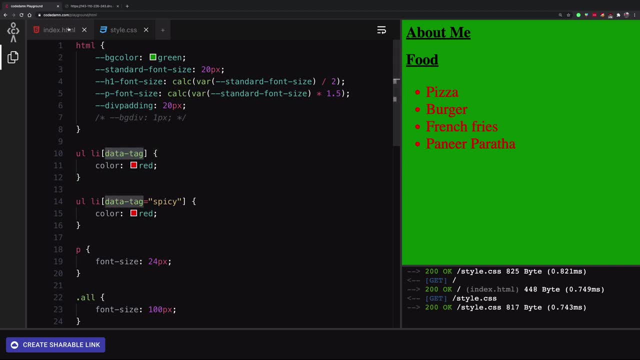 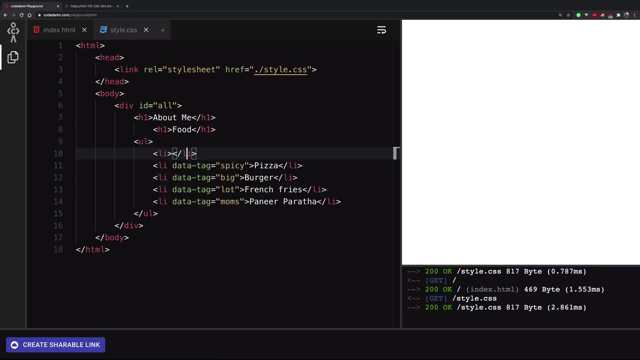 all the elements which have at least data tag attribute as as the value set, right? So if I go ahead and create an li which say something like Pepsi, right? So you can see that this is not going to turn red. 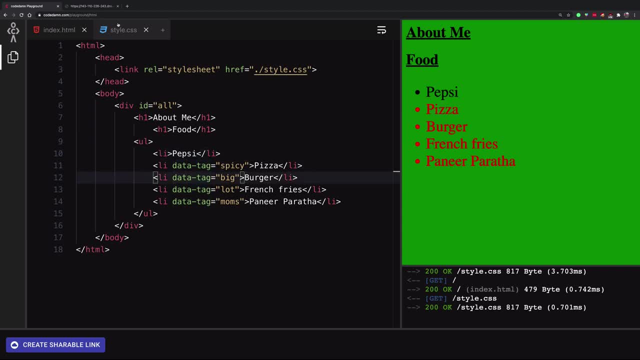 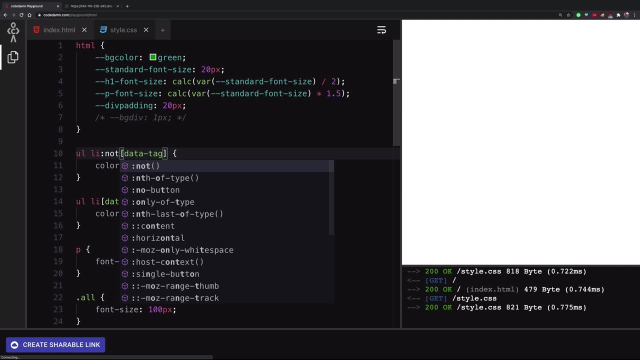 because this does not has a data tag at all. So what you can do is- it's actually again an advanced CSS selector. I'm I've not really discussed it, but you can go ahead and select a pseudo. 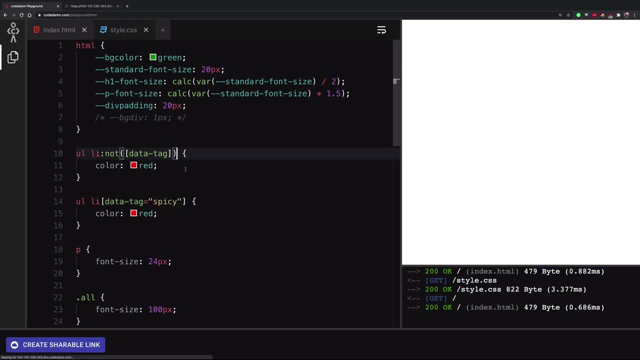 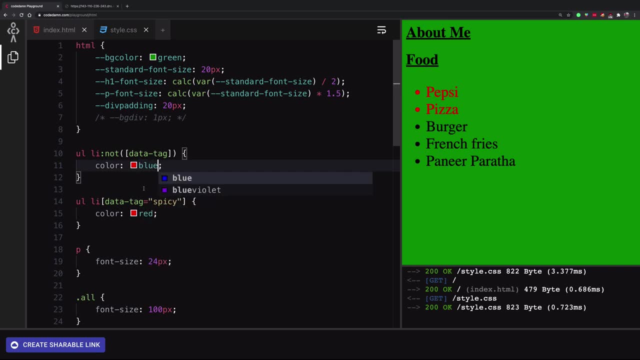 selector with not right, And I'm gonna say li, which does not has a data tag, and I'm gonna give it a color of blue because you know we are getting a confusion. So what this means. 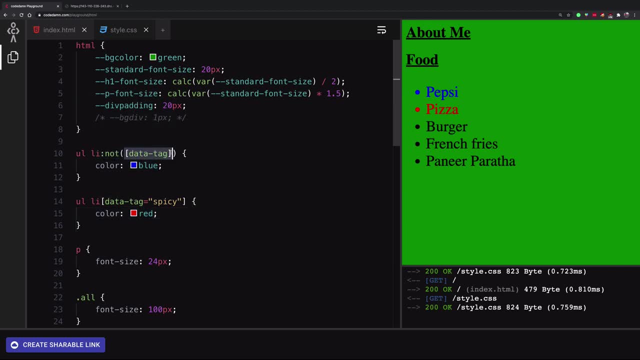 is that hey, go ahead and find an element which does not has an attribute named data tag, right? This meant this meant that li must have an attribute data tag. this not right here. 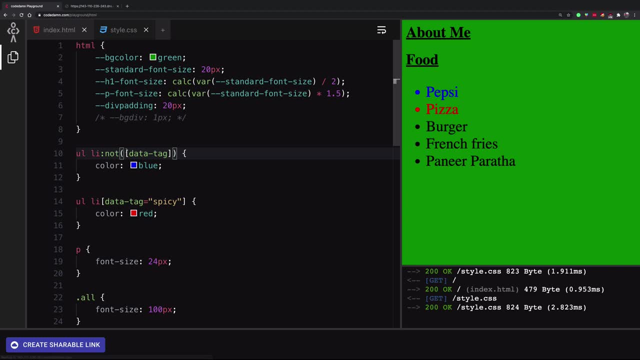 is again a special sort of selector. we could probably go ahead and discuss it in depth, but this is a special sort of selector, which means that go ahead and select every element which does not match this rule. 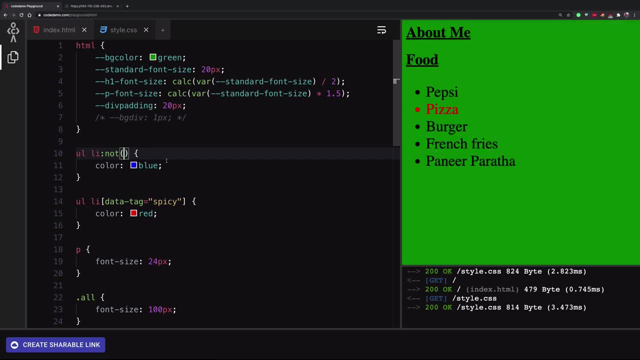 and it's not just restricted to the attribute selector. you could pretty much write anything right here, like an ID of li tag, or maybe like a class name, you know, or just like I said, attribute. 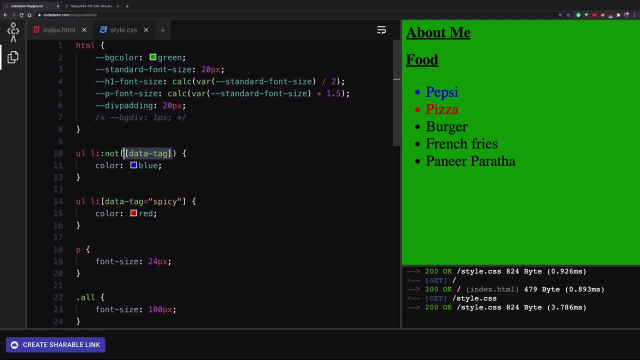 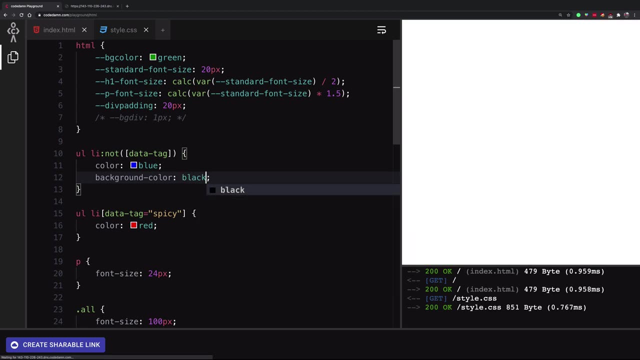 so anything would work. but anyway, with that being said, once you have written something like this, you can have this or, you know, you can just give it a background. you can basically play around with it a little. 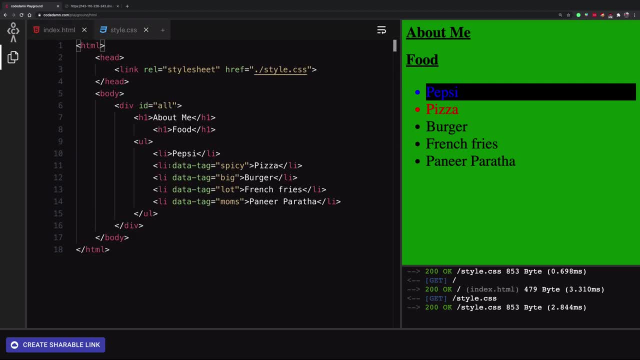 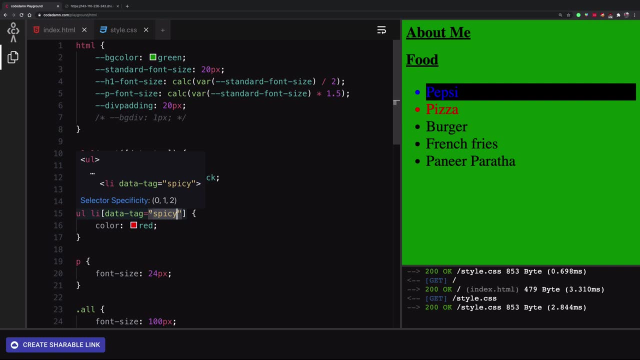 if you want right. so that's how it works. now, once we have discussed like the exact match, what we can do is we can also target elements, which starts with a particular value. so in this case, 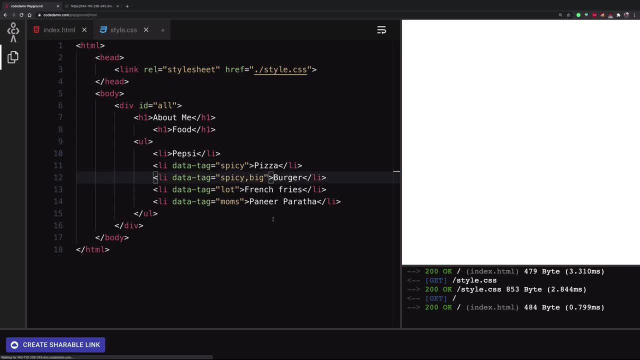 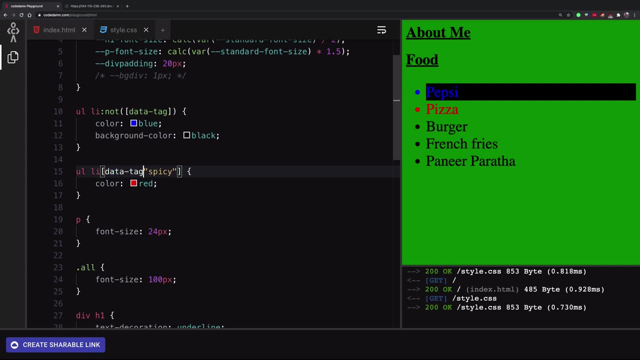 let's see. let's say this: I want spicy and I want pig, right? so what I can do is, instead of targeting just spicy, I want to say: every element which starts with spicy should be targeted. 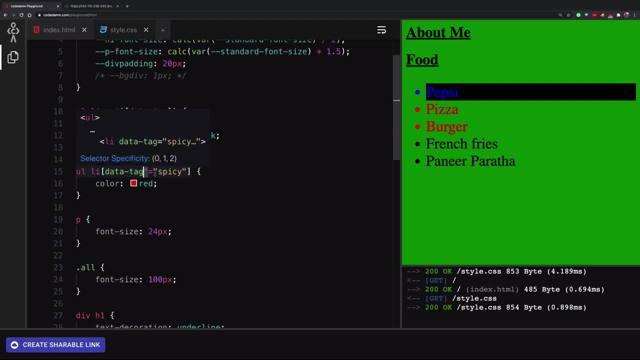 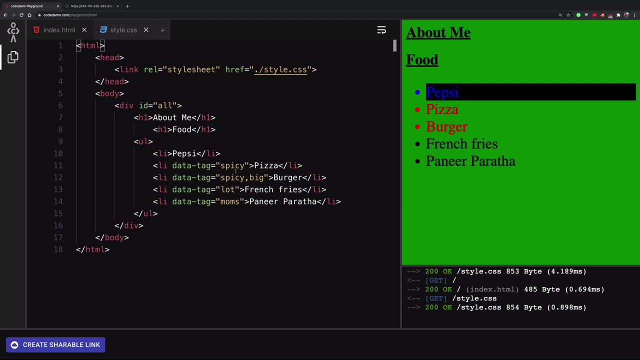 so in that case I'm gonna make use of this carrot symbol and then an equal to sign and then I'm gonna write spicy. now you can see pizza and burger get highlighted as red, because they both start with spicy. 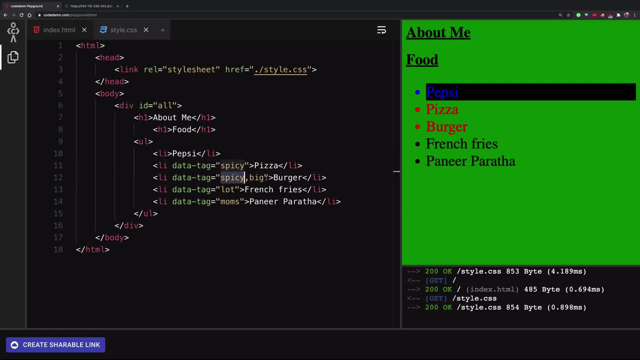 this one has just spicy and this one has spicy and big, right, but this is gonna create a problem for you. if you have an order, something like big and spicy, right, because now it starts with big. 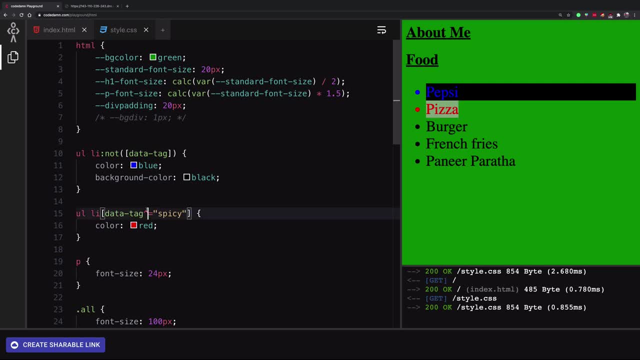 so it not, it will not be targeted. so there's another way. you can actually go ahead and put a star right here, which means that, hey, just go ahead and find every element which contains this word right. 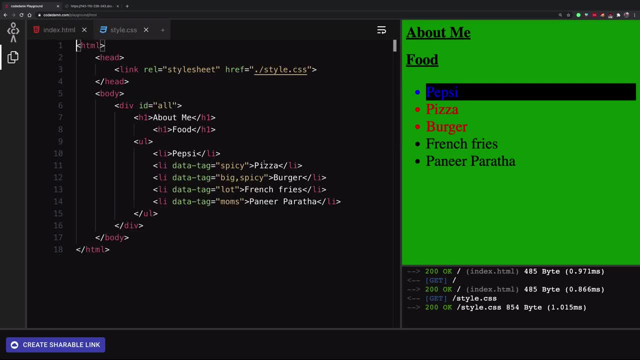 irrespective of whether it's at start, middle or end. it should just contain, so you can also have big spicy and you know, salty or whatever, however you like your burgers, but you know it'll still match.